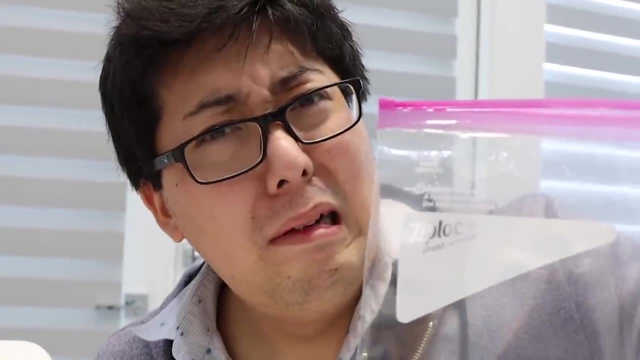 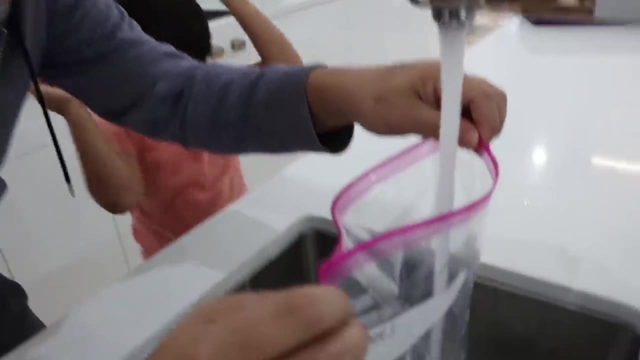 That's a true fact. Uh-huh. First, let's put water inside the bag. Okay, let's fill it up. Hopefully, Ryan's telling me the truth, because I don't want a big mess Now. we're going to put in food coloring for fun, I'm going to use blue. 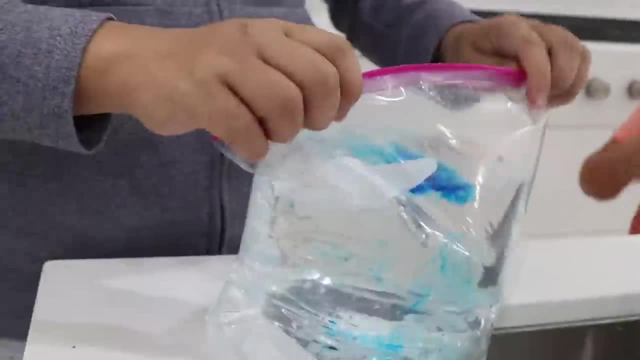 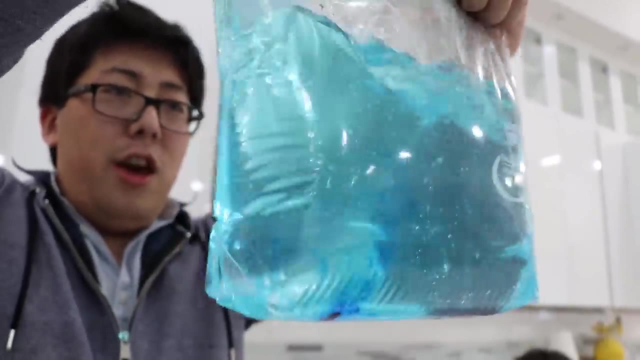 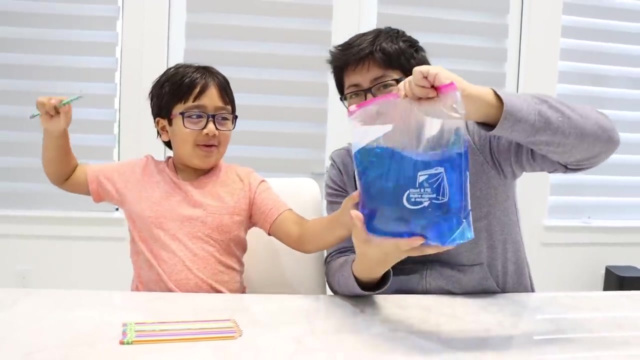 Alright, maybe one drop. Look at the color Nice. look at the ocean Next up. we're going to need a sharpened pencil. Don't forget to ask your grown-up for help. Alright, here we go, We're going to poke it through. 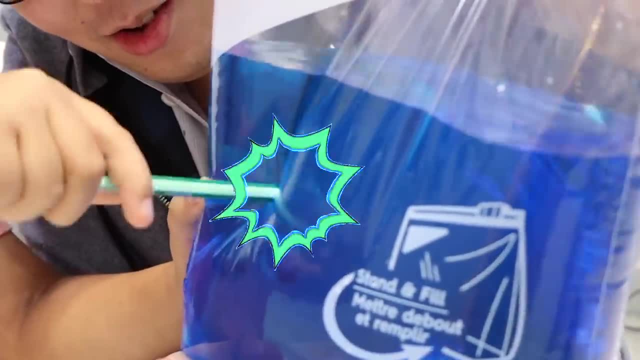 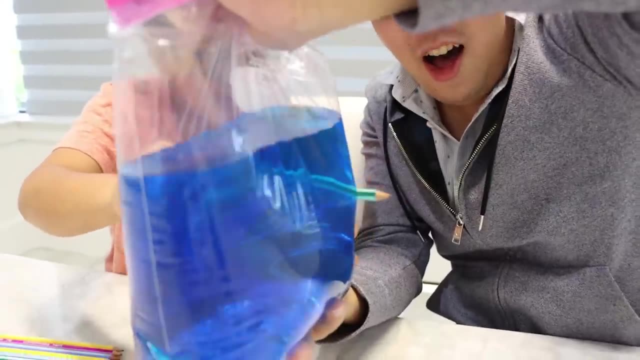 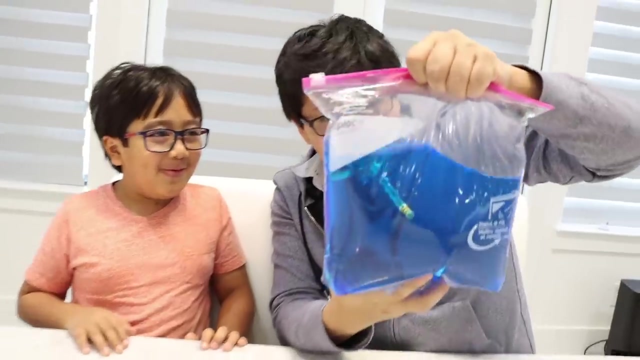 Is it going to work? Yeah, it's not going to make a mess. Oh, it's poking through. Look the pencil's inside. Oh, no way, guys, There's no water coming out. What? Why is it like this? 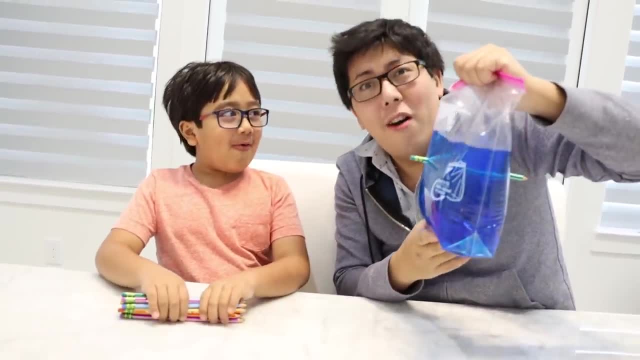 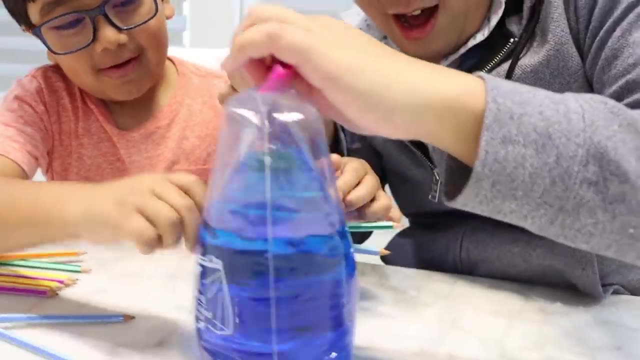 How's it working? Ryan, Whoa, Do more, Ryan. Okay, I'm going to do a bunch of pencils: Whoa, Whoa, What. What about you try, Daddy, Can I do it? Alright, let's see, I'm going to do it at an angle. 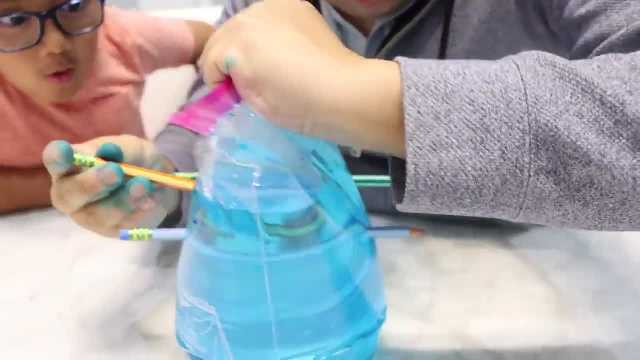 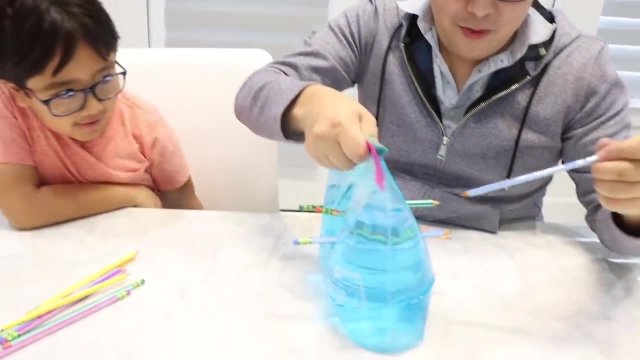 Does it work? Whoa, Whoa, it works. Whoa, That's cool. Now you do it up and down. Alright, I'm going to do it from the opposite direction: Up down, Whoa, Whoa, it's working. 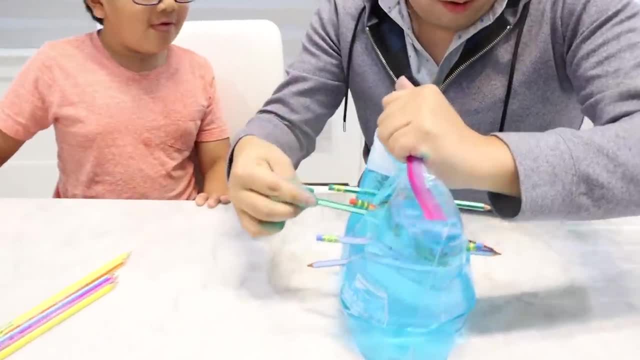 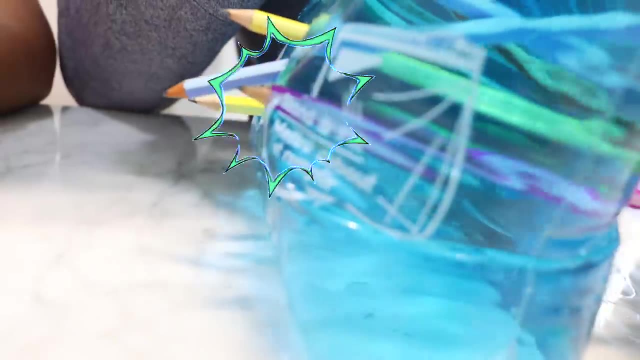 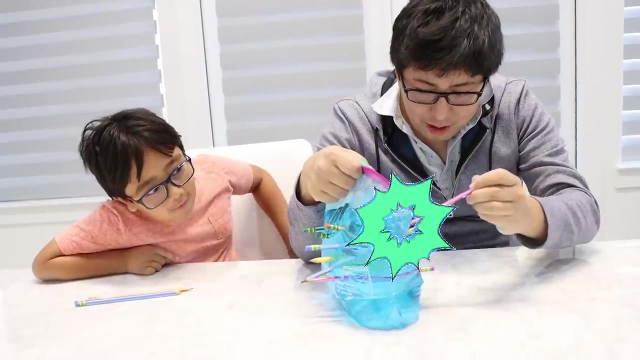 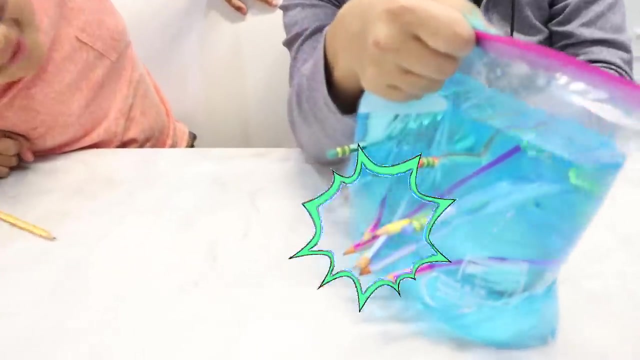 Yeah, it is. I'm going to do more. Whoa, Whoa, Whoa, Whoa. There's so many pencilss. All right, I'm going to keep going. Let's see if I can do all of them. 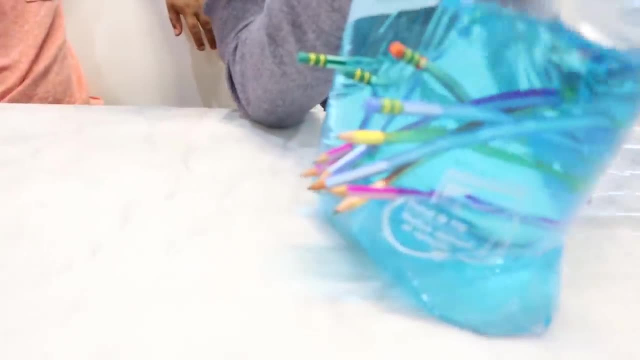 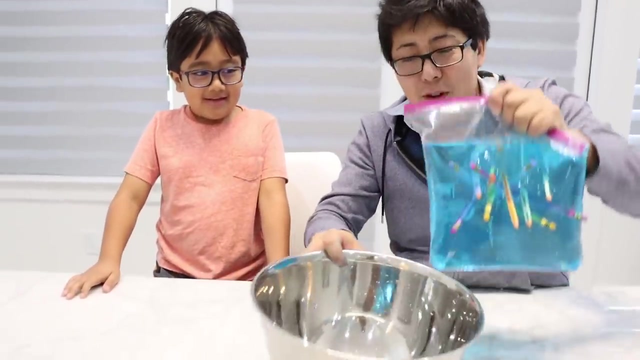 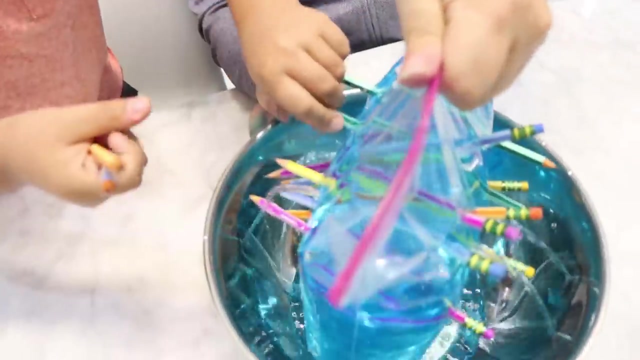 I think I poked too much. Daddy, what about we take out all the pencils and see what happens? Good idea, Let's put them in the bowl. All right, Let's see what happens. Whoa Water's coming out. 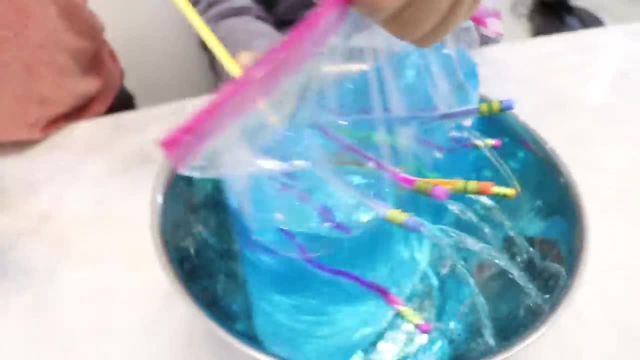 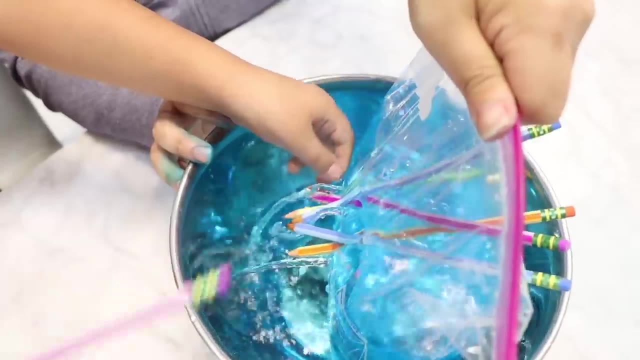 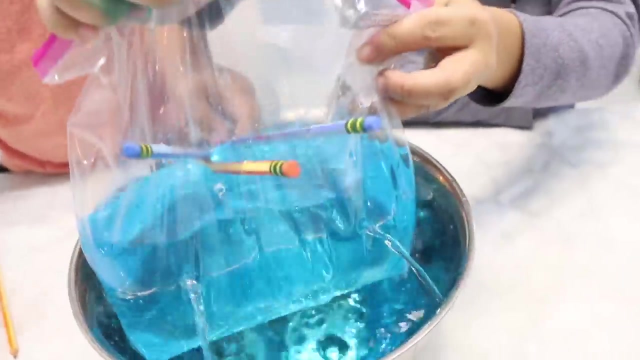 Water. There's so much water, Water, Waterfall, Water, those- Whoa look at that. Well, there's so much water coming out. It's like a shower, It's a waterfall of water. Whoa, there's so much. 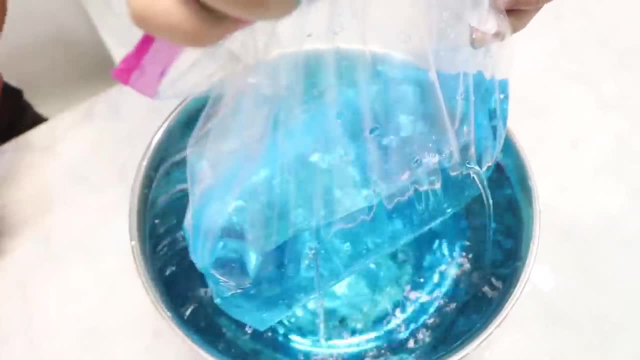 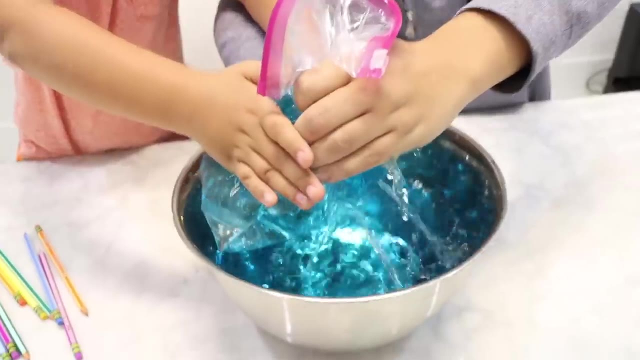 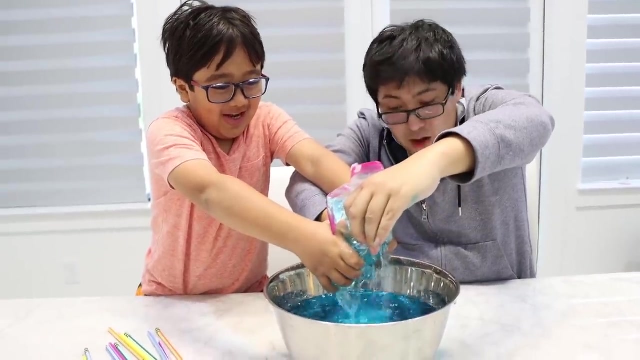 I am in a spree. I'm in a spree. You see that I'm gonna squeeze, get all the water out. Ah, Ah, Whoa, whoa, whoa, whoa, whoa, whoa, whoa, big mess. 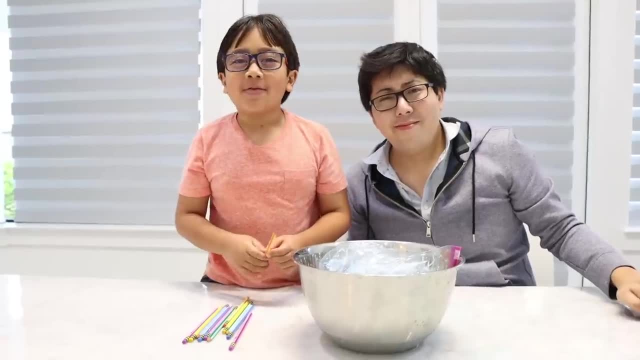 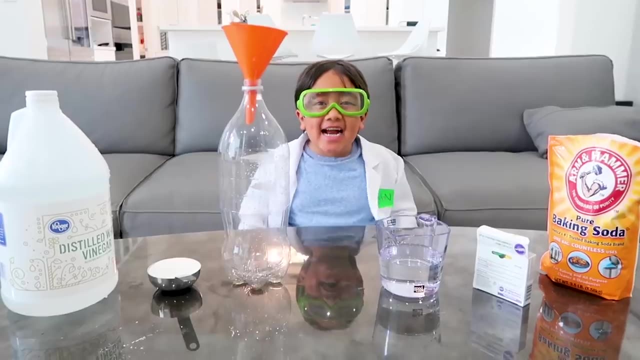 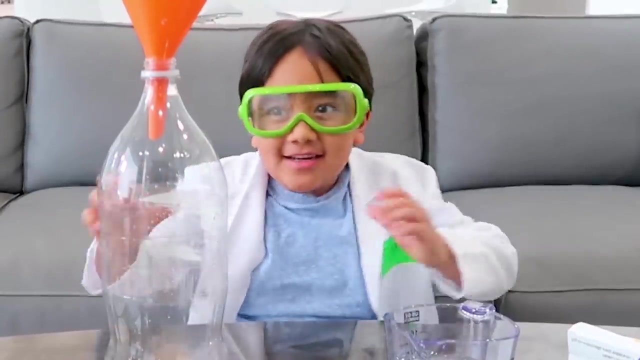 Wow, it almost filled up the whole thing. Thank you for watching a science video about pencils and poking into a bag. Hey guys, today we're doing the baking soda and vinegar science experiment, But first pretend this is a volcano- Whoa. 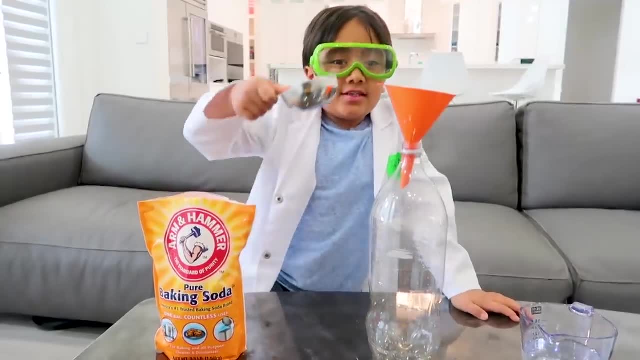 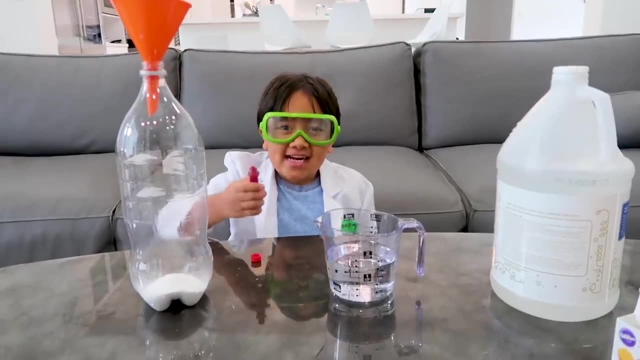 First, you're gonna need some baking soda, So we have to put it into the funnel inside your water bottle. Whoa, whoa, whoa. Okay. next you're gonna put your food coloring into your vinegar, and I choose red. 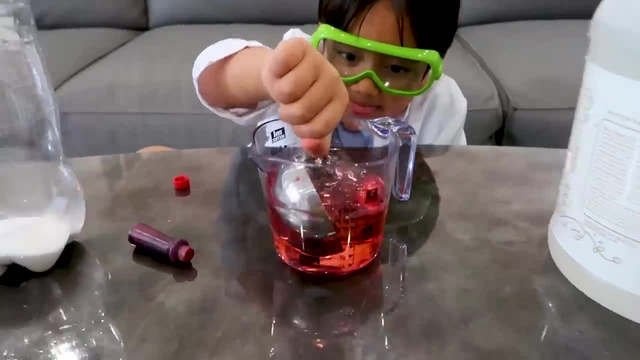 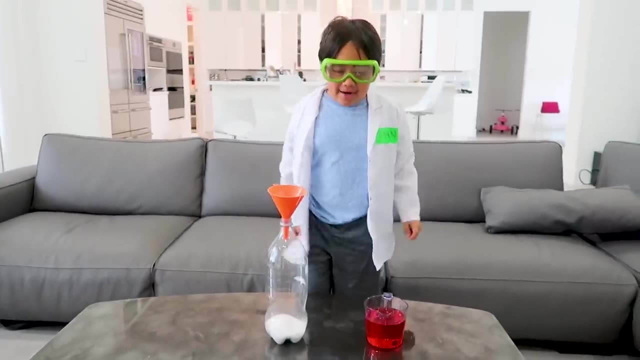 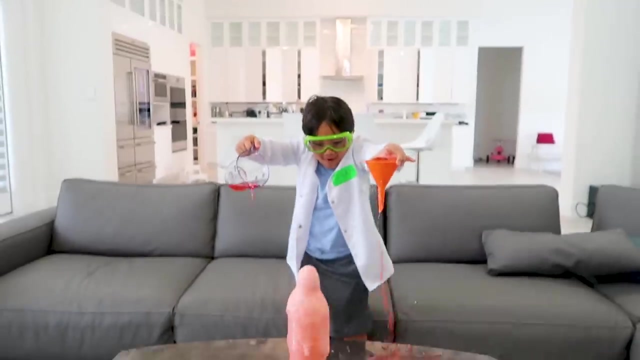 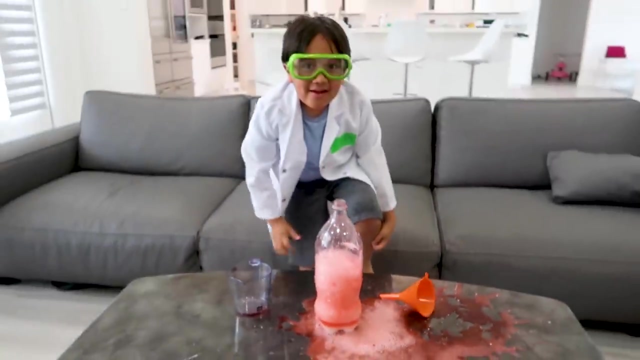 A little bit more. Okay, guys, get ready for an experiment. John, Remember, ask your parents for help. Whoa, whoa, Oh, Whoa. that came out. That was so cool. That was really fun, but I wish it was a volcano. 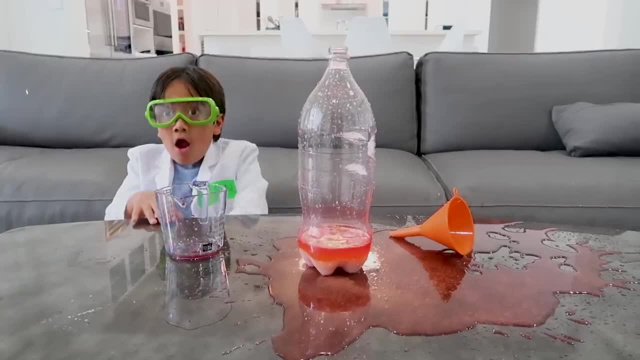 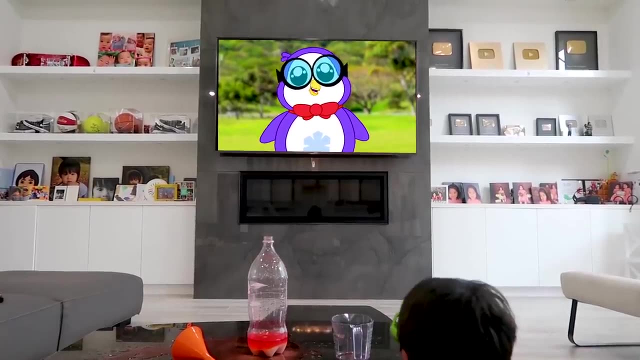 No, Oh, Peck, Hi, Peck. Gosh Ryan, did you know that you can make a volcano out of paper? What You can, Of course you can. I'll go make one for you. Okay, I'm gonna build a Lego robot. 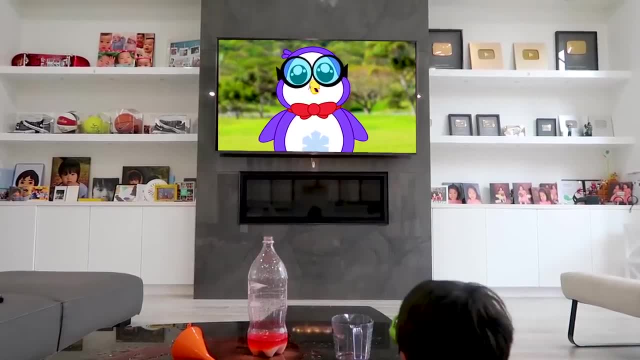 It's gonna be my best friend. All I need is the last piece for the head, and oh, it's so cute. Whoa, whoa, whoa, Uh-huh, Peck, Peck, Peck, Peck. 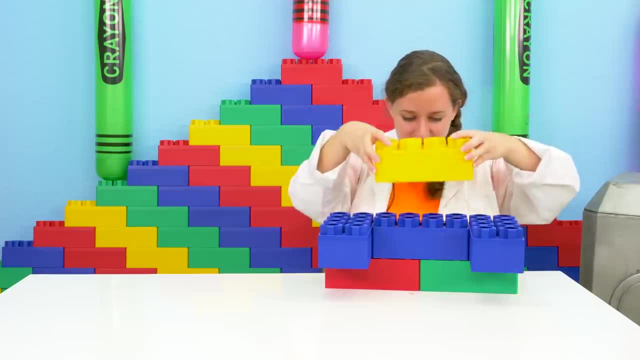 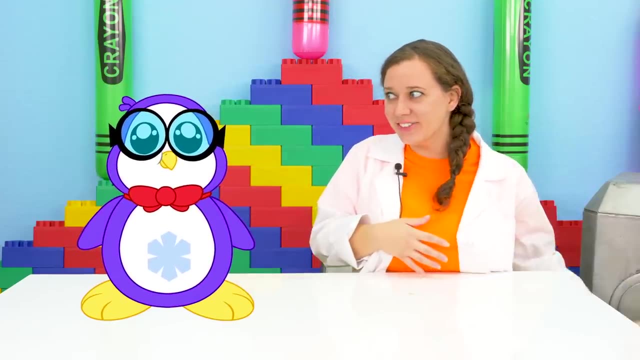 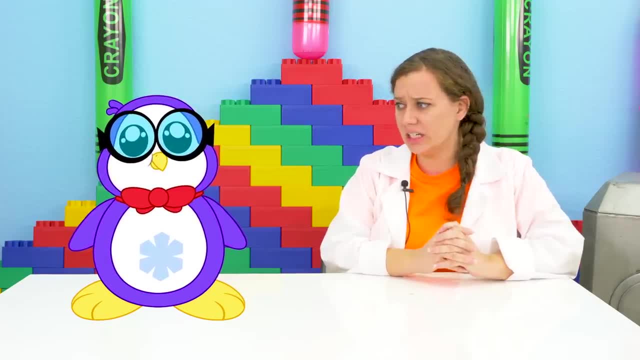 We got a new science experiment for Ryan. It's gonna be a giant volcano. A giant volcano. Well, uh, what do we need for that? First thing we will need is a giant box. A giant box- There's definitely one around here. 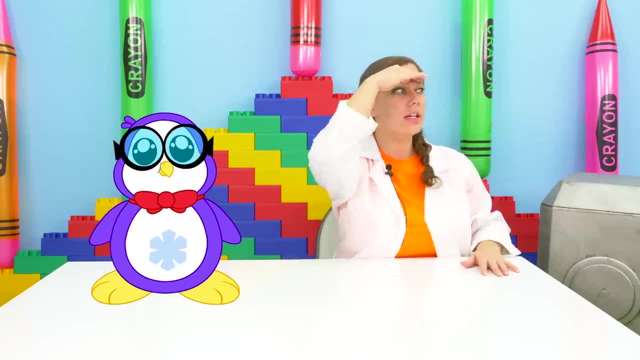 Let's see. Oh, over there by Combo, Hey Combo, pass the big box. Huh, Oh, this box. You got it. Bri, Hey Debra. I got a new science experiment for Ryan, Let's see. 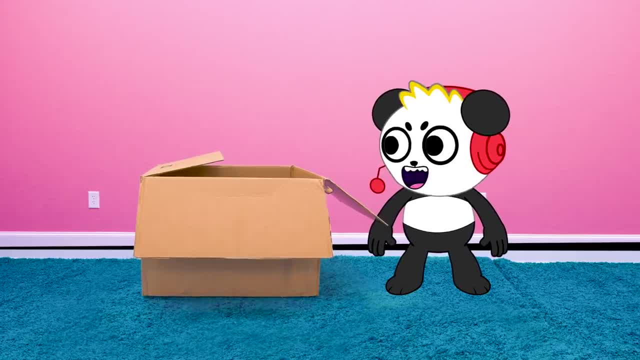 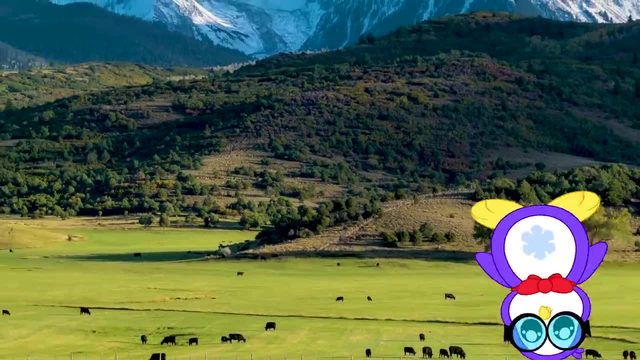 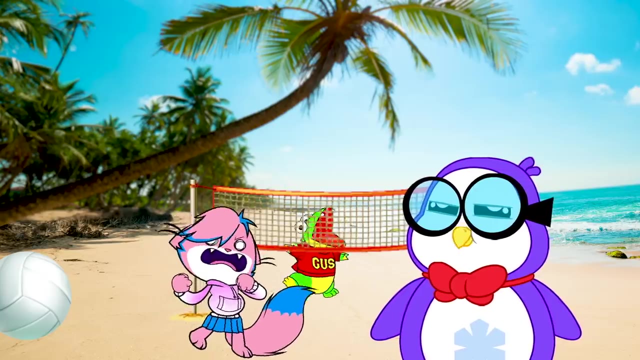 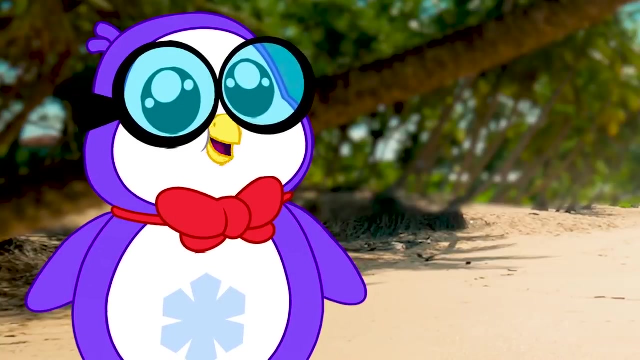 Oh, over there by Combo. Hey, Combo, pass the big box. Huh, Oh, this box. I'm a little teacup shark. whoa, yeah, perfect. this place doesn't seem too familiar. what's that? looks like there's a volcano nearby. let's go investigate. whoa, this box is huge. 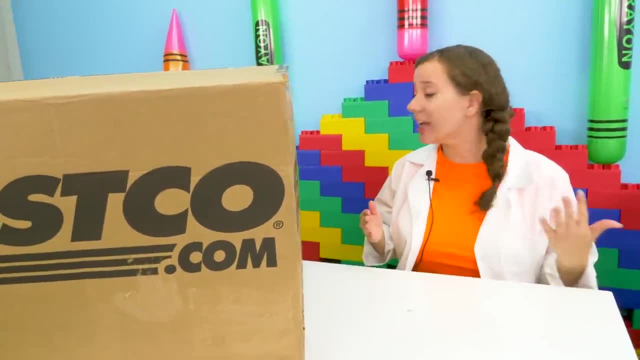 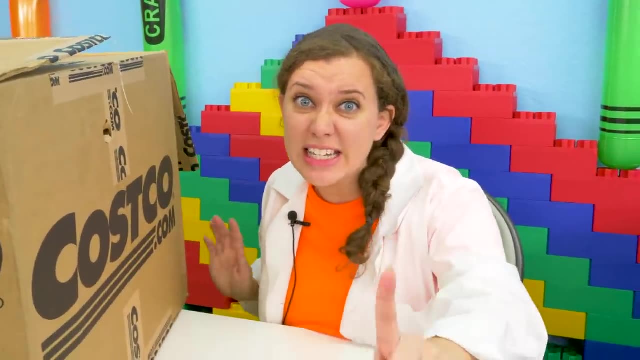 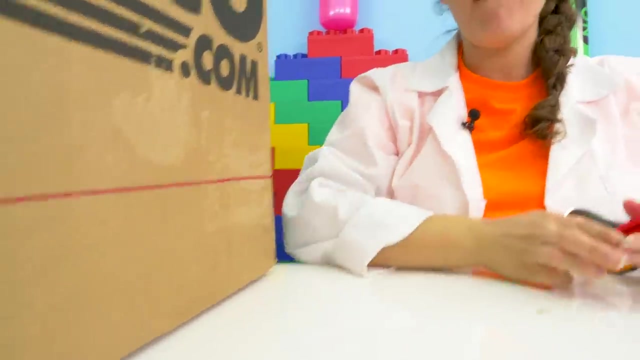 and it is going to be the perfect base for our volcano, don't you think, pet Peck? where did Peck go? oh well, let's get started. the first thing we need to do is cut this box down, so I finished marking my line where we need to cut. it's about 4 inches. 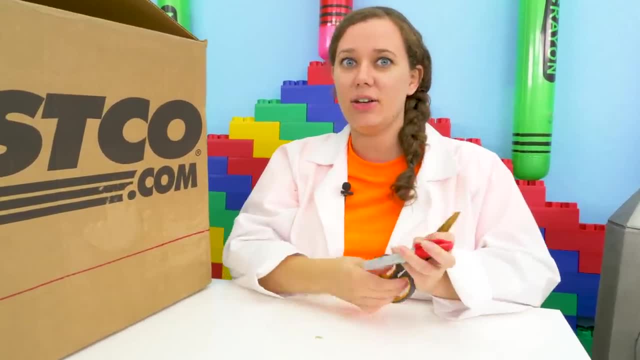 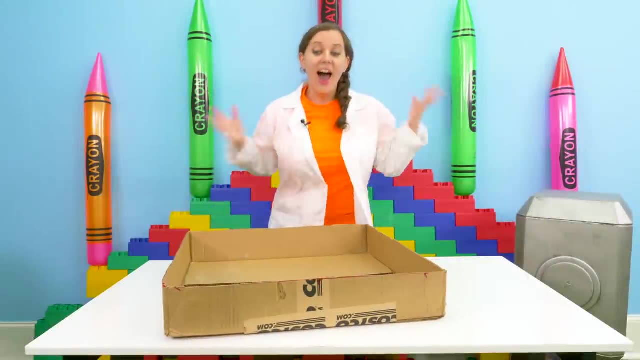 high, which I think is going to be a good height to keep all the lava inside. so now all we need to do is cut, and once we cut the box, it should look like: and there it is. that is the perfect size for our base. look how big it is. and now we need to cut. 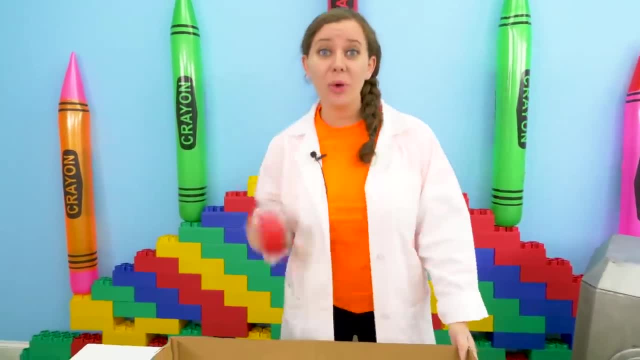 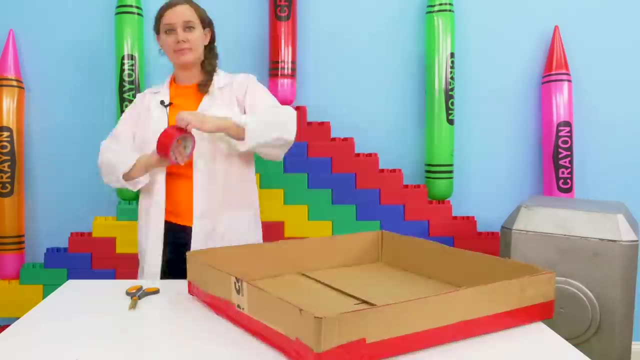 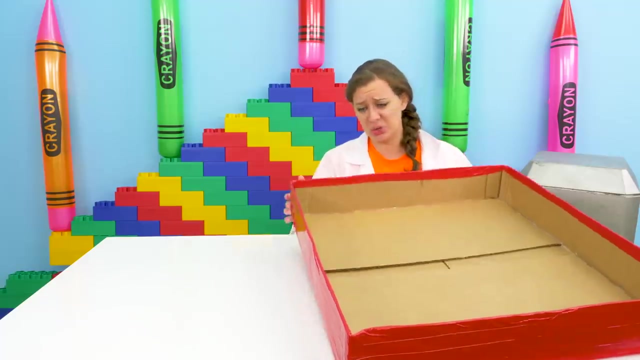 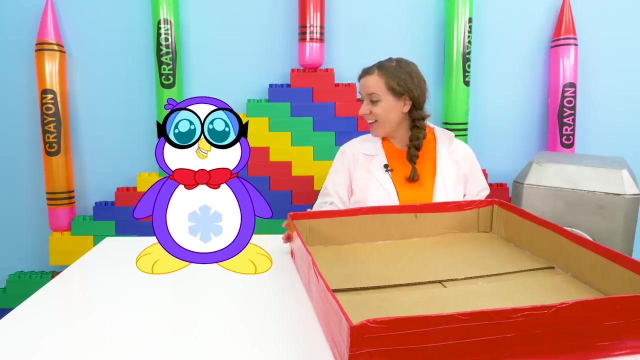 this now to make sure that our base is good and strong. we're going to use duct tape. Well, the box looks great, but how do I build a volcano Incoming? Oh Peck, there you are. I just got back from gathering research data. 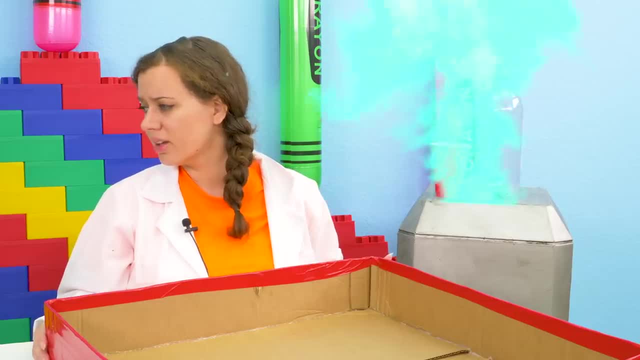 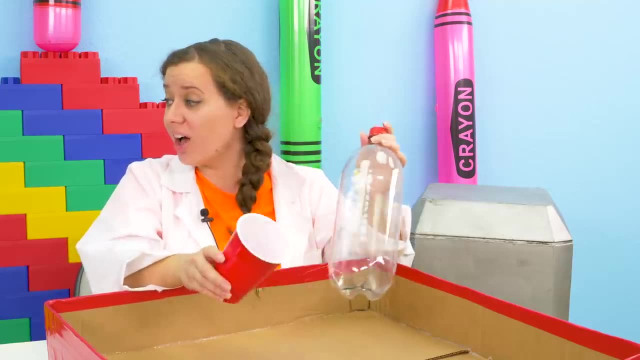 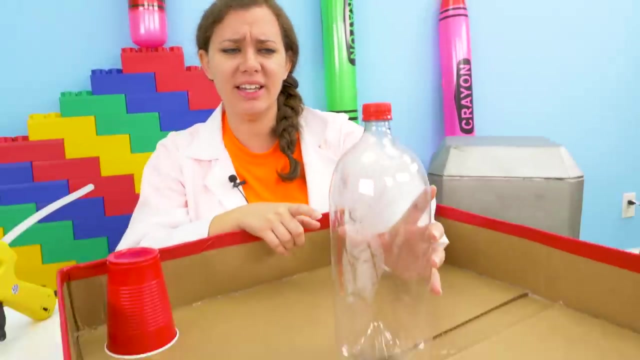 First gonna need these: A bottle and a cup. I think we can use this for the center of our volcano, Precisely So. this bottle is gonna be perfect to put all of our ingredients in for the lava, but I think it's a little too short. That's why we 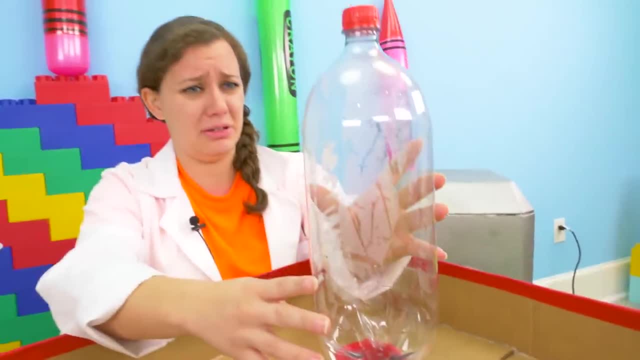 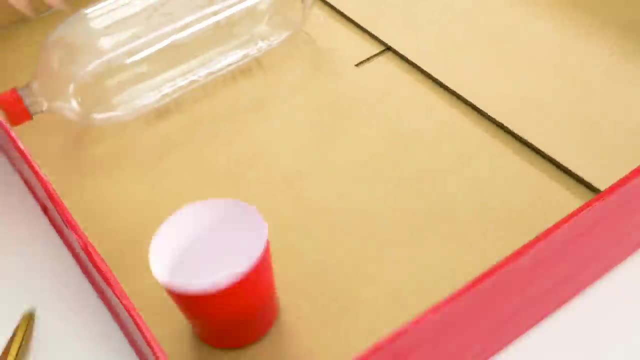 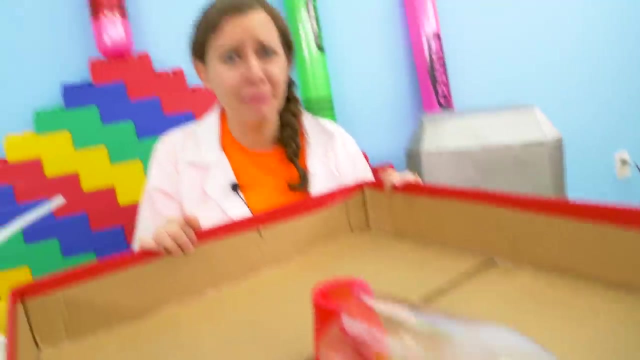 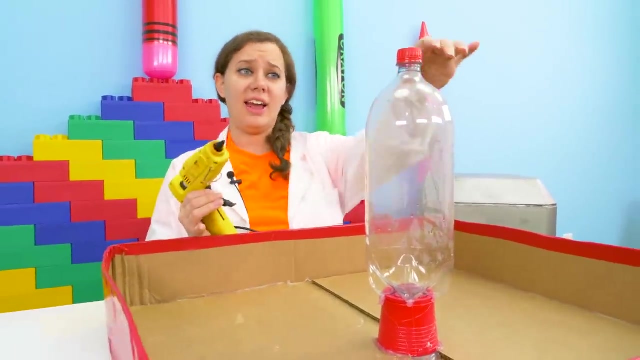 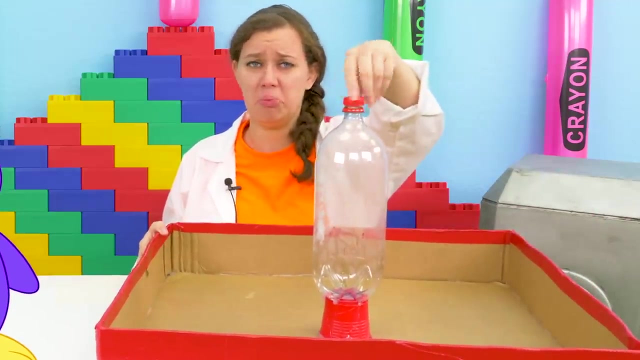 have this cup. I think that might be a little too tall. We can work on this. Oh, that is the perfect height. Maybe we should glue it in place. Okay, Just a little bit more glue, and I think that should do it. I don't think it's going anywhere. Okay, our bottles not going anywhere, but we 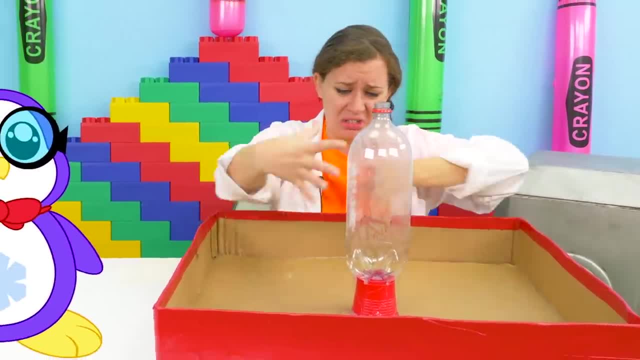 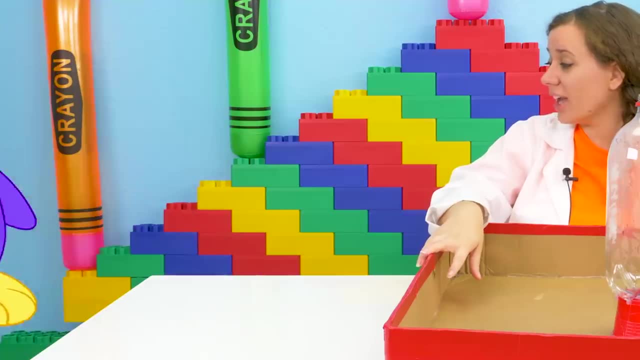 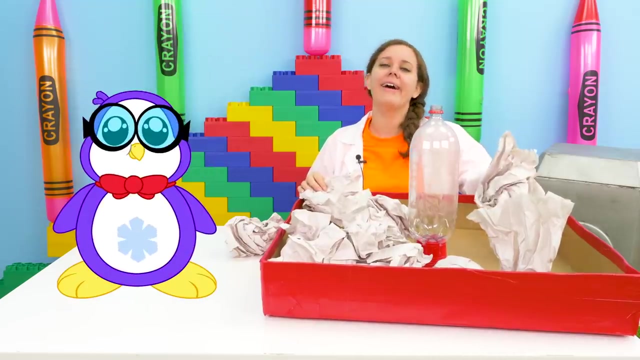 don't need this cap. It doesn't really look like a volcano. We need something- I don't know what We have- to build the body Boop. I know what'll work. Okay, Trash Paper, That's a great idea. 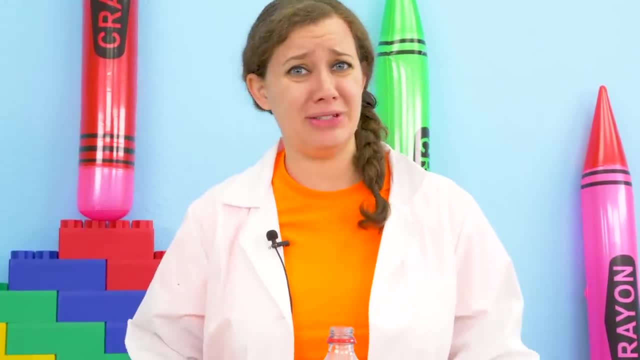 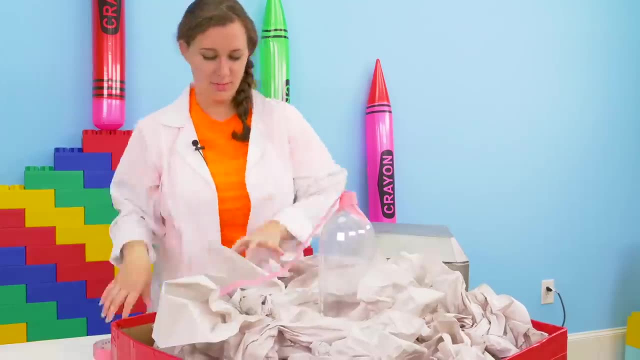 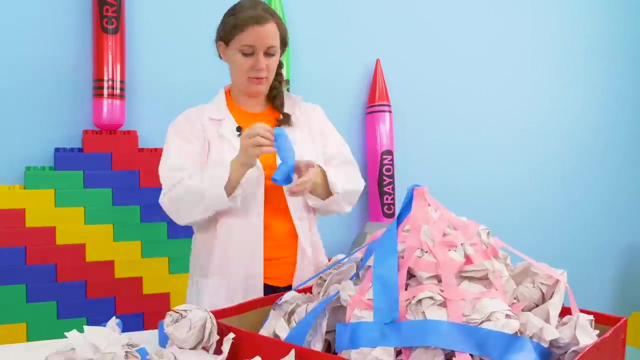 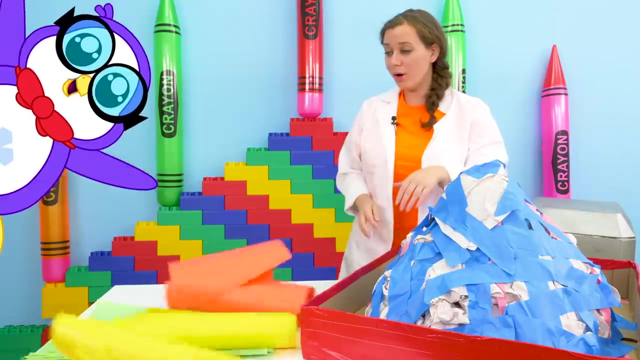 So we're making the shape of our volcano. It's kind of a mess right now, so we're going to use tape to hold all of this together Now to form the body of the volcano. with some tape, More paper, Whoa. 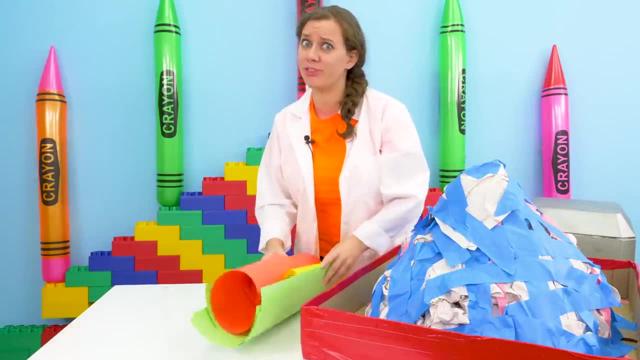 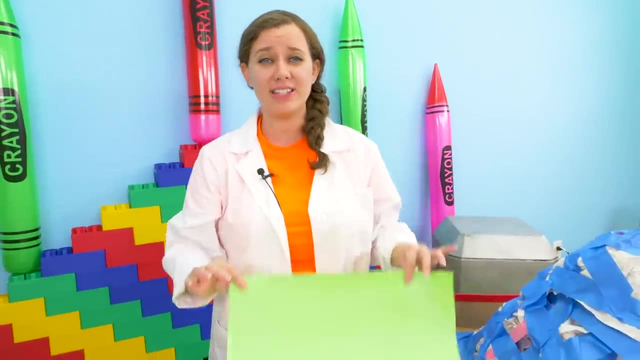 Wow, Peck, you found a lot of paper. This is going to be perfect. So the first thing that we need to do to start paper machining this giant volcano is: we need to take all of this paper and tear it into pieces that we can actually use. 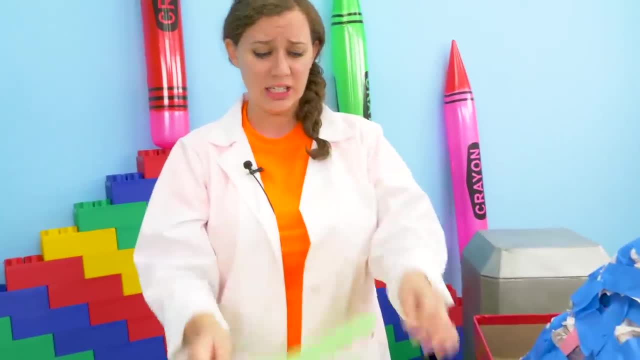 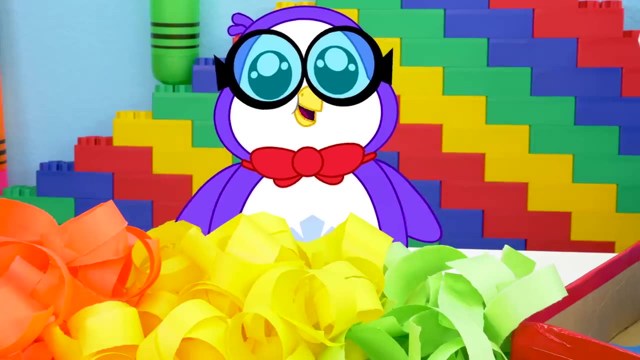 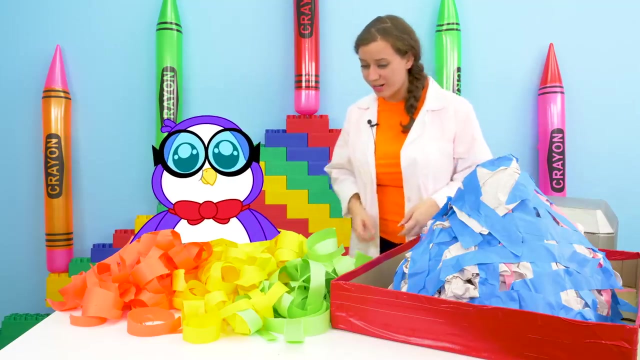 So something about like that, But we're going to need a lot. This guy is very big, so, Yeah, This ought to do the trick. Rip the paper, Whoa Peck. great job, This is a lot of paper. 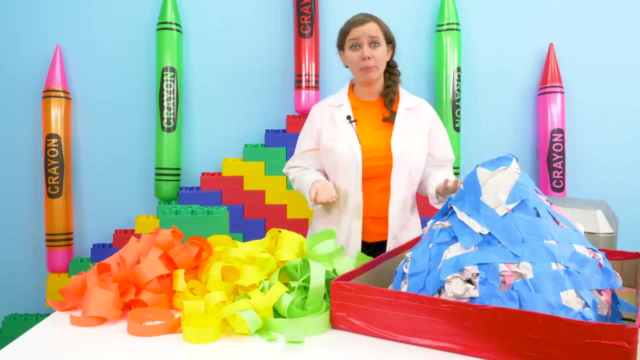 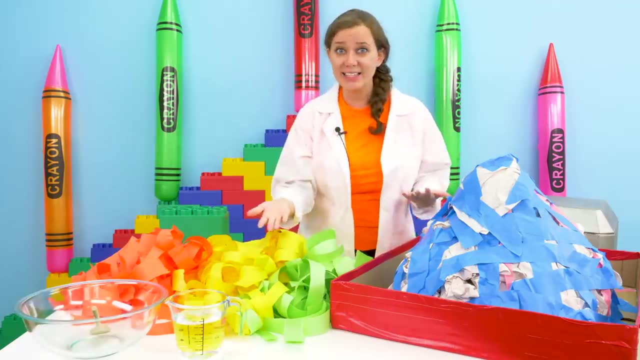 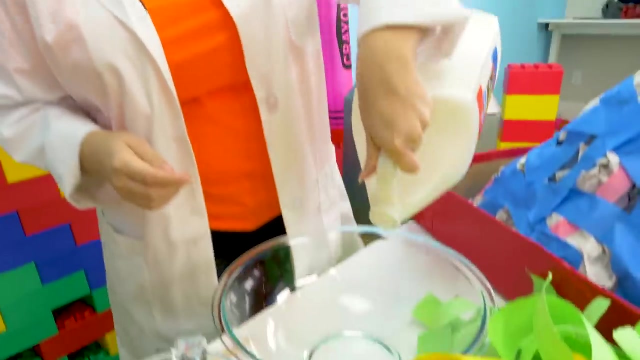 What else do we need? Well, to make paper mache, we need paper, which we already have, And then we need a bowl, some water and, the most important part, glue. So this glue is way too thick. So the first thing we're going to do is add glue. 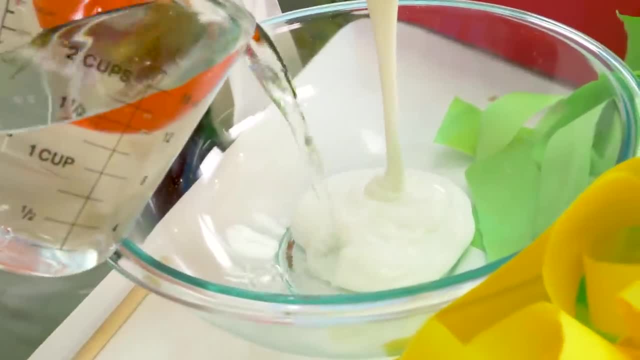 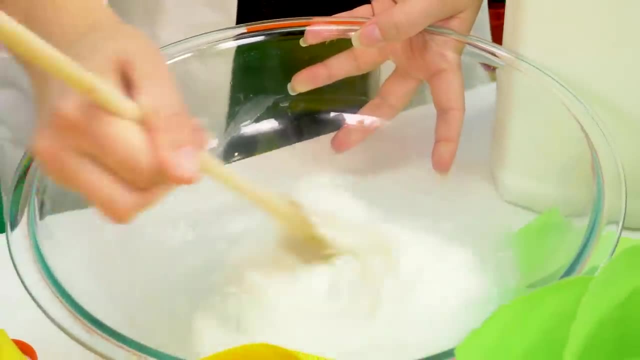 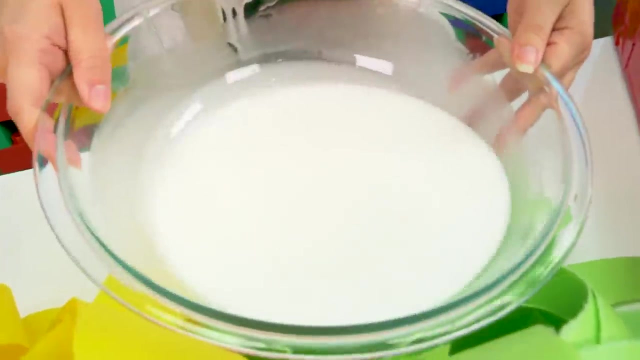 Then we're going to add water and stir it all together to try to thin it out so we can put it on our paper. Now all we do is stir Or agitate, Agitate, agitate, And when you're done, it should look something like this: 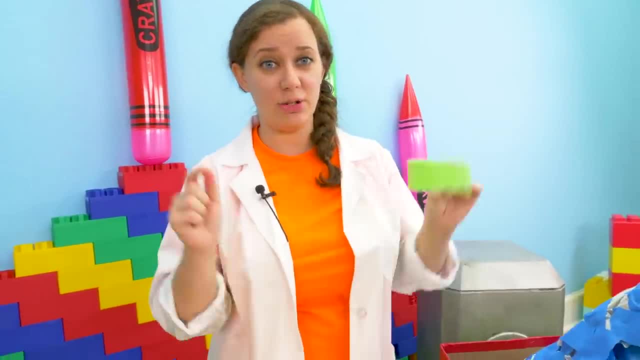 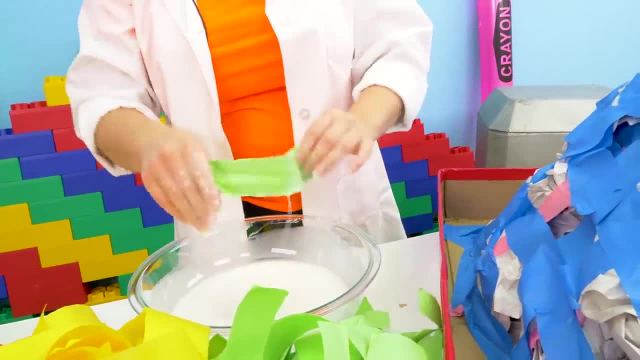 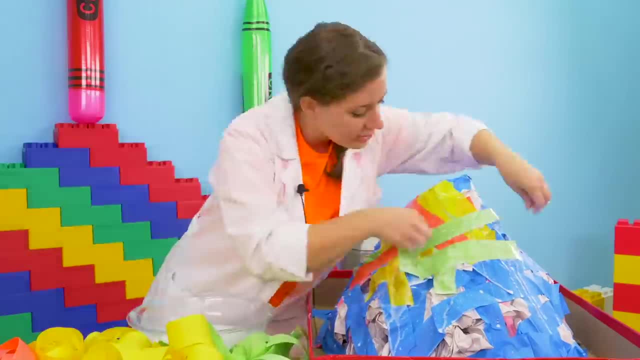 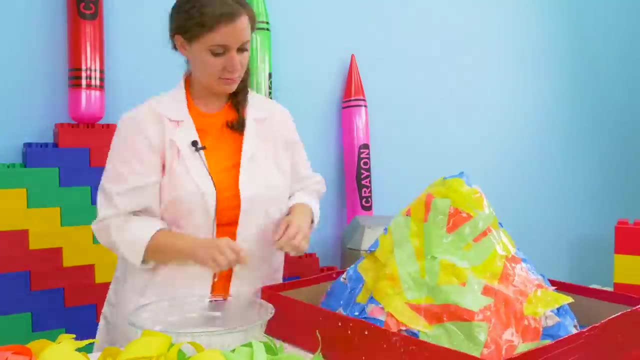 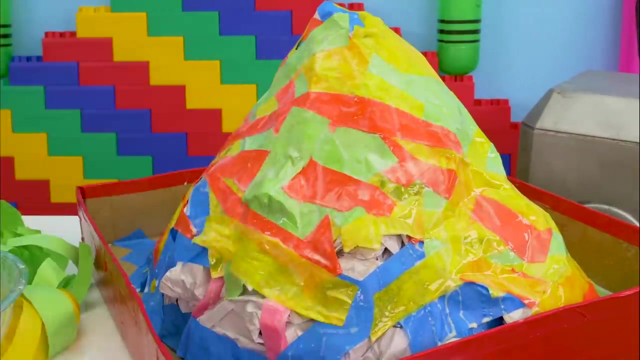 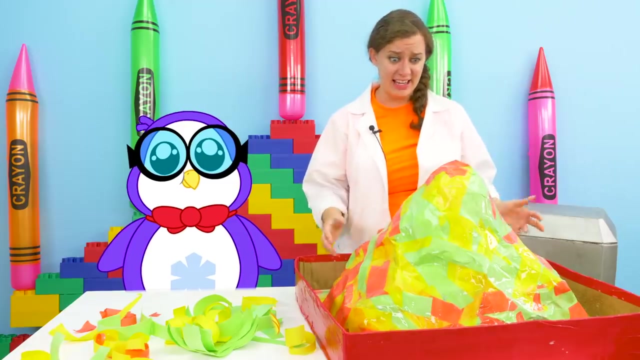 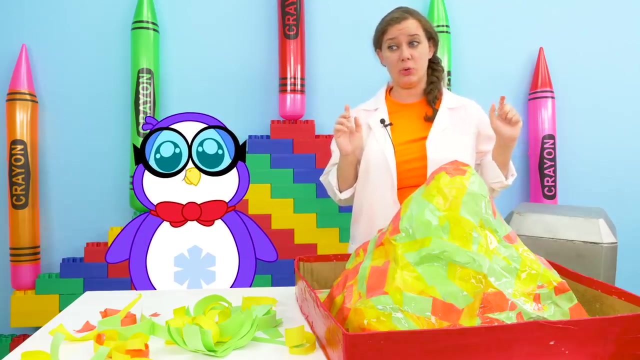 Slimy. Now the hardest part. We have to wait for this to dry. The volcano will take a while to dry. Let's go wash our hands. Ugh yeah, I'm very sticky, So we'll meet back here later. 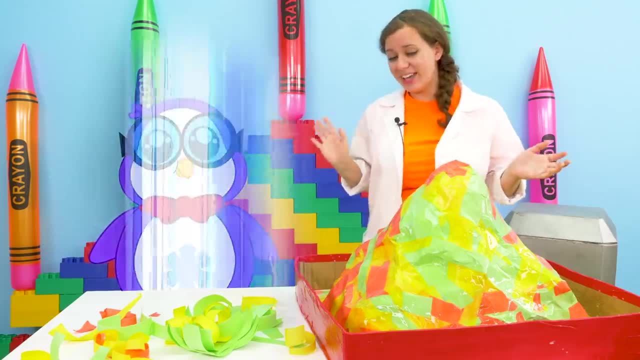 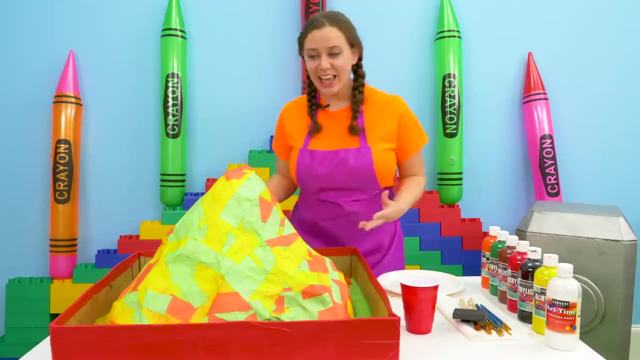 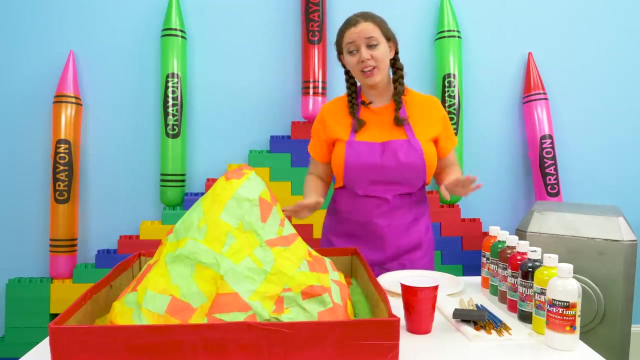 Yup, I'm going to go gather more research. Bye, Oh shh. One day later, Whoa, It looks so good And it's really dry. Let's see. It's definitely hard and sturdy, Ready for paint. 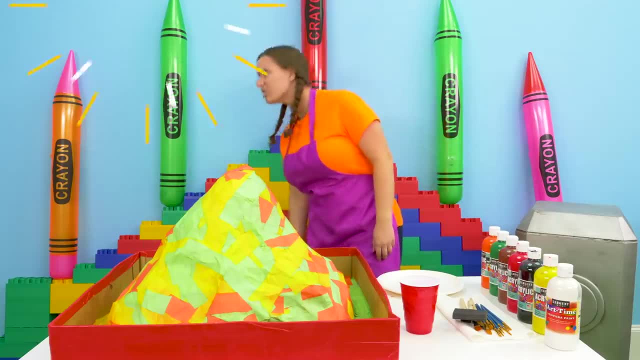 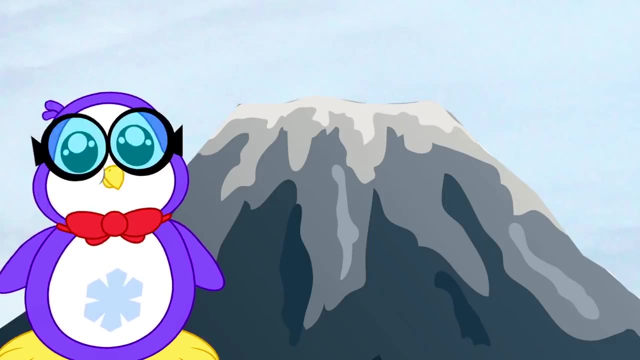 But where is Peck? Peck, Are you free Peck? Oh yeah, I'm at a real volcano And I think we need to use a gray paint. Well, we can definitely make gray Peck, But just make sure you stay safe, okay. 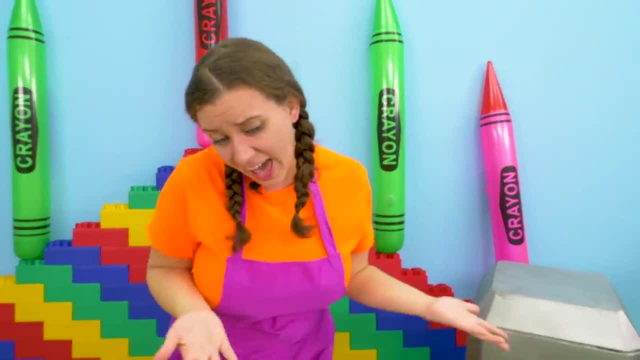 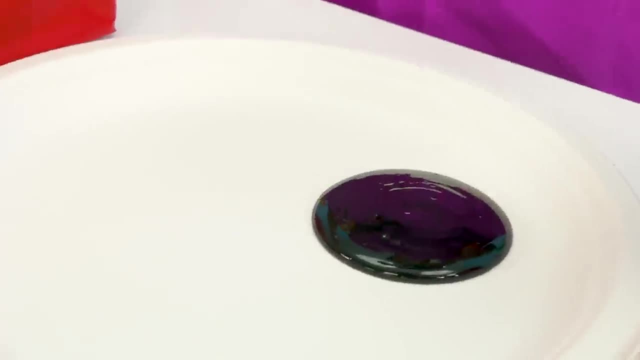 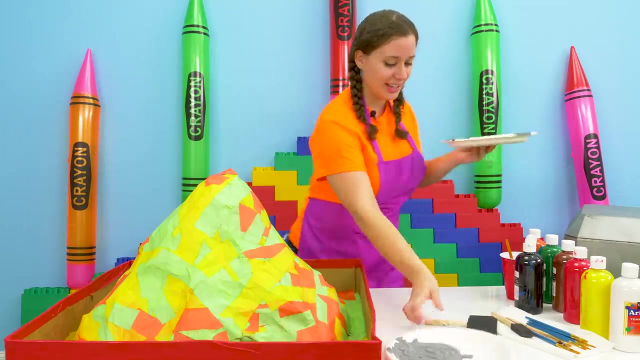 Be careful. Now. gray we don't actually have, But we can make it with black and white. All right, Peck. How do these grays look? Good for me, All right. Well, it's a big volcano. 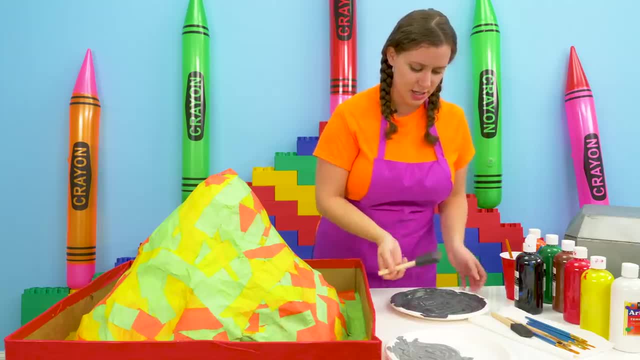 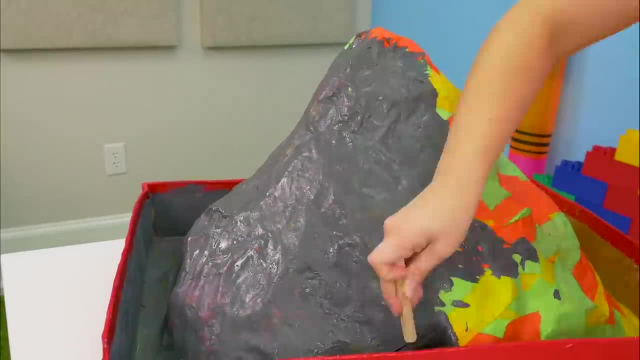 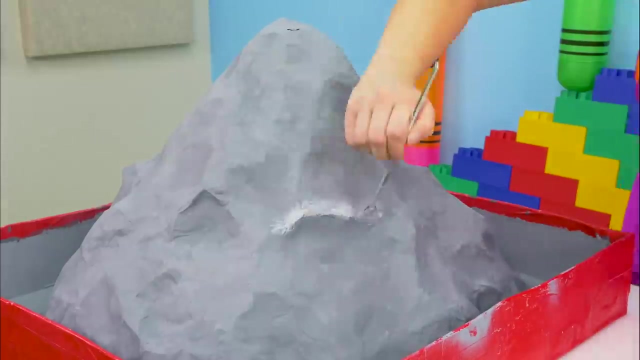 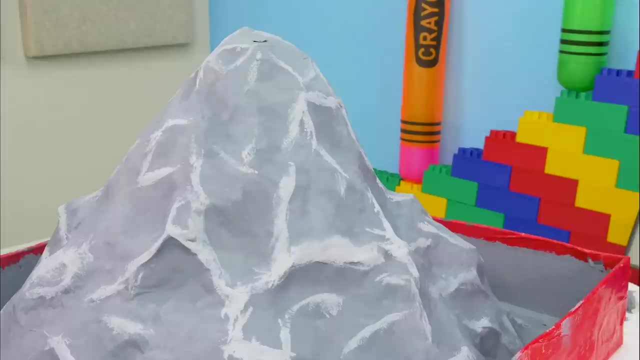 We're going to use a big brush And let's get started Peck. how does it look? It kind of looks just like a mountain. It could use some lava, Some lava. Oh yeah, Some lava. I'm going to head back now. 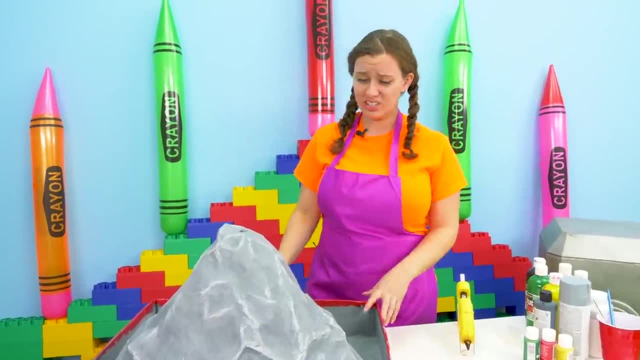 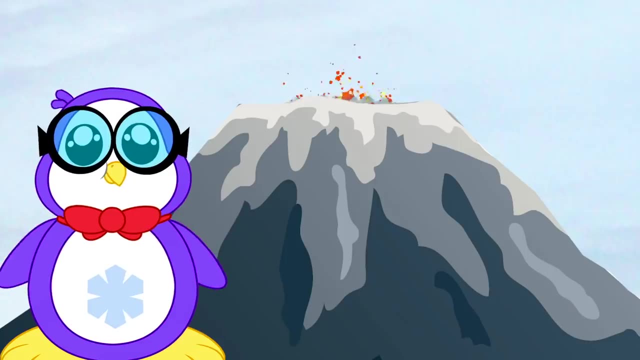 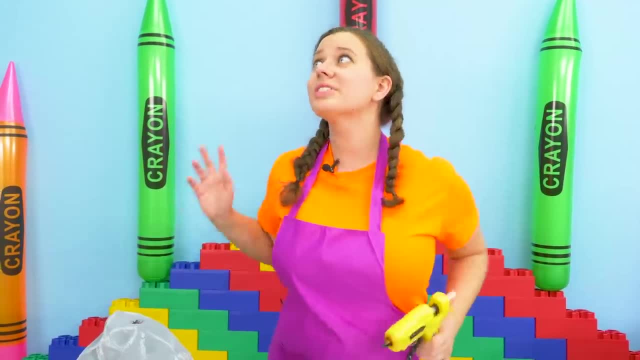 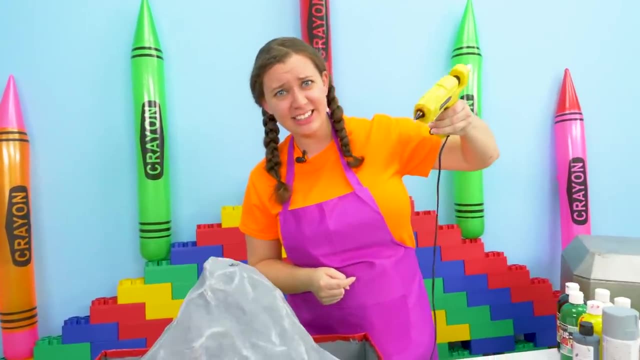 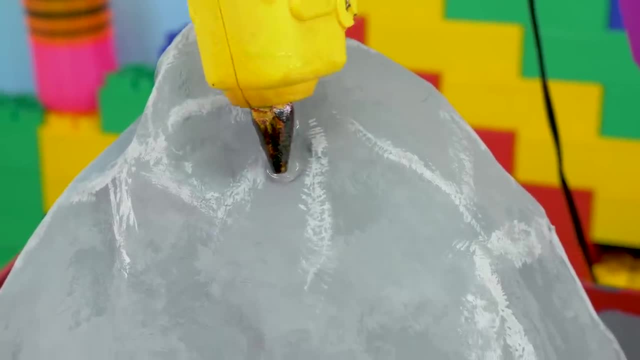 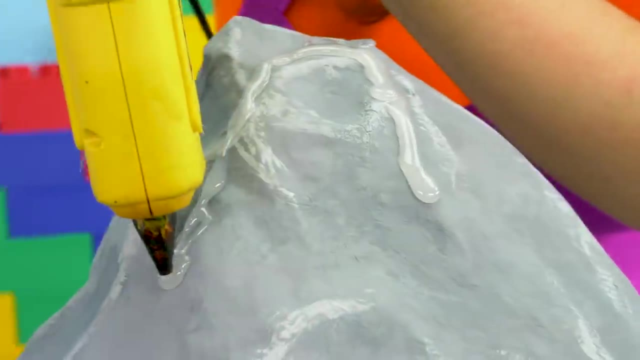 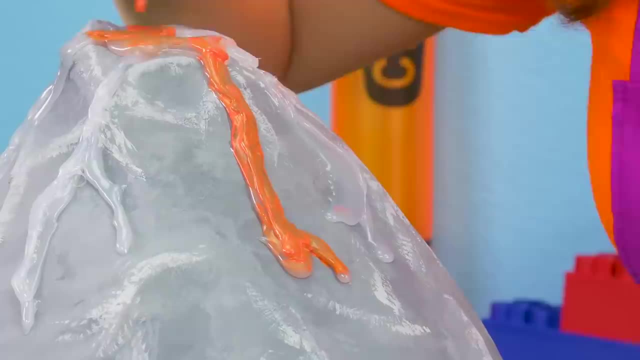 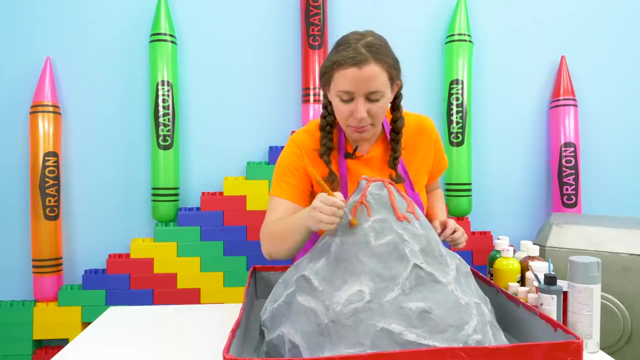 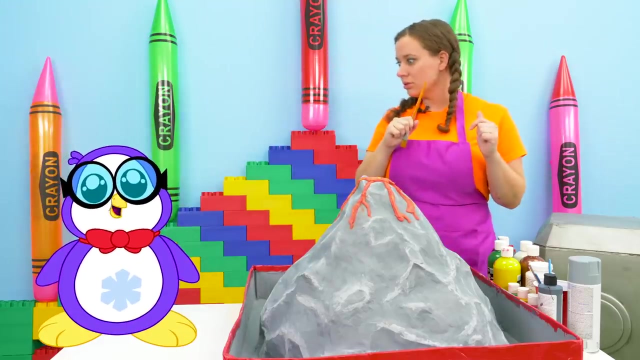 What better than hot glue? I mean, it kind of looks like lava, right? Maybe use some orange and some yellow to give this lava some color. oh, just a little bit more lava paint, and I think I hear Peck made it just in time. oh hi, Peck. so 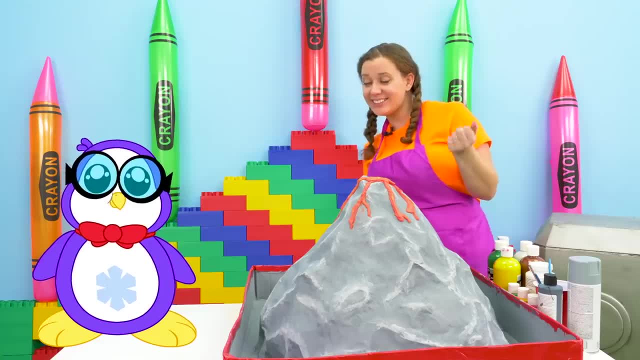 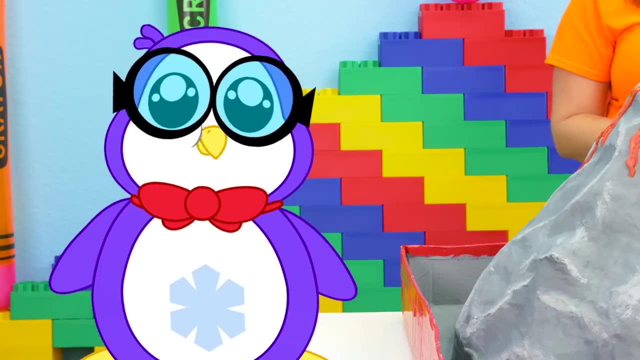 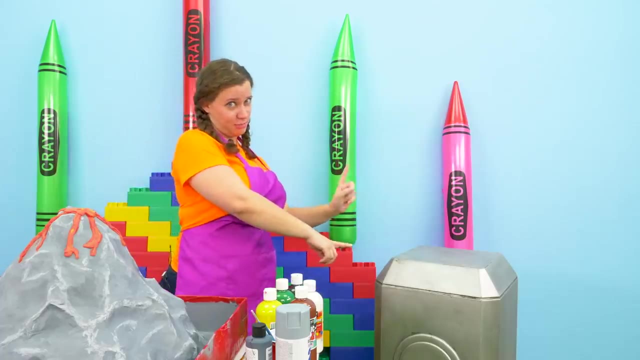 we just finished our volcano and what do you think about it? I think our volcano is complete. looks like the real deal. huh, looks like the one I saw earlier. let's teleport it to Ryan. yay, the last thing we have to do is to get this on to our teleportator potater, so let's just lift this guy. I'm just 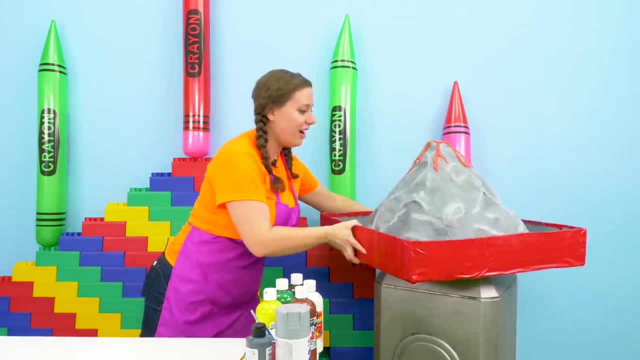 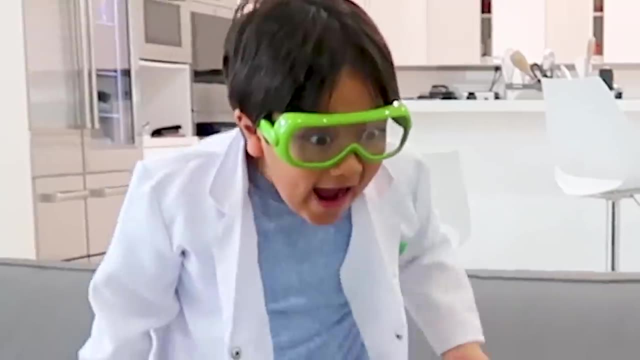 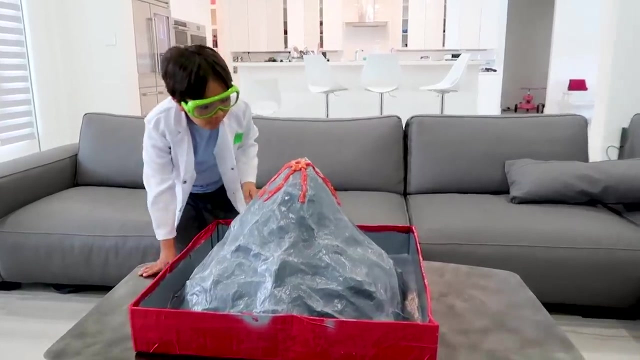 kidding, it's paper mache, it's really lightweight. and off to Ryan we go. good bye volcano. have fun, Ryan. wow, thank you so much, Peck for this paper volcano. it's so cool, super cool. wow, thank you so much, Peck for this paper volcano. it's so cool, super cool. 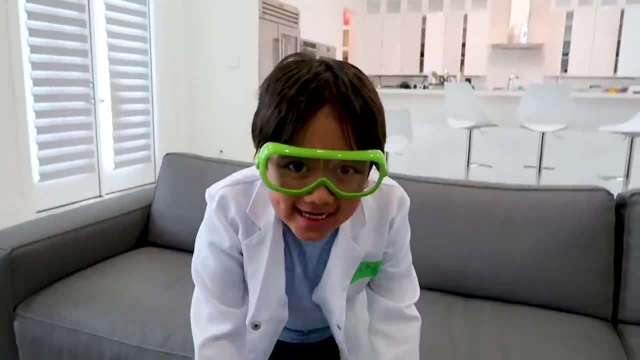 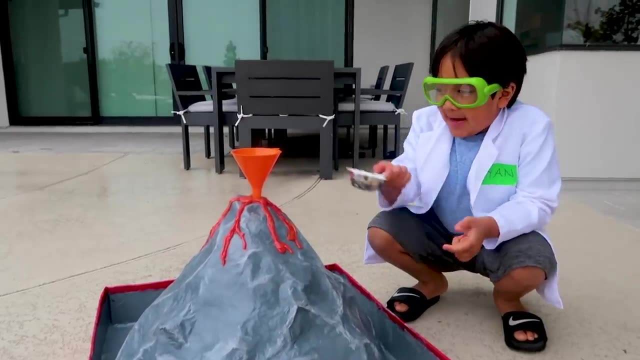 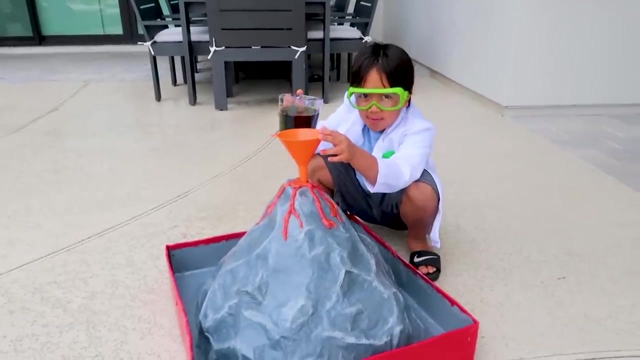 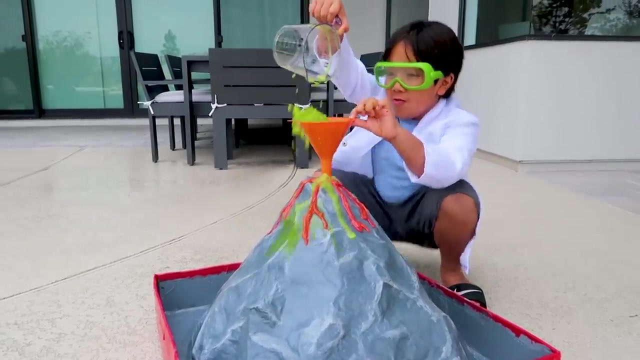 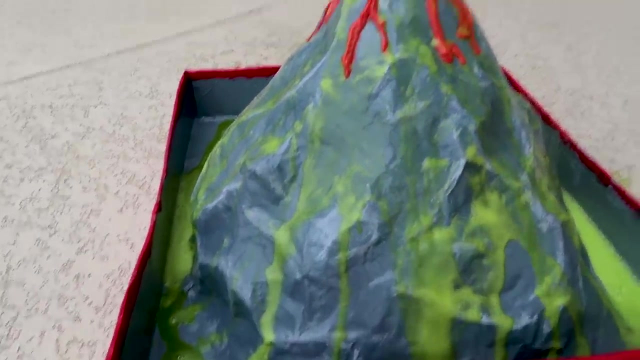 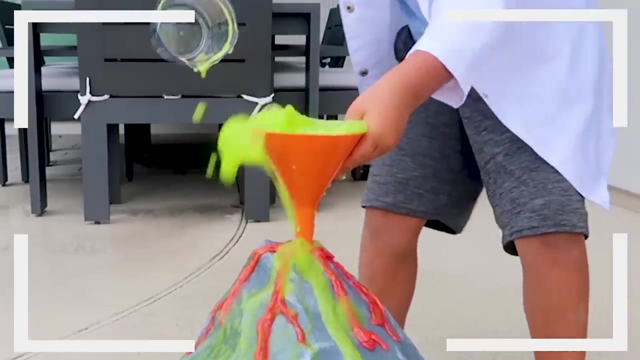 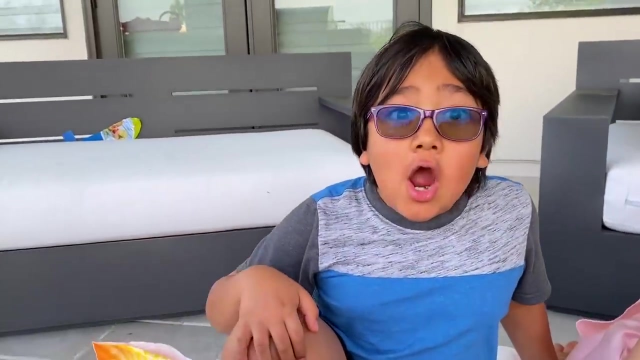 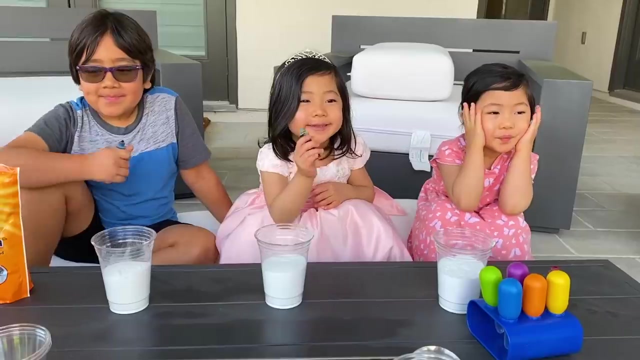 I'm gonna bring it outside and then I'm going to rock it. let's go first thing. baking soda- cool, okay guys. so let's pour in the vinegar. know, baking soda and vinegar science experiment. are you guys ready? and vinegar science experiment: are you guys ready? yeah, okay guys. first step is you just gonna need a cup of baking soda and then your favorite color. 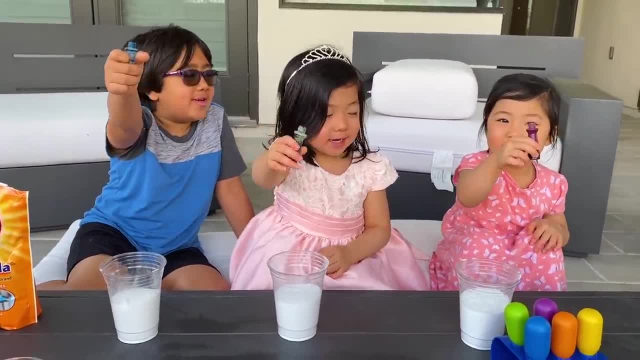 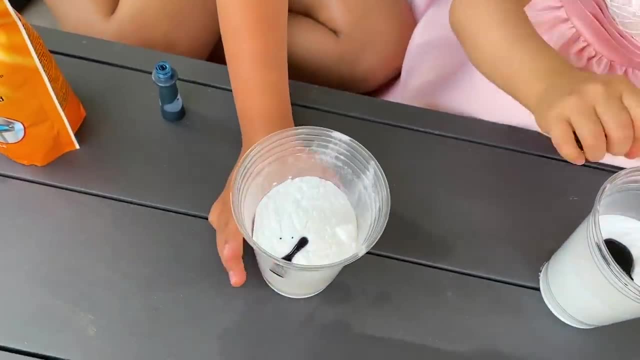 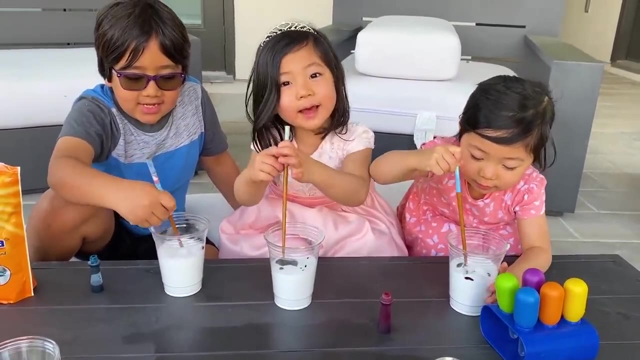 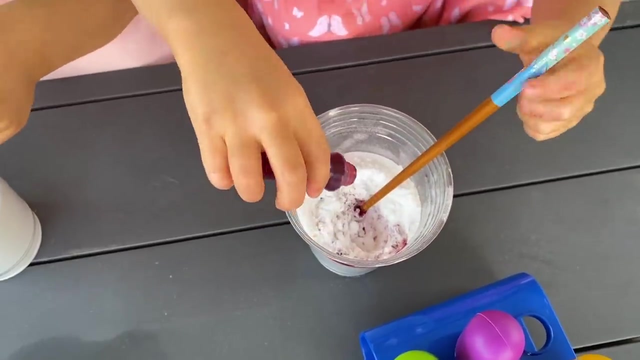 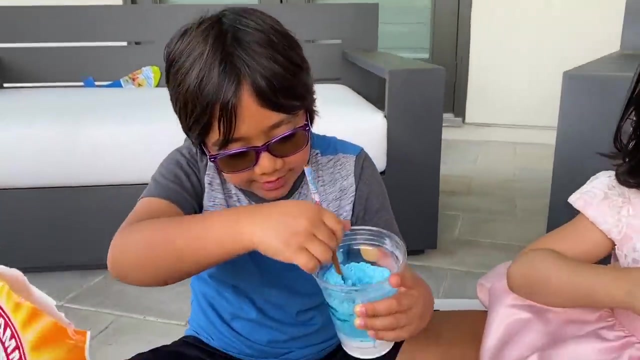 so what color are you guys gonna add? green, okay, go ahead. kate did some red, emma did some green and ryan did blue. next, you're gonna need to agitate to get something to agitate. good girls, good emma, good ryan. look guys, mine's almost fully blue. wow, yeah, agitating good. 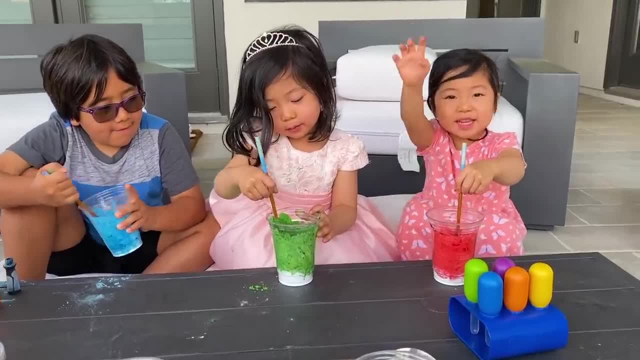 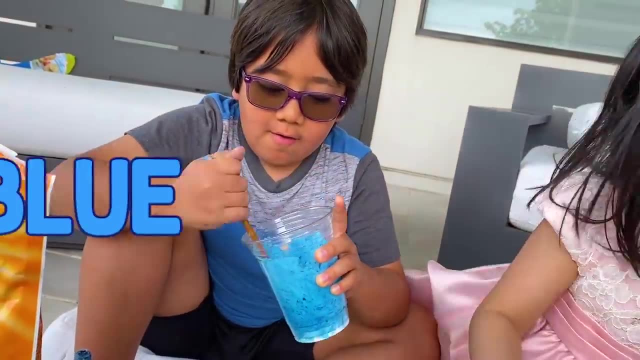 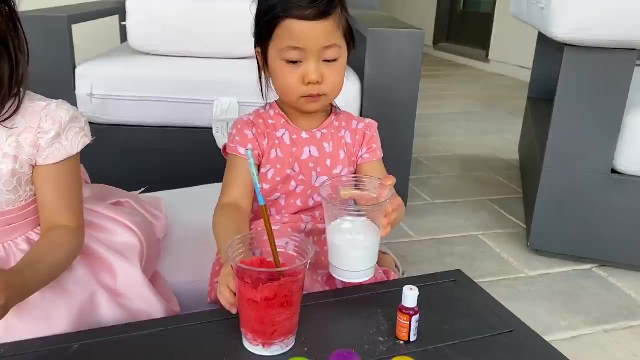 i'm gonna mix it a little more. i'm gonna mix it a little more. yeah, so you guys, colors are coming. good, see, red, green and blue. good girls and boys. okay. so we done with our three cups. now we're gonna do these three. okay, so kate's going to do orange and then emma's gonna do yellow and then ryan's gonna do. 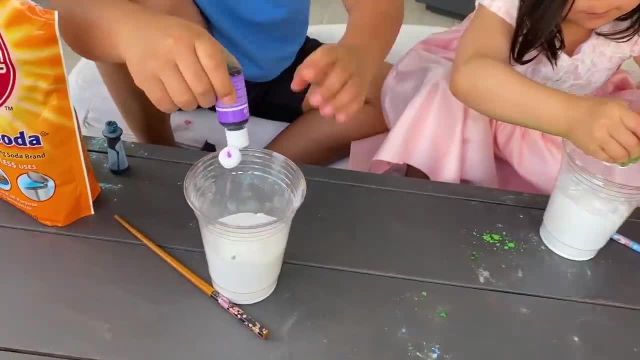 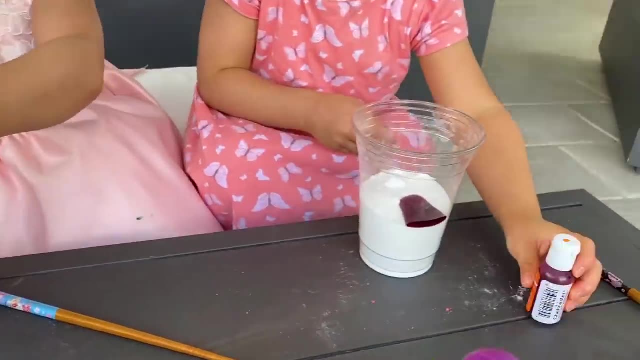 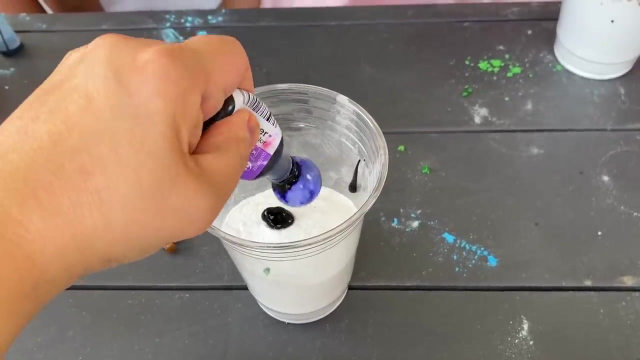 purple. good, there you go. add your color purple. it still doesn't look like yellow, it will. good, there you go. yellow: kate got her orange. okay, there, it is purple's out, but it's okay. oh, look at the bubble. look at that giant purple bubble. all right, start. 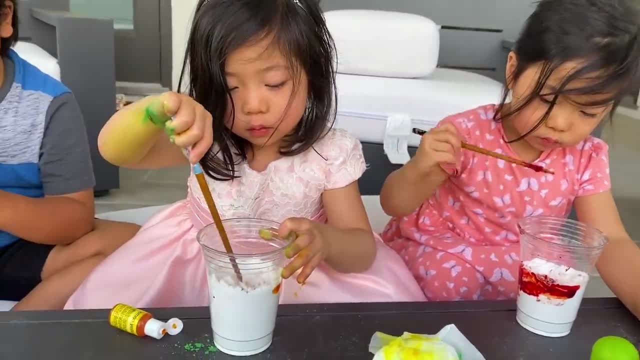 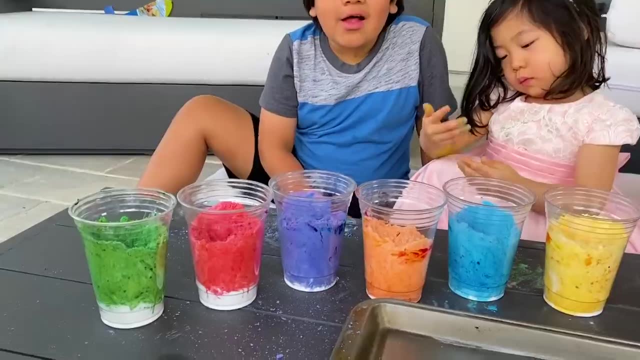 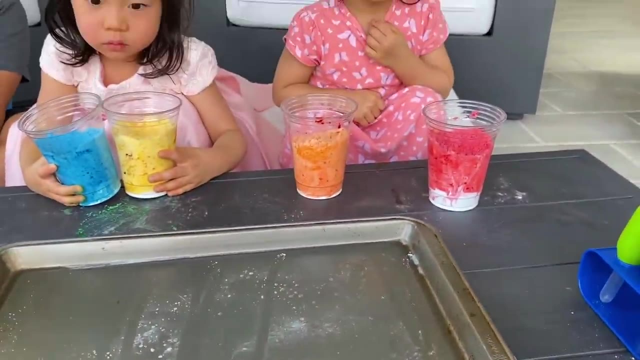 agitating. there you go, agitate, agitate, agitate, agitate, agitate, agitate, agitate. okay, we got our rainbow colors nice, okay, guys. so now we're gonna pour all the colors into this pan here. so, kate, you can start first with red pour it in. 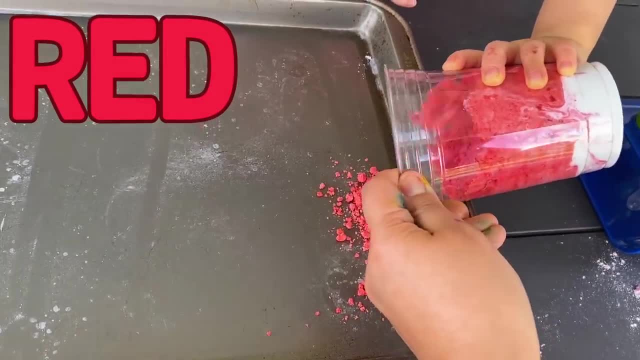 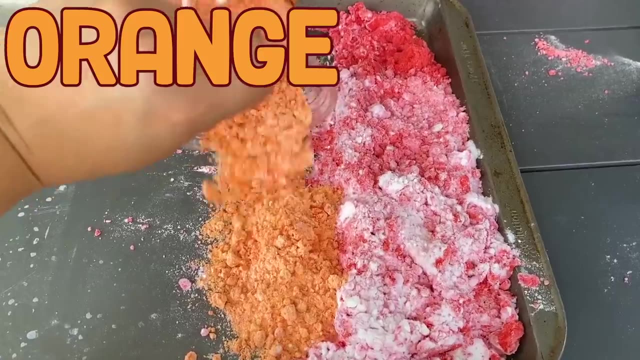 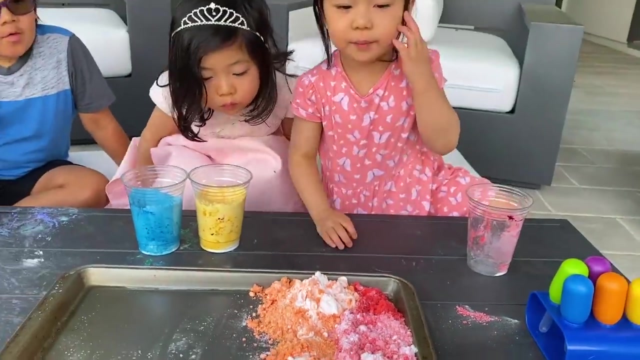 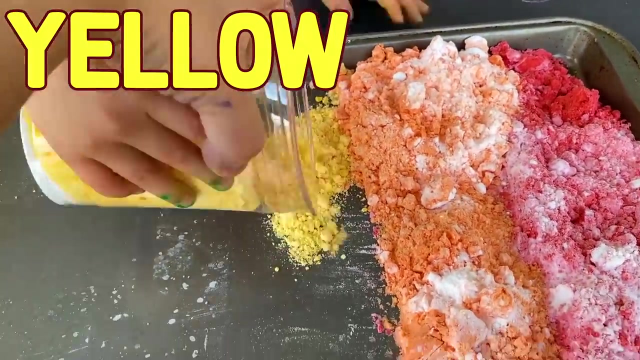 yeah, there we go. okay, we got our red and now we're gonna do an orange. all right, there we go, orange. oh nice, good job, kate, let's go there, you go. good, i help you. it's okay, there you go. good girls. wow, so beautiful huh. 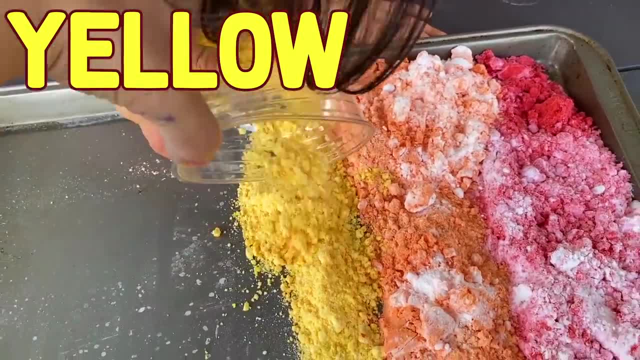 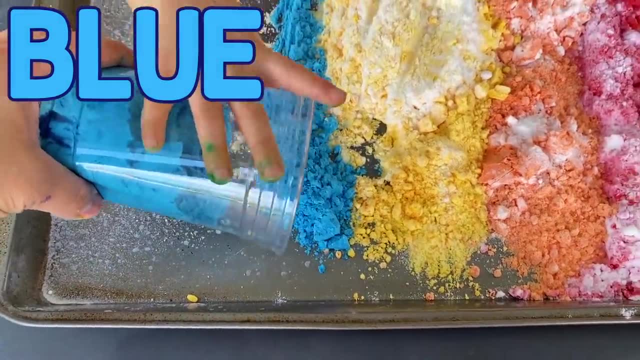 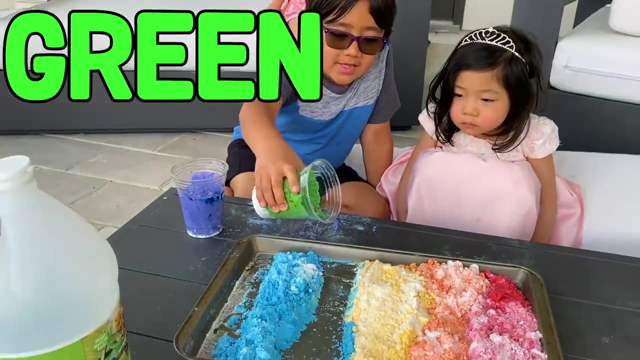 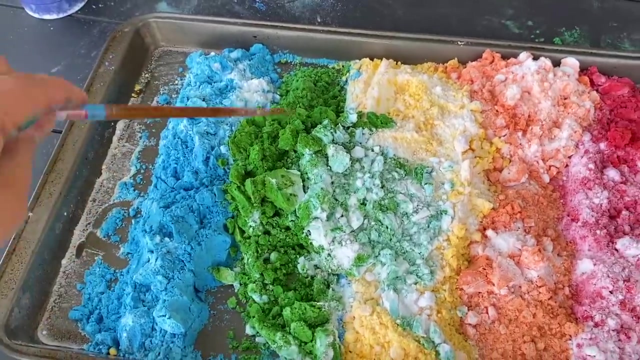 it's like a rainbow. yeah, now we do blue. good, there you go. yeah, beautiful, okay. so we accidentally forgot the green here, so ryan's gonna pour the green. yeah, there we go. whoa, it's okay, we can fix it. spread out the green. it looks pretty huh. 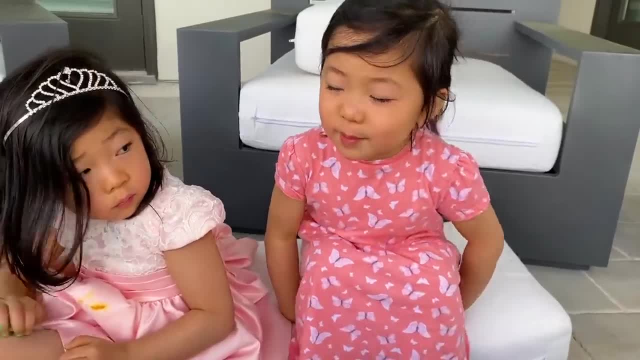 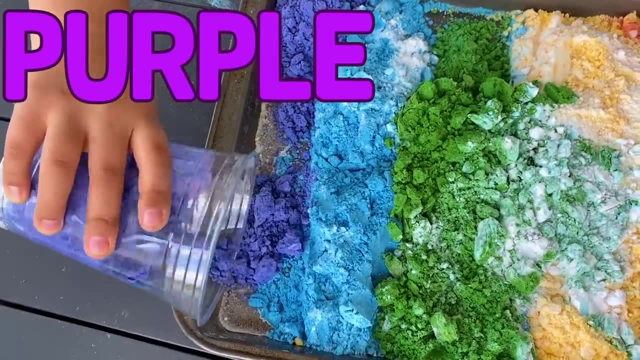 yeah, it's actually a lot of girls. yeah, like a rainbow, but now we need purple. that's right, purple. yeah, wow so beautiful. yeah, it's like a rainbow, but now we need purple. that's right, purple. yeah, wow, so beautiful. looks like a rainbow it does. now mom can use these. 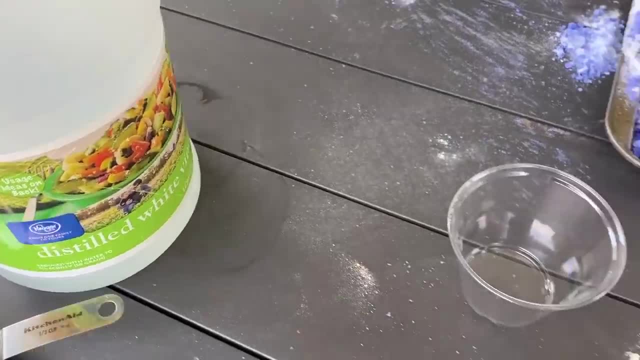 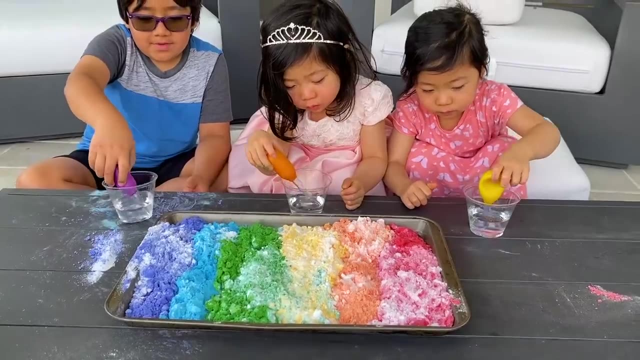 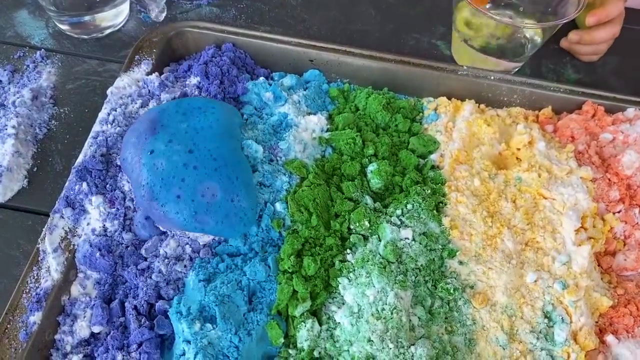 yeah, almost done. good job, guys. you gonna need some vinegar here. yeah, help me. yeah, of course. okay, i'm gonna pour some vinegar in each cup for you guys. okay, there you go, pick up some vinegar and then just do it. yeah, emma, squeeze like this. you see the bubbles? 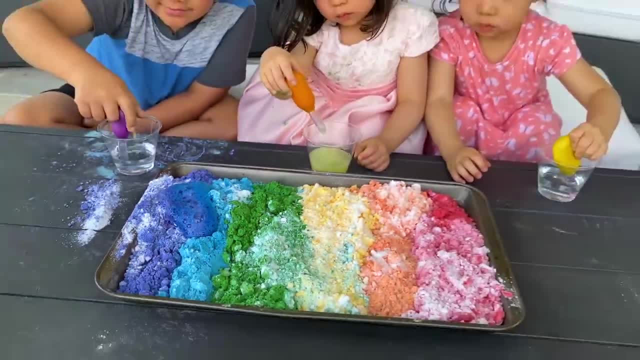 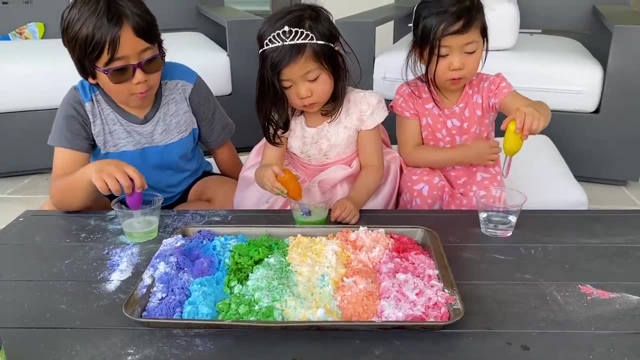 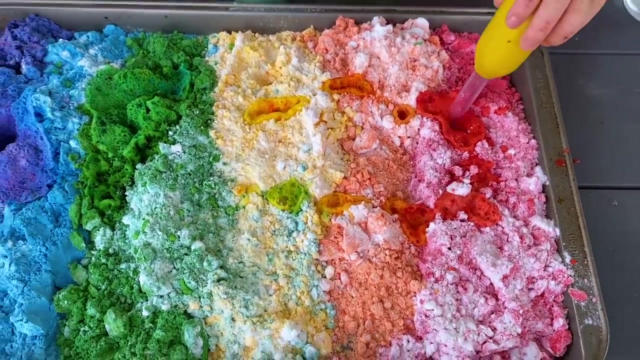 emma, look, emma, look, i put some bubbles. Wait, are you mixing them together? Whoa, Whoa, Whoa. Look, mine is even getting taller. Wow, Mine has so many colors. at the same time, Mine is growing. 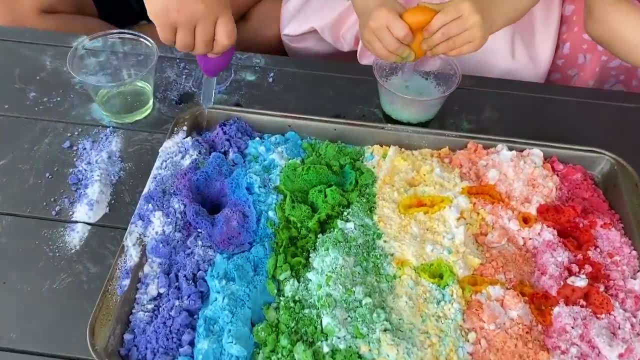 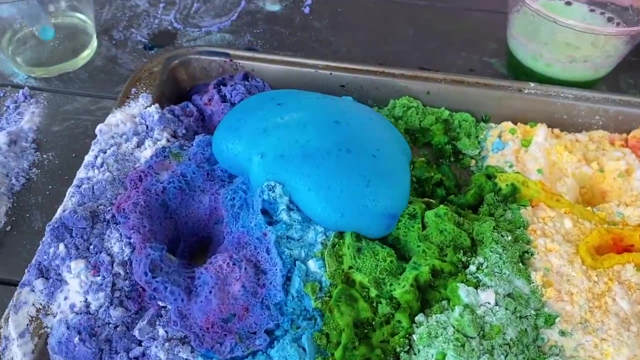 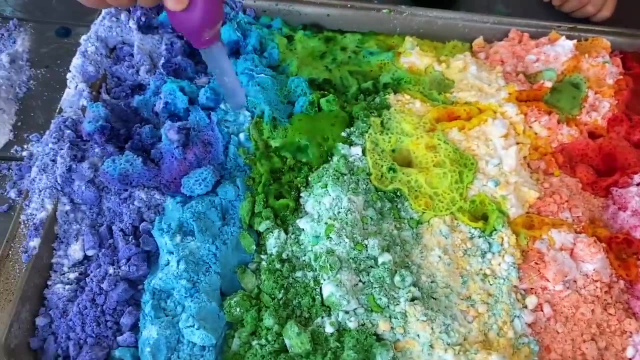 And that's just mixing over there. Mine is mixing with all of the colors. Mine is mixing together. Whoa, that's cool. Whoa, That's a big one. I have a reaction inside my cup, Whoa, Whoa. 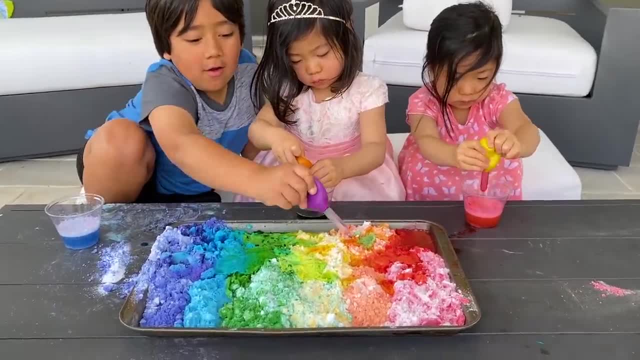 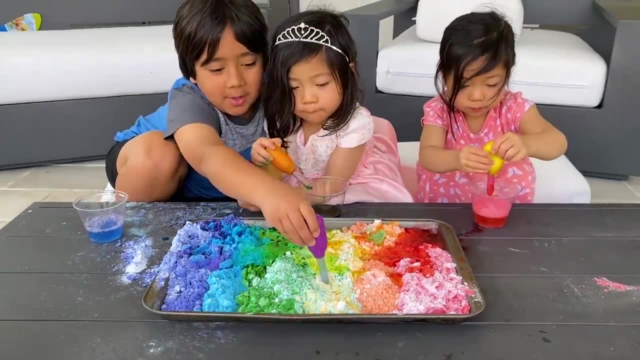 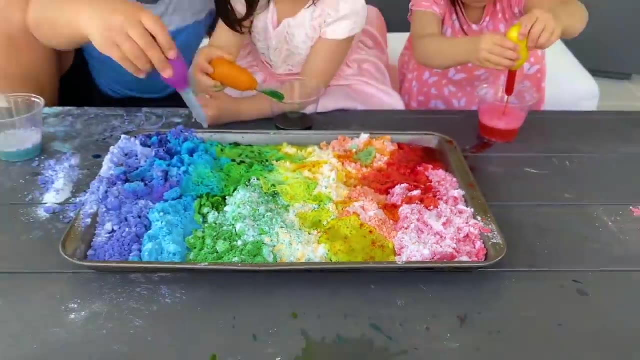 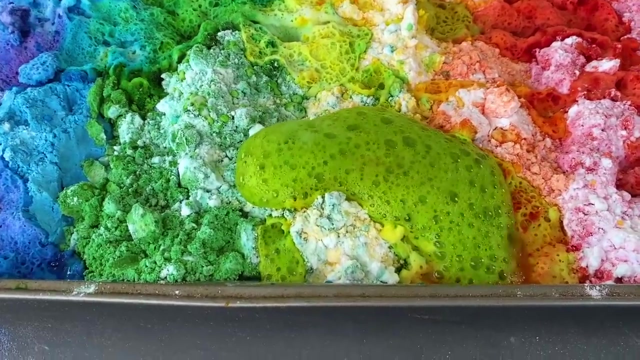 That's cool. Whoa, There's a spot you guys haven't done yet. Okay, I'm going to do it on one single spot. Okay, Whoa, that's giant. Another one: Wow, Whoa, That's a really big one. 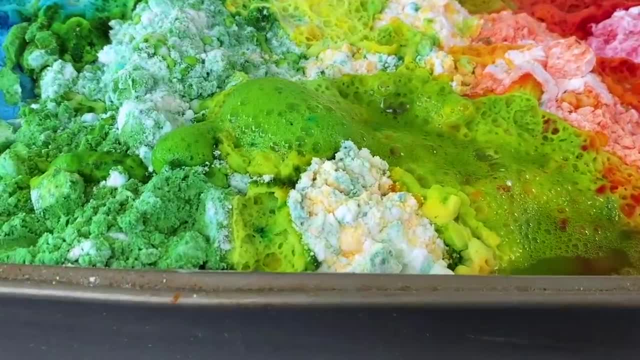 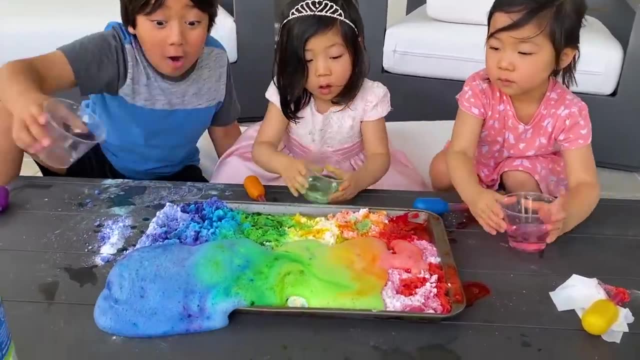 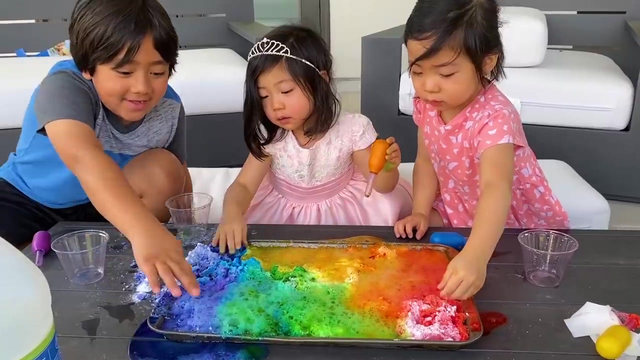 Yeah, Whoa, look at the bubbles. Okay, Okay, we're going to pour it now. Whoa, Whoa, Rainbow, Can I touch it? Yeah, Whoa, It looks so cool. That was fun, huh. 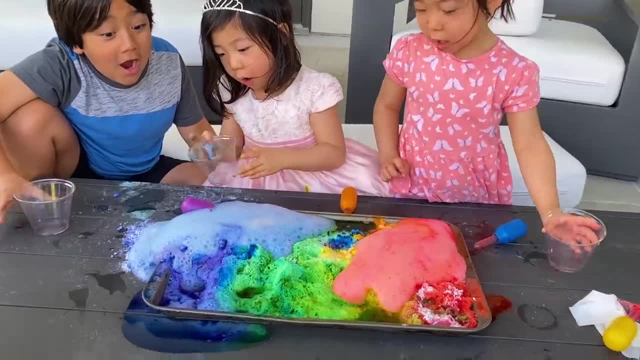 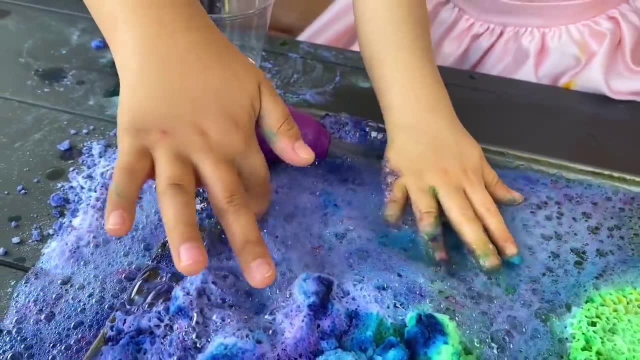 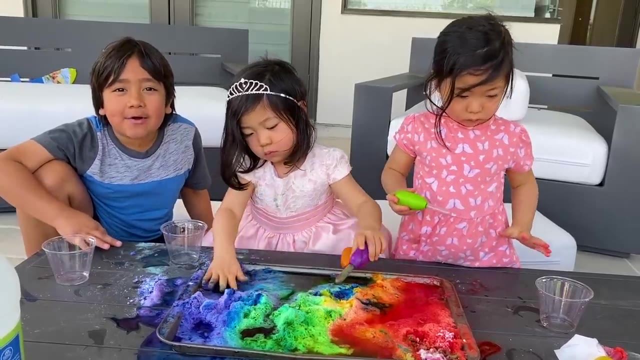 Yeah, Whoa, Can I touch it? Yeah, Okay, Whoa, That's super cool. Yeah, Thank you for watching our baking soda and vinegar rainbow science experiment. Guys, today we're going to learn how important it is to wash your hands. 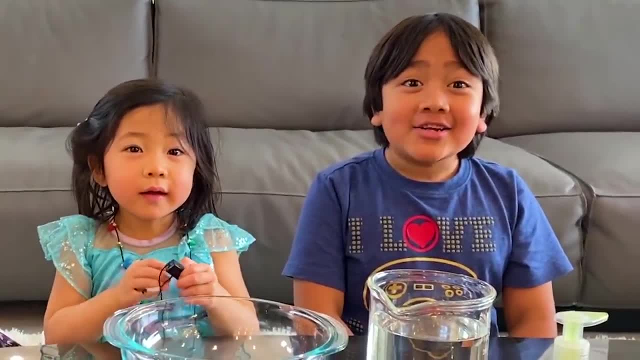 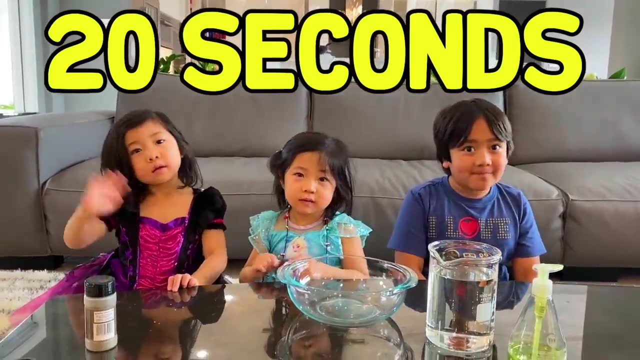 Yeah, so you know how long you're supposed to wash your hands for? Yeah, How long You're supposed to sing happy birthday two times. That's right. so it's about 20 seconds, Okay. So here's the experiment I want you to do. 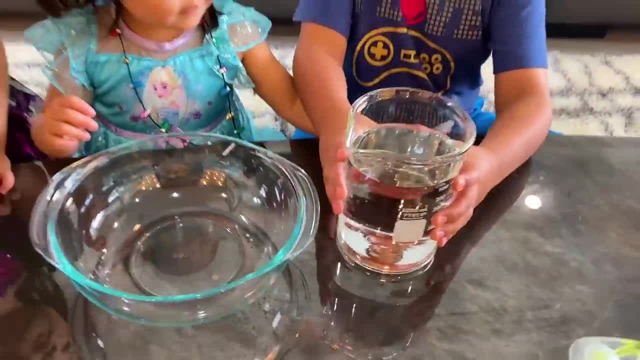 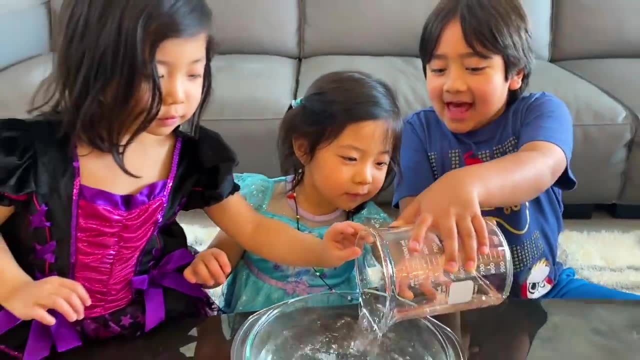 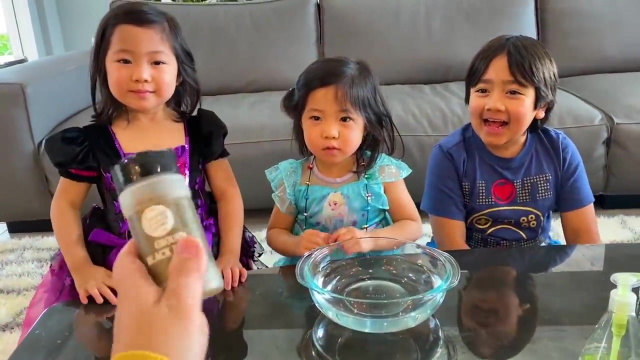 This is water. Pour the water in there. Okay, Do it very, very carefully. The whole thing, The whole thing. yeah, I helped Ryan. You did help Ryan. So this is pepper- Any pepper you guys have. this is the one that I have in the house. 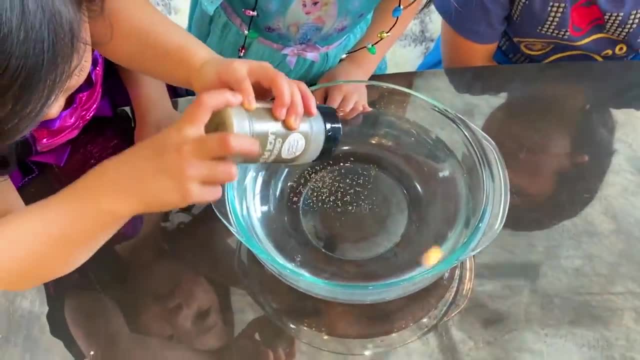 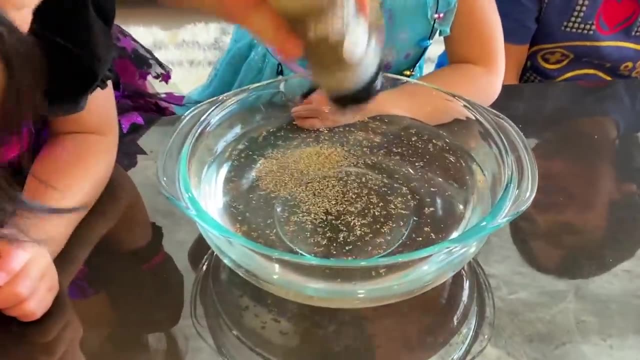 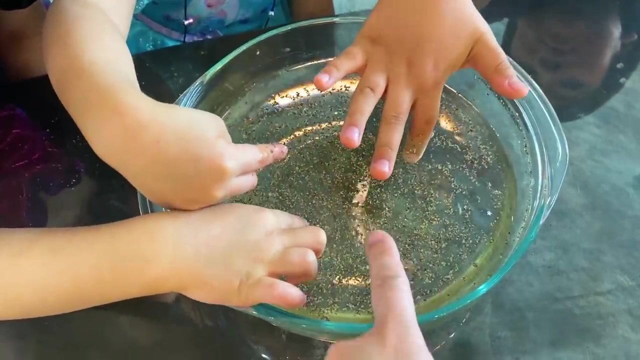 Okay, so sprinkle some peppers in there. Yeah, take turns, Sprinkle more, Not more than that. There you go. That's a lot. Next step is I want you to take your little finger and dip it into the pepper water. Now I want you to pretend. 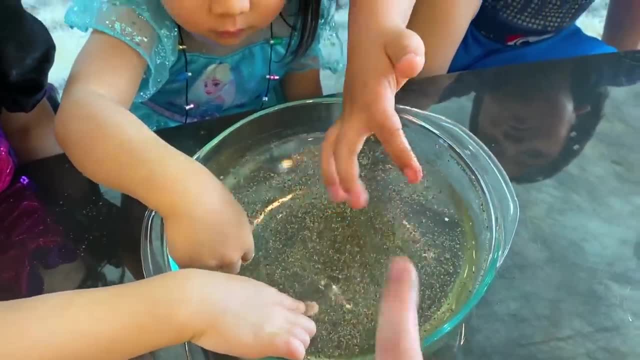 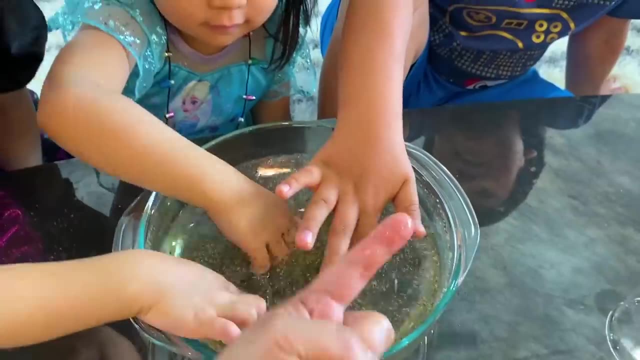 these pepper water are germs. What happens when you take your hands out? Oh no, There's germs. Yeah, you see, And if you touch it, there's germs. right, Look how there's germs on you. 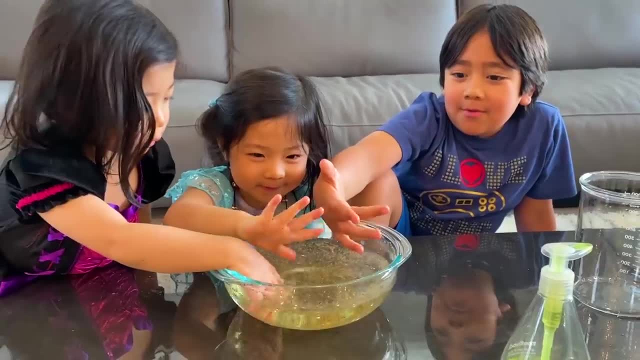 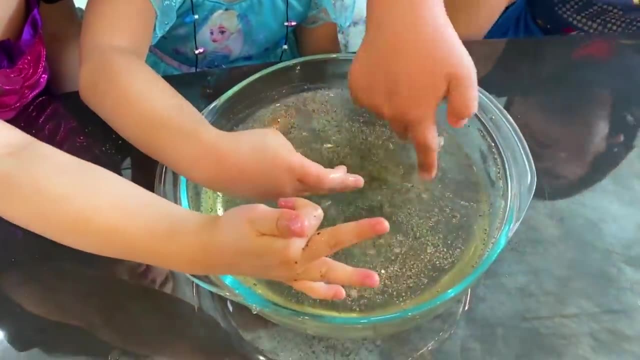 There's germs on me. I know, You see the germs, Yeah, Okay. That's why it's important to wash your hands. You ready? Yeah, Okay. so that's what happens without soap: It just sticks on your hand, right. 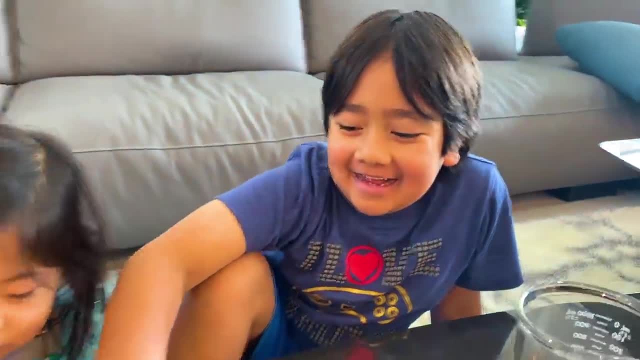 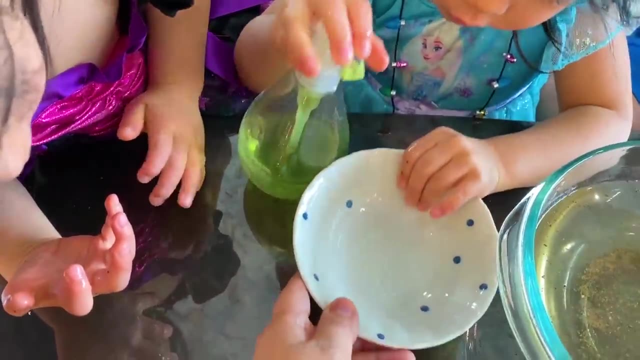 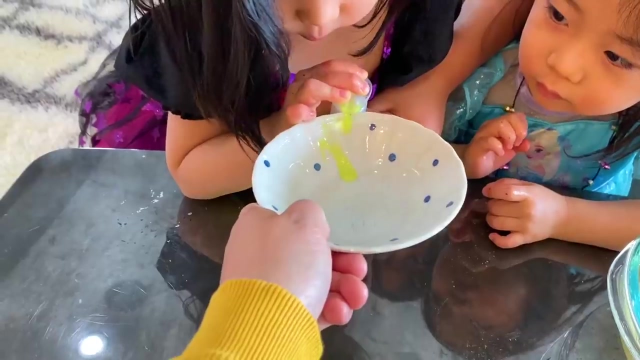 Oh, germs everywhere. Next, I want you to squirt soap into here. I want to do it, There you go. Can you squirt some soap into there? I hold for you There you go. Good, Alright, cake turn. 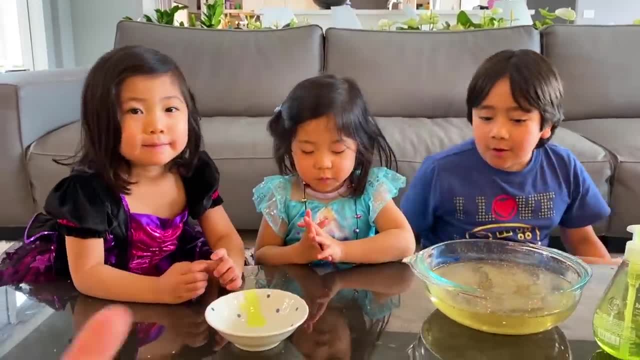 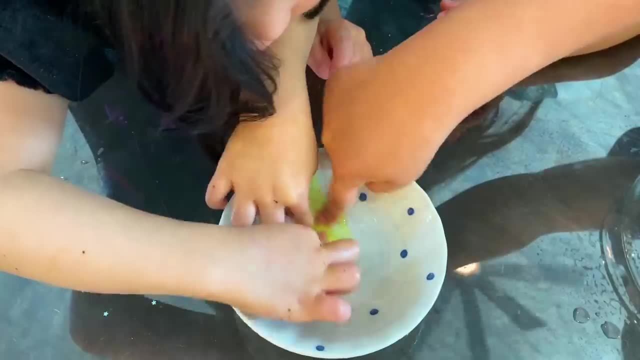 There you go, Alright, Okay, that's a lot. Here's what I want you to do: Take your little finger and then dip it into soap. There you go, Dip in a lot, Okay. So this is why soap is important. 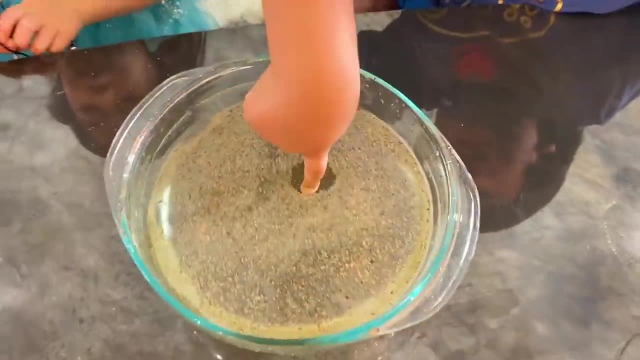 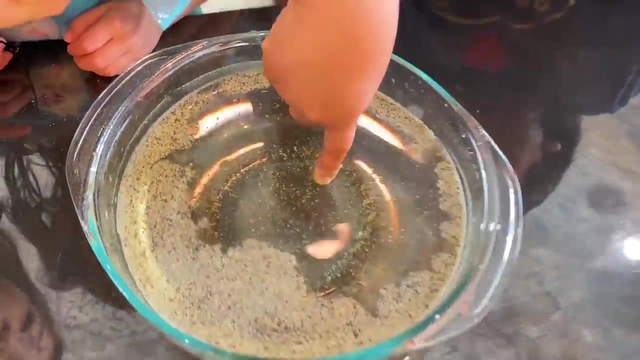 First, Ryan's gonna do it. Okay, go ahead. Whoa, What happened? The pepper's going away from the soap. I know It looks like the pepper's running away from the soap, right, So think about it. So if these are like germs or bacteria, 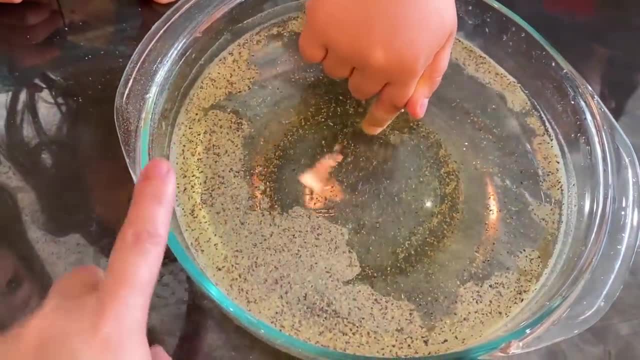 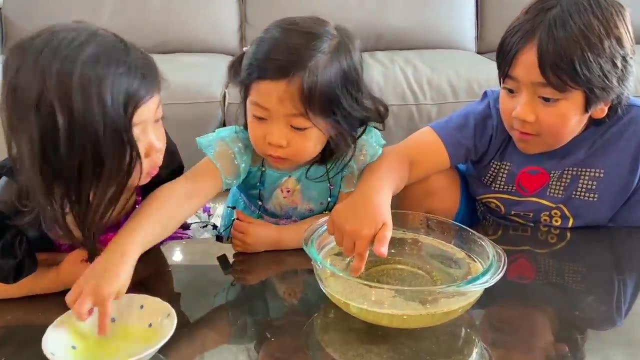 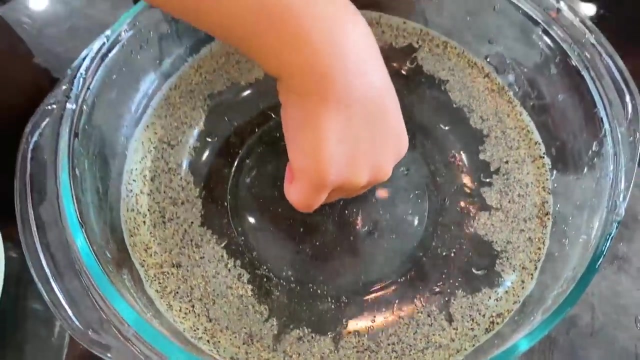 when you put your hands in soap right, All the germs and bacteria are no longer on your hands. They're running away. Yeah, of course It's my turn. Whoa, that's so cool. You see how it's running away. 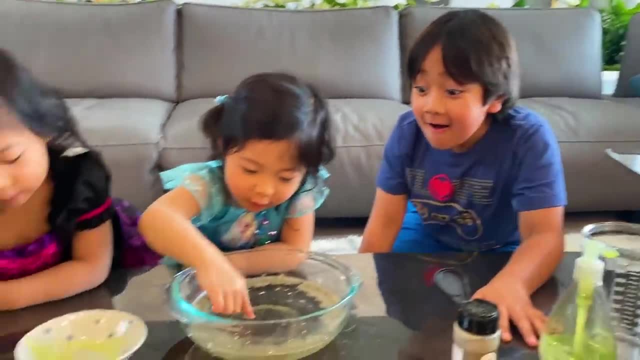 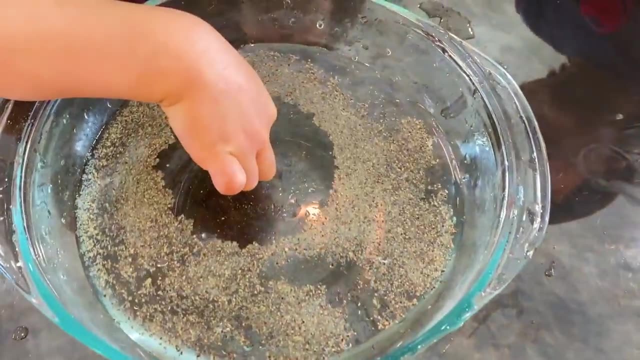 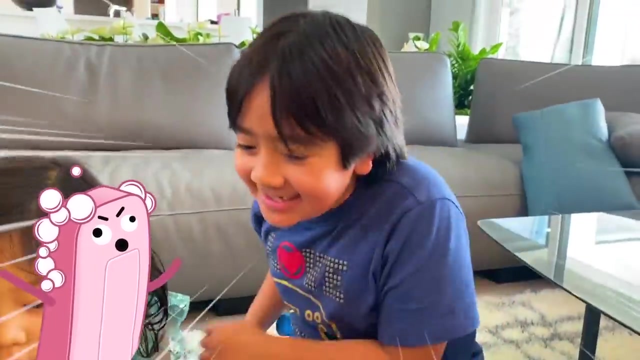 Whoa, That's so cool. Whoa, Alright, Kate, you want to try now? Okay, guys, it's my turn. Whoa, it's running away too. Yeah, Yeah, It's like oh, no soap. 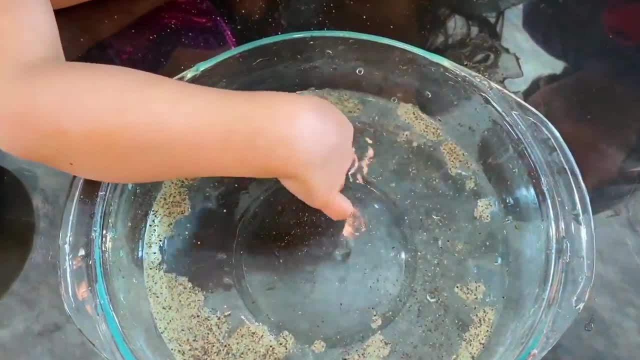 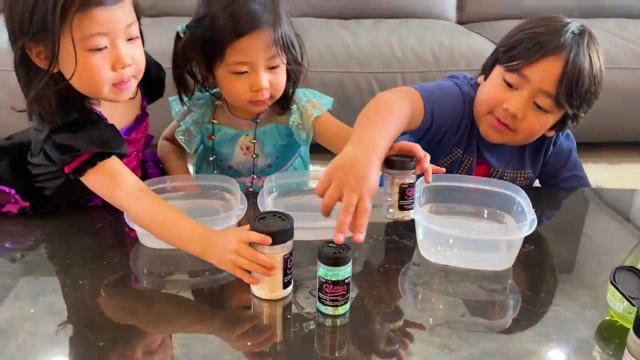 That's why it's very important to wash your hands. Now we're gonna do it with glitter, Yeah, so you guys can take a glitter or a share- I want this glitter- And put it into water and pretend these are germs. 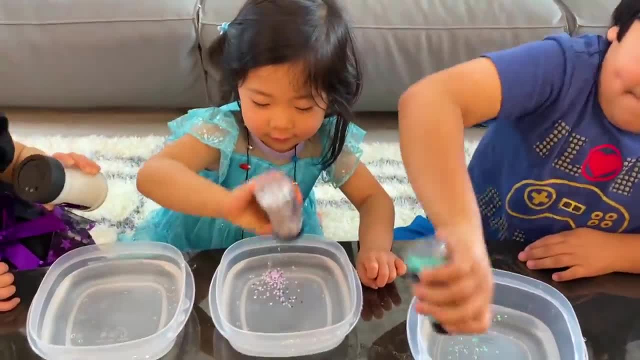 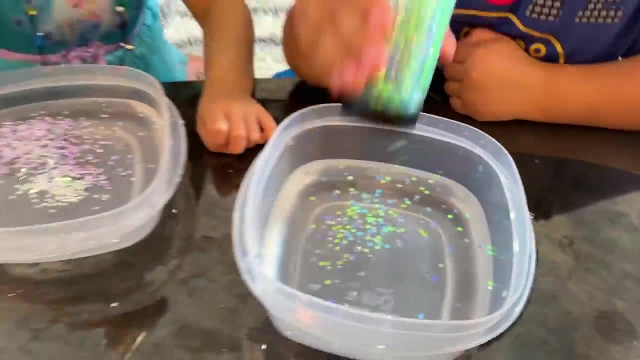 There you go. I'm putting a lot, You're putting a lot of germs. Yeah, I'm gonna put a little bit. Okay, a lot of germs for Emma. There you go, Whoa, And then we can all share. 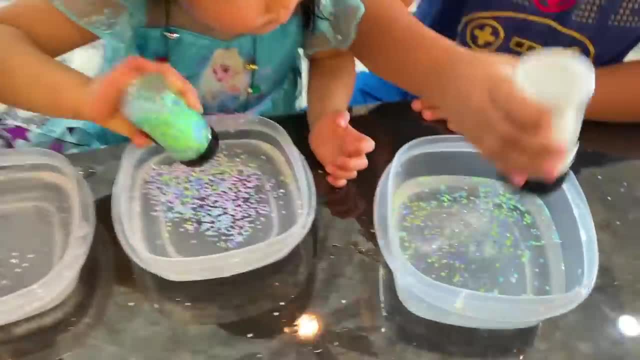 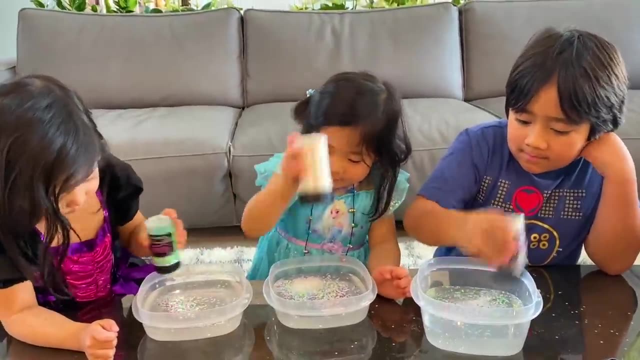 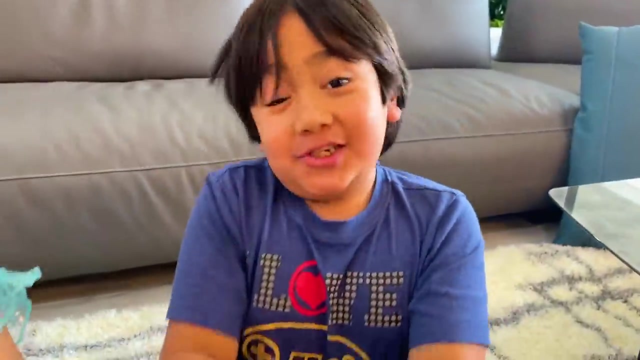 Ooh cool, Kate. There you go. I'm adding some white germs. now I want some white germs, Different types of germs. Shake, shake, shake, Shake, shake, shake, Shake the glitter. I mean shake the germs. 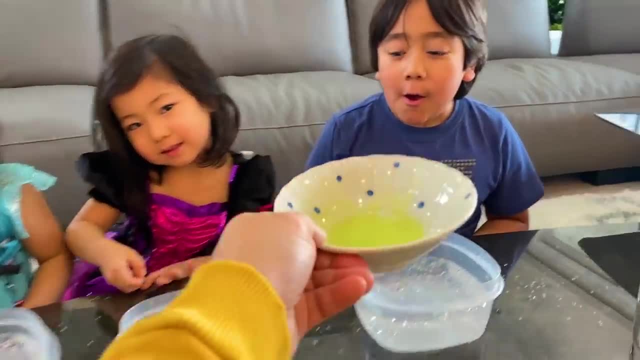 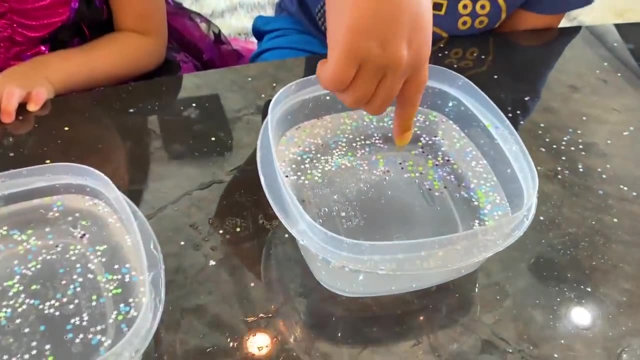 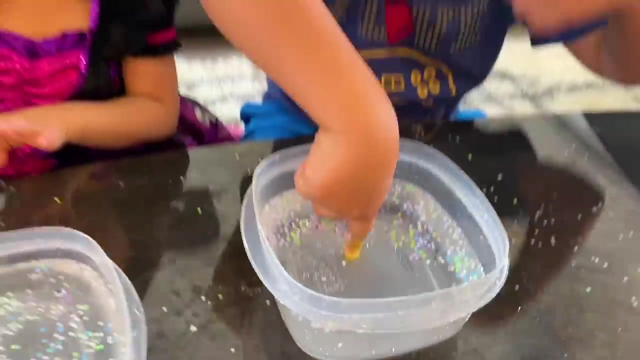 I'm shaking the glitter. Good, Now let's try the power of the soap. Okay, Soap on And then put it in. Wait, it's going away. Yeah, it's moving away from your finger. Yeah, it's like whee. 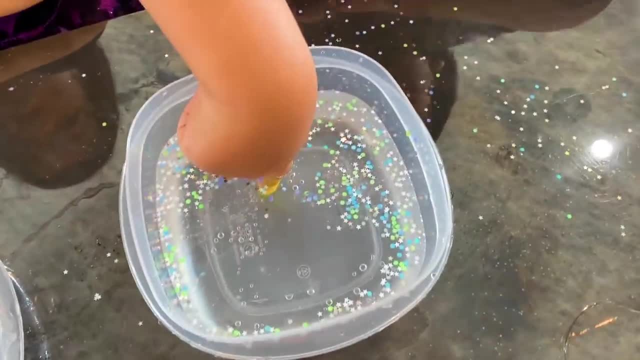 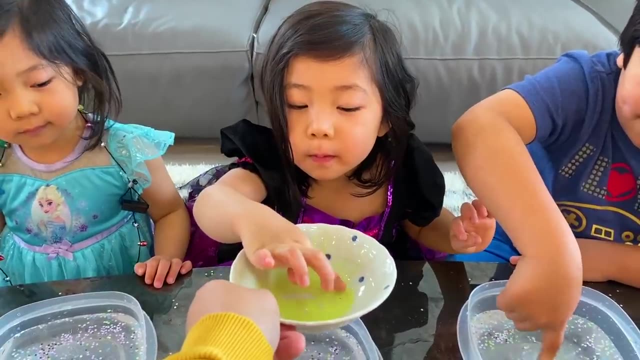 There was one right here and it was like poof. Yeah, All right, Kate, your turn. It's yours, Dip it in there. We're gonna use quite a lot of soap. There you go. Good job, girl. 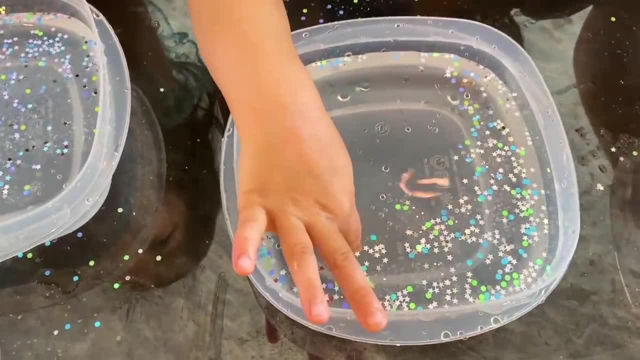 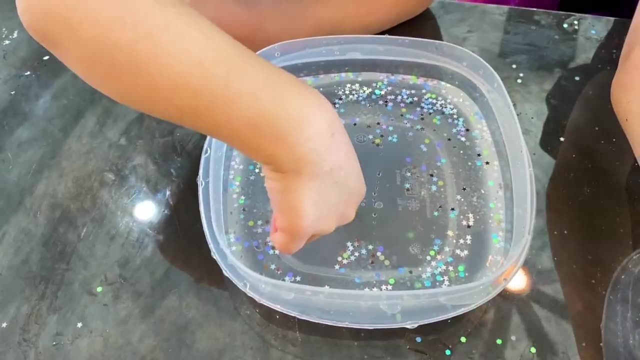 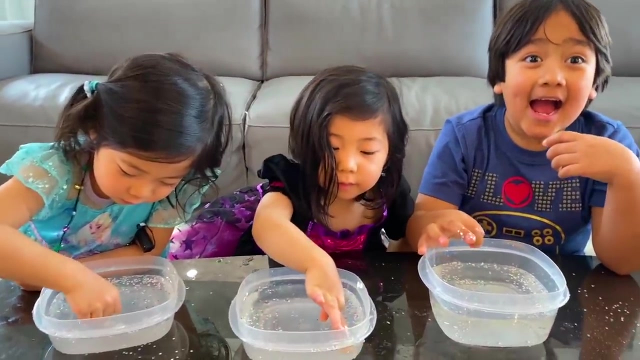 Yeah, Look at it. Look it went away. This one went away. Go, Emma, Whoa, did you see how it separated? Yeah, it separated. Good, All right, that's so cool. So now you learned why you should wash your hands. 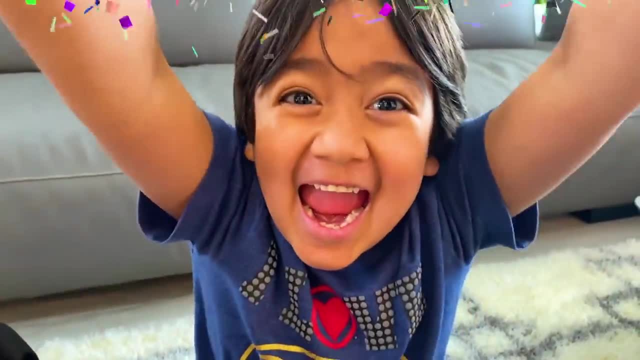 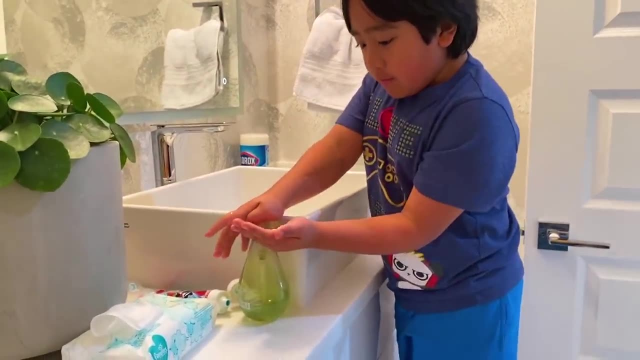 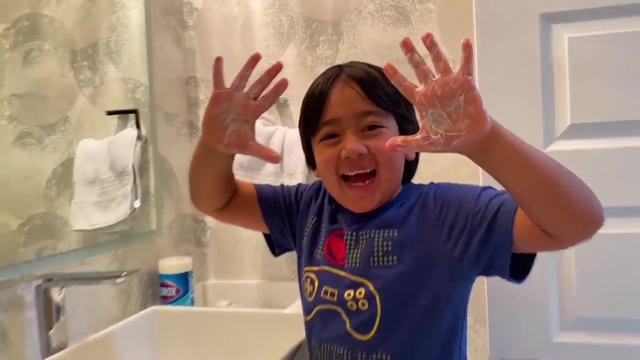 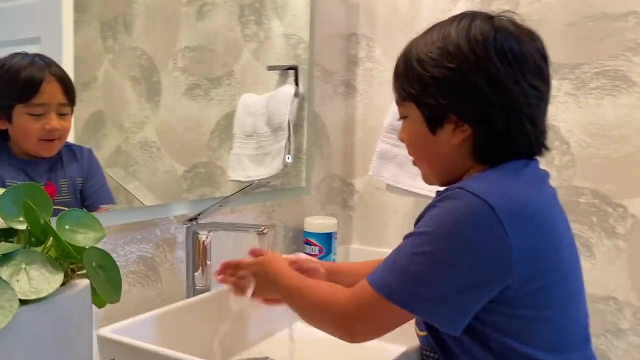 It's time to wash your hands. Yay, Now it's time to wash my hands. Okay, Soap on, Run around, Wah, Okay, Let's do this. Happy birthday to me. Happy birthday to me. Happy birthday to me. 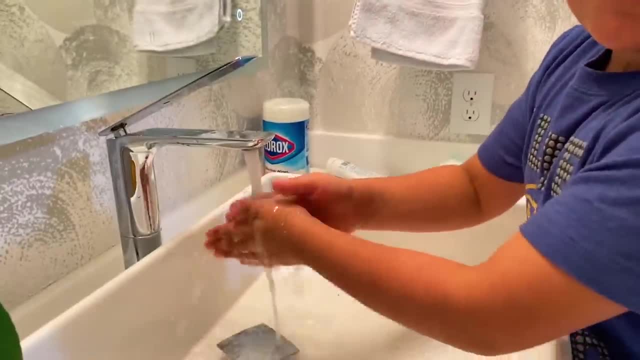 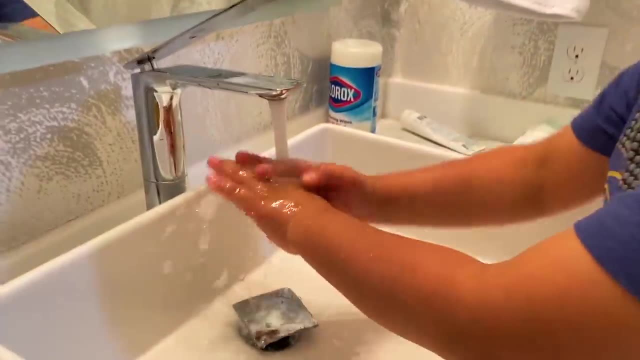 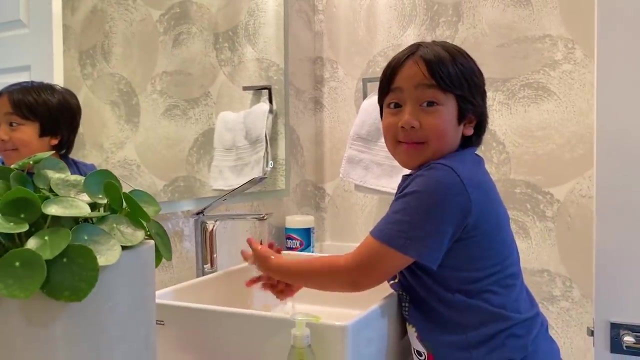 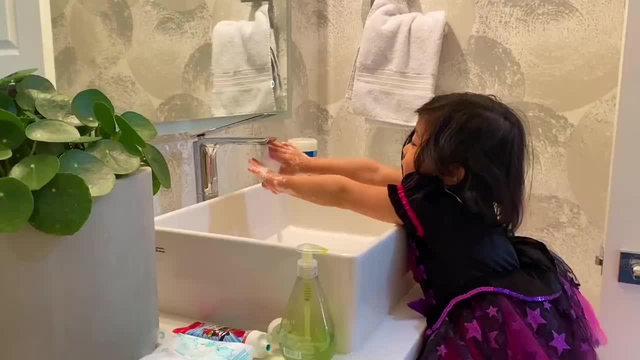 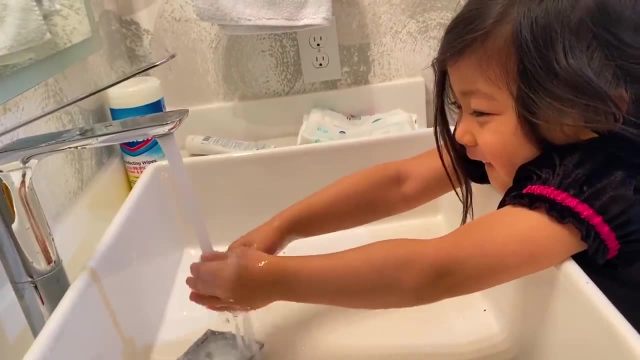 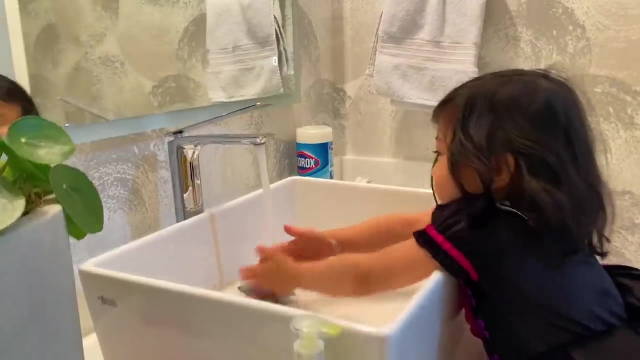 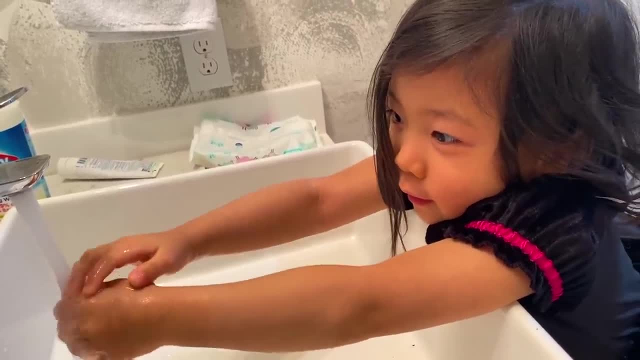 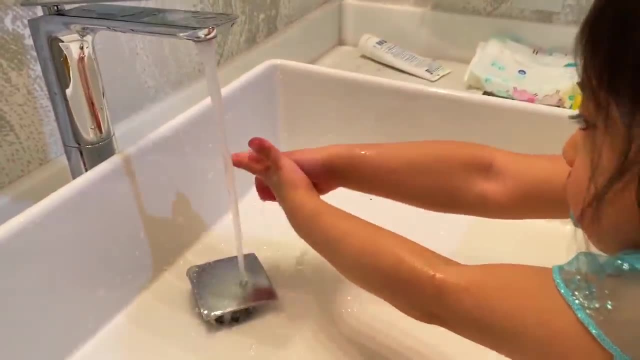 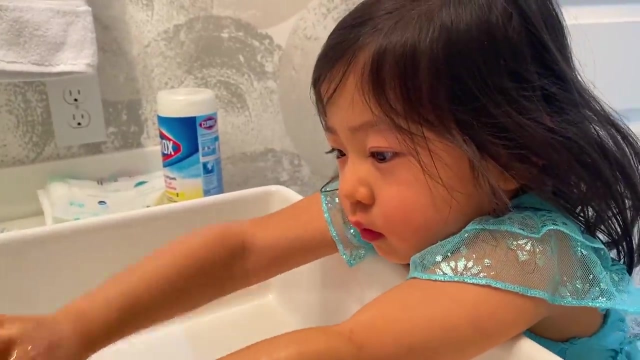 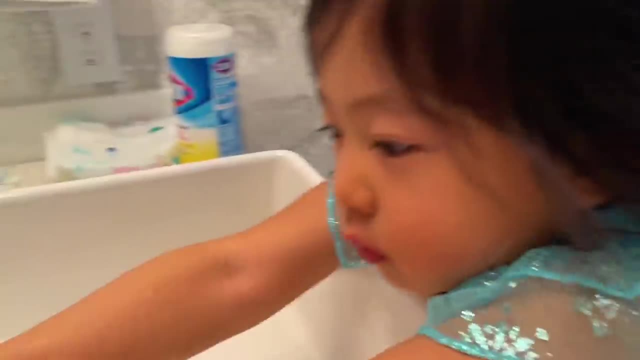 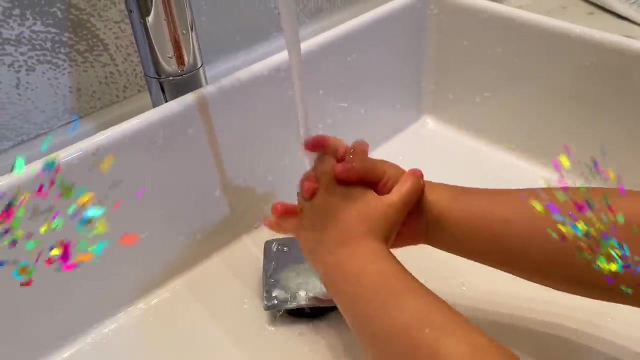 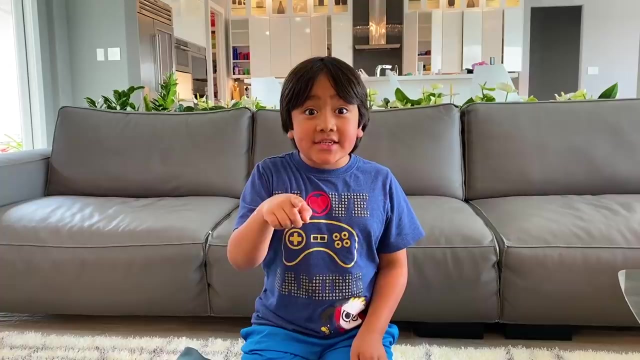 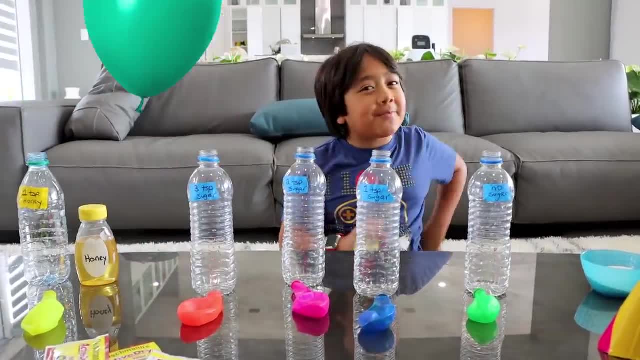 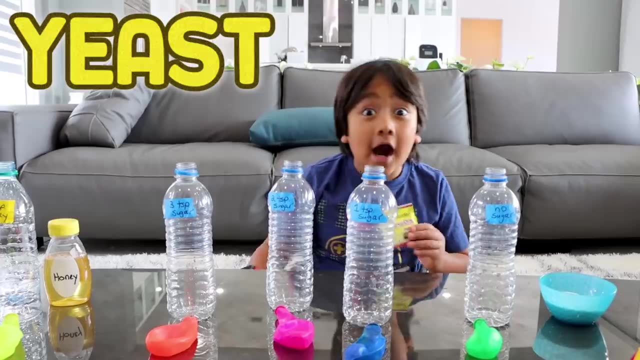 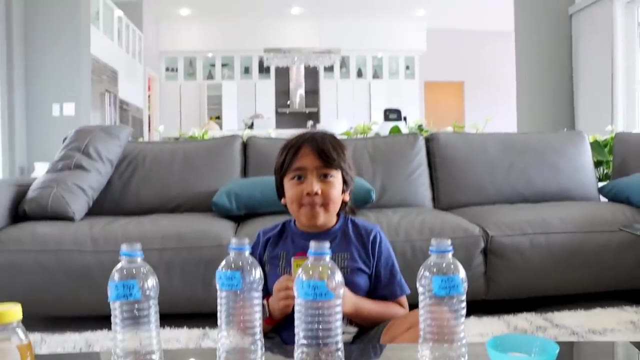 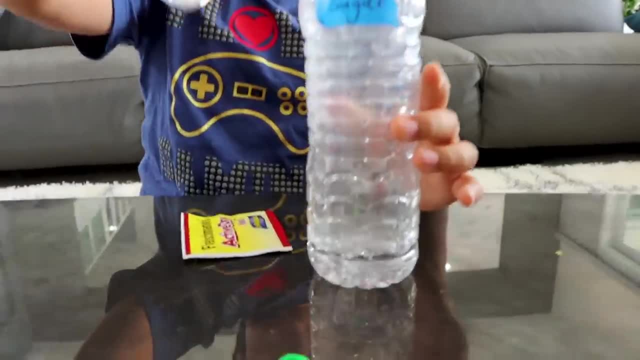 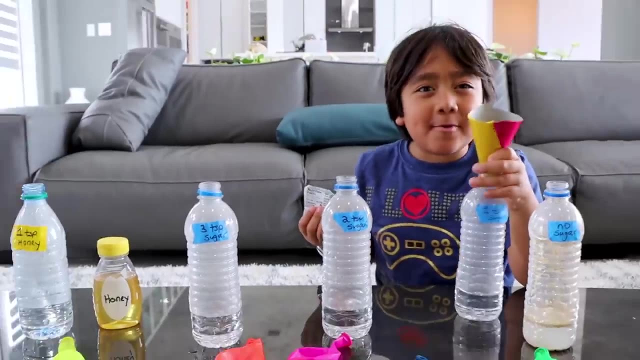 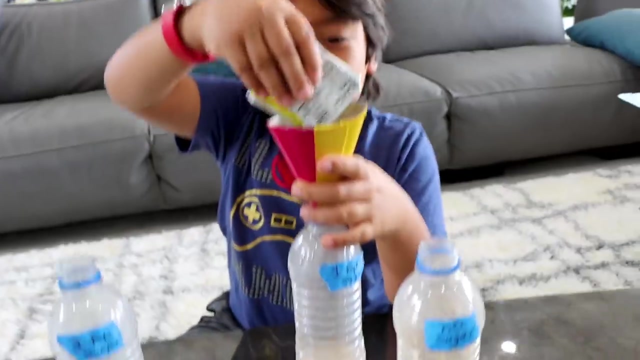 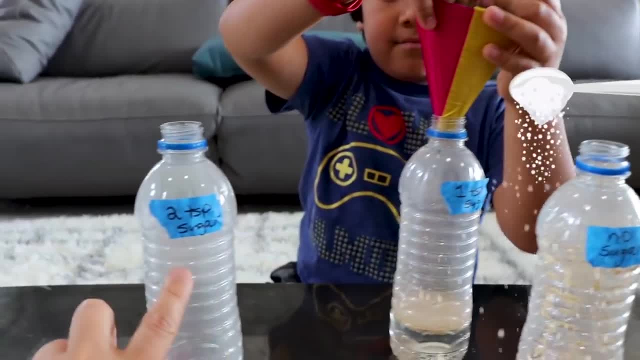 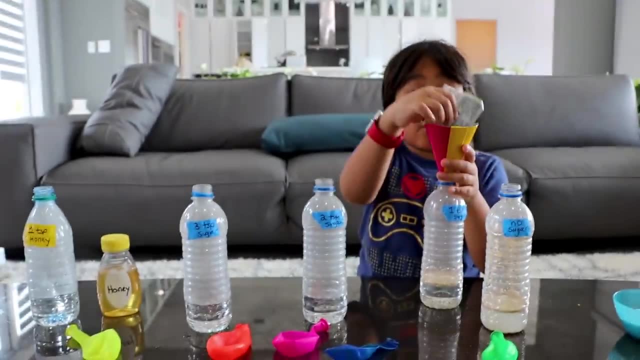 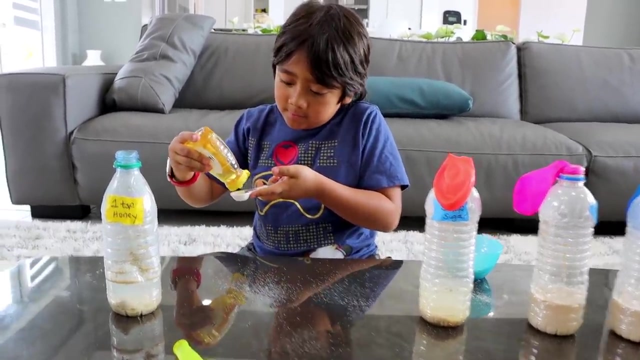 why is this one? we're gonna have no sugar. one teaspoon of sugar, two teaspoon of sugar, three teaspoon of sugar and this one. instead of sugar, we're gonna use honey. yeah, see if it works and how much of a different it makes over here. we're gonna use honey instead. yeah, we're gonna use one teaspoon of honey. whoa. 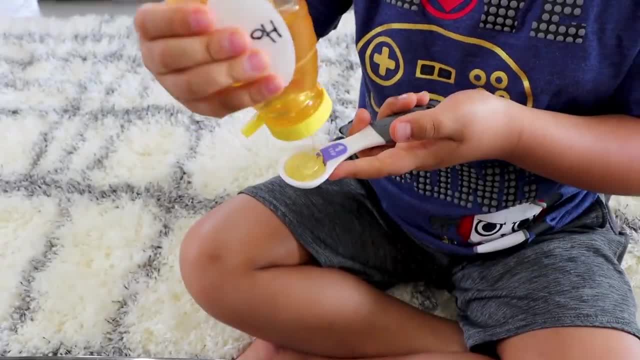 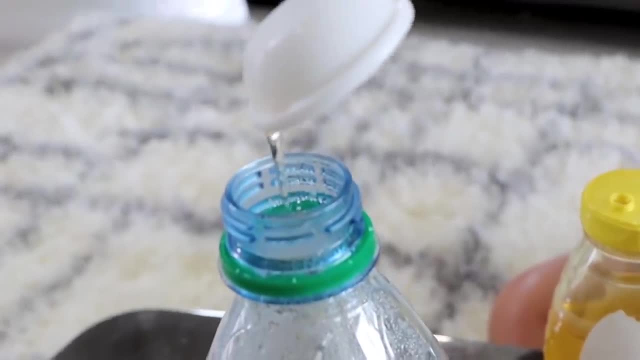 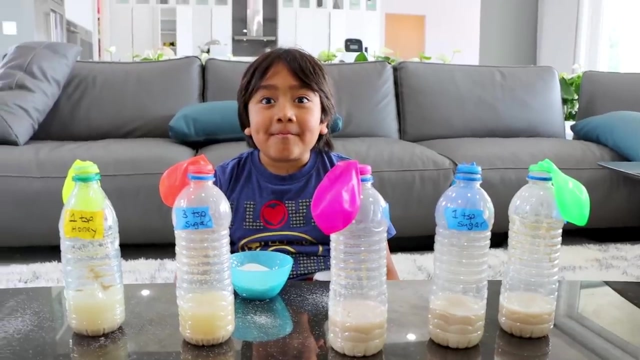 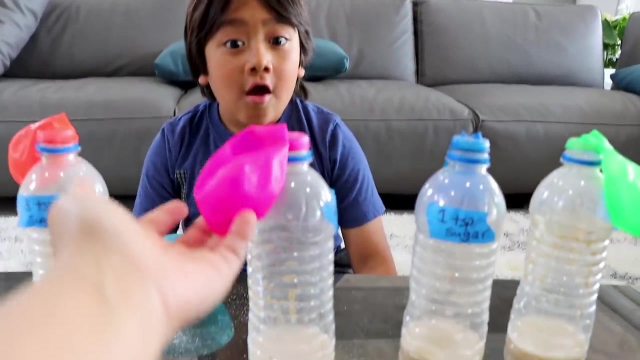 this is a lot of honey. I think that's one teaspoon, mm-hmm, okay, okay, let's put this on. okay, yeah, so, Baker, also put yeast into the bread and the bread will rise, just like how the yeast will also rise up this balloon. okay, okay, Oh. 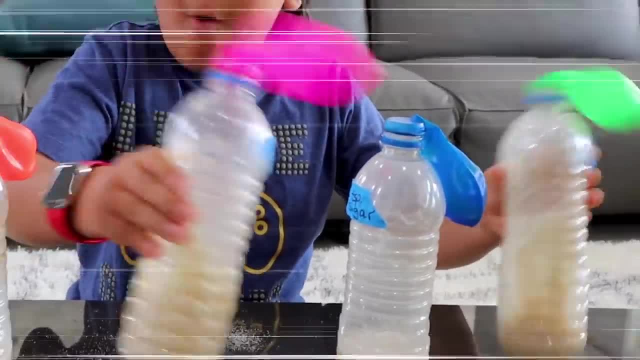 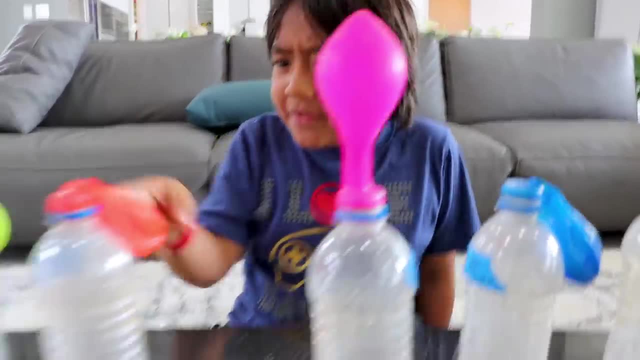 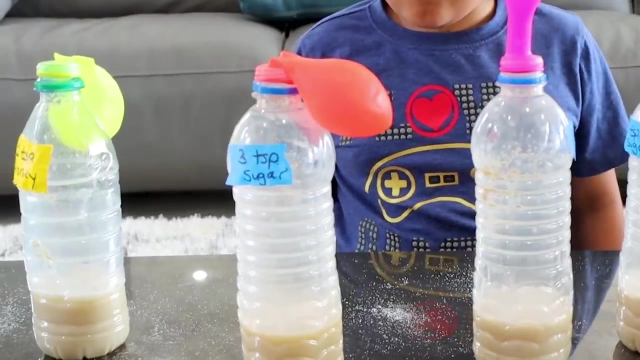 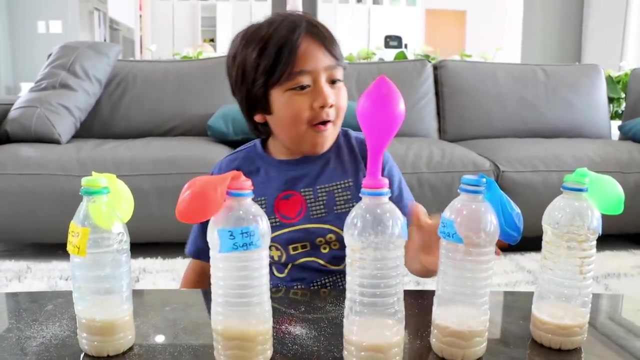 I know it's going up already. what about the third, the one with three? yeah, maybe we didn't shake it hard enough. it's starting to. maybe it just takes more time. yeah, I'll find out. all right, we will be back. yeah, one hour later. hi guys, now we're back. 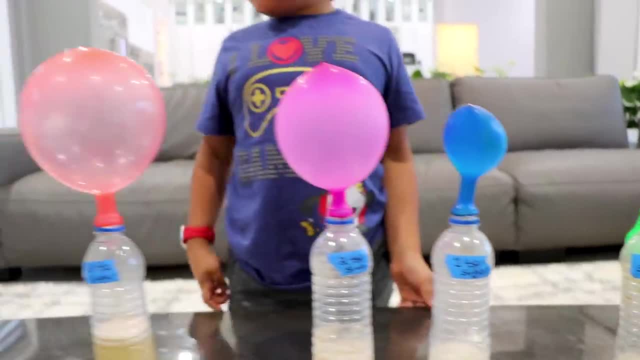 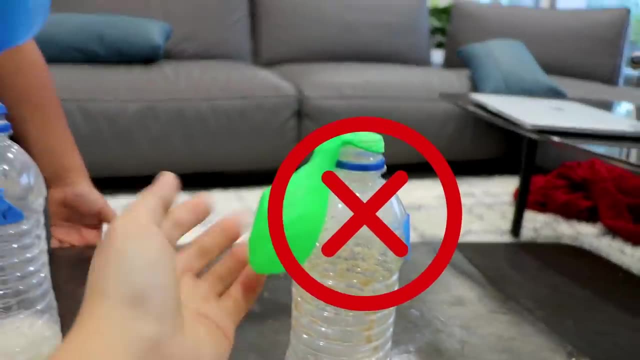 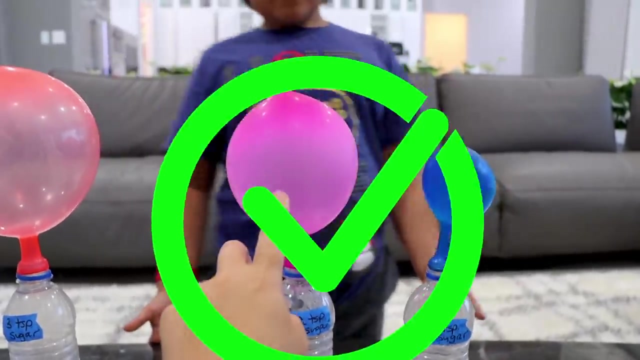 back. all of the ones with sugar and honey worked. yeah, actually moved a little bit, yeah. so what did you notice, Ryan? so the one without any sugar did it work? no, you're right, No site has it worked. okay, cool guys. ryan did it work. yeah, so it did work, or maybe you just missed it. 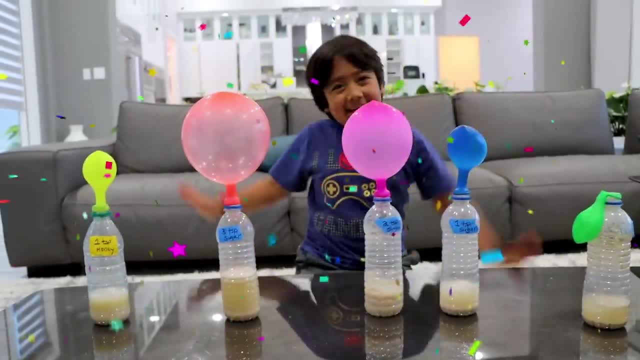 ryan's sugar worked perfect. yeah, ryan, about half of it. it did work five times a handful of this is three siJust to be sure, five pieces full. yeah, oh, that's a lot Arc. I'm so puisque trip. I took it from my add plan on YouTube. back. all of the ones with sugar and honey worked. yeah, so he looked a little bit. yeah. so what did you notice, Ryan, first, as we just came and did we use honey working? no, no, the one with one teaspoon of sugar worked a little bit. yeah, the one with two teaspoon. 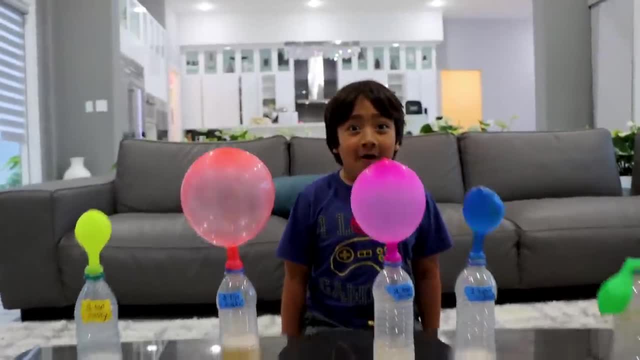 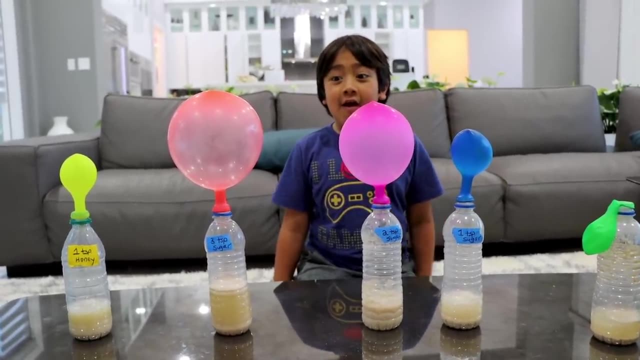 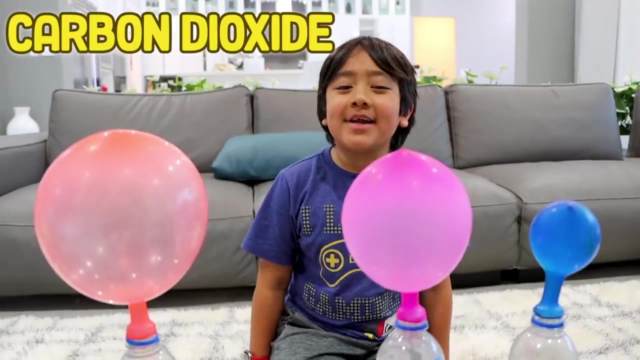 of sugar a little bigger, and the one with three there by the one with three is even bigger. yeah, so they'll give over the zach for you. fermentation, can you say it? fermentation, fermentation, that's right. so the yeast feed on the sugar. and then what came out of it? what's in here? gas, gas, what kind of gas? carbon, oh, carbon. 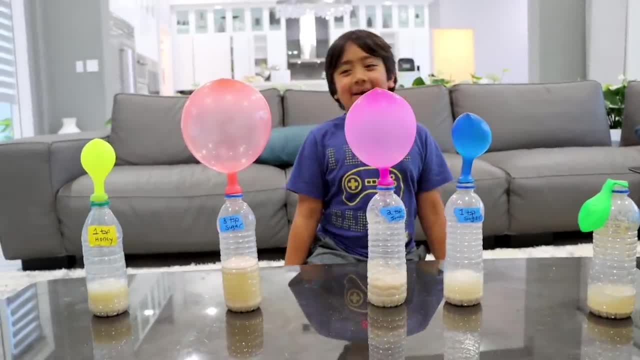 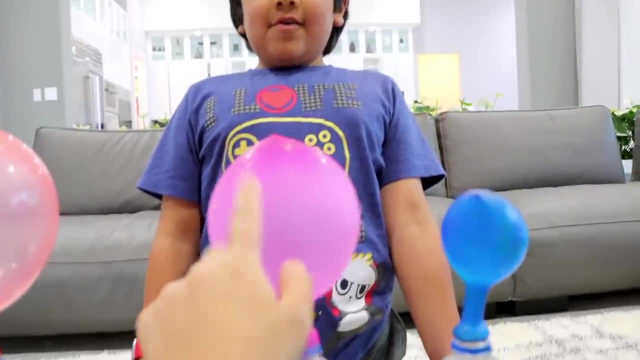 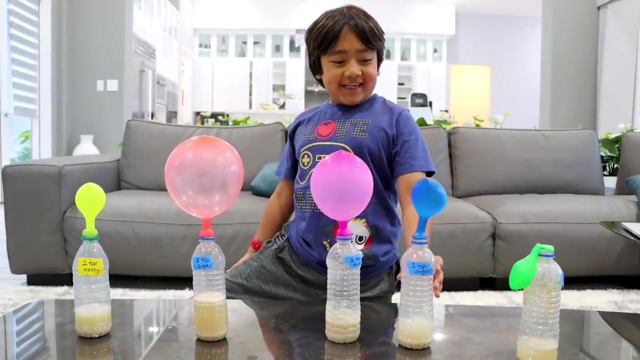 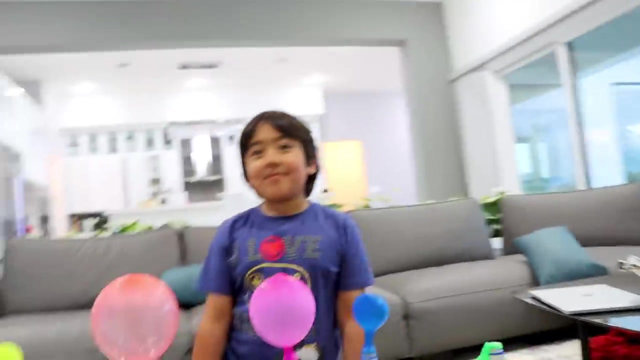 dioxide, carbon dioxide gas, that's right. yeah, it also also releases an alcohol called ethanol, but ethanol stays down here and the gas goes up into the balloon. maybe you guys should also try this out. but instead of one teaspoon, do like one tablespoon. yeah, and lots of honey, right? so instead of honey also, maybe you could use like syrup. 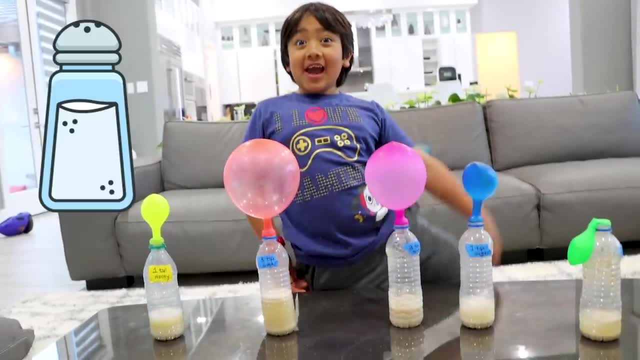 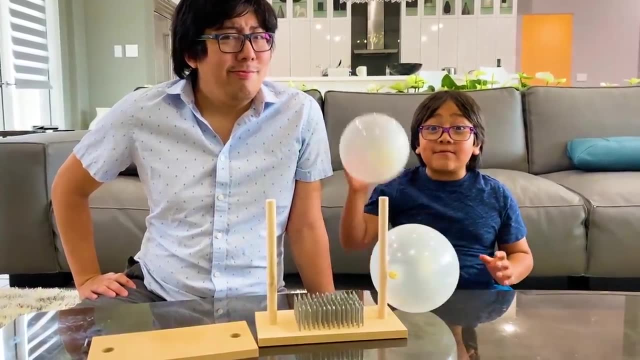 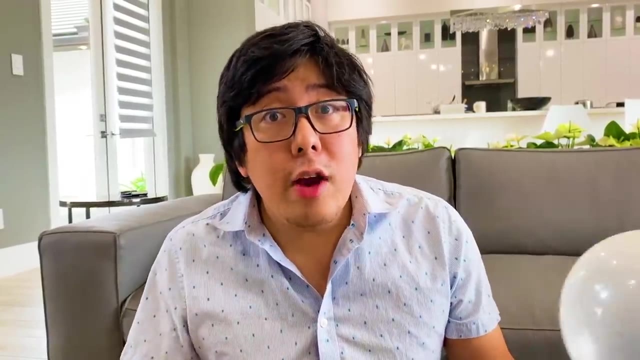 or anything that's sweet. what about salt? what do you think salt will do? right, yeah, if you guys test it out, let us know. hey guys, what do you think would happen if we put a balloon on a bed of nails? so you guys, if you do this at home, make sure you ask your parents for help. all right? so today i'm in. 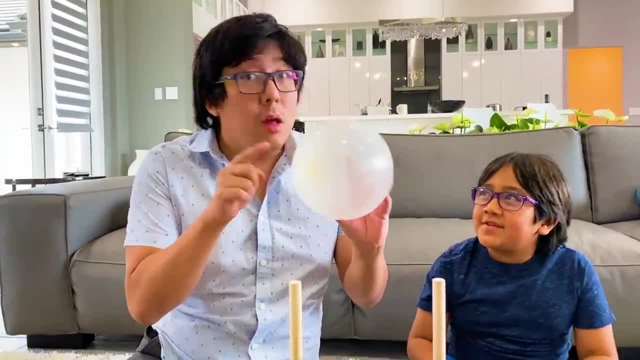 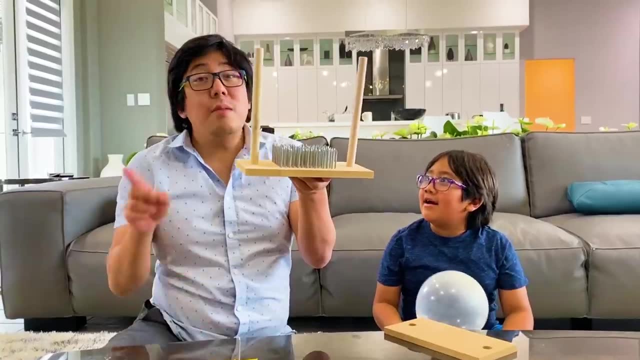 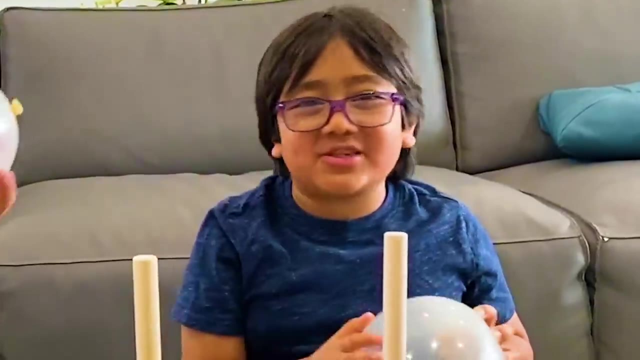 charge ryan, yeah. so what do you guys think? do you think the balloon's gonna pop or stay the same on top, yeah, on top of this nails. instead of trying it out with a lot of nails, let's do it with one. let's see what happens. i think it's gonna pop if you put a lot of pressure. 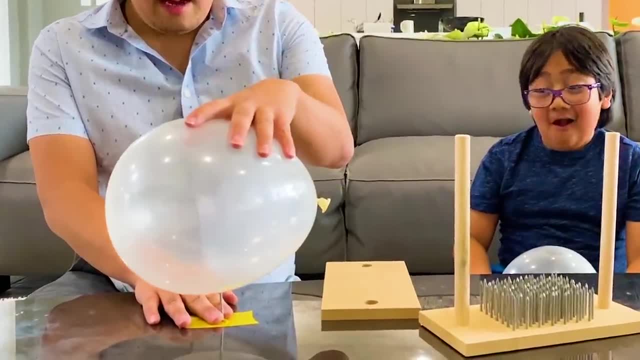 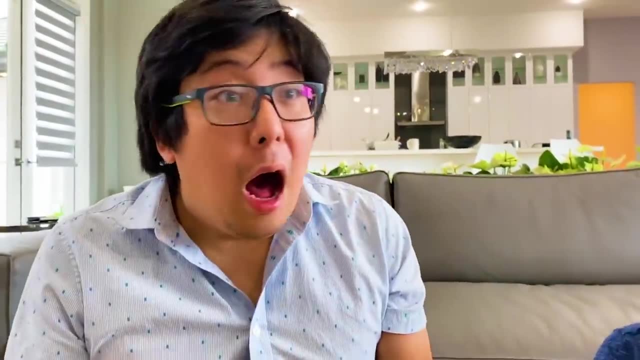 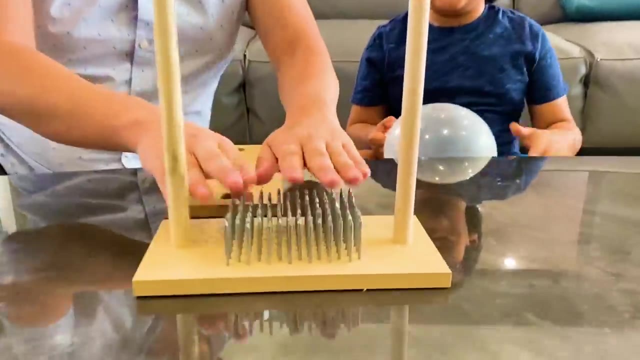 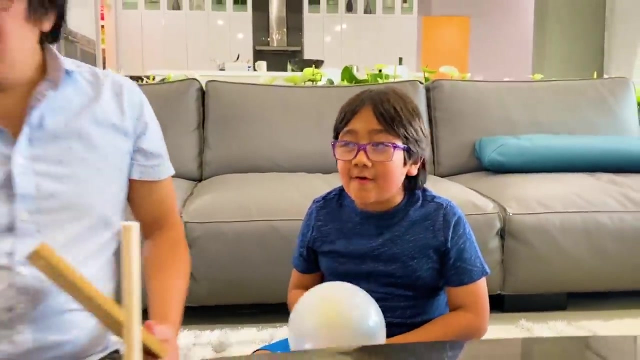 all right, let's see what happens. you guys ready? yeah, all right, try same pressure. all right, so, guys. so now let's try the same thing with a lot of nails. yeah, guys, remember there are a lot of nails, so remember, ask the grown-up for help. yeah, because they're pointing right, so you don't. 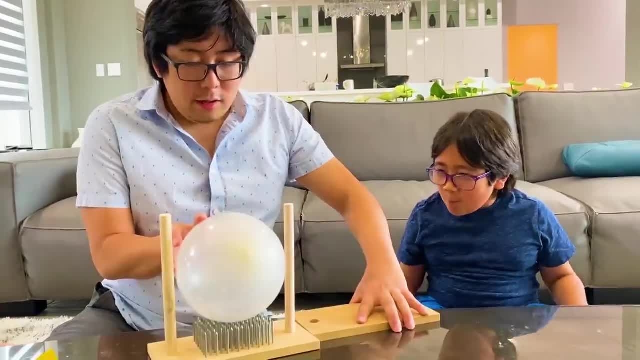 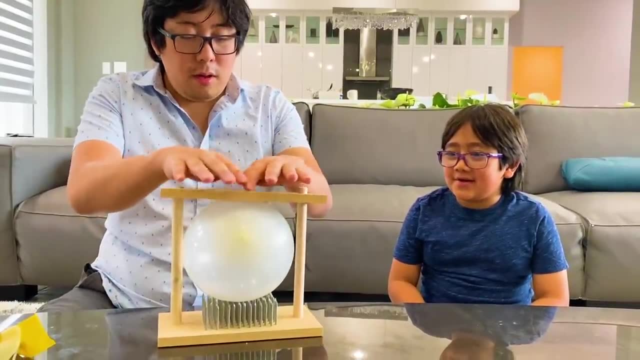 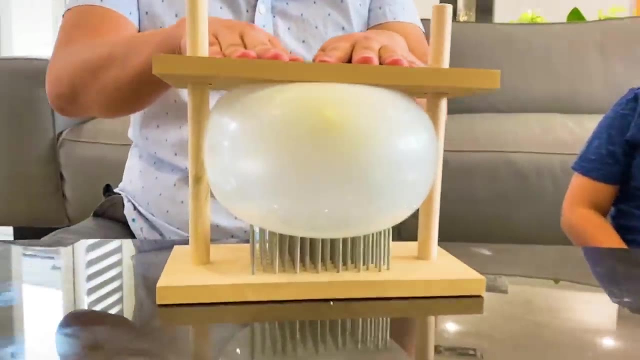 want to touch it here? all right, you guys ready? so set balloon. i think i know what's going to happen and i'm going to use this board so it won't go up in here. ready, press it, good guys. i'm pressing really hard, but it's still not popping, you see it. 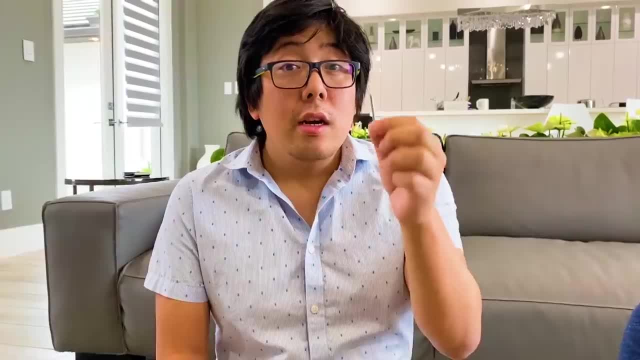 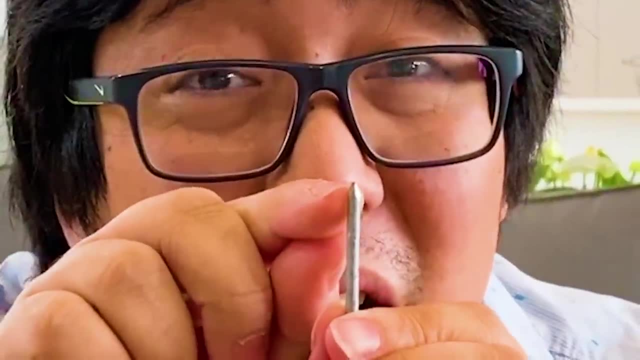 how come there's so many nails, daddy? but it didn't pop the first time. we apply the force into one nail, so the area that we apply the force is very tiny area right here, okay. second time we applied same amount of force, but this big of area. 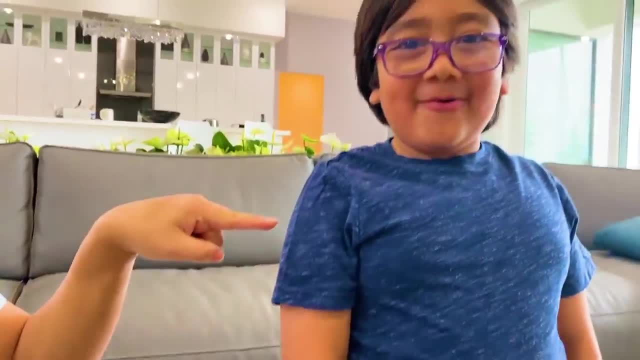 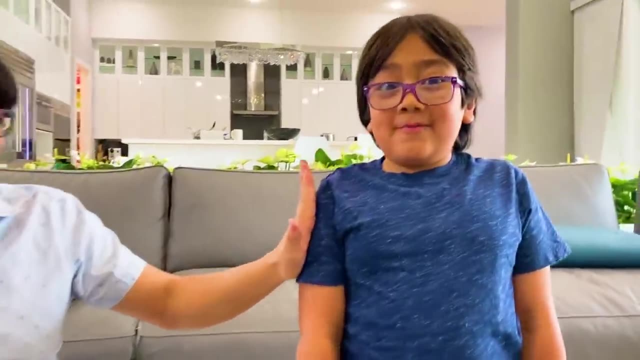 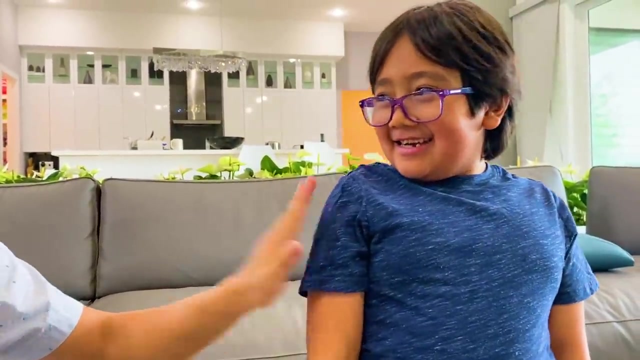 for example, if i press you with my finger out, right, so then same amount of force. but if i do it with my palm, doesn't hurt, right? no, but i'm applying same force but in different areas. but, daddy, can we see how much force it takes to pop the balloon? 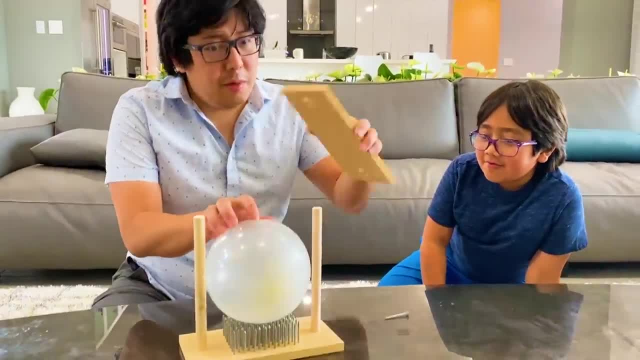 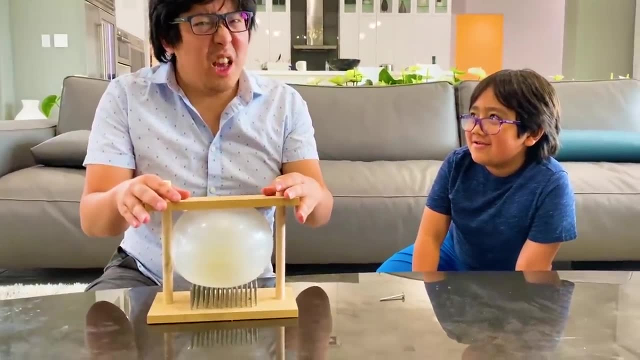 with the giant area. all right, let's see, because earlier we couldn't pop it, that it was like all the way down here. all right, let's see, because earlier we couldn't pop it, daddy, it was like all the way down here. but if i press it on my hundred percent force, what's gonna happen? 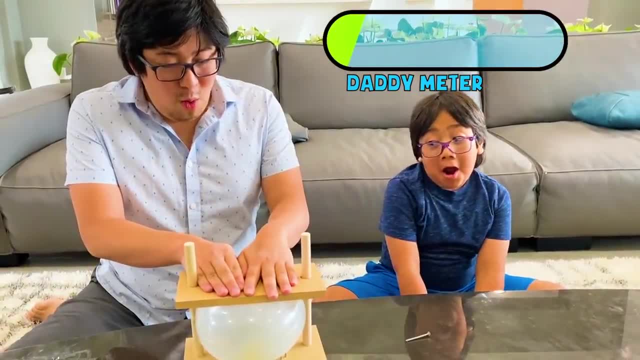 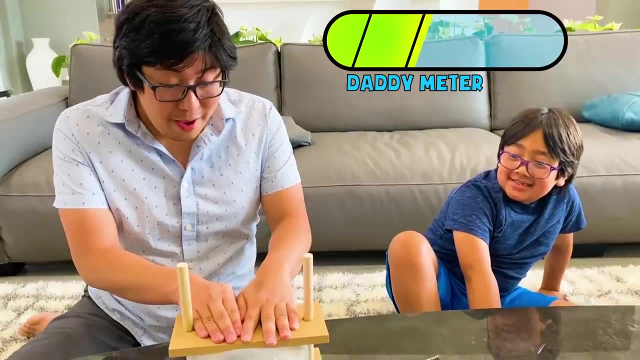 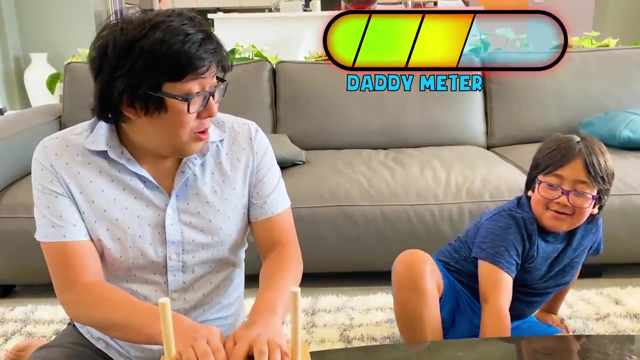 are you doing a hundred percent? no, not yet. oh my gosh, it's still not popping. can i even pop? no way, it's still not popping. are you at a hundred percent yet? yeah, oh my gosh, you ready. i'm gonna reach my hundred percent, you ready. 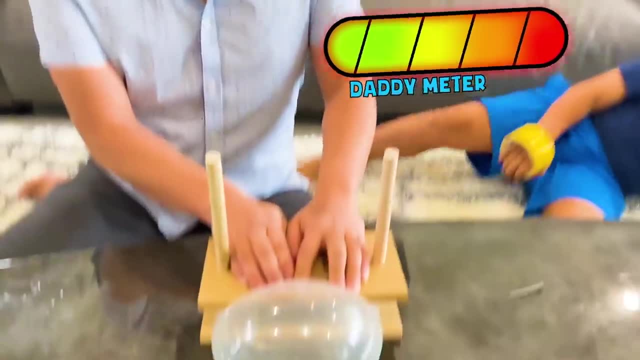 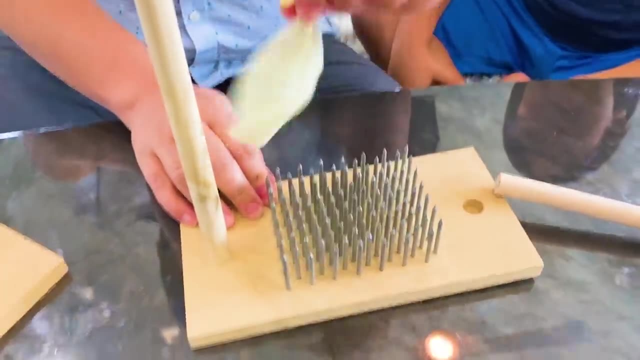 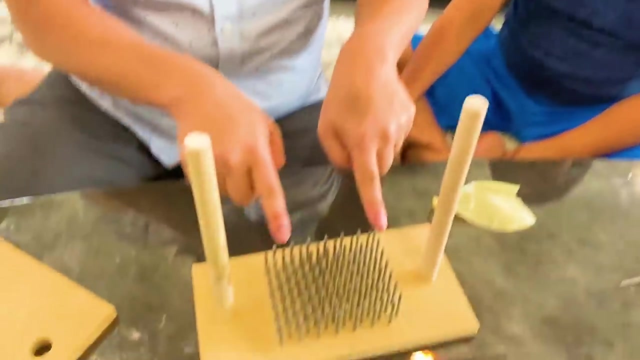 still not popping. look at this, look at that. oh, look at that. whoa. oh, that was hard, but did you see how much force i applied? yeah, because the area was so much bigger, so i have to place a lot bigger force to pop the balloon. that was so cool, so now we're gonna see it. 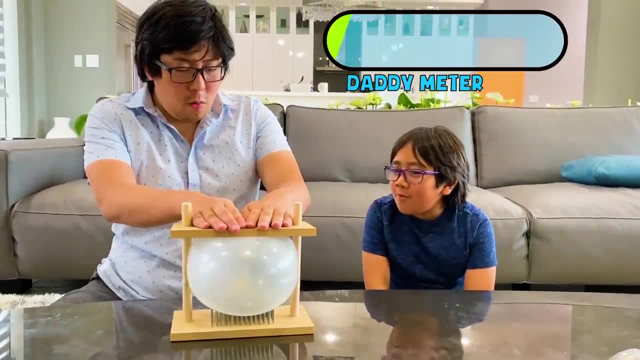 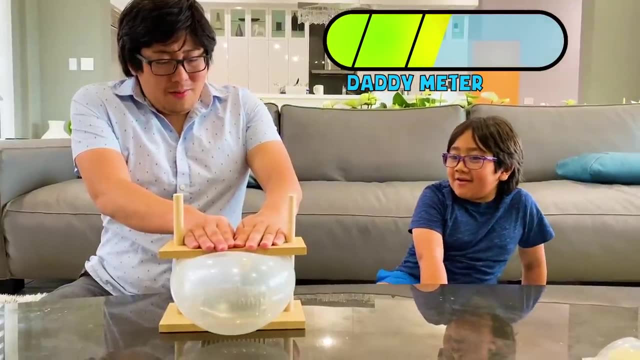 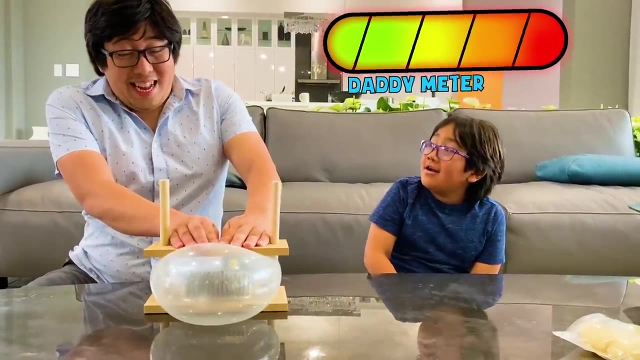 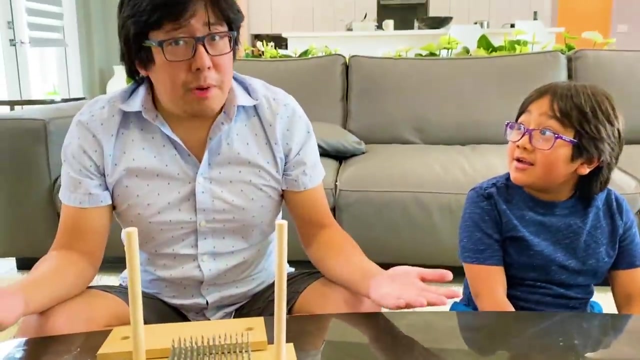 in action again. all right, let's go whoa again. i'm pressing a lot, pressing a lot. you have to go all the way up to go all the way back down again. still no, whoa, almost all the way down. that was so cool. yeah, this experiment teaches you the concept of pressure. 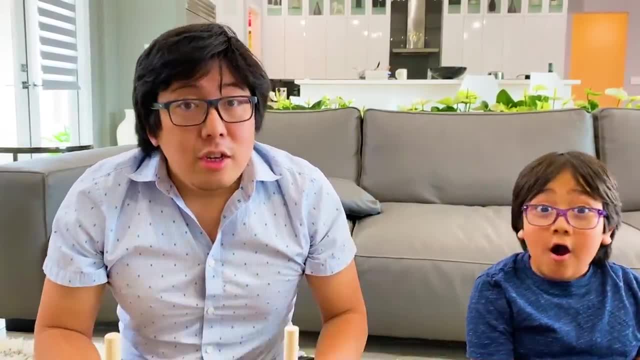 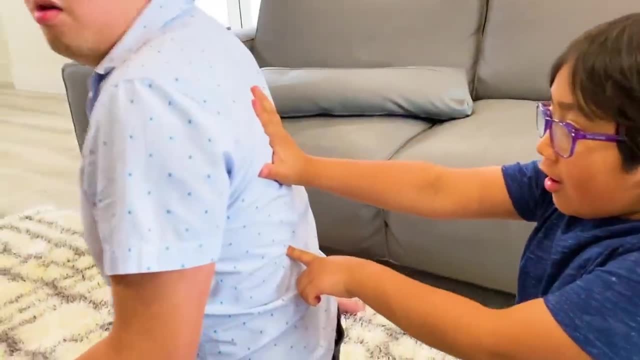 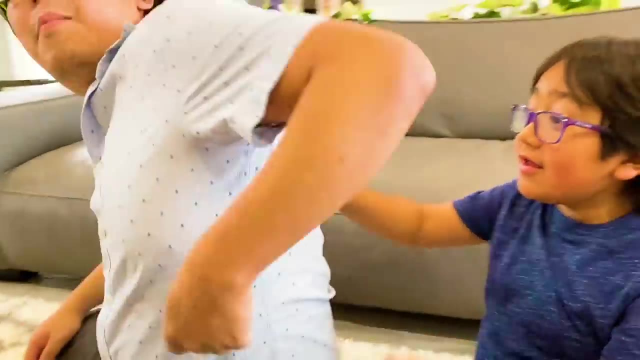 the pressure is the amount of force applied over the area. so the smaller the area is, the higher the pressure. for example, with the same amount of force but applied in a smaller area, It makes the pressure higher. Ow, Your finger hurts, Ryan. So same amount of force, but the one you're pressing with your finger. 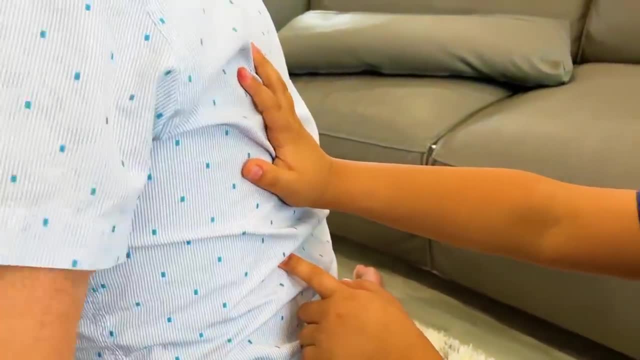 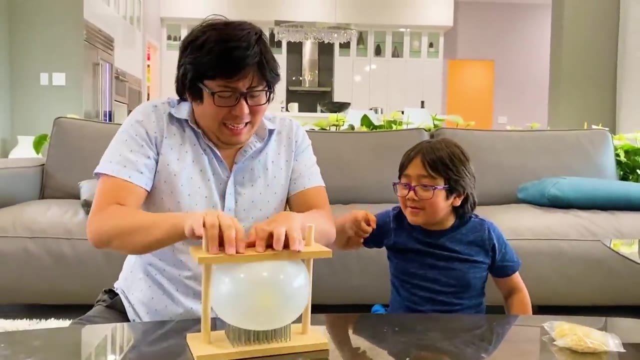 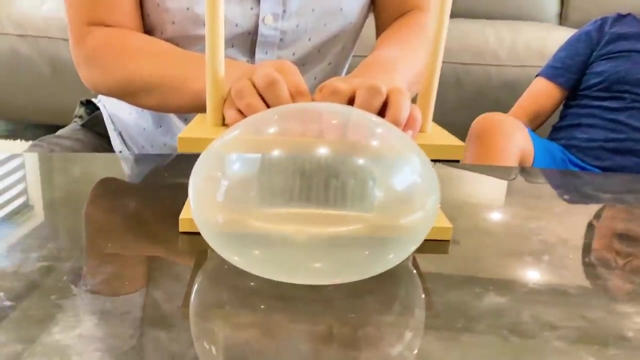 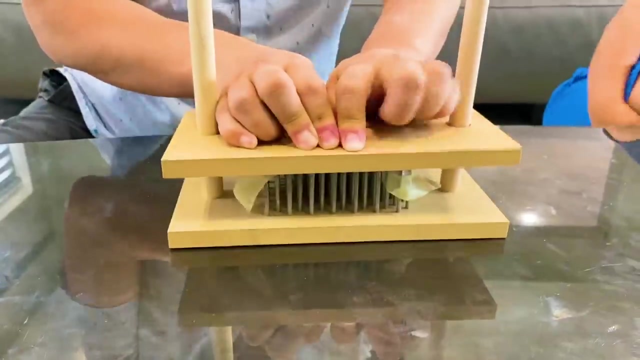 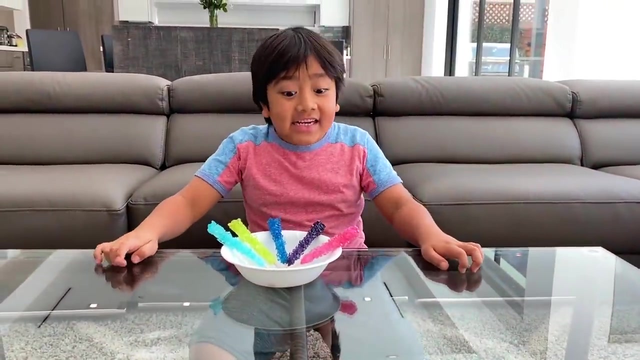 is higher pressure than the one you're pressing with your hand. Okay, guys, remember, always stay happy and rise up. Bye, We're going to pop another balloon now. See, it's really hard Rock candies. I wonder where these came from. 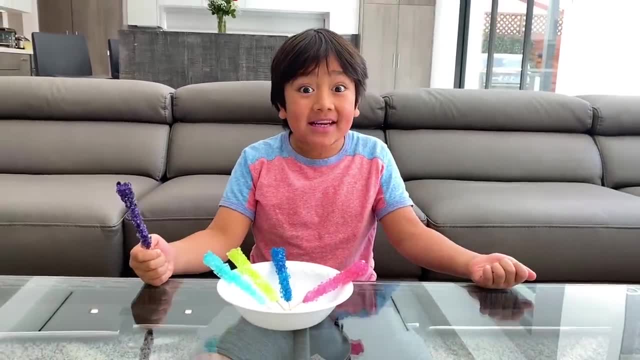 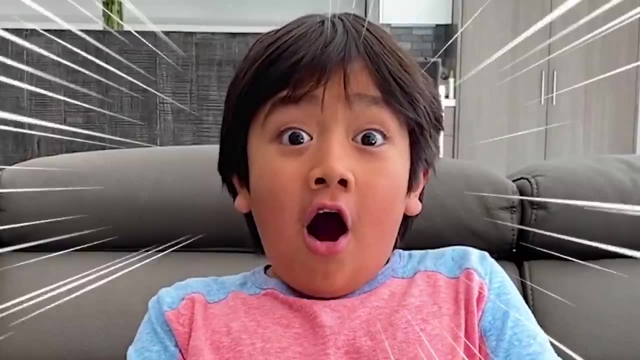 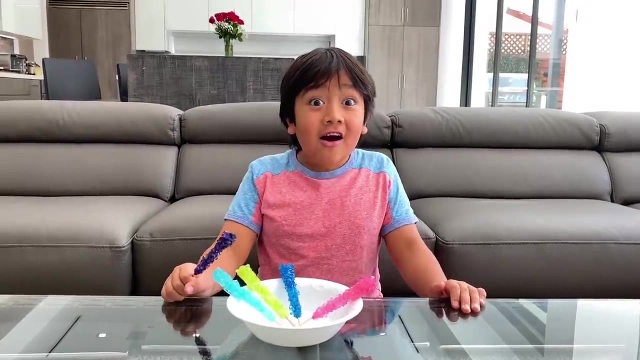 Whoa, I wonder how these were made. Hey Ryan, Hi Peck, Did you know you can make rock candy at home? You can. Yeah, Ha-ha, Want me to show you how Sure, Then let's go. 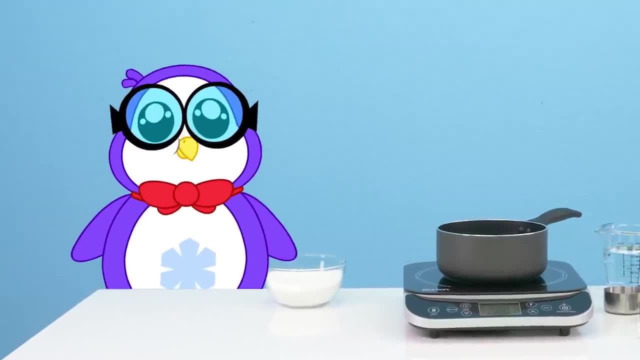 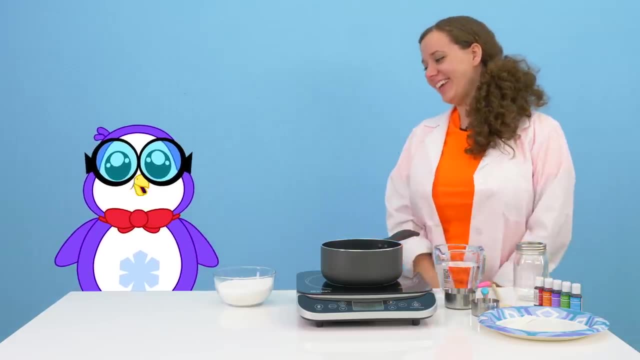 Okay, I got this. Um um, maybe just a pinch of sugar. Hey, Peck What you doing? Oh gosh, Definitely not eating sugar. Uh-huh, This looks pretty cool what you got going on. 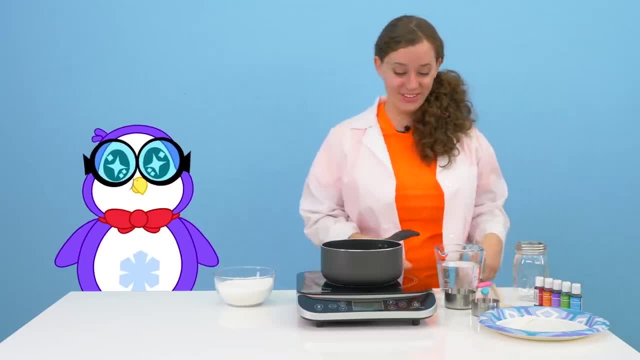 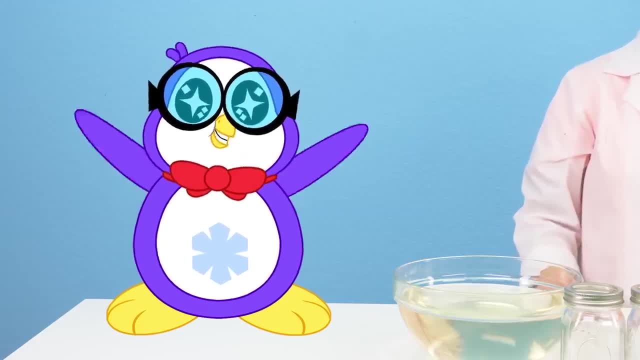 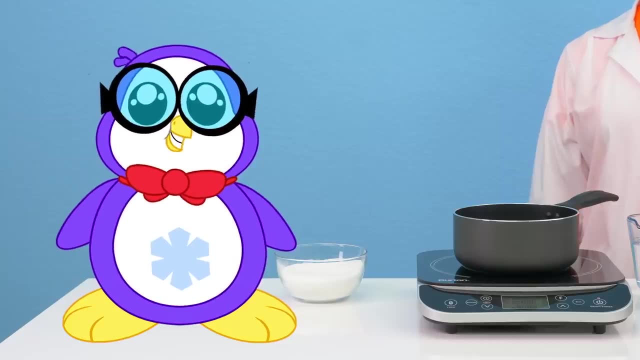 Bink: Sugar, Sugar, Sugar, Sugar. He really likes candy. Let's get started. And it looks like geodes, which is cool and it's the best. And it's also on a stick, so it's easy. 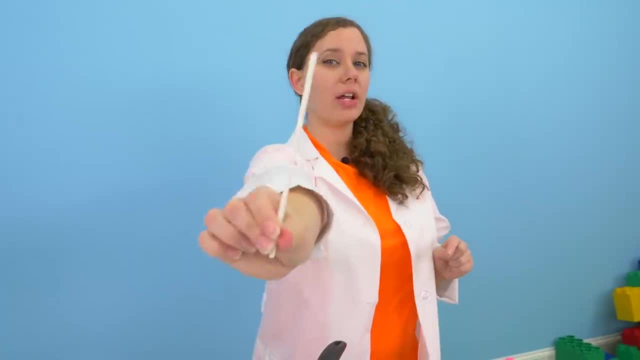 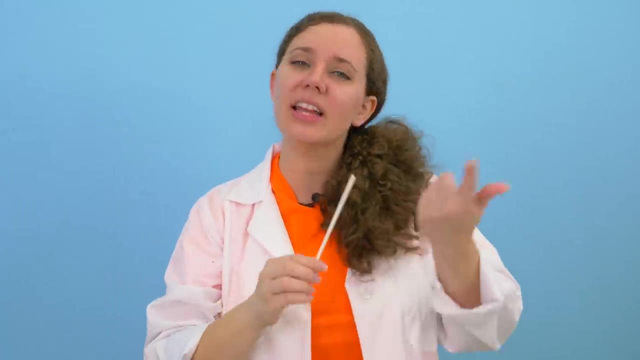 The first thing that we're going to do is build the very center for our rock candy. Now we are going to use these paper sticks- Mmm, Paper sticks. You don't eat the paper stick. It's kind of like what would be in the center of a lollipop. 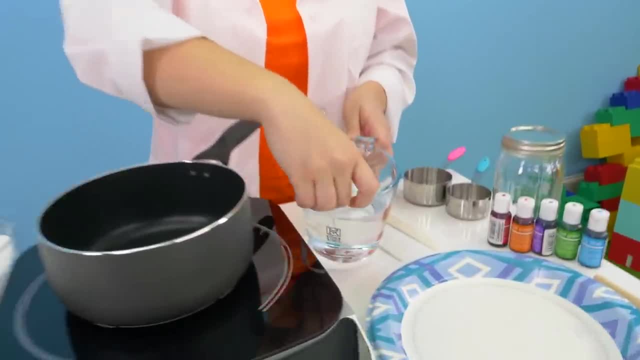 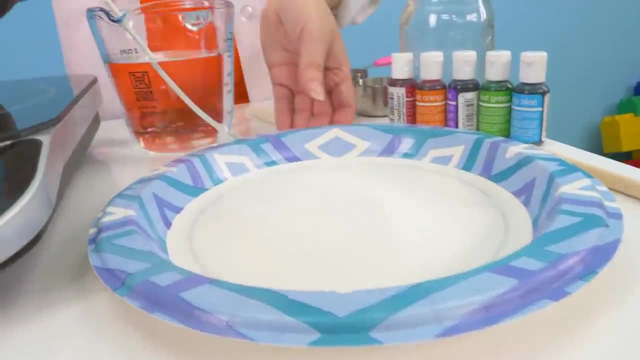 We're going to take the stick. We're going to dip it in water like this. Well, we need sugar too. We definitely need some sugar. So let's get some sugar on a plate. Perfect Yay, Sugar, Woohoo. 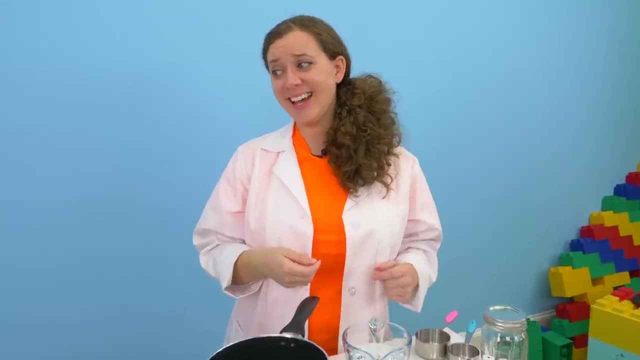 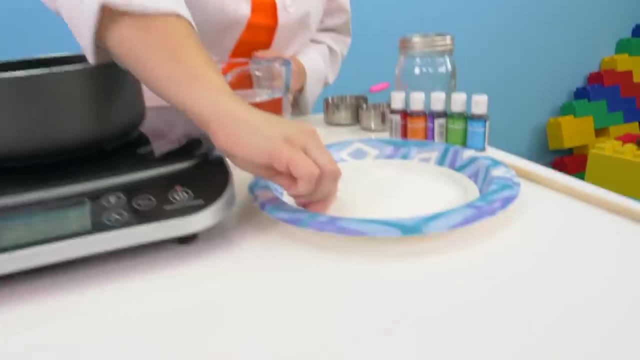 Sugar, Sugar, Sugar, Sugar, Yeah, sugar. There's going to be a lot of that. Now that we have our stick all nice and wet, we're going to roll it around, Get some sugar on here And it should look something about like that: 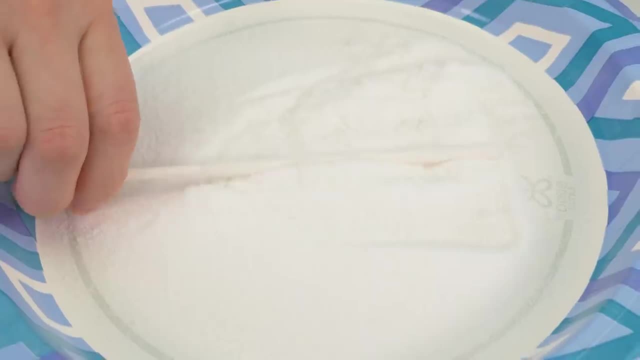 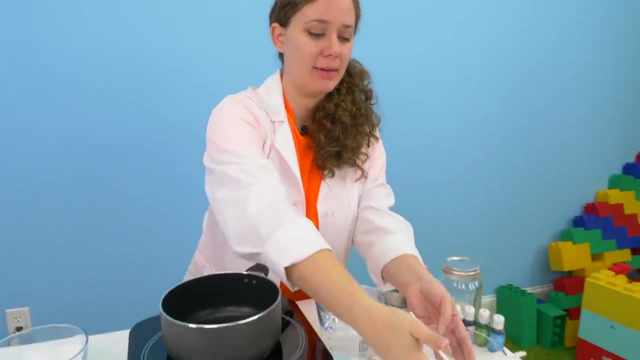 And then we're going to roll it out, which this will give our rock crystals plenty of stuff to grow on. Now that we have all of our sticks coated in sugar, we're just going to set them aside and let them dry so we can use them later. 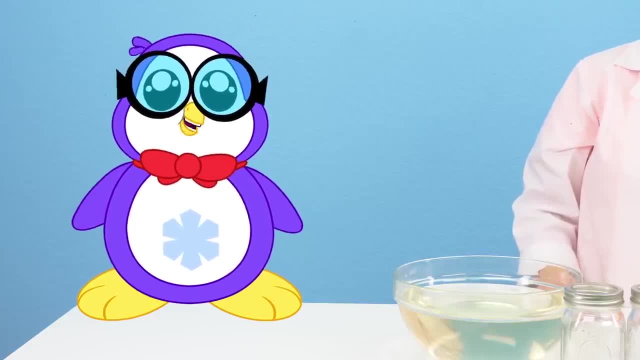 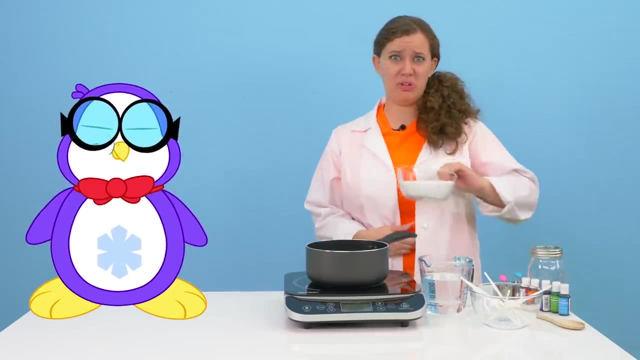 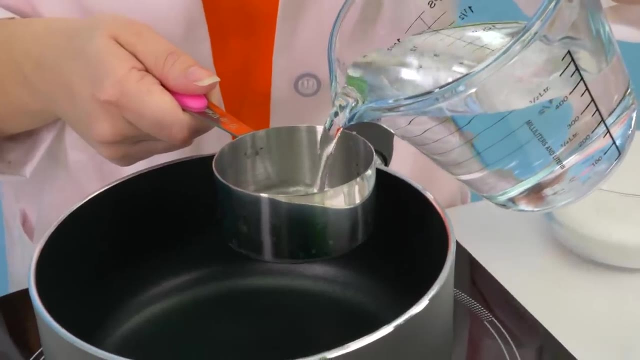 Now we can commence with the creation of our rock candy. That's right, Peck. Maybe I should just take this sugar away and put it over here. So the first thing we're going to do is add water. We are going to add one cup of water, which all I could find was a half cup measuring cup. 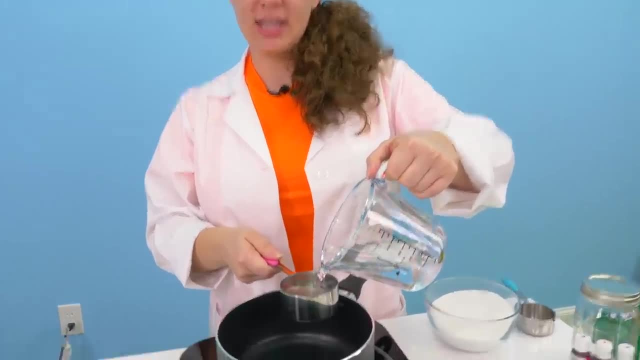 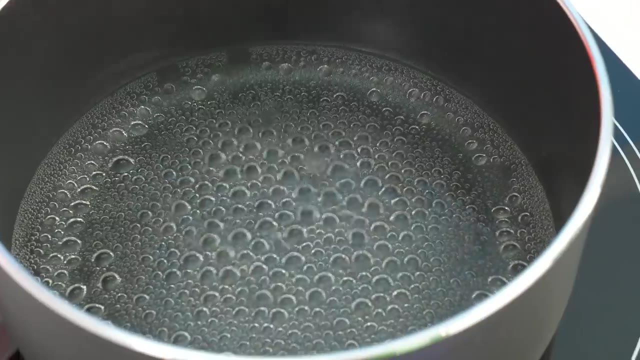 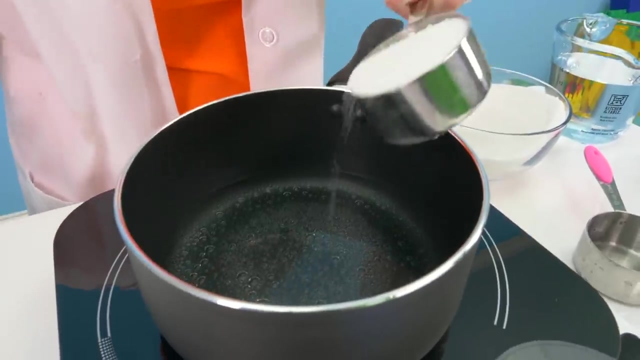 So we need two of them. Then we're going to turn on our cooktop and we're going to turn it on boil so we can get it cooking. Ah, Bubbles. Now we're going to add our sugar. We're going to slowly mix it in. 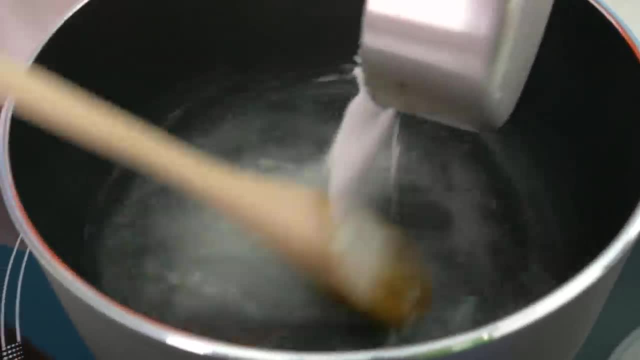 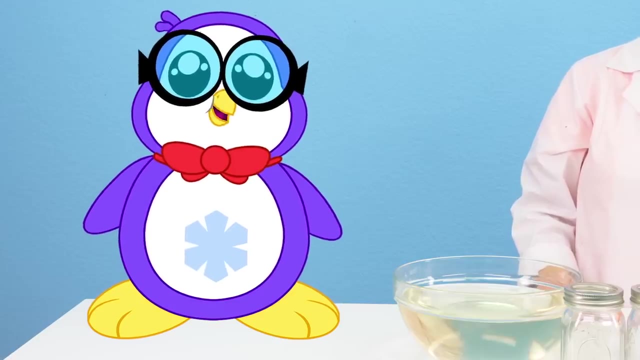 We're going to try to use about two-thirds of our sugar Two-thirds cup, But we have to make sure it dissolves fully in the water. We have a bowl of sugar water now. What are those jars for? Well, that is a good question, Peck. 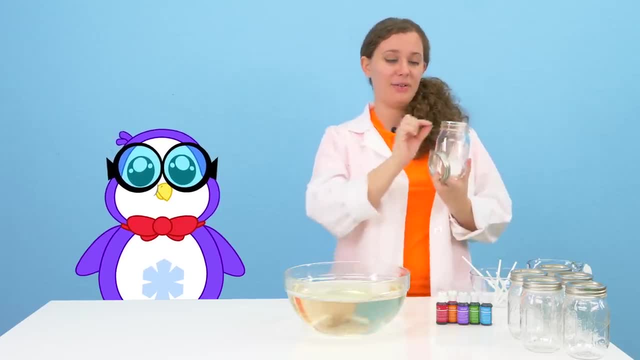 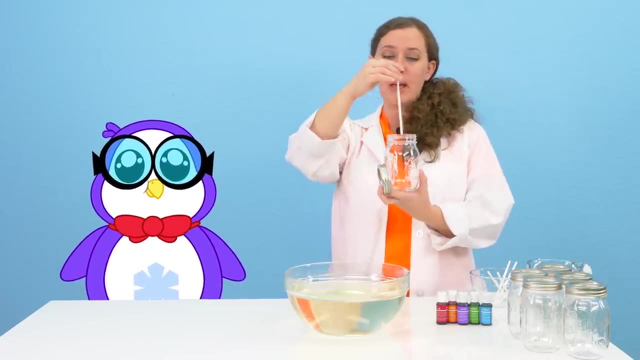 We are going to use all these different jars to grow our individual rock candies. Now, we don't need the lid, because this is actually going to go in here just like that and grow all of our crystals. What about the color? I want to see a rainbow. 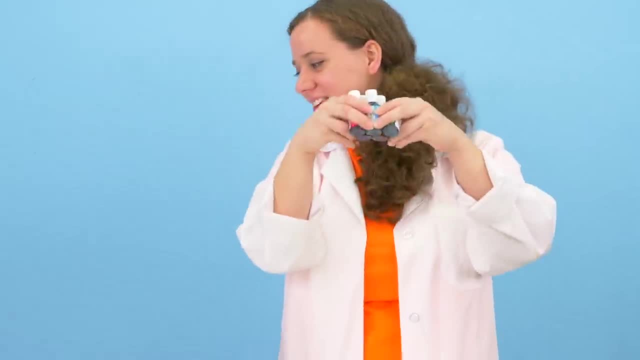 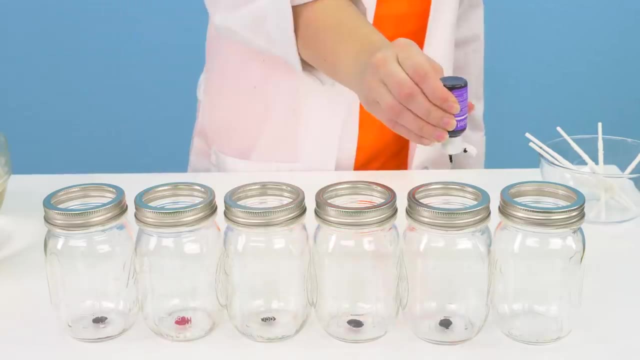 Well, Peck, why do you think I have all this food coloring right here? For our rock candy we're going to make red, orange, green, blue, purple, and I think I'm going to leave the last one clear, because I just want to see what the regular rock candy looks like. 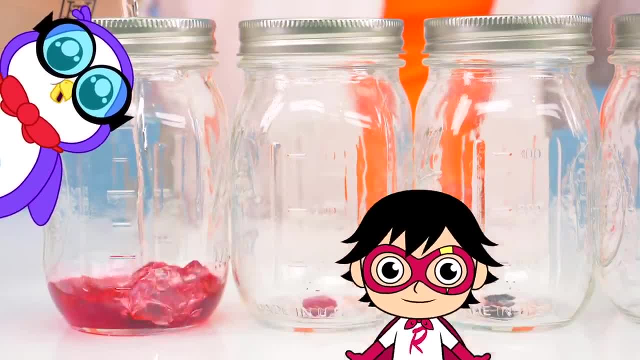 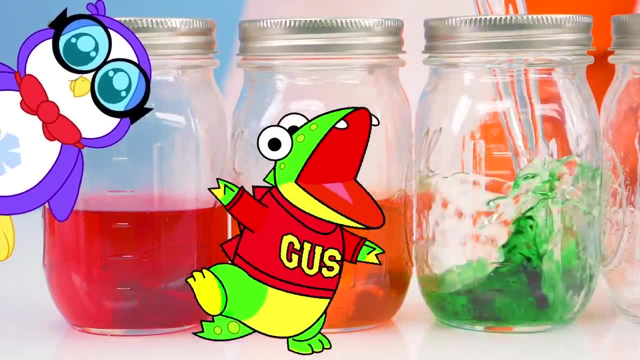 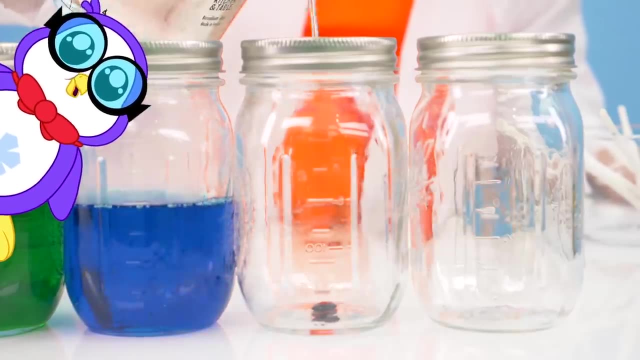 Red like Red Titan, because he's super red. Orange like Moe- he's so crazy. Green like Gus, because he's a gator. Blue like Gil, because he's super chill. Purple for Peck, because purple's the best See-through, like a ghost. 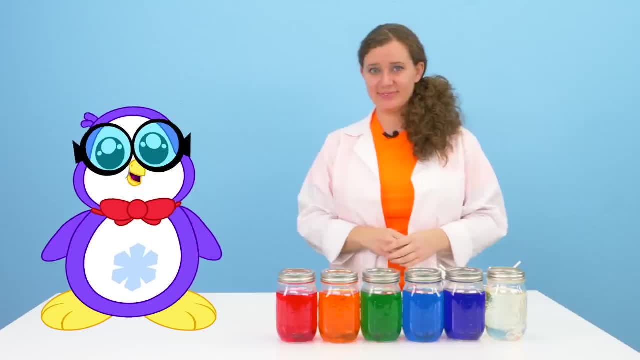 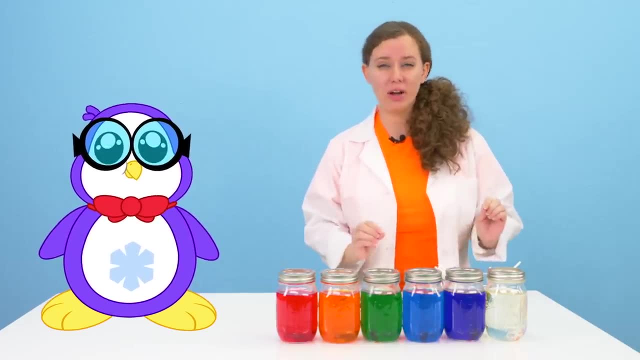 No one's kind of scared. La, la, la, la, Wow, Peck, that was really something Moving on. the last thing that we have to do to make our rock candy is we just take the center piece, our sugar sticks, and then we just put them right in the center. 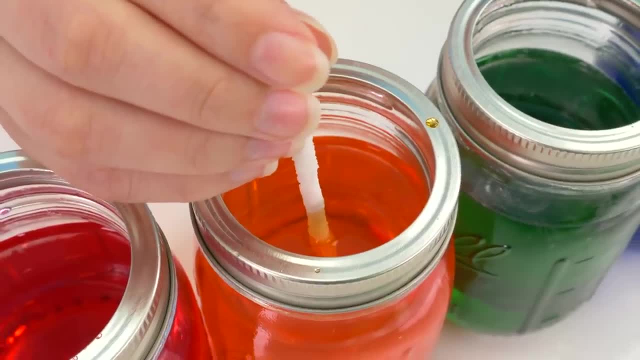 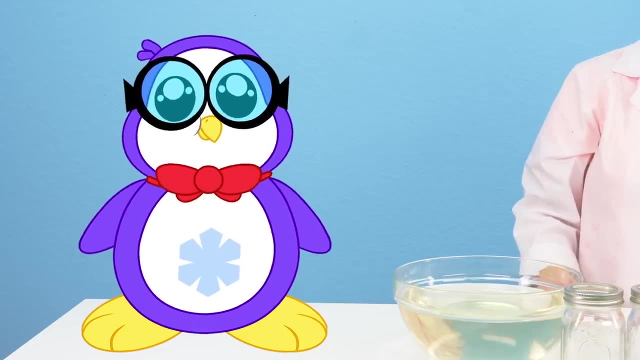 And wait, we need to hold it in place. and well, I don't have six arms and if I let it go it's going to fall off, And oh no, Oh, don't worry, Bree, I know what we can use. 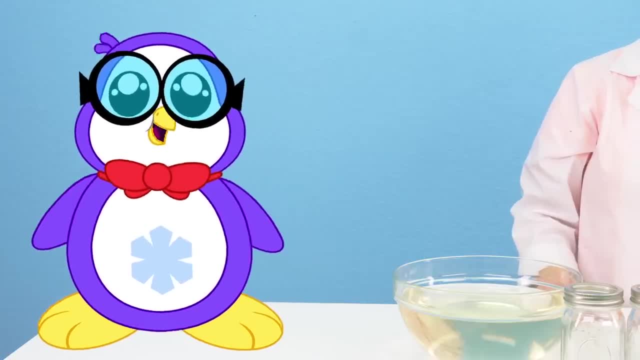 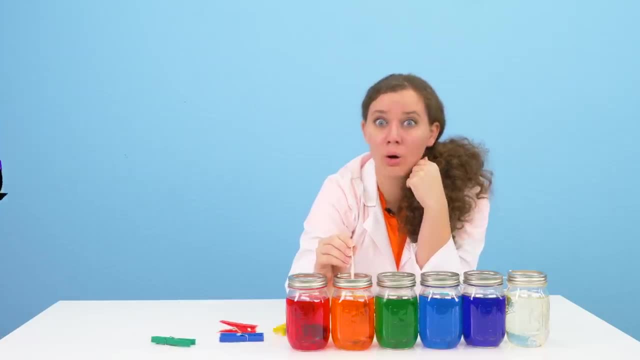 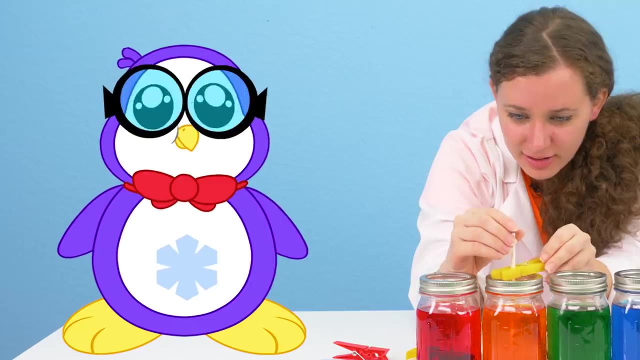 Okay, Peck, hurry, Be right back. I sure hope Peck gets here soon. I'm getting so tired. Hey, these are perfect. Oh, that is much better. It was a success. Now we can start making the candy. 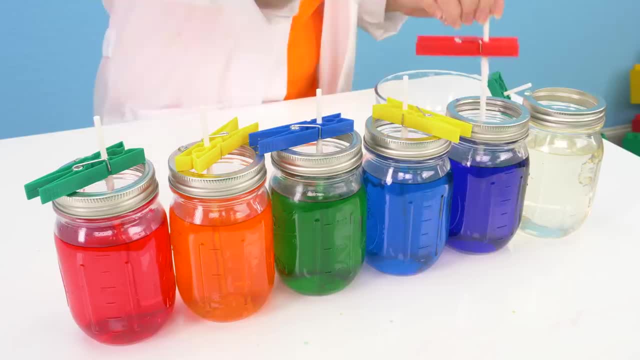 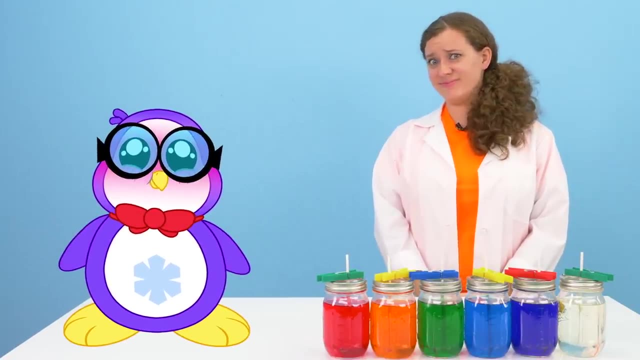 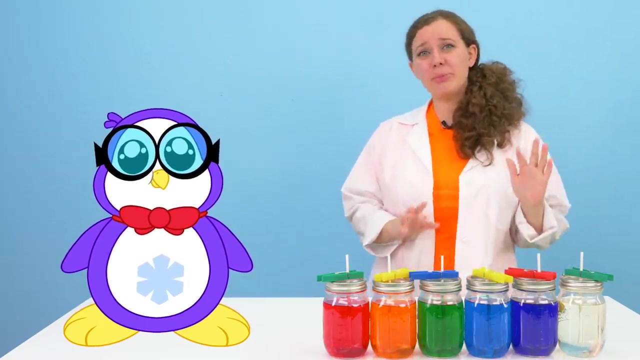 Hmm, hmm, hmm, Oh, ha ha ha. yeah, How long do we have to wait? Like five minutes, Oh, I mean 10 minutes, 30 minutes, No Peck, it's going to be more like five days. 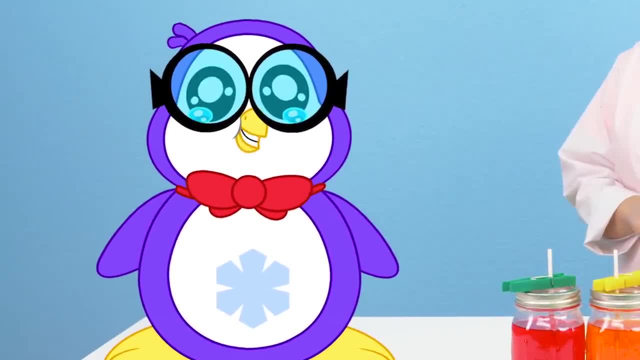 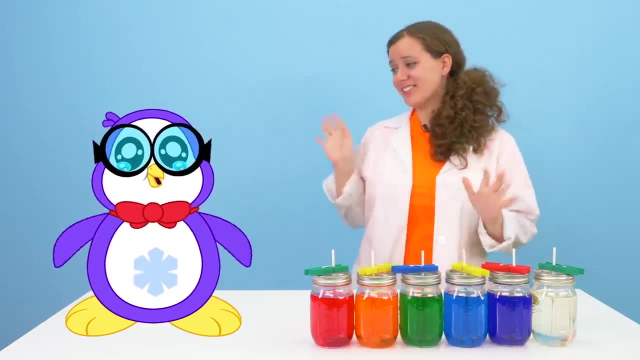 Five days, What? But that's like 7,200 minutes. No, Okay, I'm just going to go. Don't worry, Peck, You got this. I'll see you in five days. Bye, Bye, Bye. 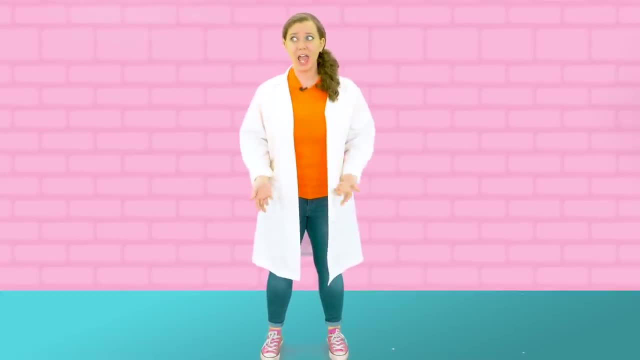 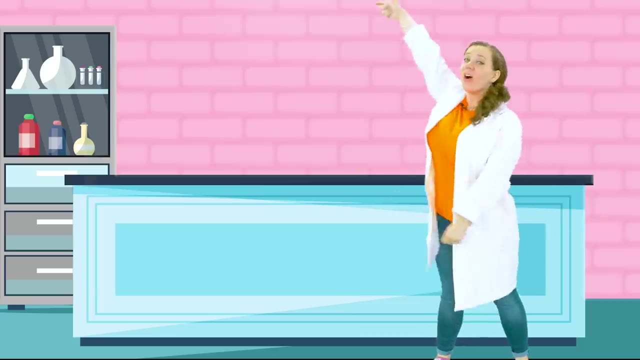 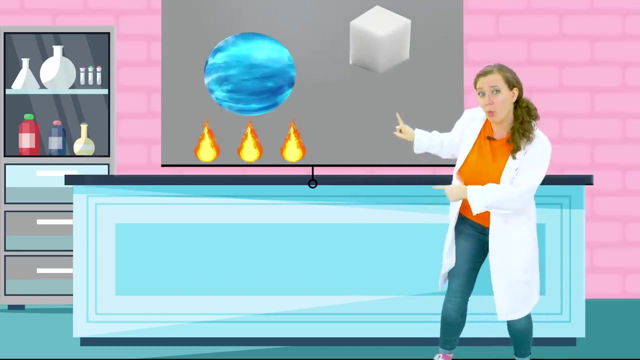 Bye. Well, since we're just waiting here, how about we take a look at the science behind rock candy? So water and sugar are both molecules. Now, when we heat up the water, the water molecules spread apart, and then we're left with all. 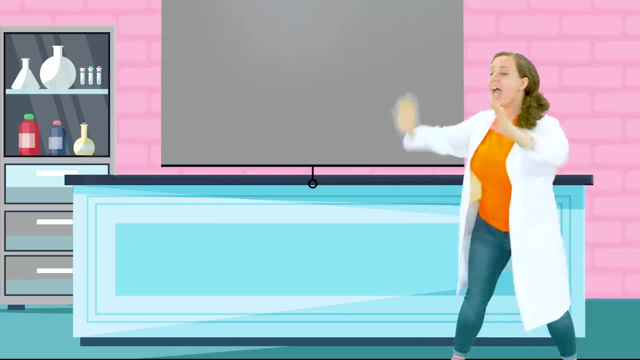 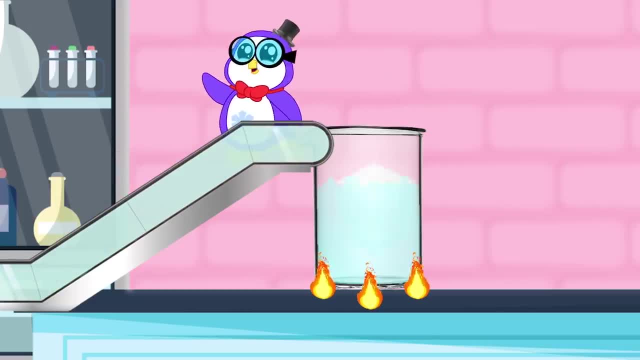 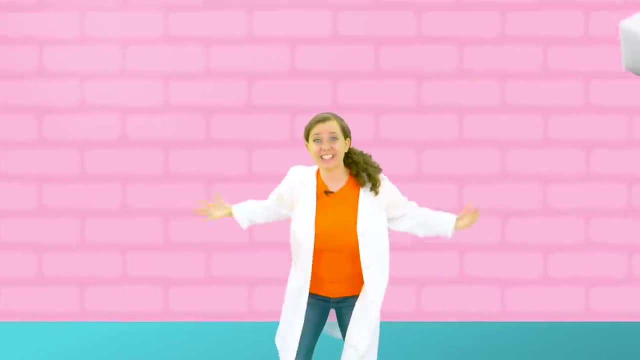 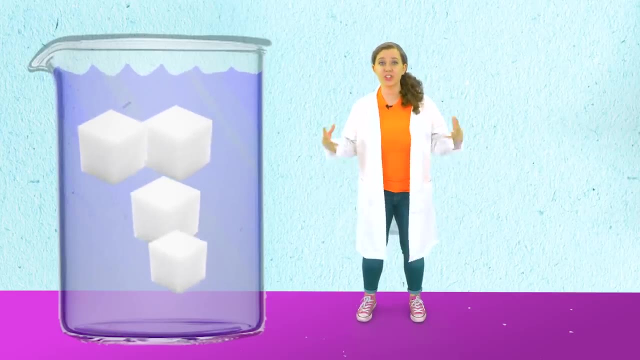 Ha ha ha. Great job, Pecks. Now that we have all this sugar, this is called a- Super Saturated Solution. As our solution cools, the sugar begins to crystallize and these crystals form more and more. 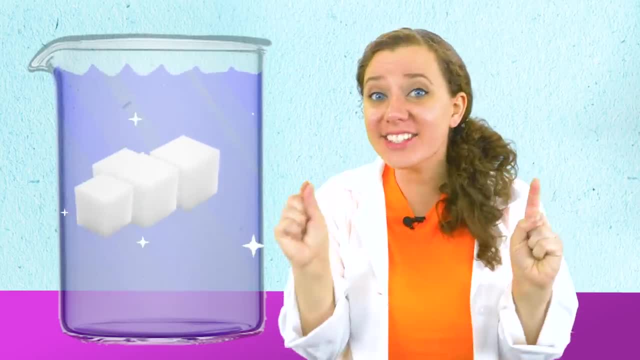 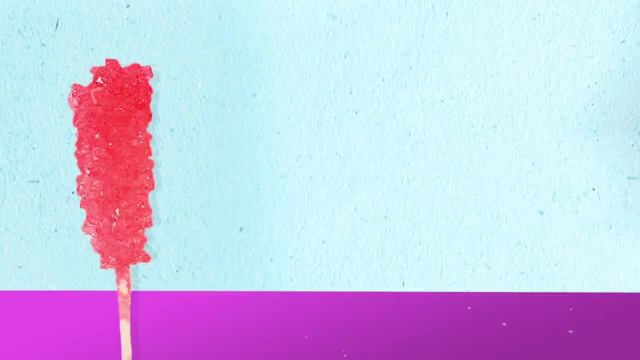 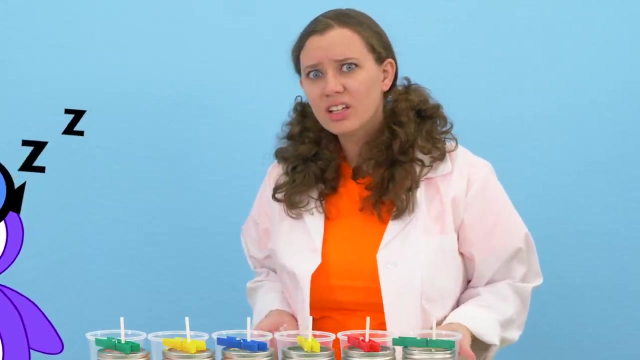 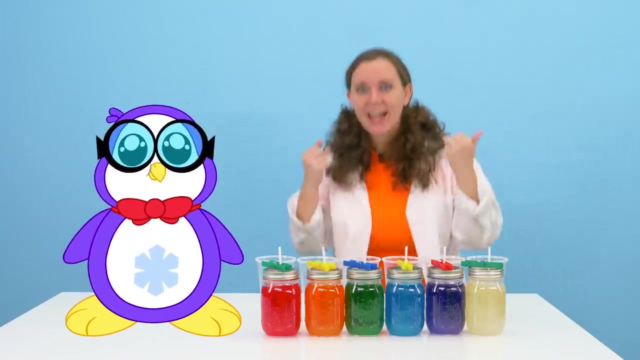 Cool, Cool, Cool, Cool, form rock candy. Speaking of rock candy, I think ours is ready. Let's go, let's go, Hmm candy, Hmm, sure, Peck, Peck, Whoa, has it been 7,200 minutes? It has, which is why I'm here. It's candy time. 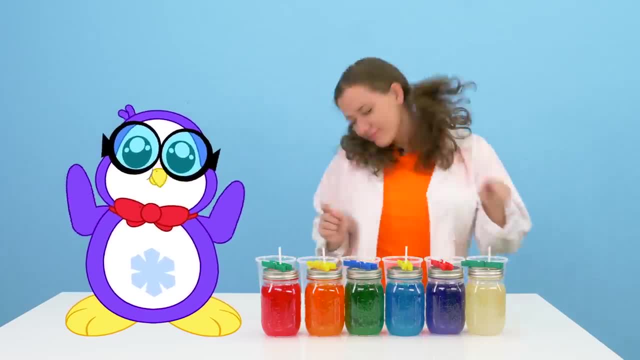 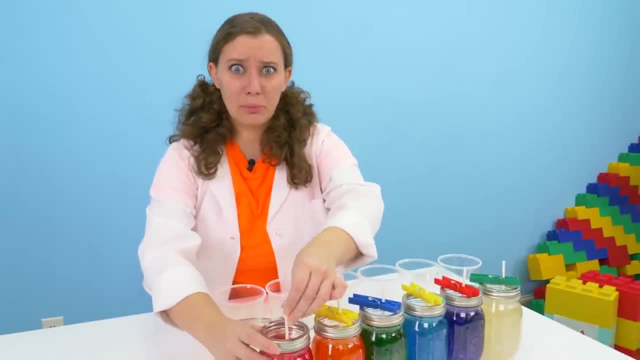 Candy, candy, candy, yeah, But but how are we gonna get the candy out? You're right, Peck these are stuck in. pretty good, but I think we can use this regular plain-jane spoon to maybe chisel it out. 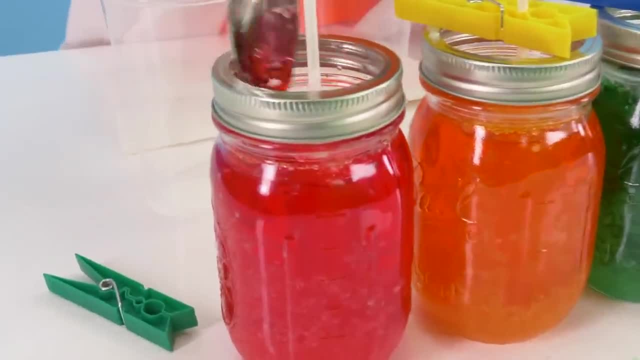 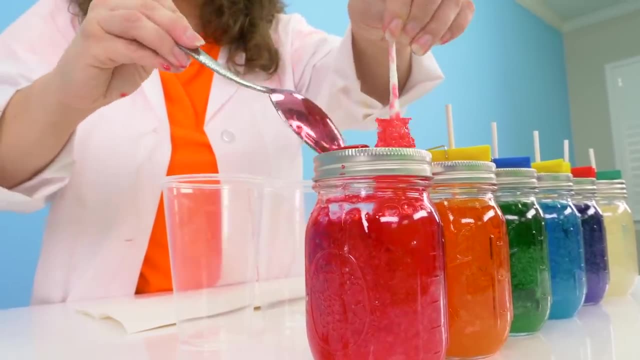 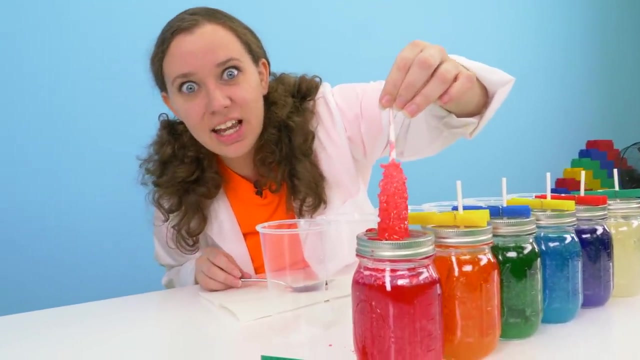 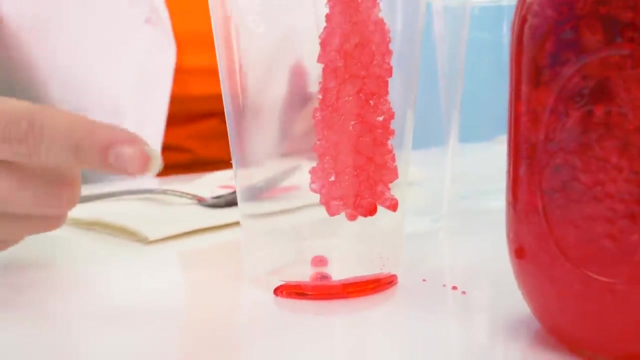 So we need to break the top layer. Oh, oh, my goodness, that is a lot of sugar crystals. Oh, there we go. Oh man, it is all sugary and sticky and yummy. We definitely need this to dry. So we're gonna use this cup to let our rock candy dry so it collects all this really sticky stuff and we don't make a mess everywhere. 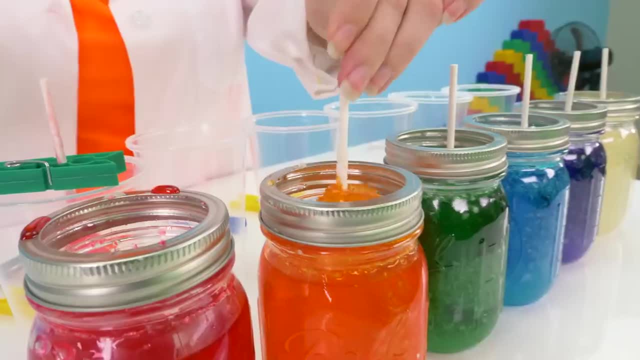 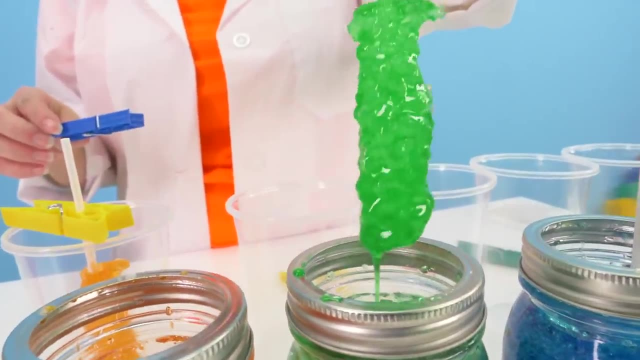 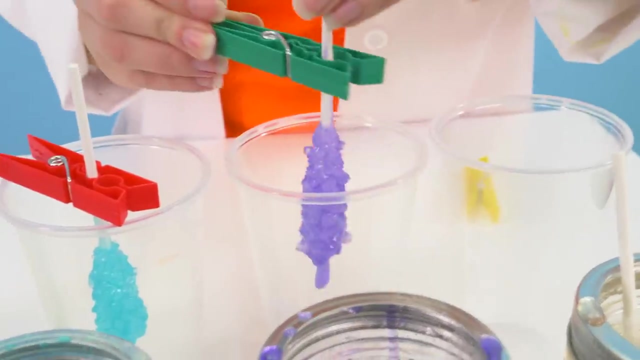 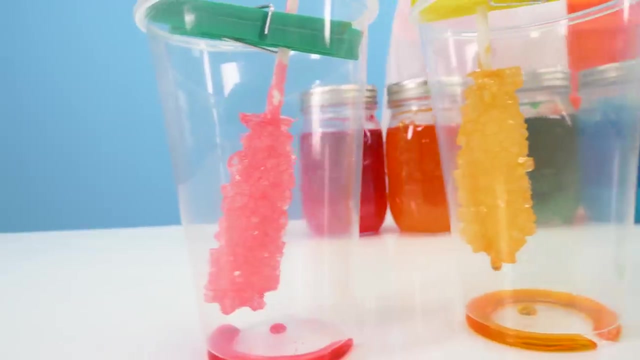 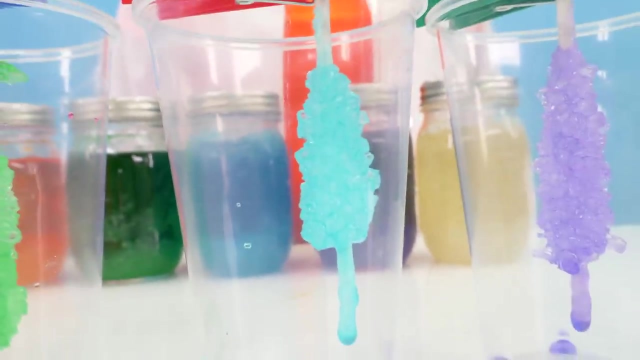 Oh wow, it looks so tasty And crunchy. Phew got it. Oh, oh gosh, I can't wait to try some. Hmmm, hmm, hmm, hmm, Wait a second. That blue one looks broken. What happened? 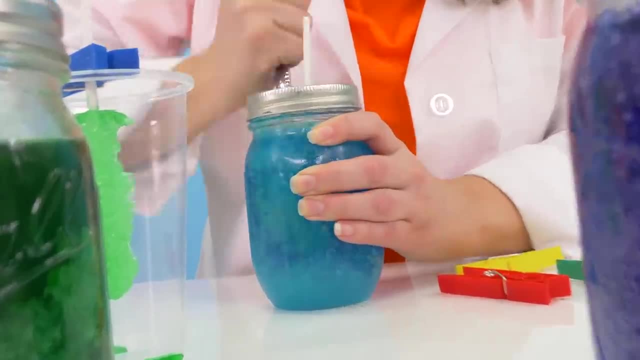 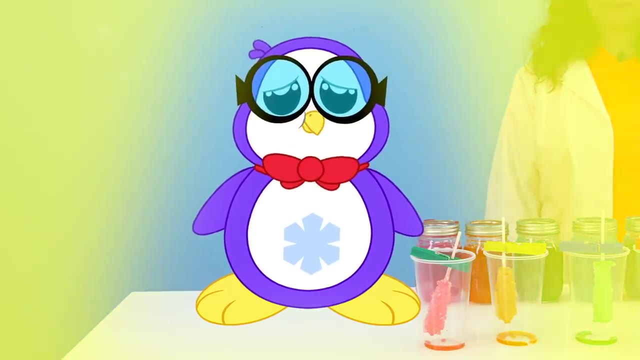 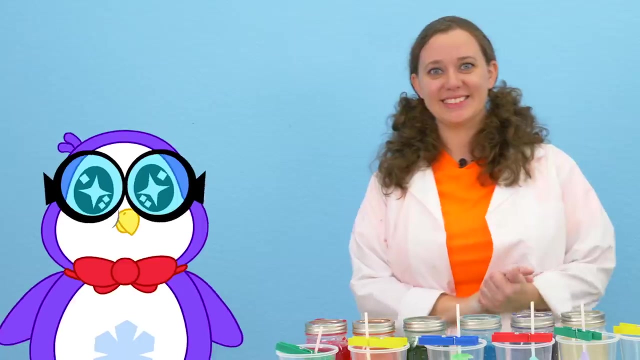 Well, Peck, the stick got stuck in the jar when I went to pull it out and that's because it was a little too close to the bottom and all these crystals grew around it. Um Bri, Is it okay if I try some of the candy now? I've been so patient and helpful. 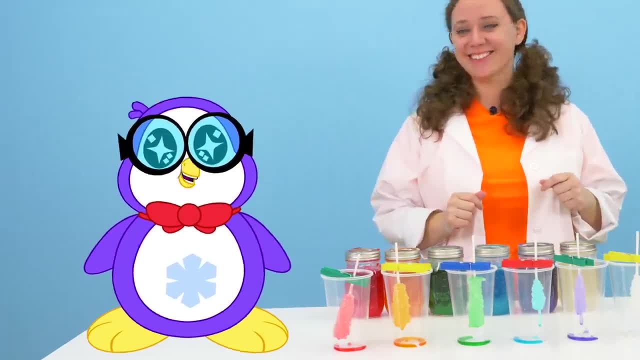 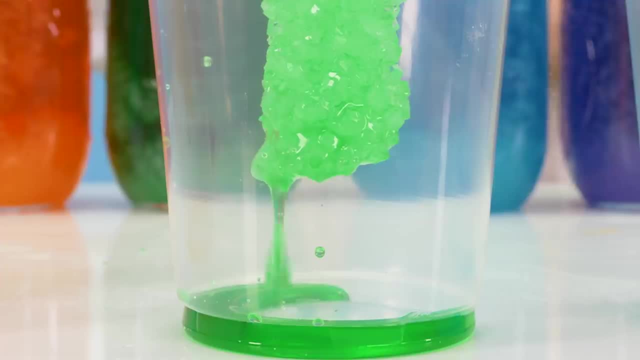 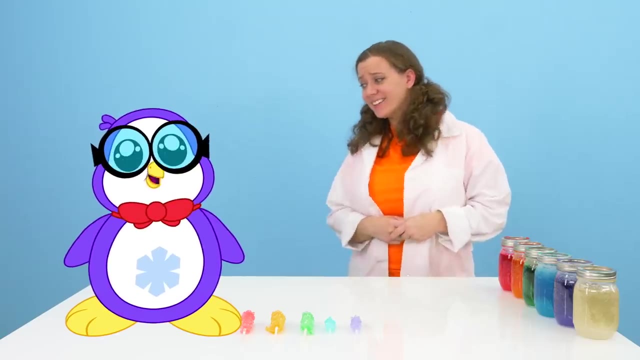 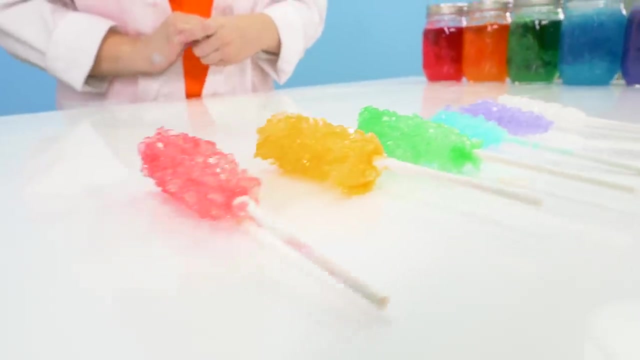 Ha, ha ha. We can definitely eat all of it. eat all of this rock candy really. as soon as it dries. oh gosh, i can't take it anymore. the candy's ready. my patience finally paid off. uh, yeah, sure, good, good job. peck now is the best part we get to taste. test. 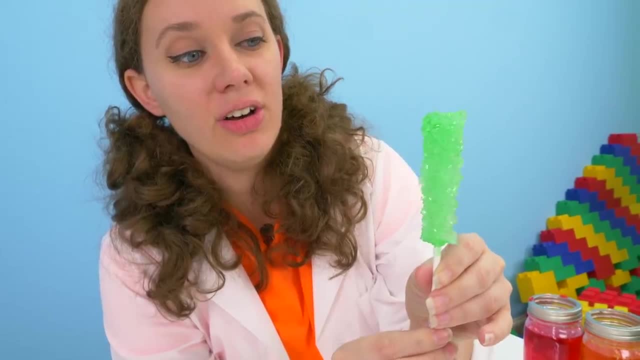 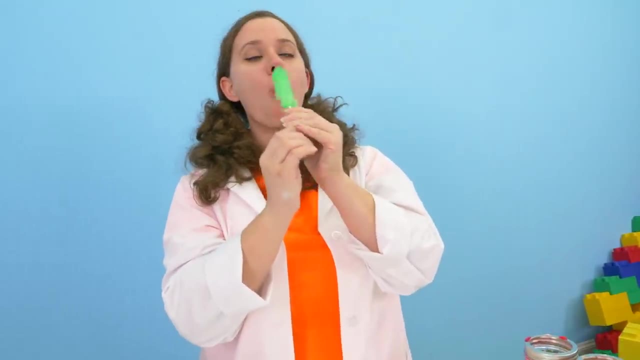 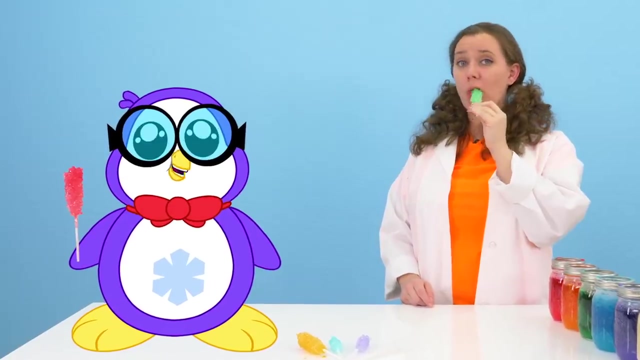 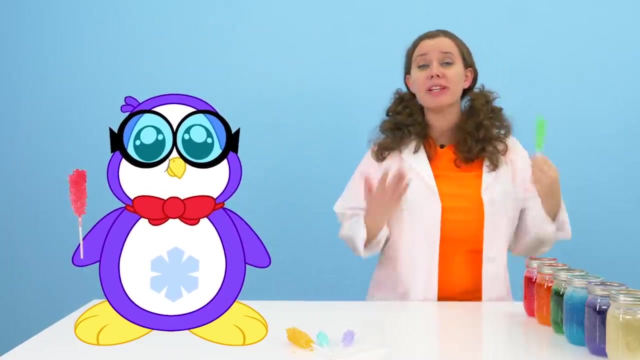 oh shiny. look at all those crystals. they are so yummy and shiny. and the best part, that's really good. this is so good. it's filling me with energy, whoa. and the best part about this is it's so simple to make. you can make it at home too. 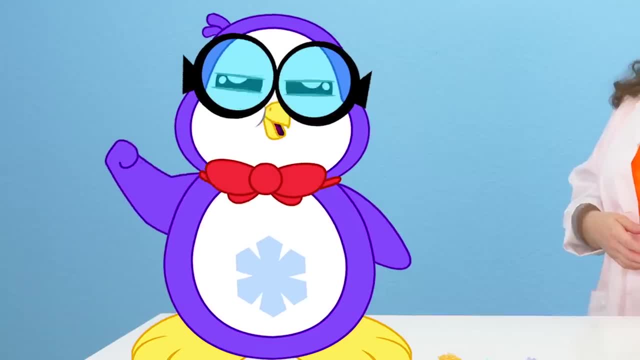 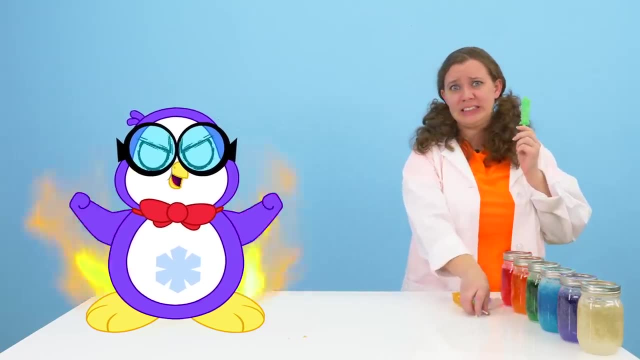 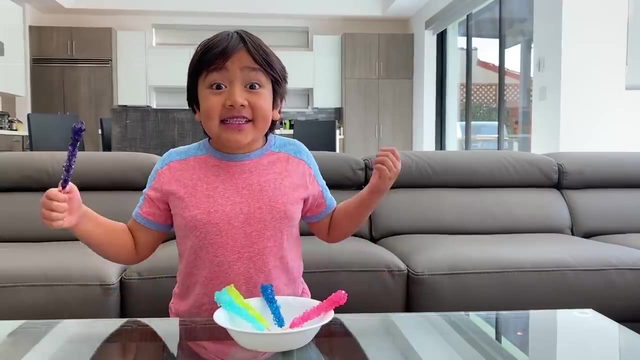 it just takes a little bit. it takes a little while. Yeah, I'm gonna eat the rest of them. Maybe we'll save those for later Peck- okay, Thank you for showing me how to make these rock candies. Peck, It's so cool. Oh, what are those? 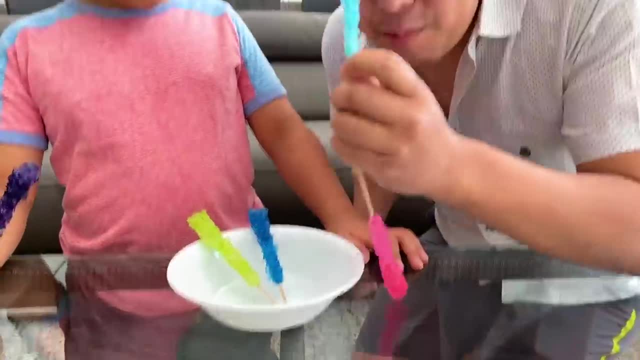 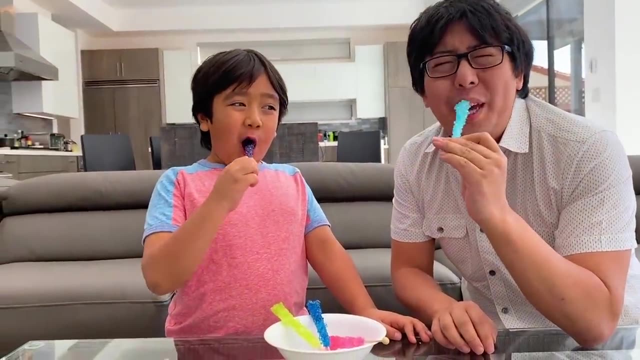 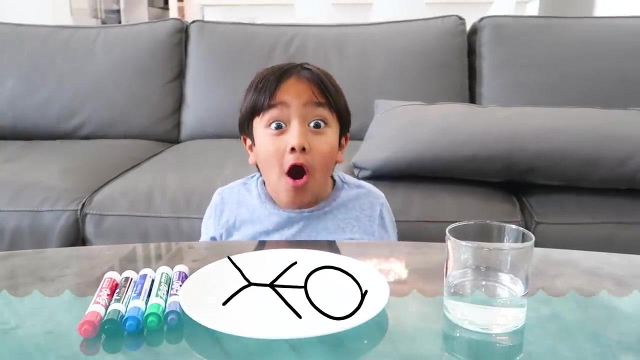 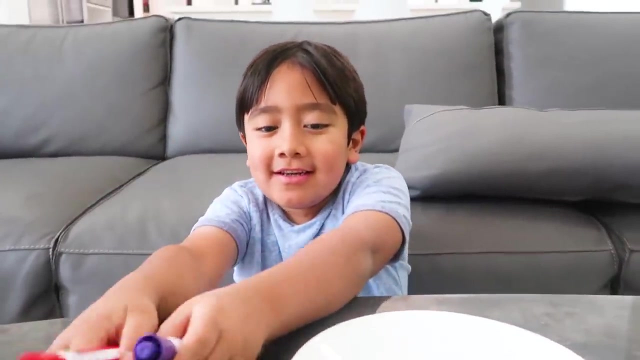 You want to try rock candies? Yeah, I picked the blue one. Oh, this is so cool, And this great horse, So sweet Guys. today we're gonna put our trawling and then make it float on water. So this is very easy. All you need are some markers, a plate and some warm water. 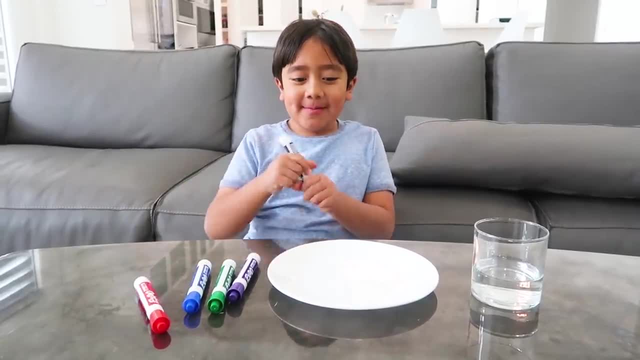 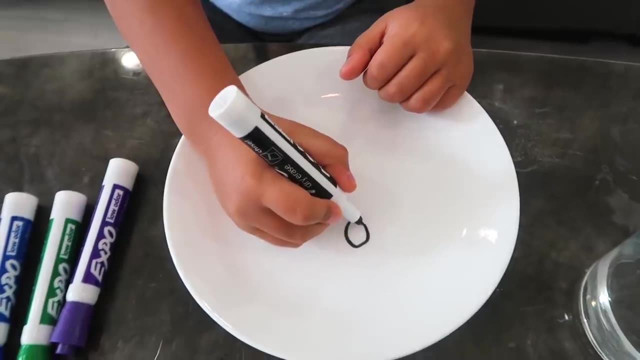 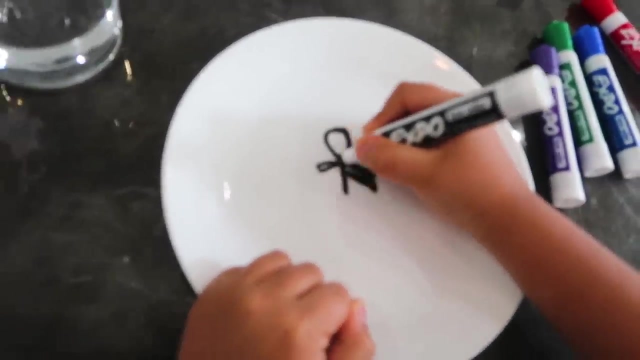 First draw what you want on the plate, What I'm gonna make: stick figures, Stick figures with multiple arms, So like this, and then you make it really thick, Like this, and you make arms, and then you make the legs. 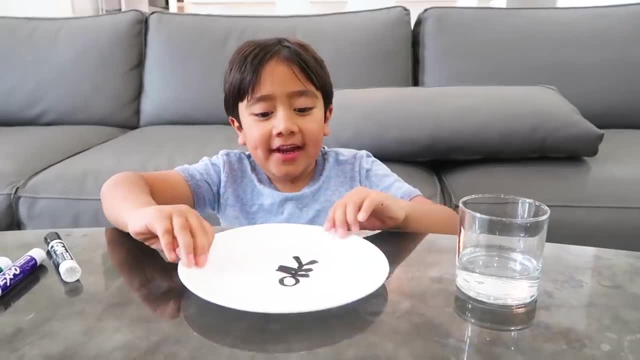 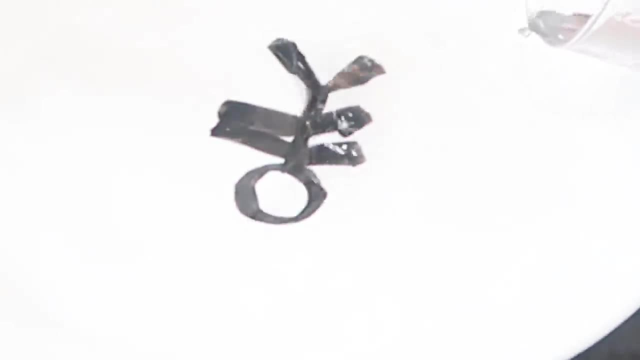 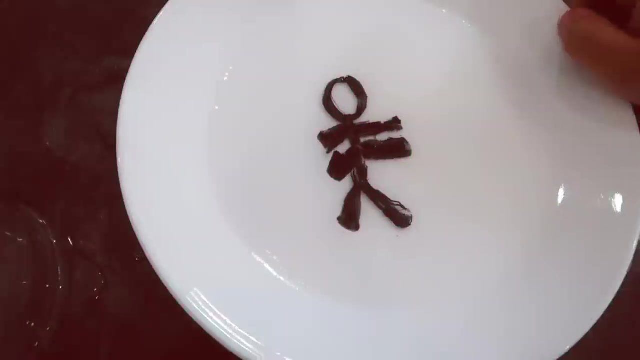 So after you make your trawling, then you put some warm water on this side. Whoa, he moved. Look he's dancing. Oh, his arms too. I feel like the arms or legs are gonna break. Oh, it's moving now. 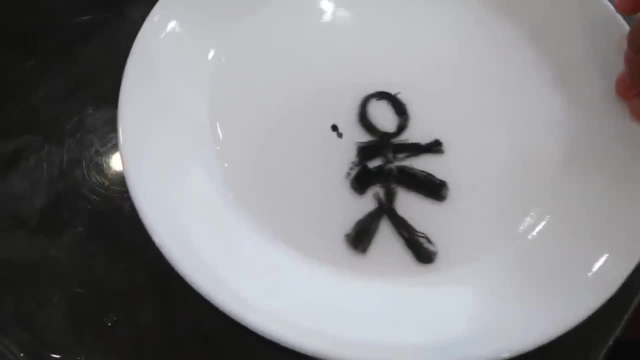 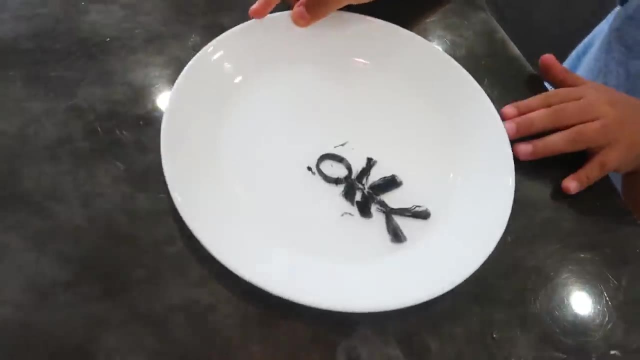 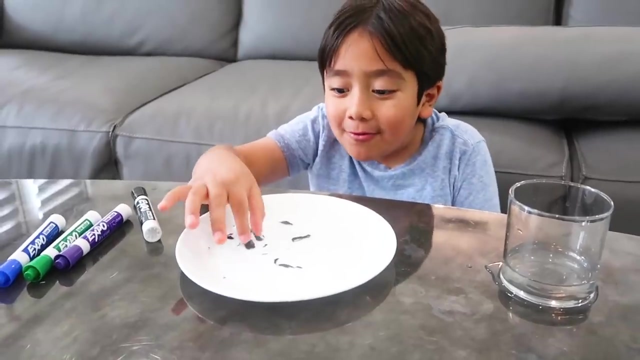 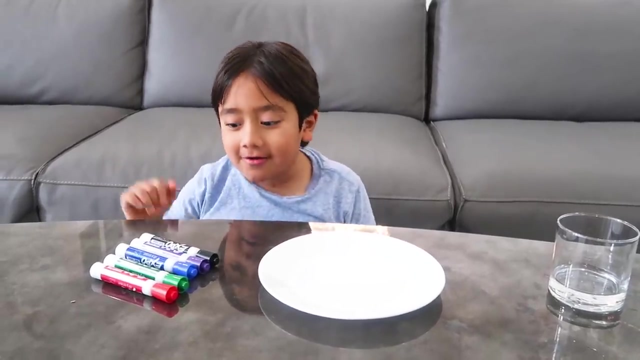 Yay, Now he can just walk. There you go. This is an easy way to make your stick figure float. He broke. This is so cool, You can hold it. Okay, guys, for the next one, I'm gonna make a dog. 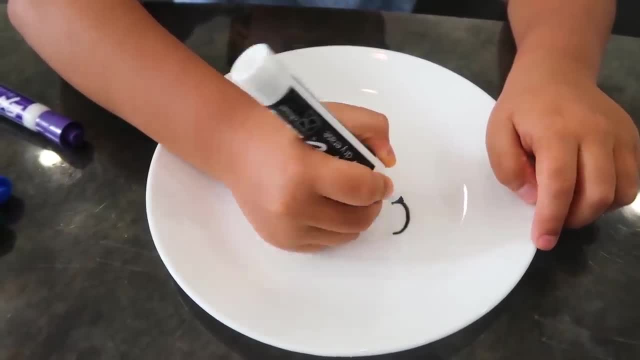 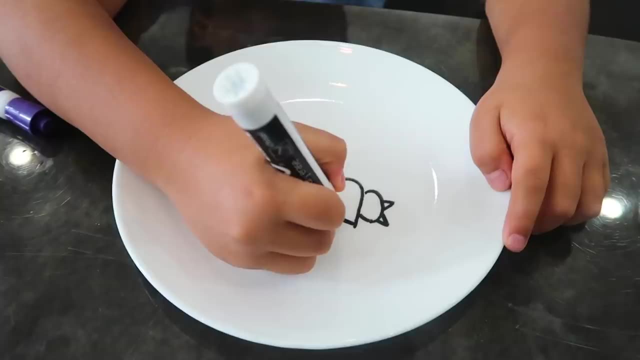 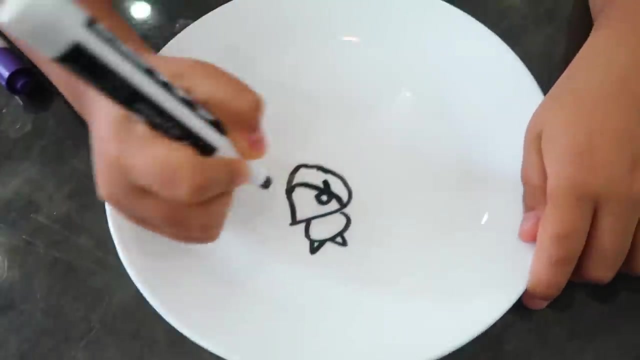 It should be like this, And then maybe I can put like ears. I feel like I'm making a cat. I'm making a big dog or cat. Oh, I can't do it right, Unless I do like this. I put an R. 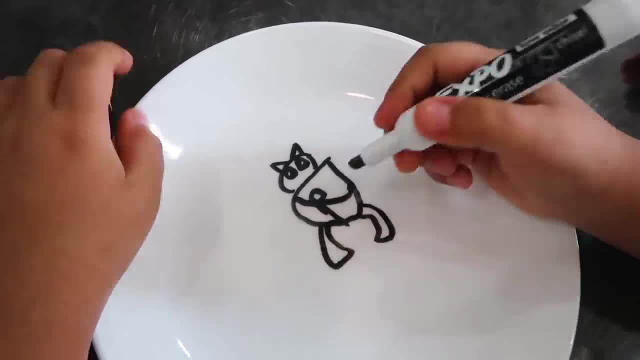 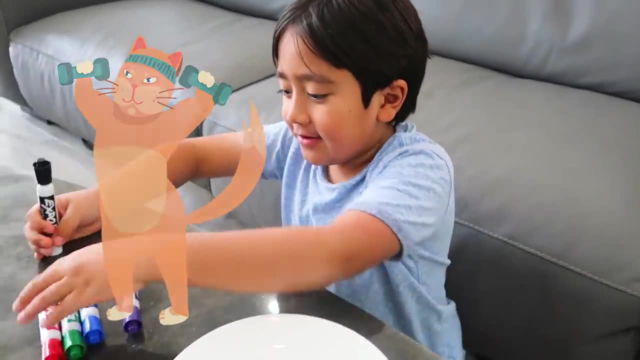 Okay, then I'll make the legs And then the arms, And then the arms, And then the arms. I feel like I'm making like a super strong cat or something. Okay, now I'm going to put this red right here. 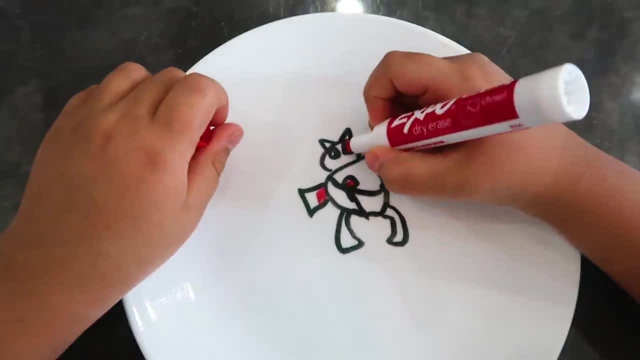 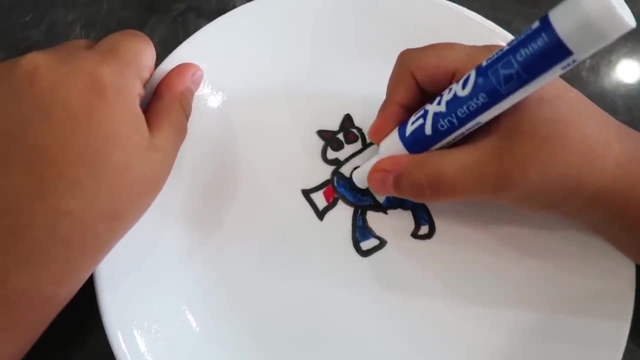 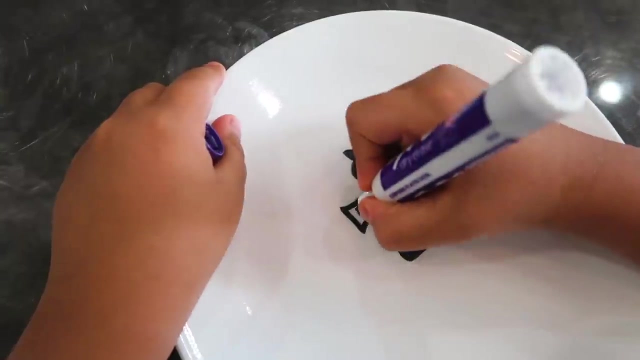 And then I'm gonna make this red, And then I'll make the eyes red On the ears- Okay, so I'm coloring the pants. He has jeans. Okay, I'm gonna make the skin color purple. Okay, I put it here: 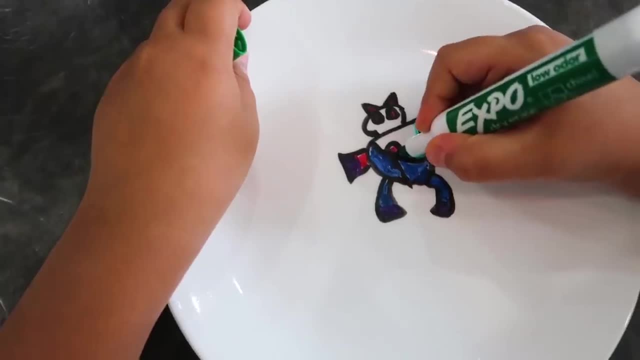 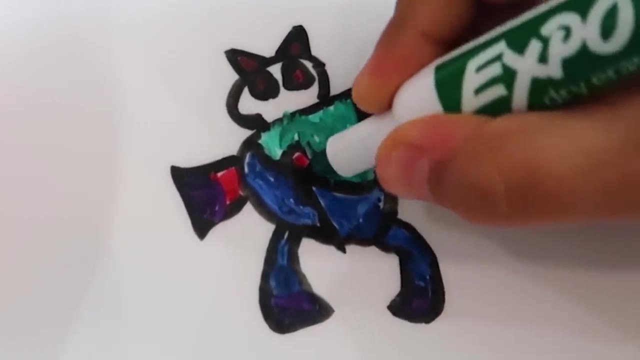 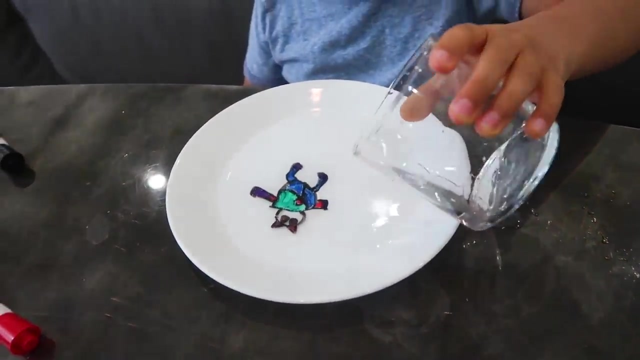 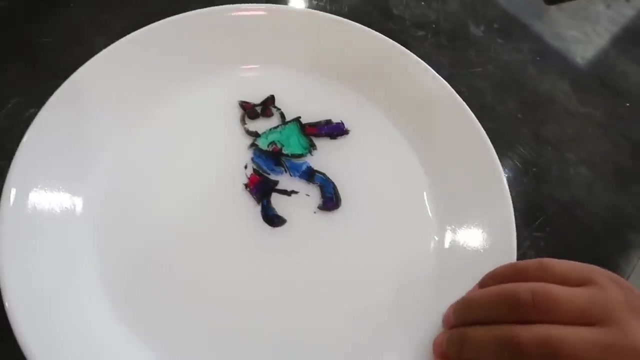 And I'm gonna put this part green. Okay, like this, And Perfect. Okay, guys, let's see if it floats. Okay, I think that's good. Oh, we're missing one leg. Oh, no, the other leg broke off. 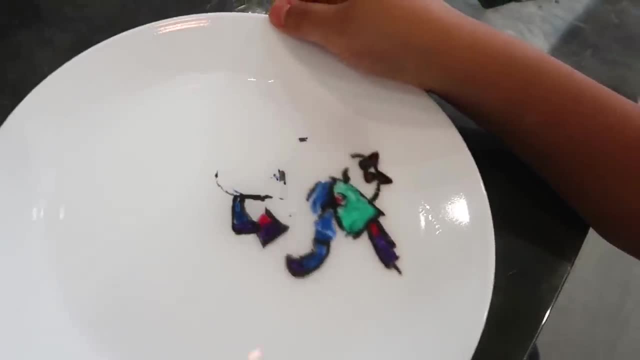 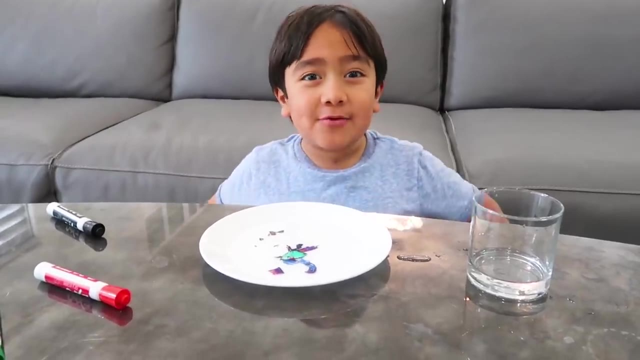 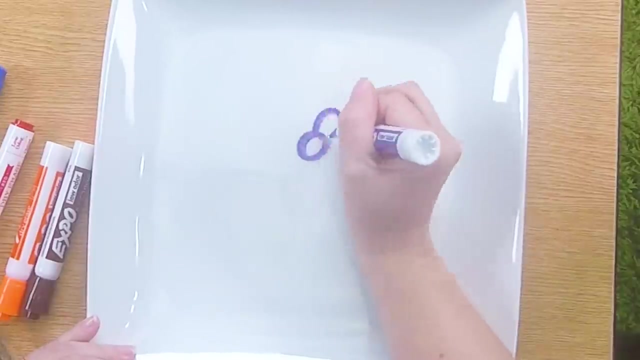 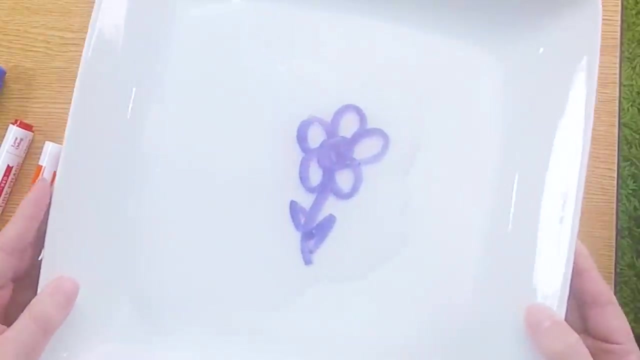 Oh, you're gonna run away though. Ah, his arm. No, no, his face. Oh no, my dog broke. That's okay, Let me show you some cool ones that worked. Roll the clip. Roll the clip. Roll the clip. 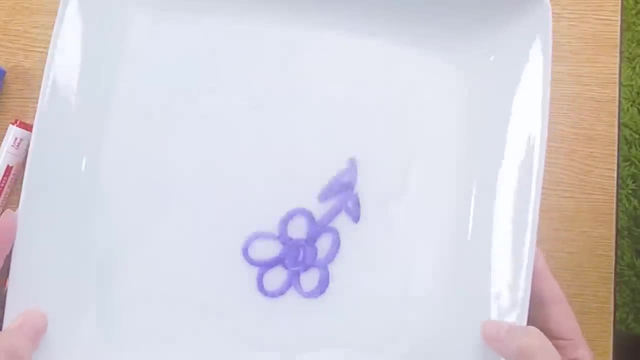 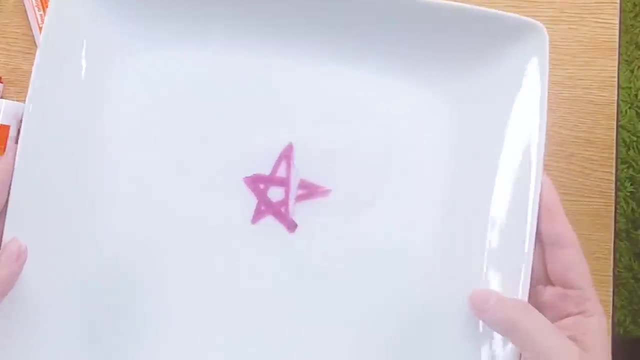 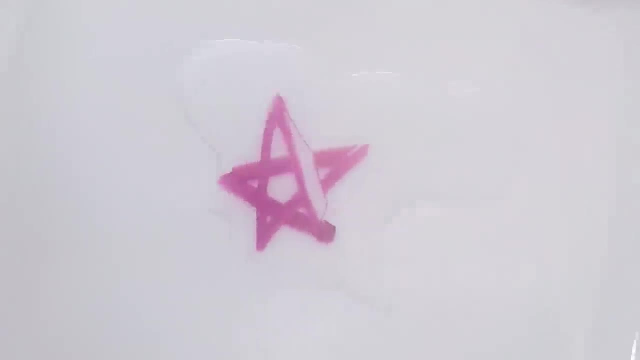 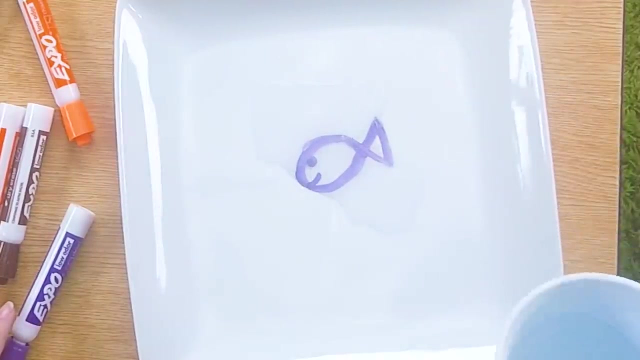 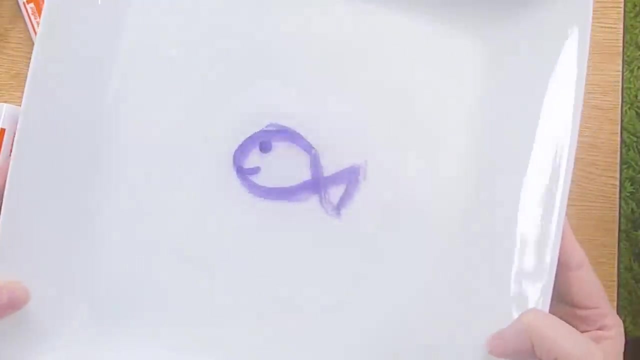 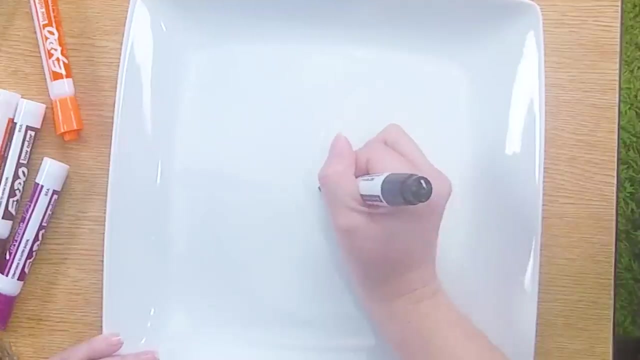 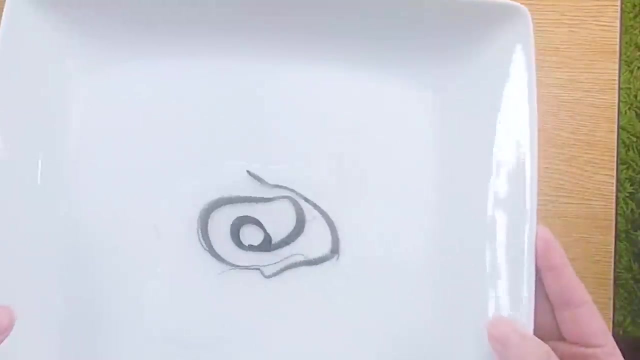 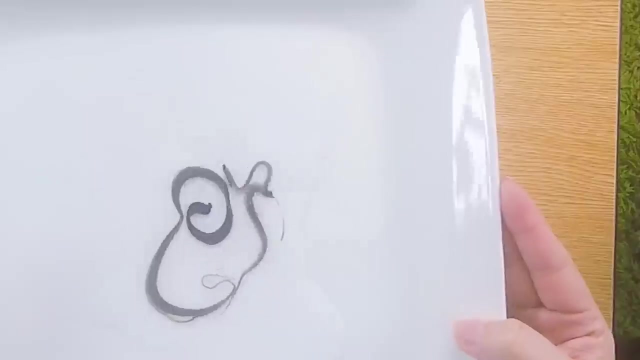 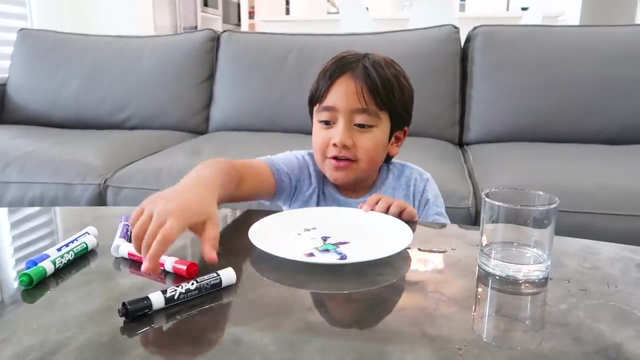 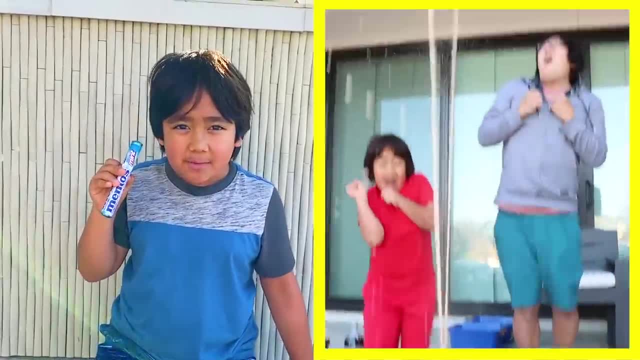 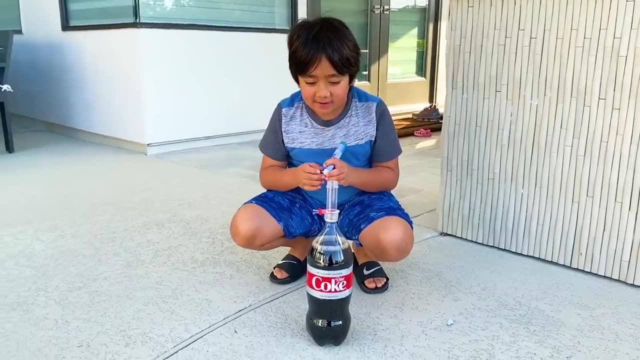 Hey guys, I know you've heard of the Coke and Mentos experiment, But have you heard of the salt and Coke experiment? So first I'm going to show you the Coke and Mentos experiment. All right, guys, Time to have some fun. 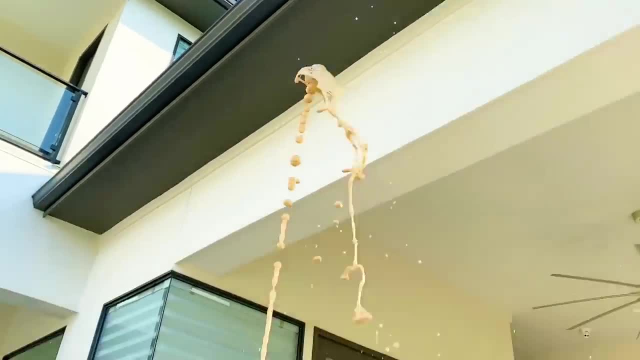 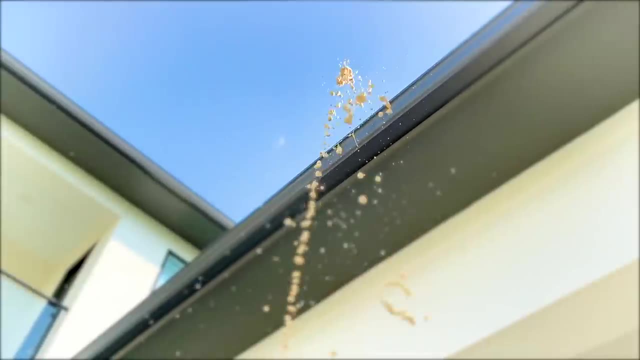 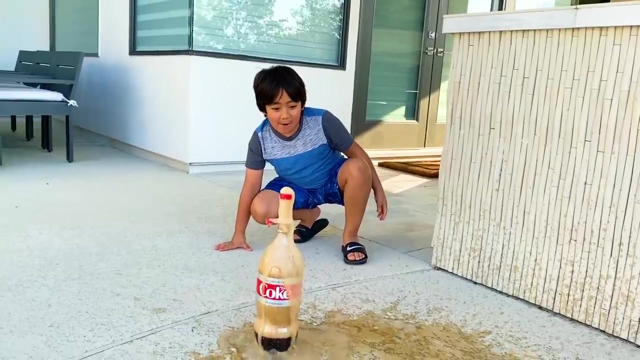 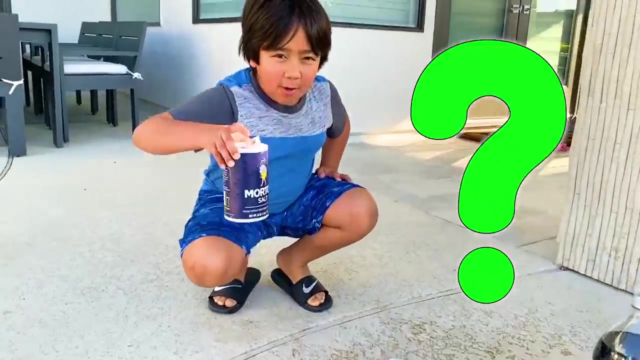 Whoa, Whoa, Woo-hoo, fix. whoa, That was a big splash. Wow, that was cool. So we know mentors works, but will salt work? Let's find out. Okay, guys, let's see what happens. 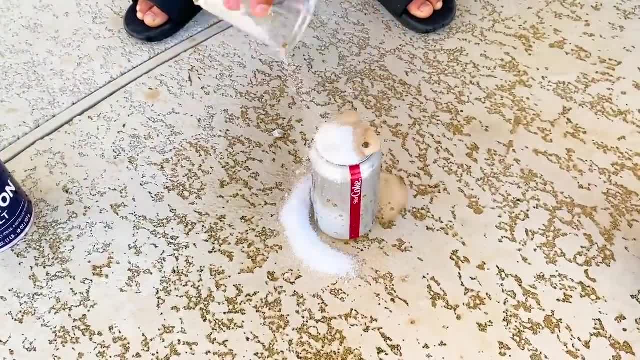 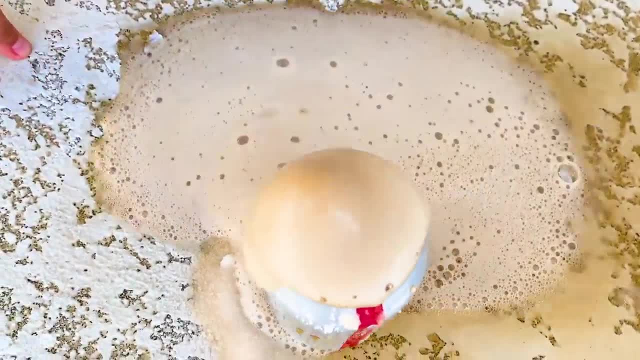 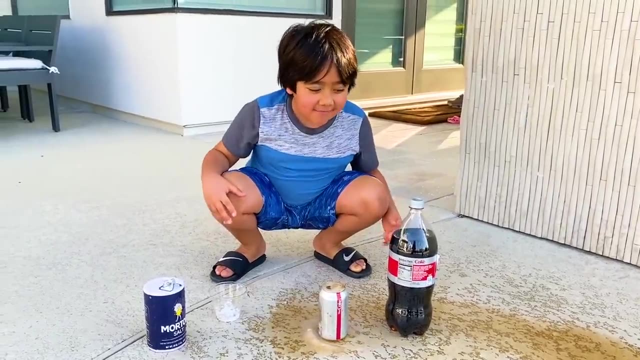 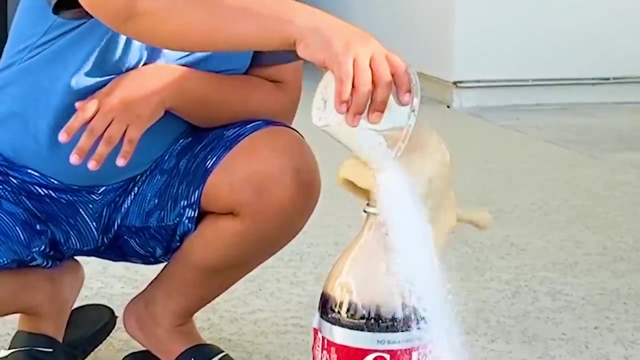 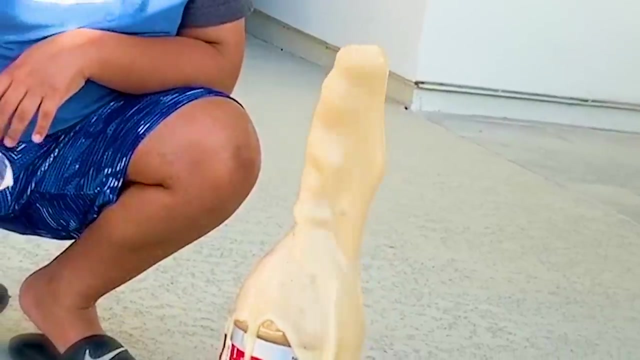 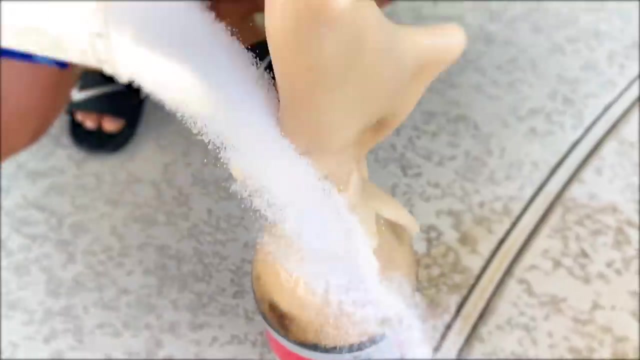 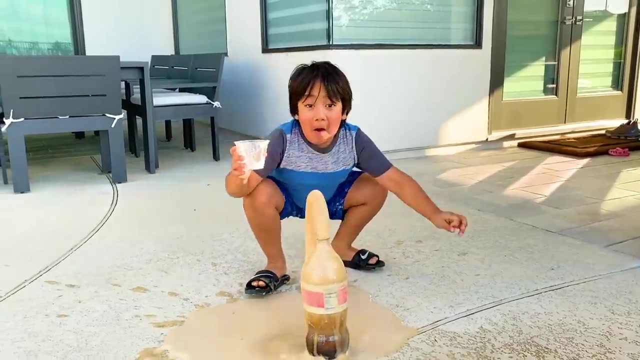 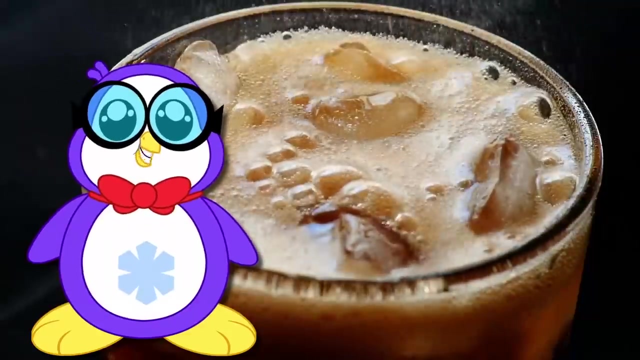 I can see. You got it, We did it. Now push, whoa, it's exploding. whoa, whoa. okay, so it does kind of work. now let's try the bigger bottle. okay, guys, time to try it out. oh so it does work. but why does it work? hey, ryan, the reason why is so? there is carbon dioxide gas. 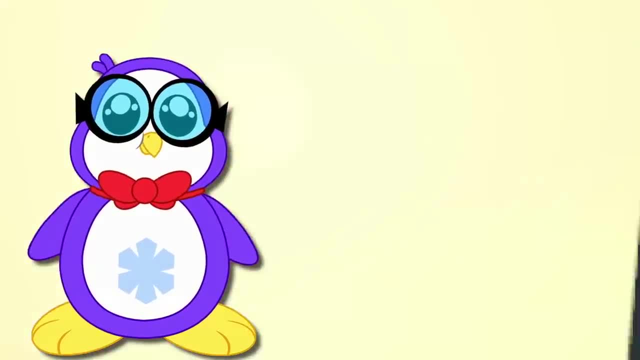 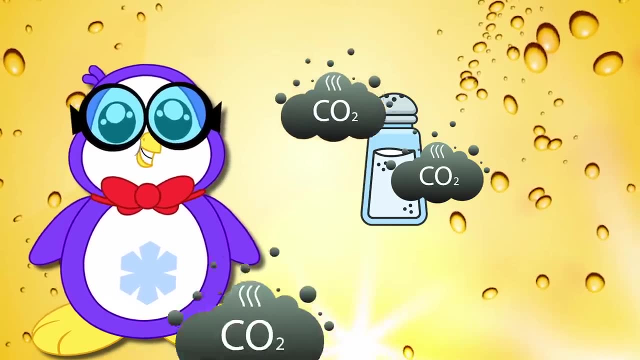 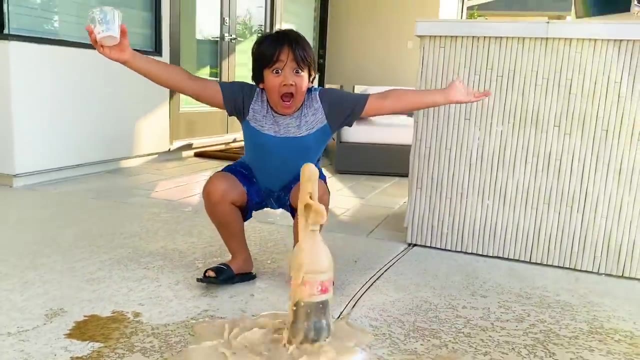 in the soda and salt is added to the soda, the carbon dioxide gas latches itself to the tiny pumps on the salt. as more carbon dioxide gas accumulates around the crystals, the gas becomes more buoyant, so it rushes out and escapes, causing an explosion. wow, that was so cool. i didn't know salt and coke. 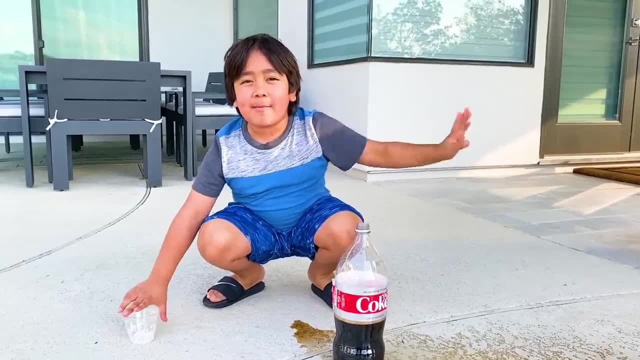 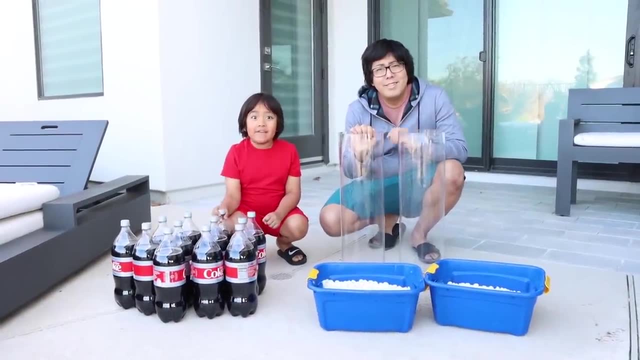 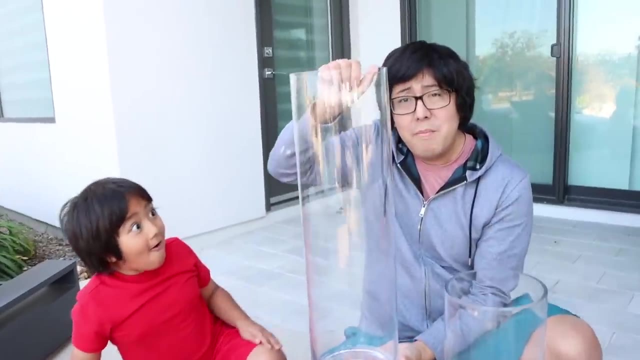 would work. bye, thank you for watching. remember always stay happy and rise up. bye, hi guys. today we're going to do the diet coke and mentos giant experiment. yeah, we got this giant container so we can putmentos in one side and on the other container we can put diet coke. 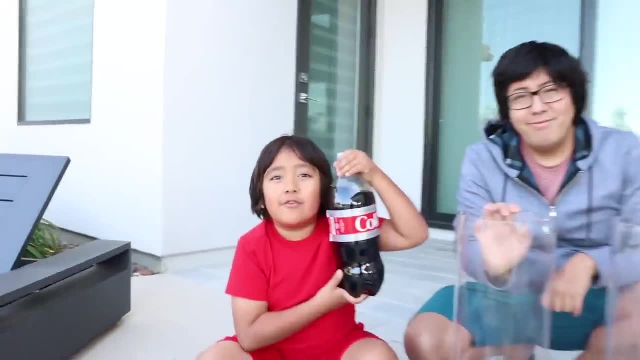 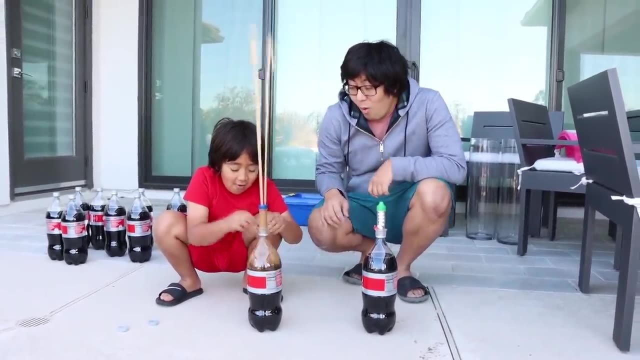 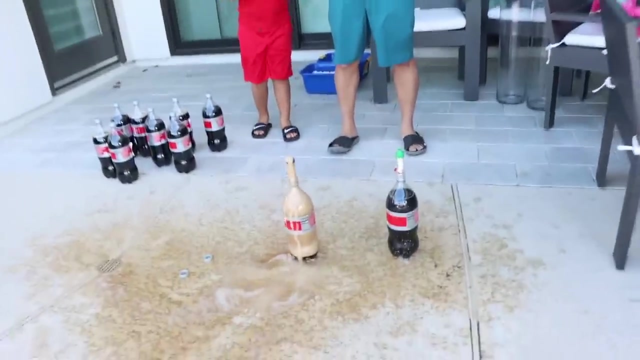 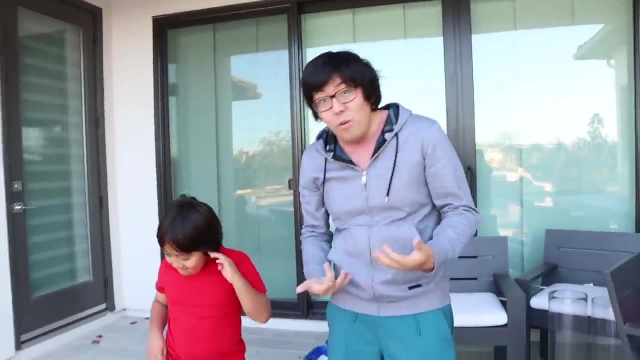 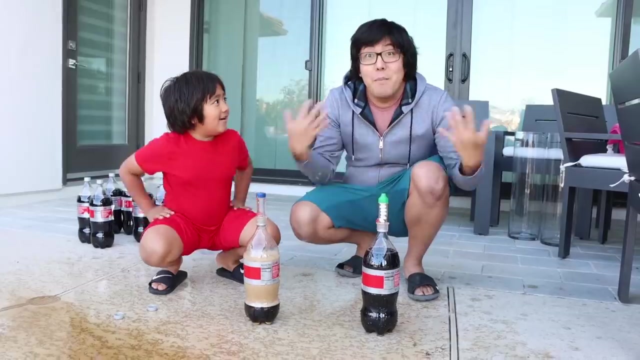 first. we're gonna do the regular way and see what happens. i'm gonna do mine's first all the time. whoa, that's so cool. i've never seen that before. Oh, it's so hot. Can mine go higher than Ryan's Maybe? Let's see You ready. 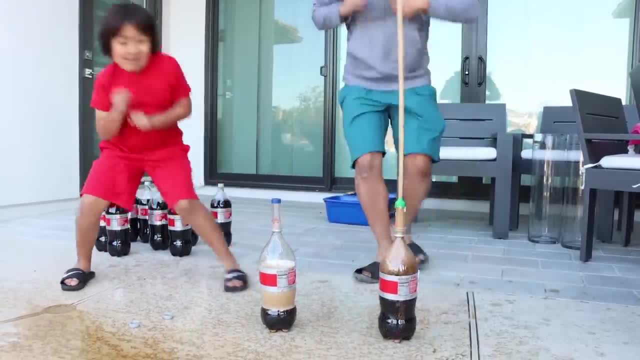 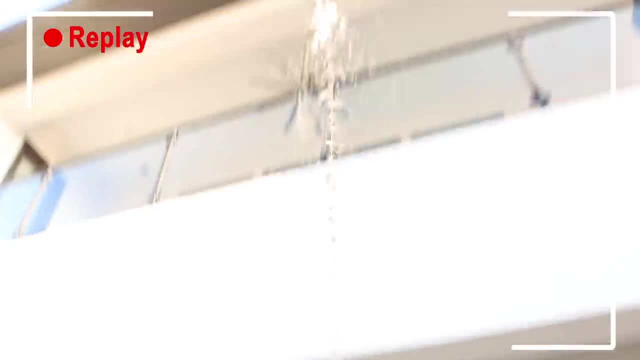 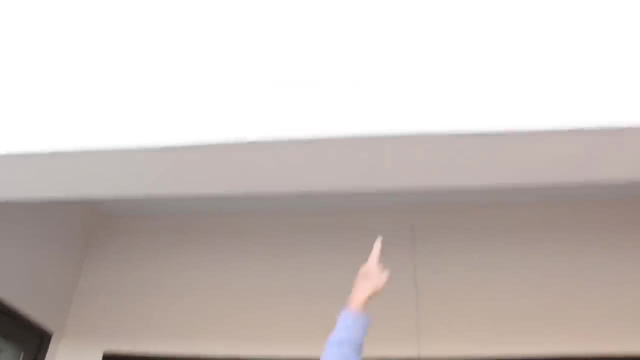 Quickly back out. okay, Ryan, You ready? Wow, Oh, It's so hot. Wow, That looks like a fountain. That's so cool. Oh, he's got something like cocoa on the wall. Okay, guys, now we're going to fill up. 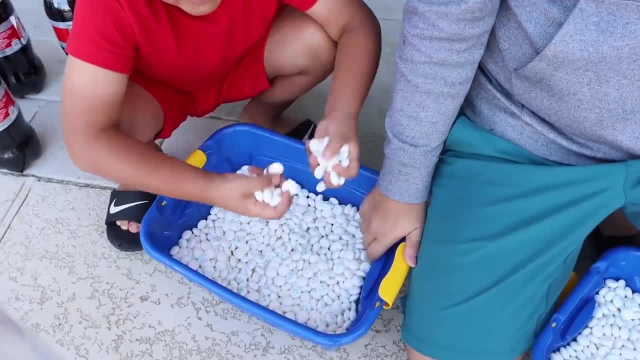 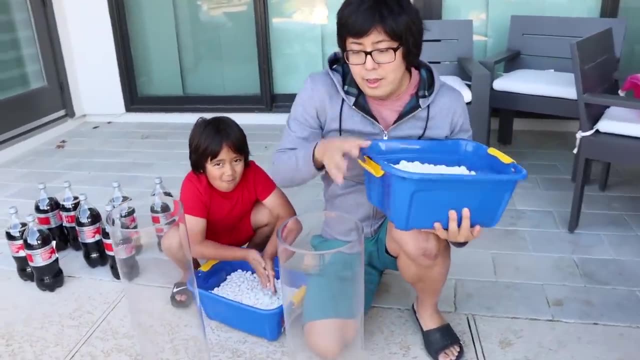 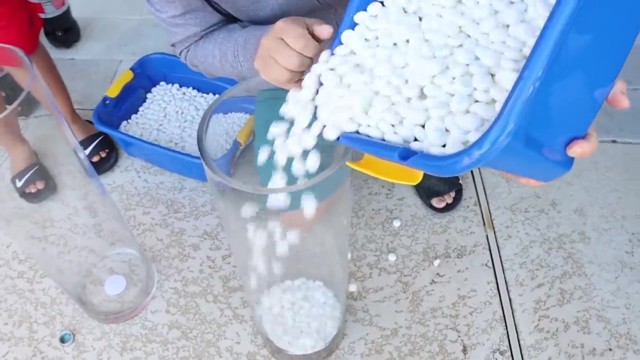 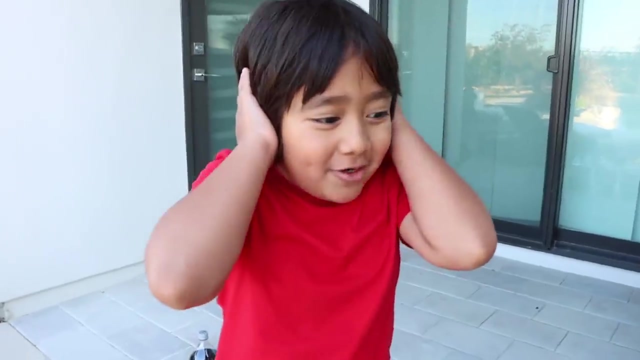 the giant containers with Mentos. First we're going to fill that with Mentos and this one we're going to put Diet Coke after that. You want to look carefully for the name, because, Daddy, that's not carefully. Okay, second one coming. 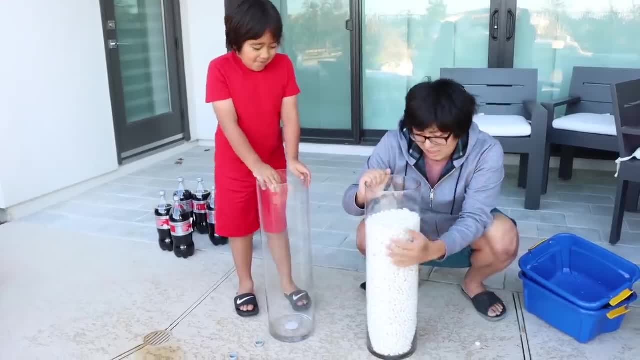 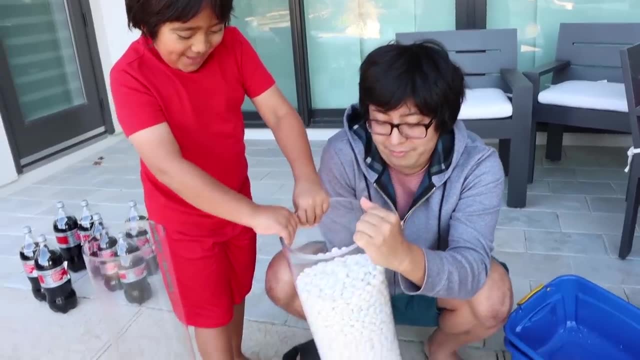 That's way too much. Nice, Alright, it's all in. Let's see how heavy it is. Can I even lift it up? Oh yeah, barely It's heavy. Let me put it down. I want to try. It's heavy, right, I can't lift it at all. 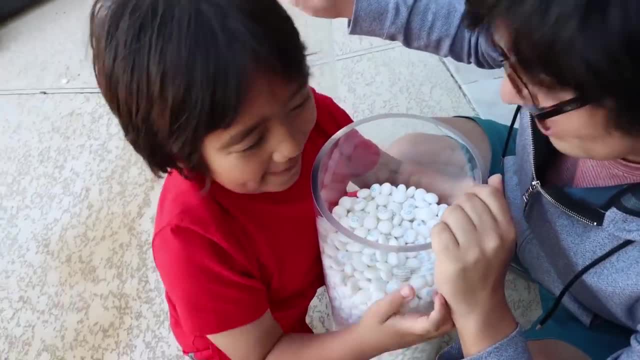 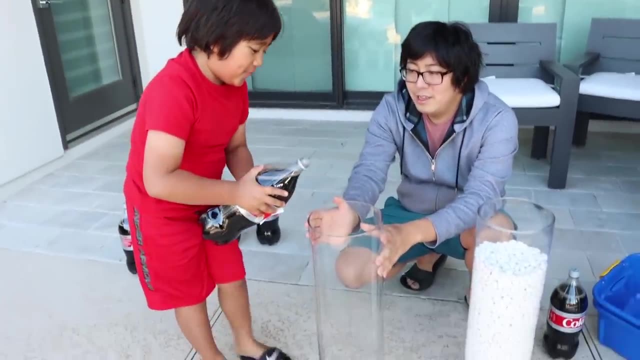 Okay, I'm going to do this. I can lift one of these, but I can't lift thousands of them. Okay, we're filling the other one up with Diet Coke. Let's see how much it fills up with just one bottle. 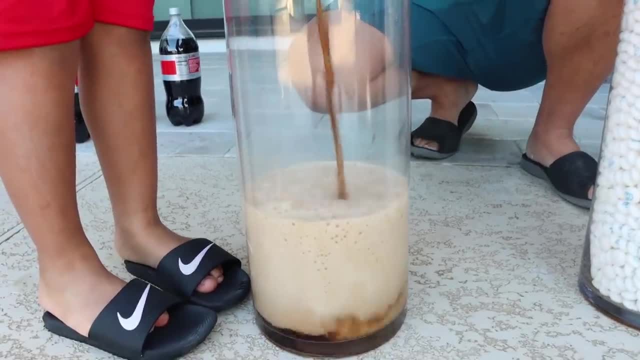 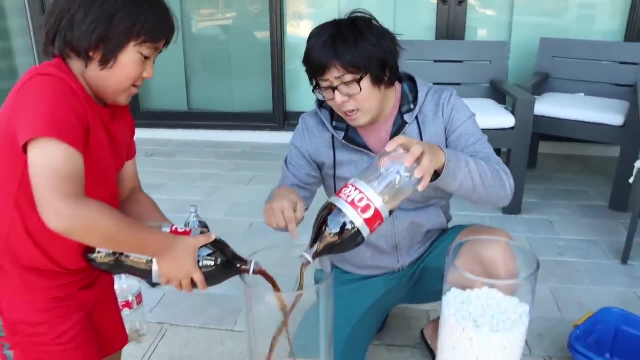 It's going to fill up a lot. We actually might only need two bottles. Why don't you guys take a guess? How many Diet Coke bottles do we need to fill this up? So far we've been using This is the third one, right, Yeah? 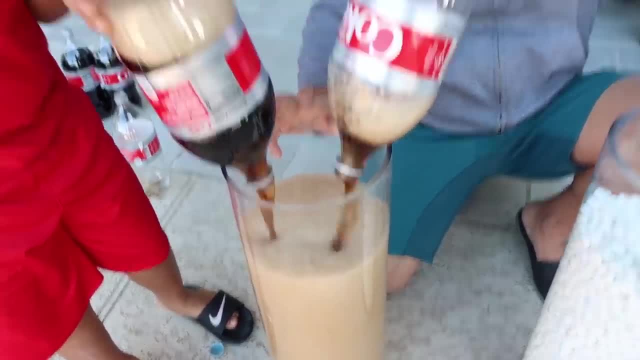 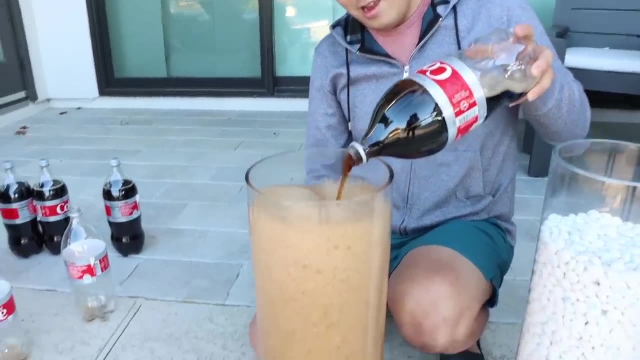 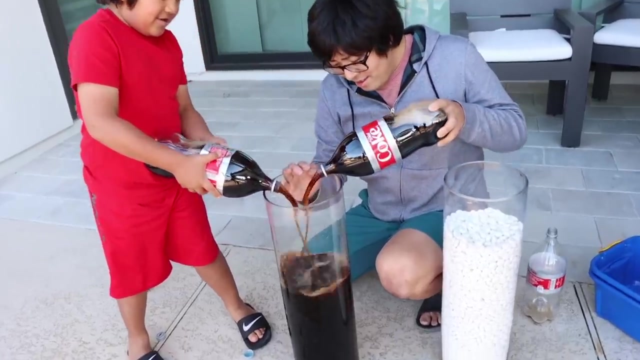 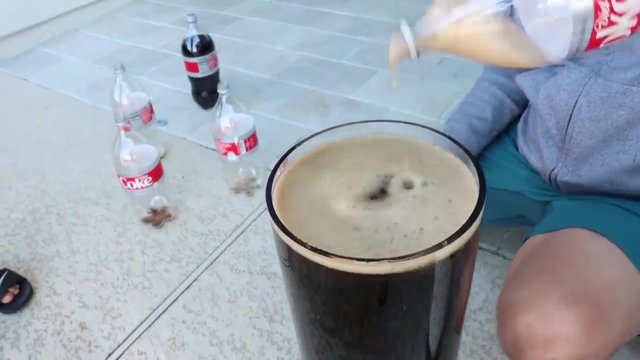 My guess is five bottles, Oh Never. We're almost there. Here comes more. This is our sixth one. We're only halfway Splashing. Oh, we did it. Okay, now we fill up too much. How is the Mentos going to go in there? 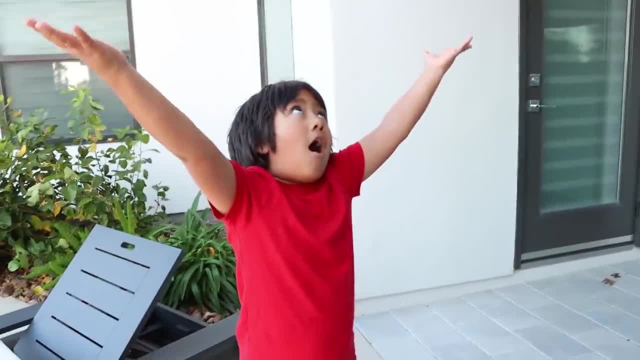 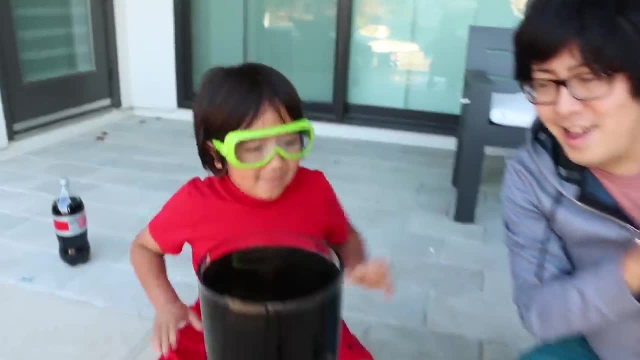 I didn't think about that. There's no space for Mentos. Wow, Okay, guys, it's time to start, But safety first. Alright, you ready? Yes, Okay, I need you to hold it steady, okay, Ryan. 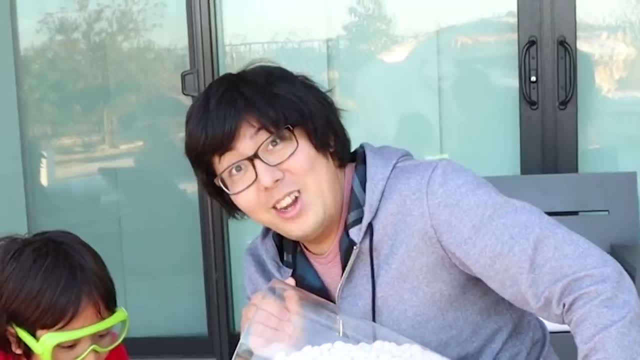 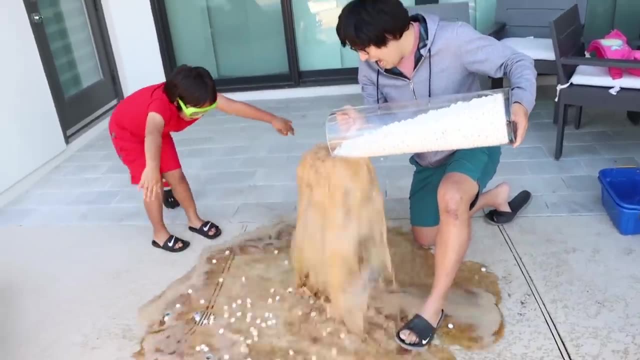 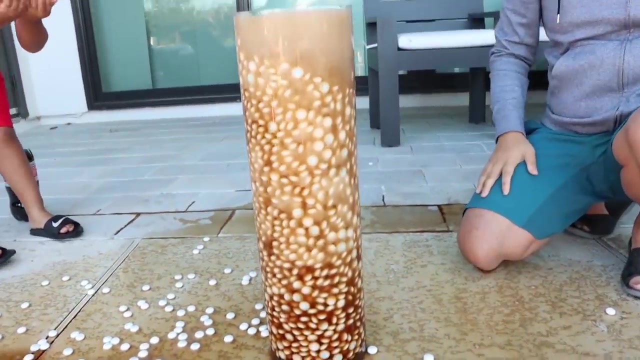 I don't want that to go over Super hard. Ready Three, two, one go. Oh, Oh, Oh, Whoa. Oh, It did not work, guys. Look it didn't splash. What are you doing, Ryan? 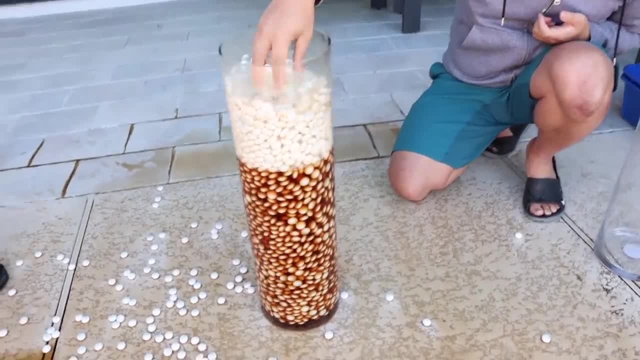 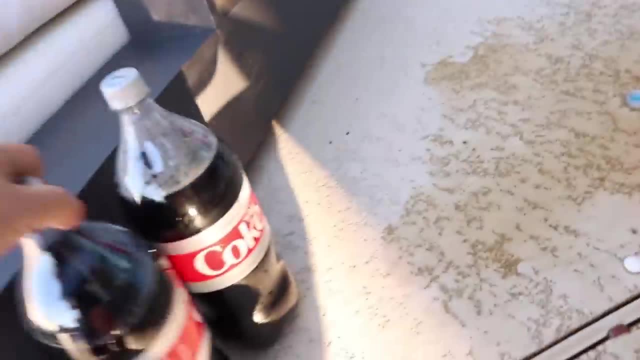 I like fumble you puppy. What's going to happen? Do we have to wait? No, I guess you didn't make a bubble. Yep, it did not work, But good thing is we have more dice Guys. I wanted to try this one. 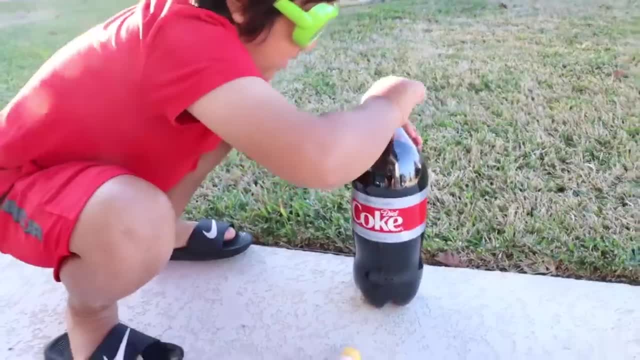 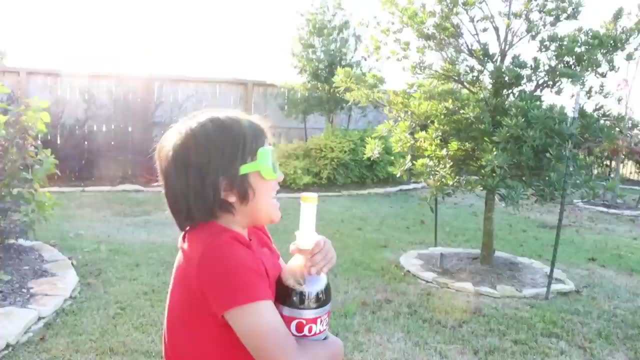 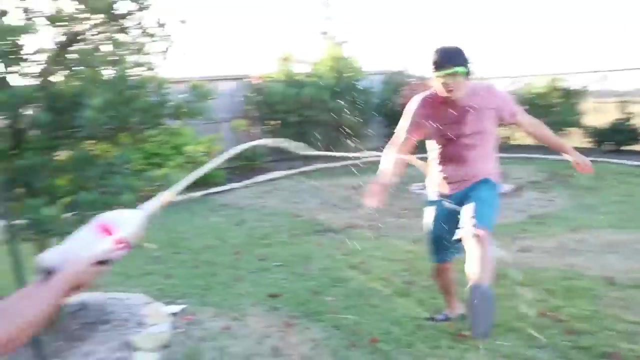 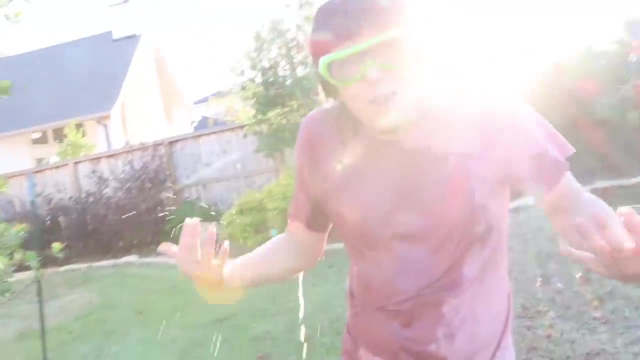 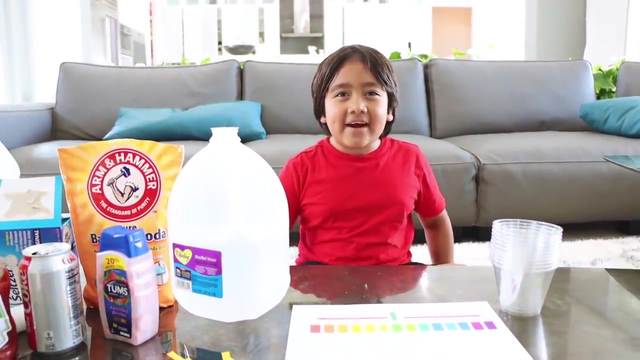 but I have an idea, Daddy Shh, Hey Daddy, Hey Ryan, Whoa, That one's soaking wet. I guess you could use that as a water blaster. Hi guys, Today we're going to be testing out items that are. 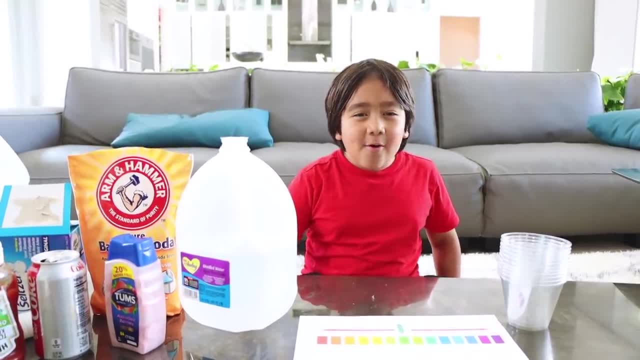 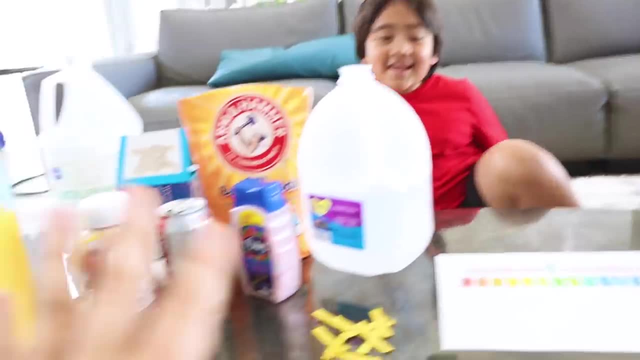 liquid in our house to see if it's acidic or if it's basic. Yeah, so we gather around ten things around the house and we're going to test to see which one of these items are acidic and which of these items are basic. Well, how do you tell? 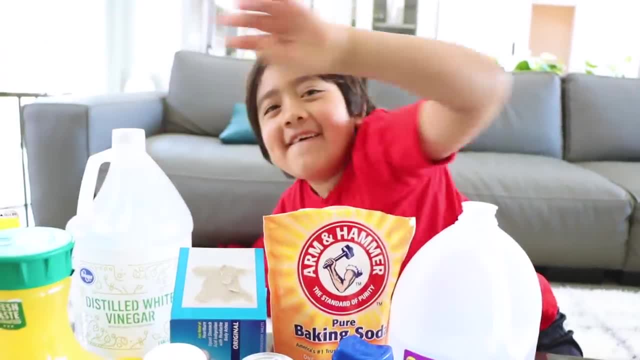 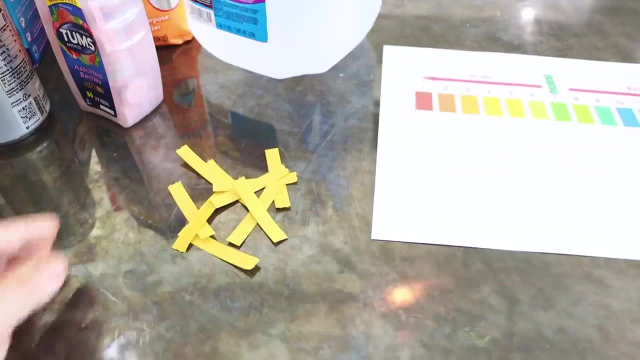 Uh, isn't this acidic? I guess we'll find out, Ryan. How do you tell you ask Acidic? You didn't ask, but how do you tell We got these strips called Universal Indicators, So it's going to indicate to us. 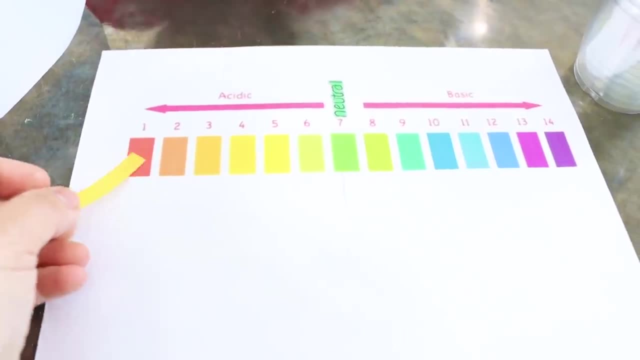 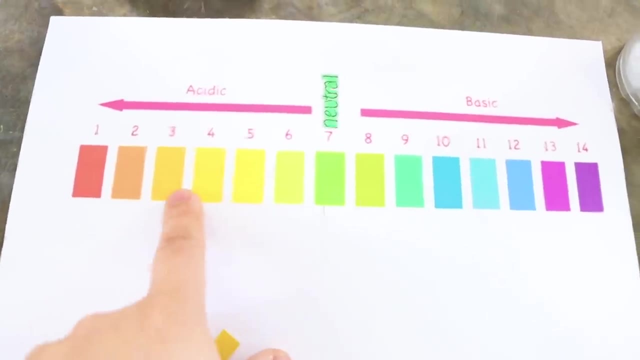 if it's acidic or basic, We're going to dip it in different liquids and it will change colors. See So, anywhere within these colors, one through six is acidic, and if it goes from eight to fourteen, if it's any of these colors, is basic. 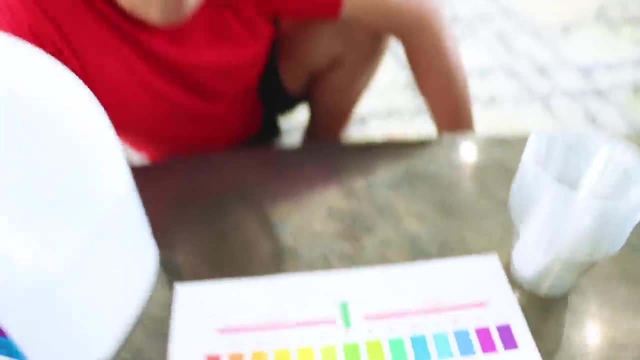 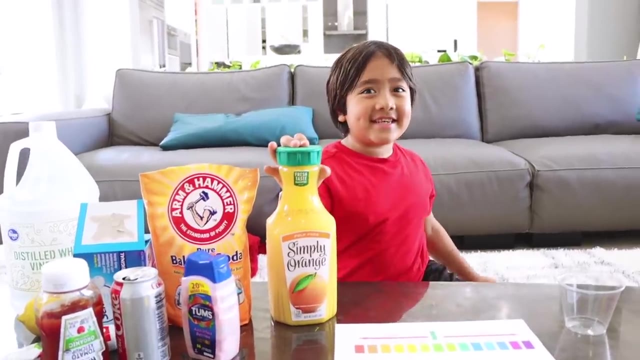 And then if it's green, it is seven, which is neutral. Okay, Ready to test them? Yeah, I'm going to test orange juice first to see. if I'm right, I think it's acidic, Acidic. Okay, I'm going to take some of orange juice. 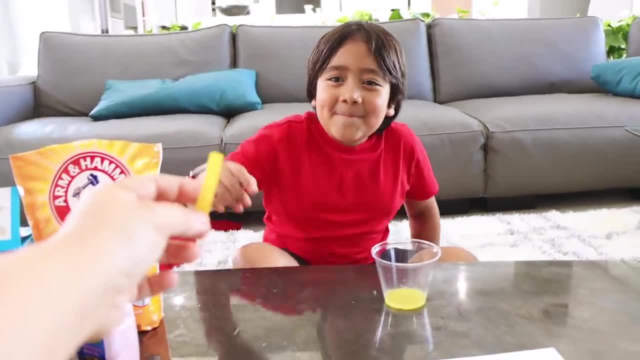 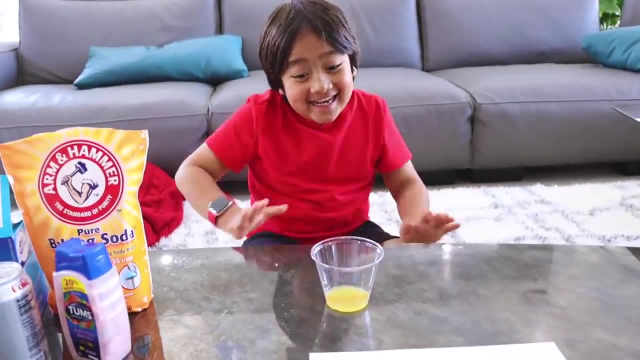 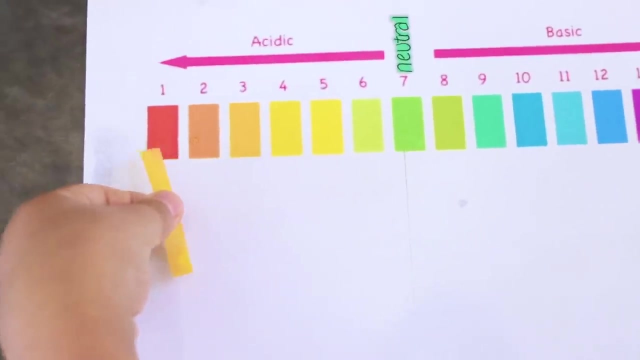 You need a tiny bit. Here is your Universal Indicator. Dip it in Now we're going to take it out, Ryan. I did say dip it. I wonder which one it is. Which one is orange juice, Ryan? Which color is it? Oh, it's three. 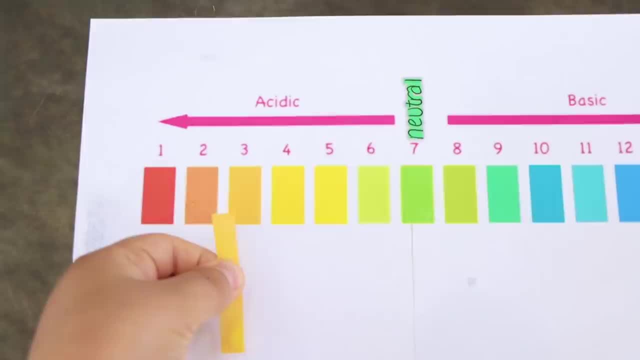 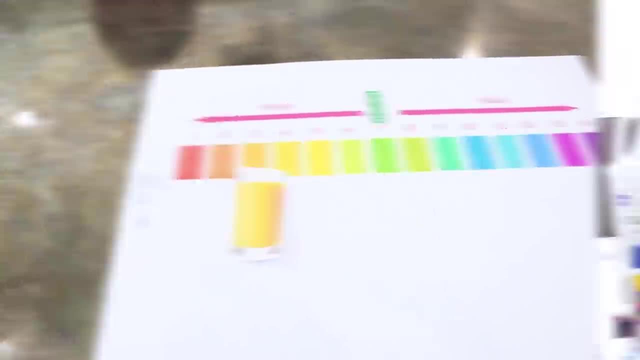 Three. Okay, so three is on the acidic, or basic Acidic Acidic, right here, Good job. So orange juice is right here. Yeah, so about number three, Good. Next, I'm going to test this baking soda, Alright, 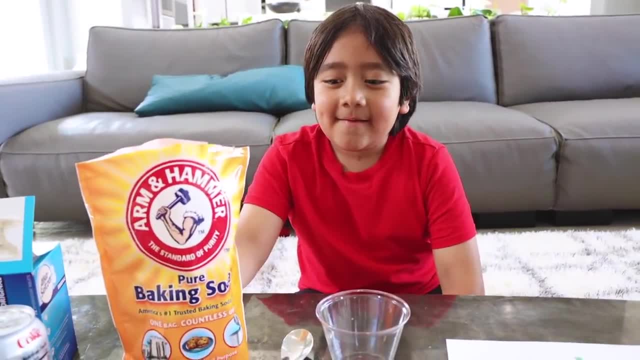 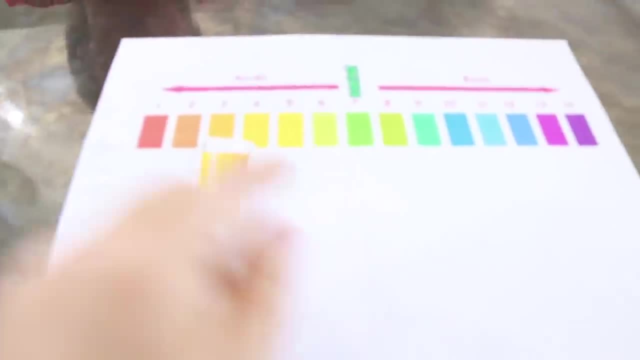 before you test. can you give me a guess: Acidic or basic? I feel like it's neutral. It's neutral. So Ryan thinks it's going to become this color here for neutral. Alright, let's see. if Ryan is right, What do you guys think? 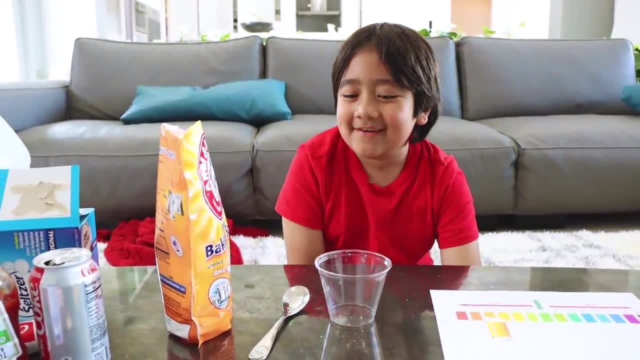 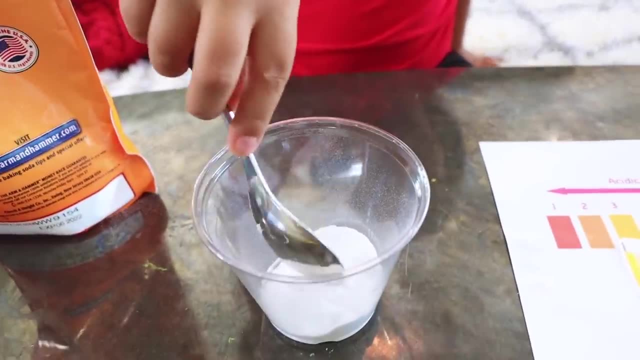 I don't think it's acidic, but I don't think it's basic. Really Okay, let's try it. Oh, It's okay. Okay, so, because it's not a liquid. you know what we have to add to make it a liquid, What It's like a wild. 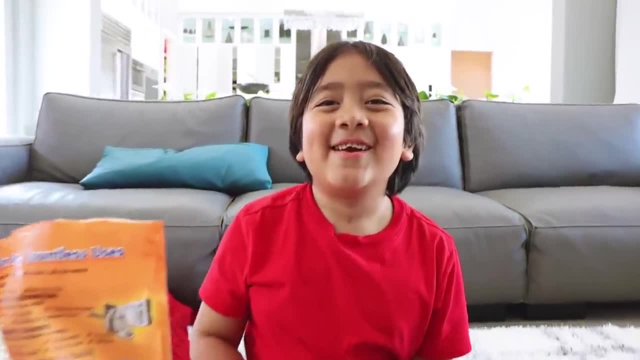 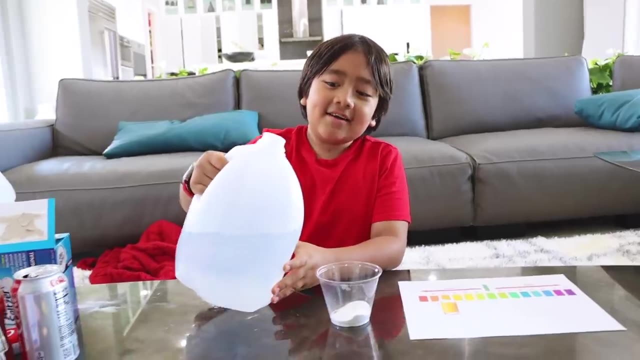 guess, Waiter, Waiter, Waiter, A waiter. Yeah, We don't have a waiter here. Water Water- Usually pure water is neutral. Yeah, But because Mommy had used some of these water, it's probably been. 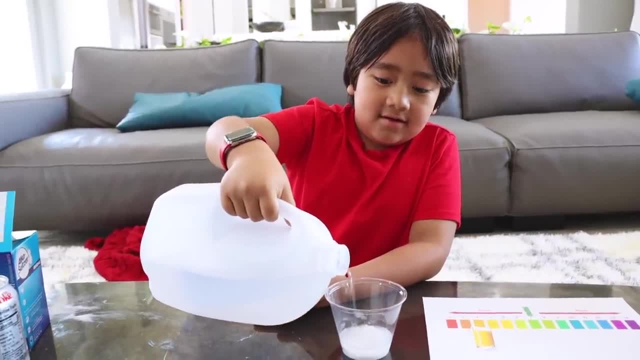 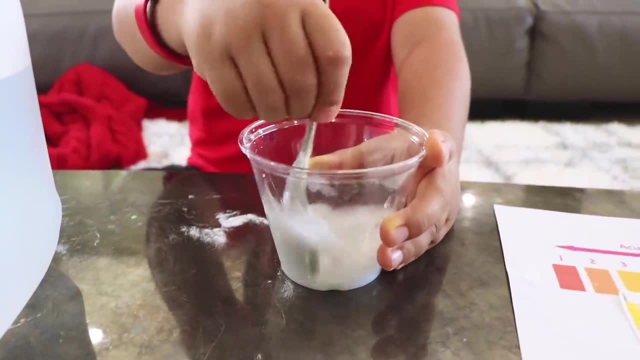 exposed to the air, and so it's probably a little bit acidic. but it's okay, It'll still work. I think that's good. Okay, Agitate, agitate. don't forget to keep agitating For ten hours. 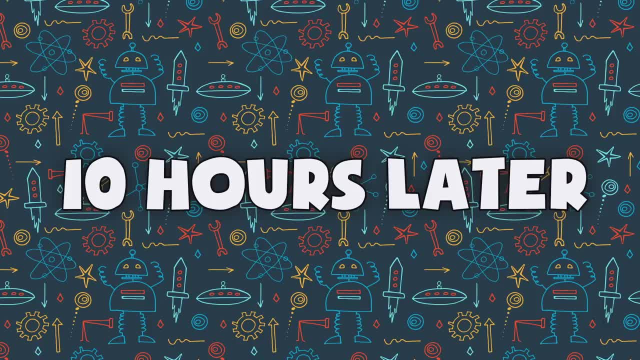 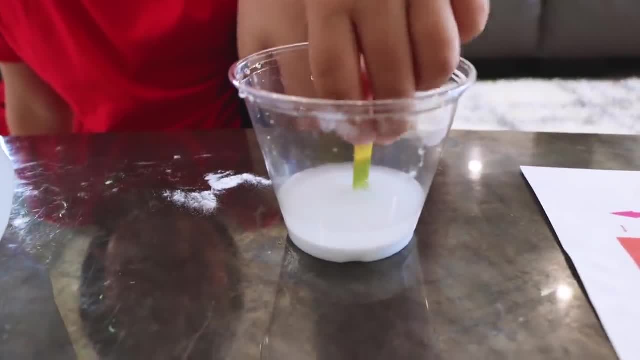 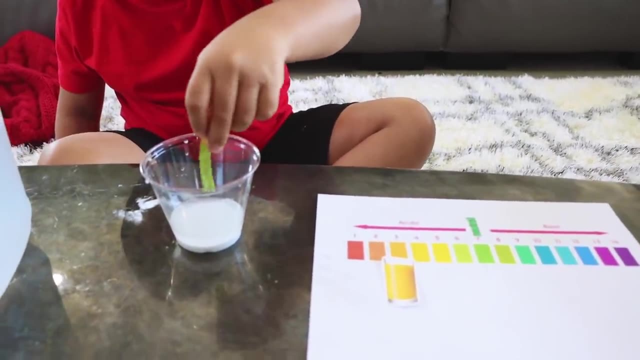 Ten hours later. Just kidding, guys. Let's see if Ryan is right. Ryan is this neutral. Let's see Whoa, It's green. Okay, so let's match it up. Okay, let me dry it off. 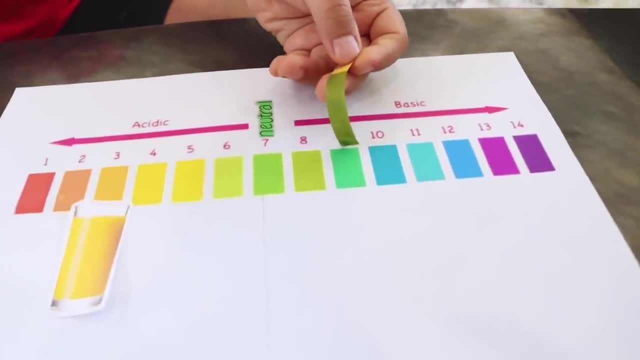 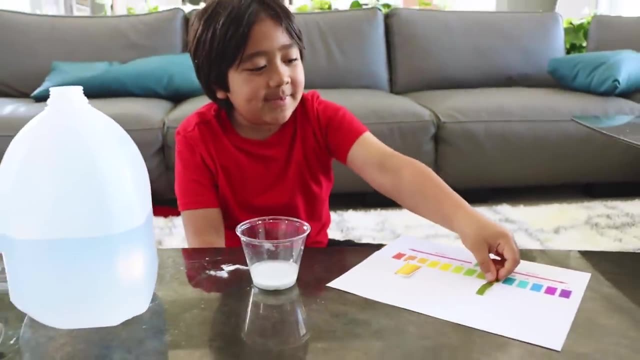 Okay, where does it go? Where does it go? Like here? You think so. Maybe It's either basic or neutral. I'm guessing it's basic. Okay, so basic, it is so Basic, Basic. We got baking soda. 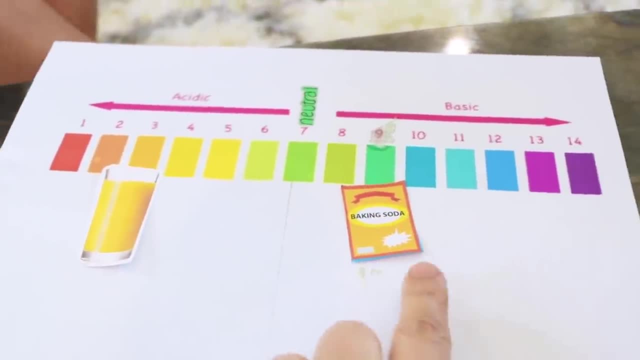 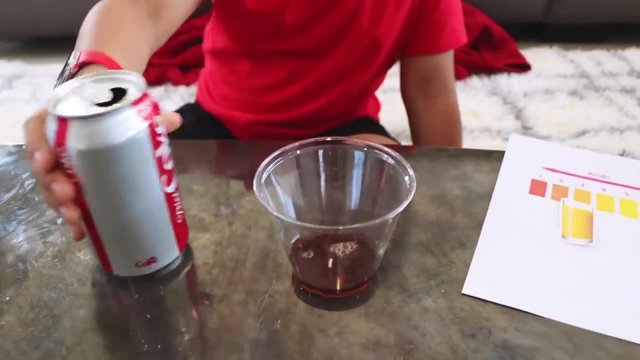 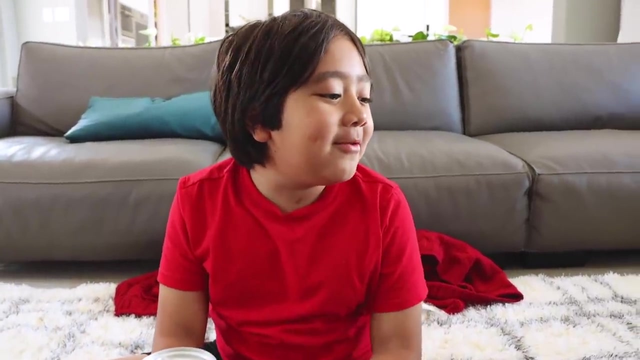 Here we go. So we have one acidic so far and then one basic. Next liquid I'm gonna test is soda. Here we go. What do you guys think? Is soda acid or base? I wonder. What do you think? Ryan, Probably. 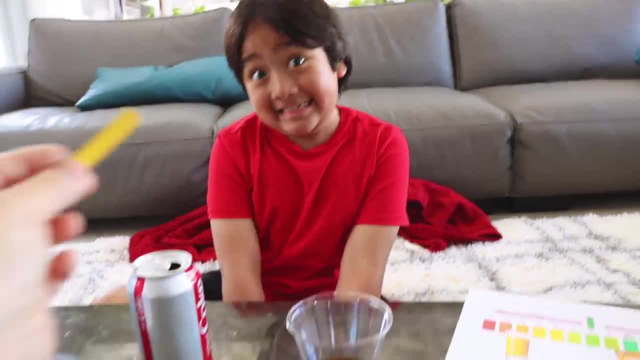 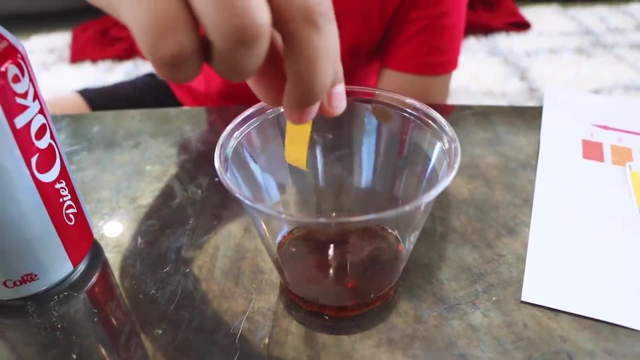 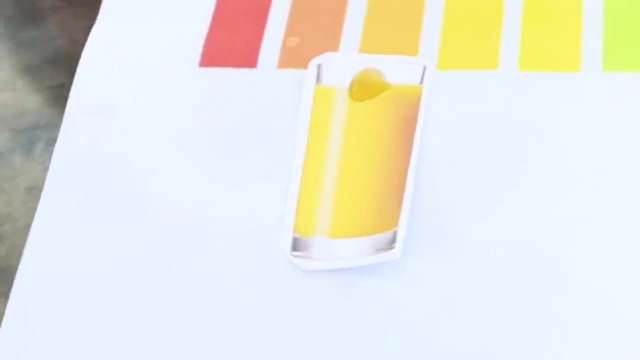 acidic Acidic. Okay, Here's your universal indicator. Let's see what it indicates. It indicates an acidic Acidic. Yeah, Oh yeah, it's like the same as the orange- Same huh. Yeah, Here it is on top. 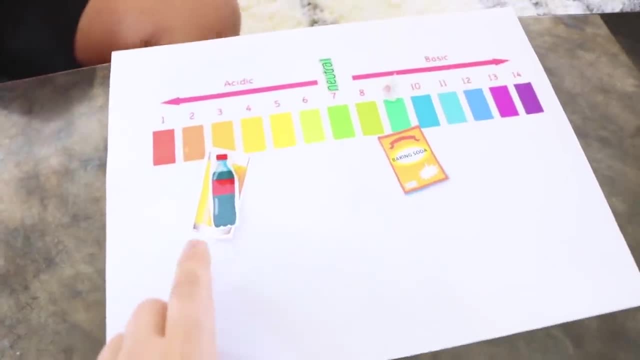 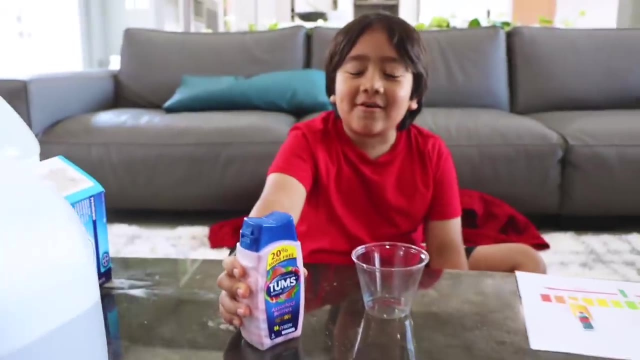 of the lemon. No, not lemonade Orange juice. So they're both acidic. Next we're gonna try out Tums. Do you know when you use Tums? When your Tums has a stomach ache, That's right. when your tummy? 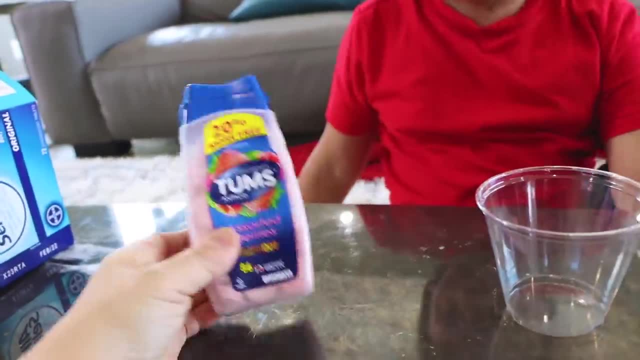 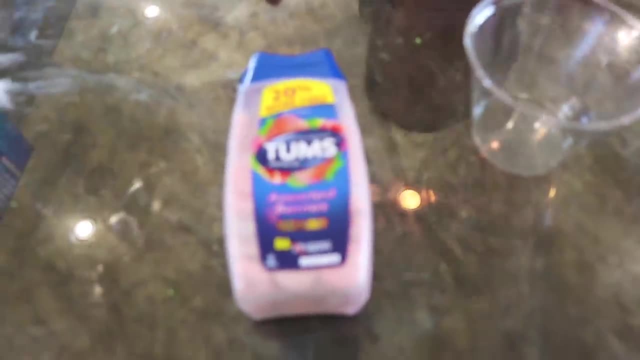 hurts, right? Yeah, So let's figure out. is the Tums an acidic or a basic? What do you think? Probably acidic, Acidic. Okay, Look at the name of Tums Ryan. It says a Tums is. 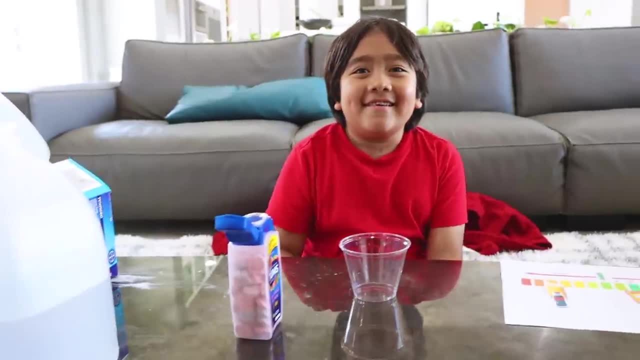 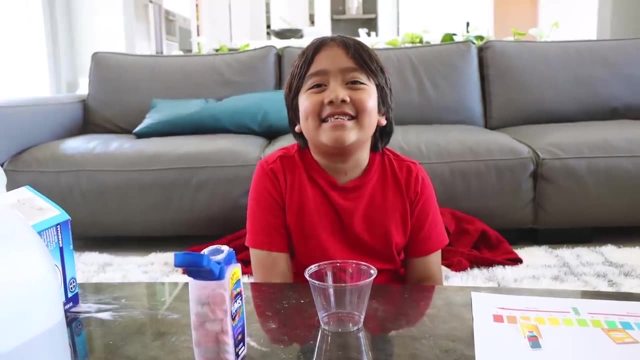 an anacid. What does an mean? Think about the word ant, like anti-bullying, anti-social. What does that mean? It means against, Against, So against acid. So what's the opposite of an acid? Basic, Basic. 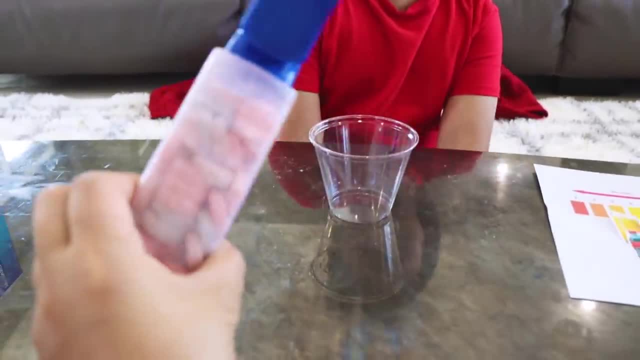 But we'll see if it's right. okay, Yeah. So first, because this is not liquid, you're gonna have to put it in. You have to put it in water, Water. Good Ryan's pouring some water. Okay, okay, okay. 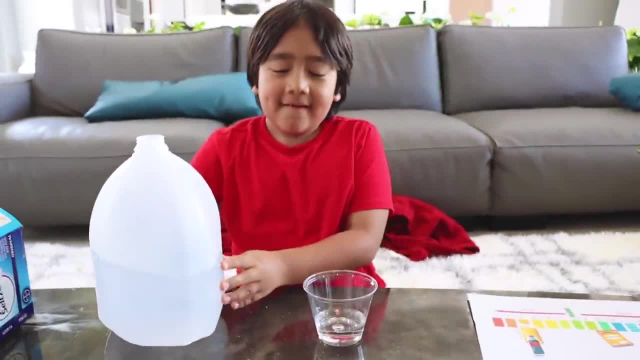 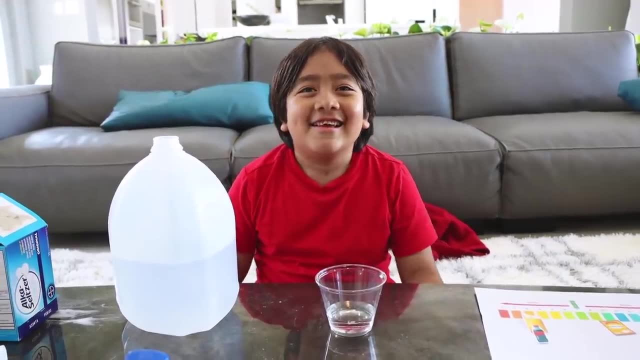 Go go, go, go go. Ryan. bonus question for water. Do you know the chemical compound of water? Uh, What? What is the symbol of water? H2O? H2O- good job. Or aqua? 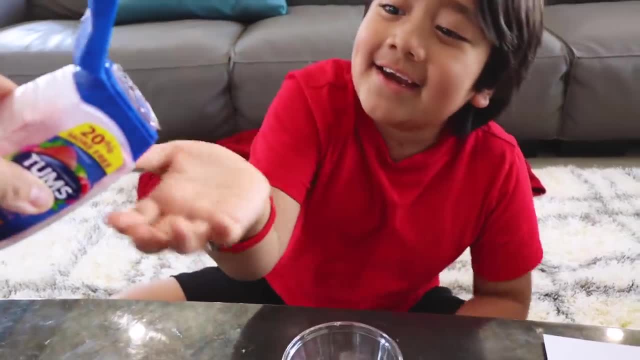 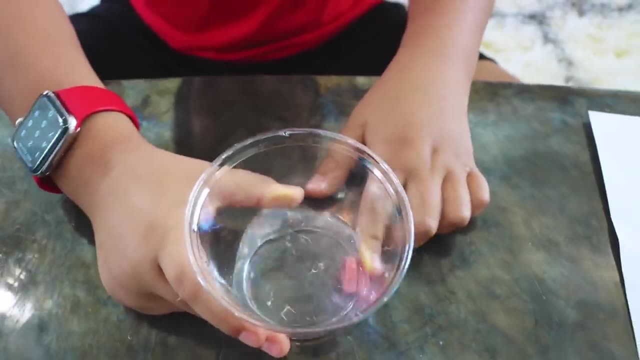 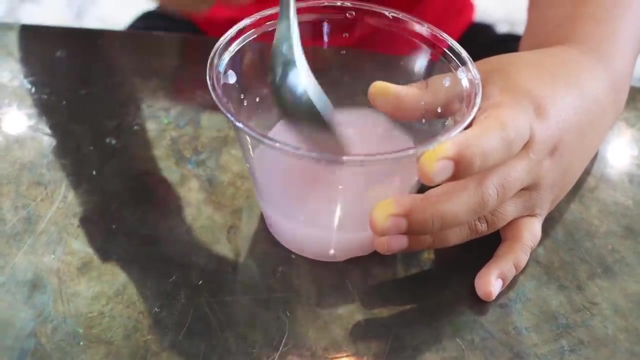 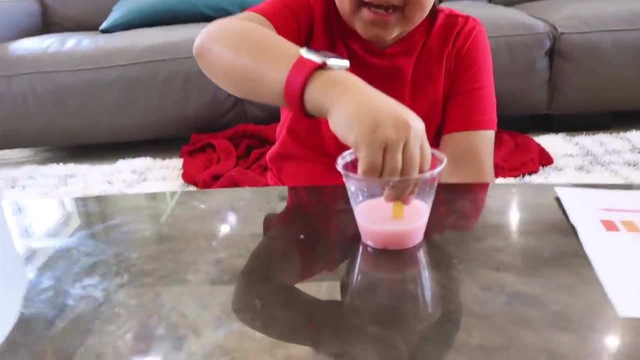 Here is a Tums for you. Okay, A Tums, Have fun Shake, shake, shake. So we might have to crush the Tums Ten seconds later. Now we put in the universal indicator And it says it's an eight. 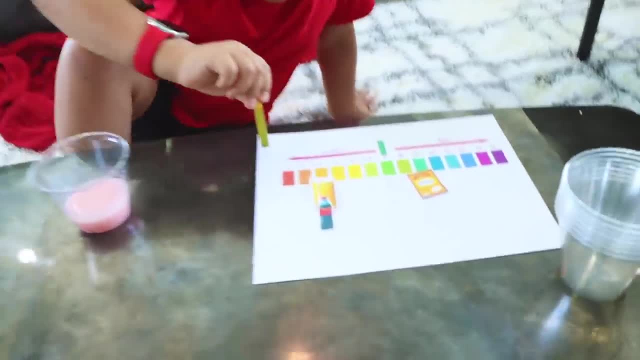 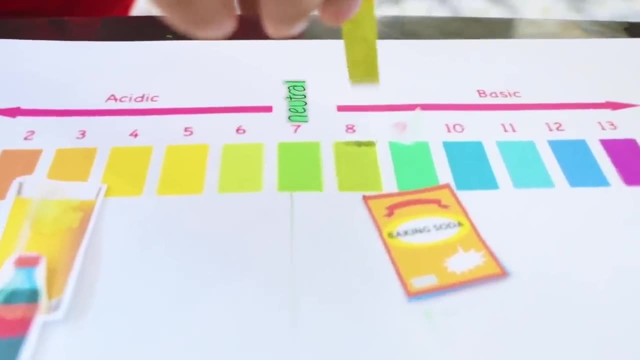 Okay, so let's test it out against the chart. Okay, let's see. So it's none of these. I think it's this one right here. It's eight. Yeah, Yeah, looks good, There we go. Tums is a basic, That's. 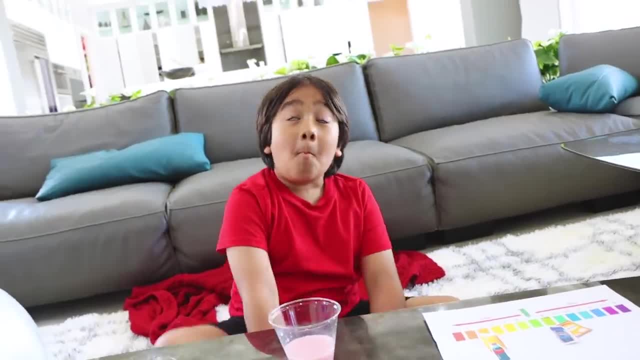 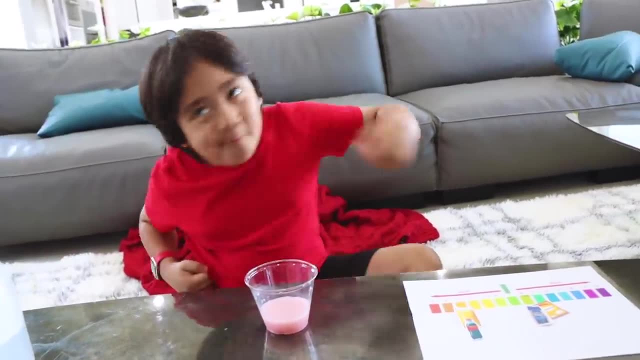 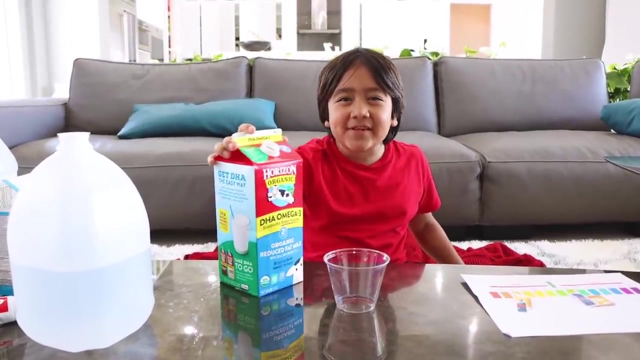 right? yeah, So when you have a tummy ache, it means your tummy is maybe too acidic. so you want something to fight against the acid, which is something basic To neutralize it. yeah, Now we're gonna try some milk, my favorite drink. 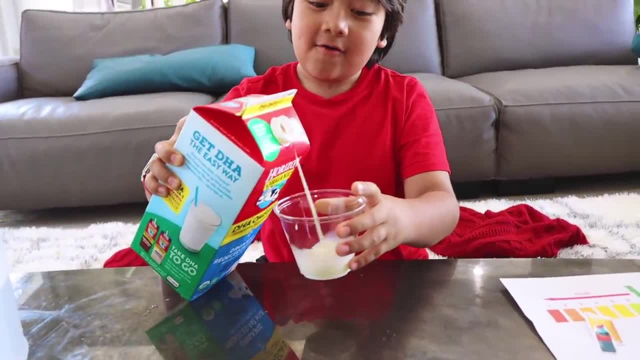 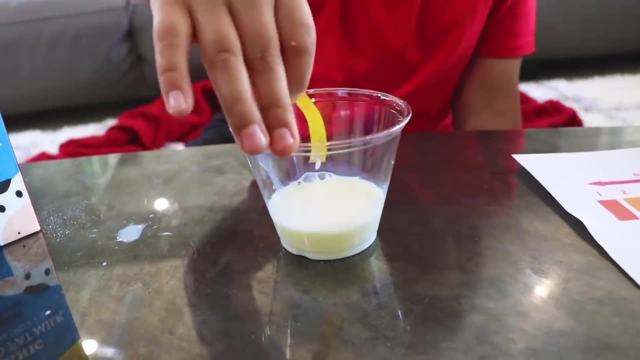 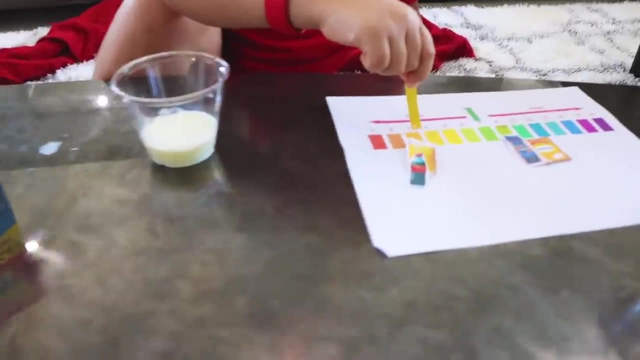 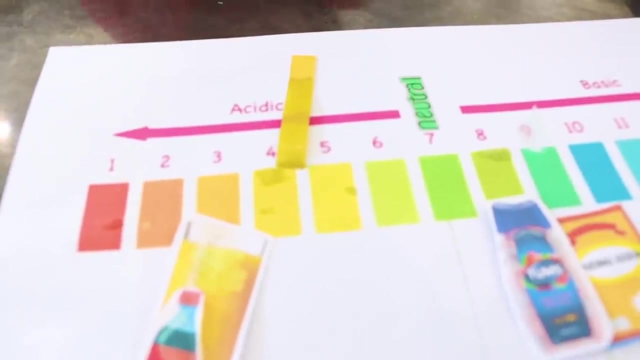 in the world. Okay, Good, Oh, And now the universal indicator. What is it indicating? It's indicating this one, I think Five or four, they kind of look exactly the same. Oh, Kind of between a four and a five, right Yeah? 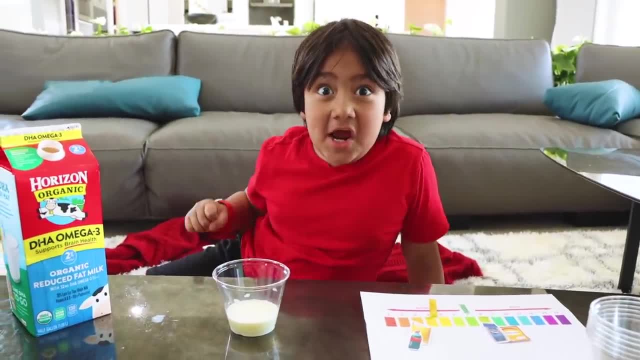 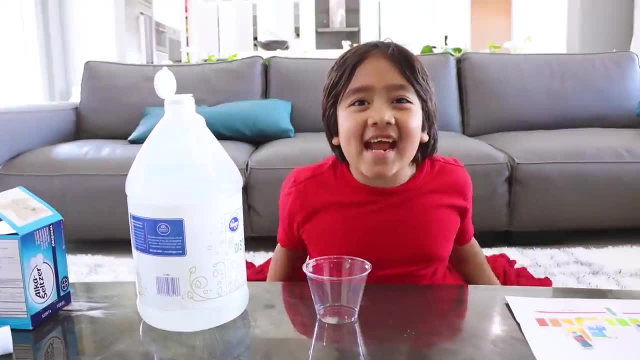 Okay, so what does that mean for milk? It means it's acidic, Acidic. So far, these three things are acidic and these two things are basic. Next we're gonna try out vinegar. I think it's acidic, You think so? 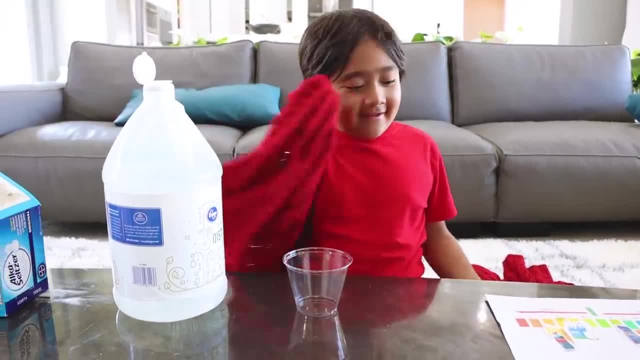 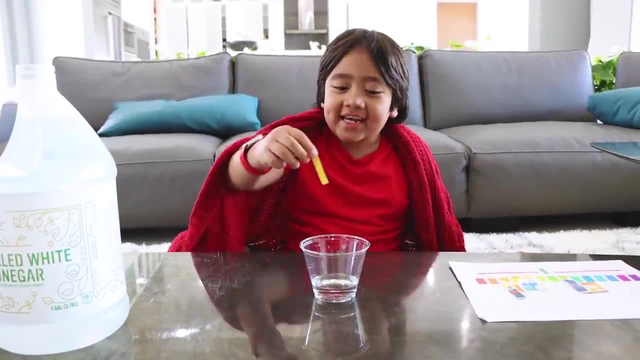 I think it's number one or two. You think it's that strong? Yeah, Okay, let's see. That's enough. there you go. That's enough Now I'm gonna use a universal indicator. Wait, it's number two. Yeah, it's number two. 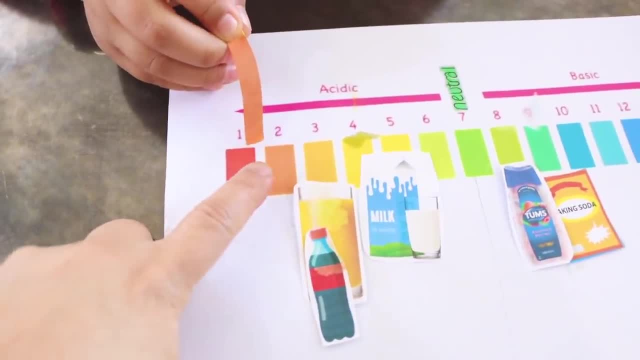 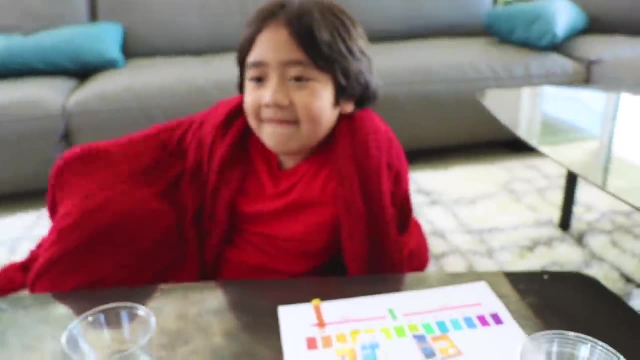 You're right, Ryan. Yeah, So what does that mean? Is it more acidic or less acidic than the milk? More acidic, That's right, More acidic. So here is neutral. Neutral is seven. So the further you go away from neutral this way, 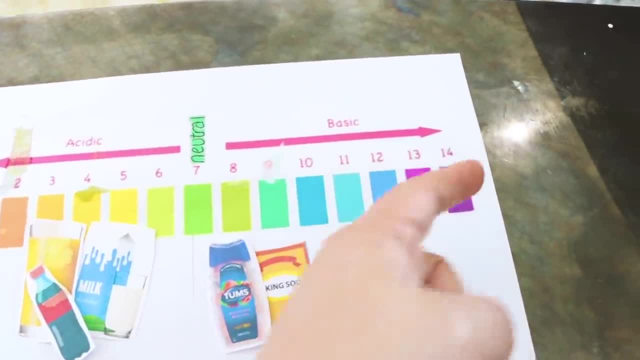 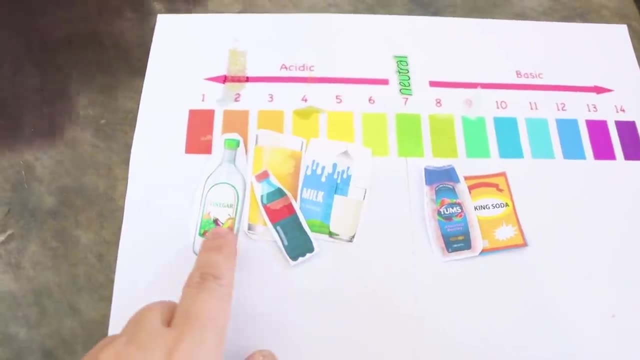 the more acidic it is, And then the further you go away from neutral this way, the more basic it is. Vinegar goes right here. There you go, So which one of these are the most acidic Vinegar? Vinegar goes further away from seven. 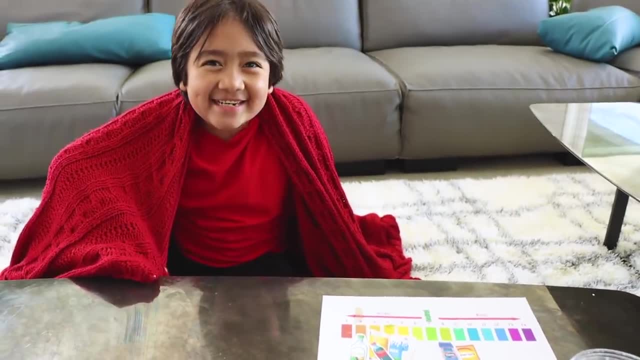 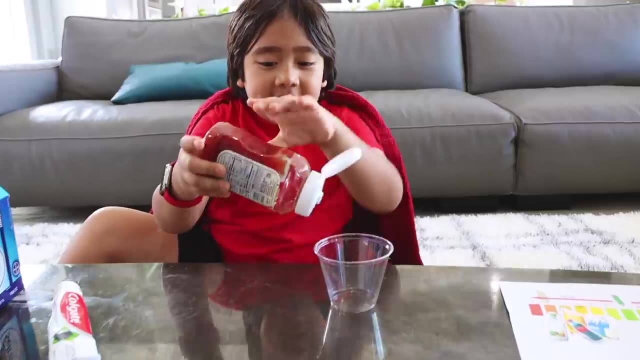 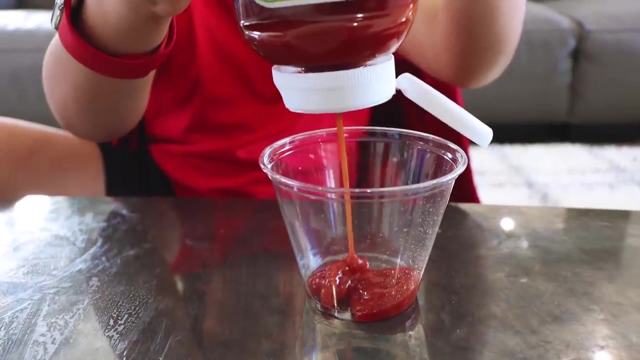 Good job. And the one that is the most acidic is basic soda. Basic soda, Yeah, Baking soda. Next, I'm gonna test out ketchup. Put some ketchup There you go. Perfect. We have to actually put a little bit of water in. 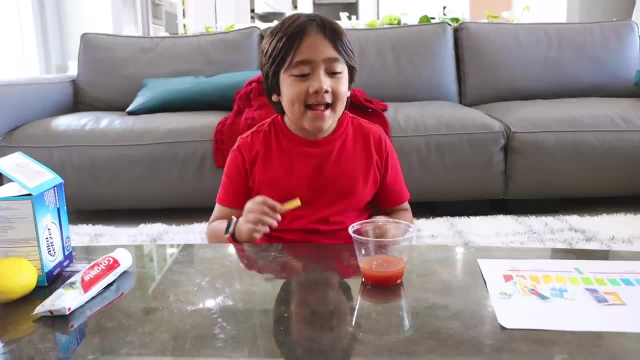 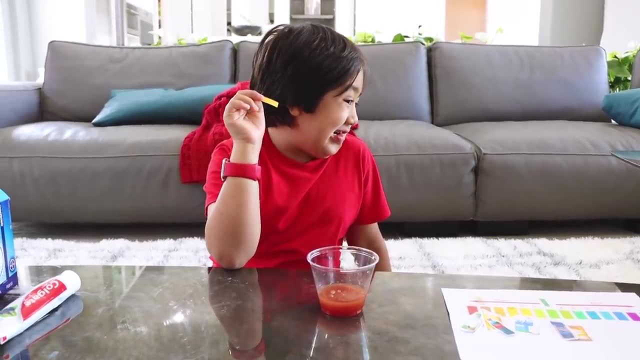 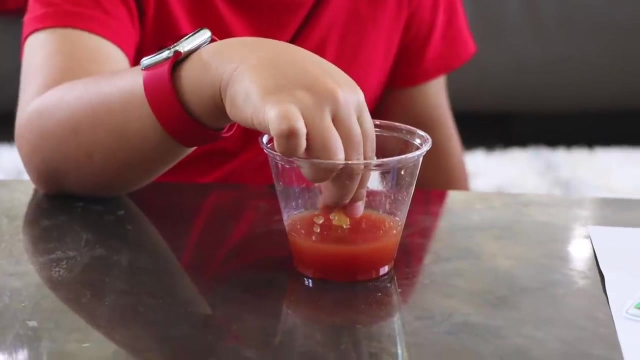 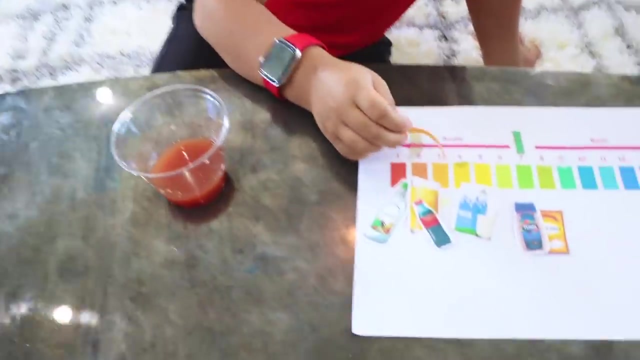 Agitate, Agitate. So what do you think it is before you use the universal indicator? Probably Basic, Basic. No, I think acidic, Acidic. It is acidic. Okay, which number? Let's see. Wait, it's number three. 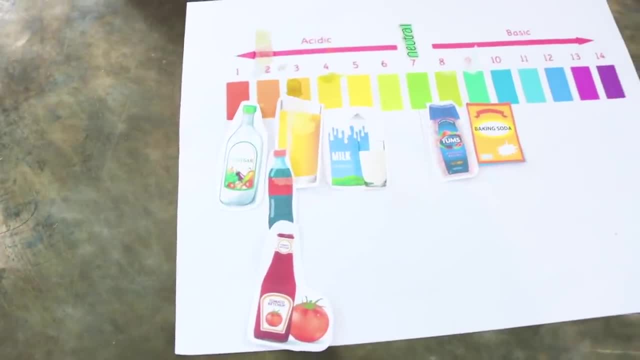 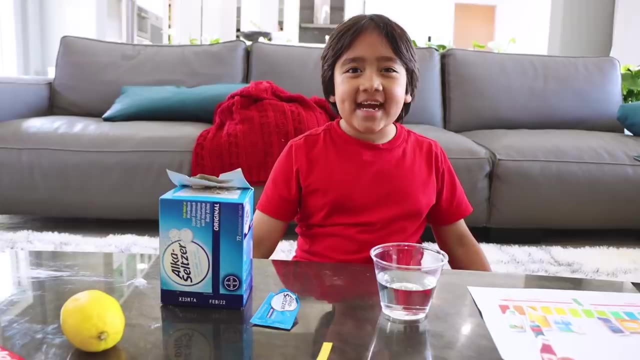 Another three. Yeah, Well, we have three threes. Yeah, you guys, if you noticed, you've been eating and drinking a lot of things that are acidic, correct? Yeah, Next I'm gonna test out Alka-Seltzer. 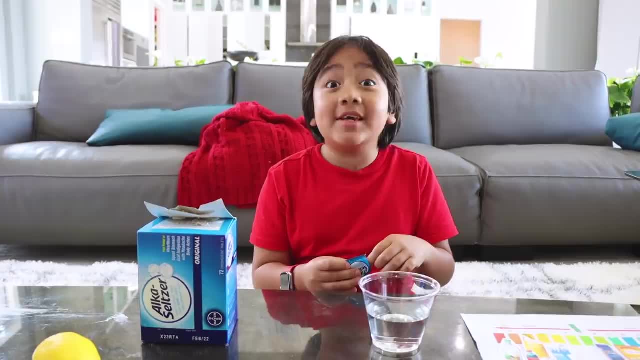 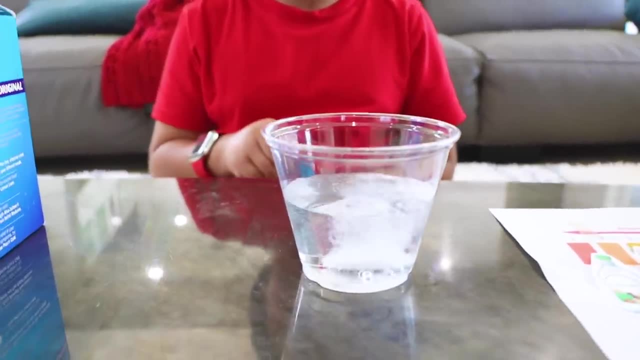 Okay, do you think Alka-Seltzer is acidic or basic? Probably basic Basic. Yeah, so you also use Alka-Seltzer if you have like a tummy ache. So it's also an antacid, Whoa, But I like Alka-Seltzer. 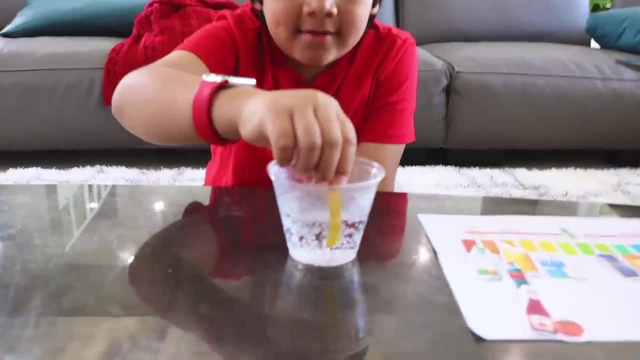 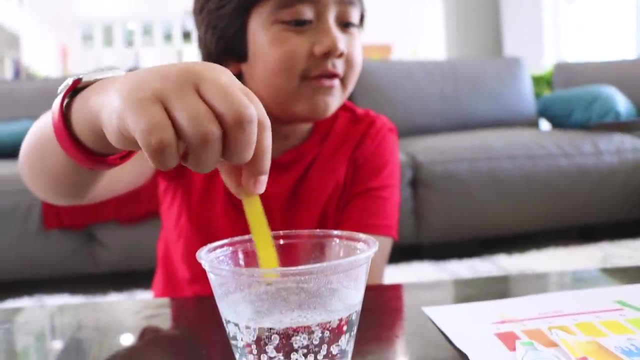 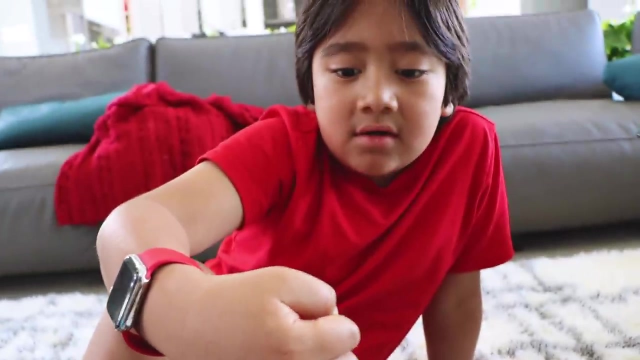 Look how it stays in bubbles. Yeah, Put it in. Whoa, It actually didn't change color. Really Interesting. That's interesting. Oh wait, no, I think it's drying. Oh, so maybe you have to wait for it to dry. Yeah, because it kind of looks. 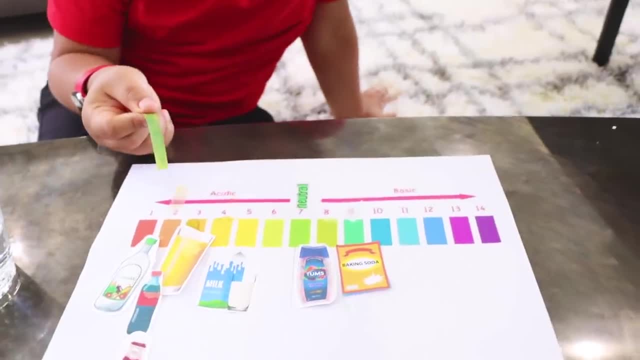 green. Perfect. Alright, I'm gonna wait for it to dry. Hmm, let's see what it is. Oh, I think it's a number nine. It's a basic. Yeah, it's a nine, So is it a weak? 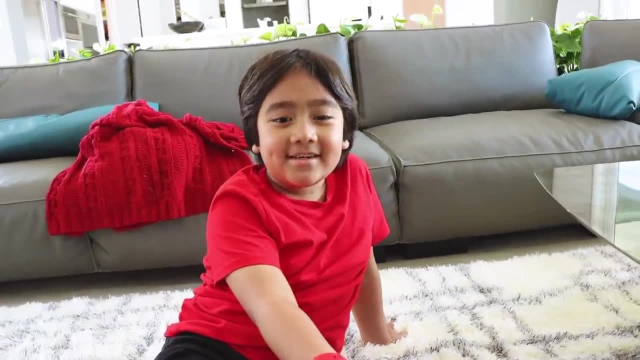 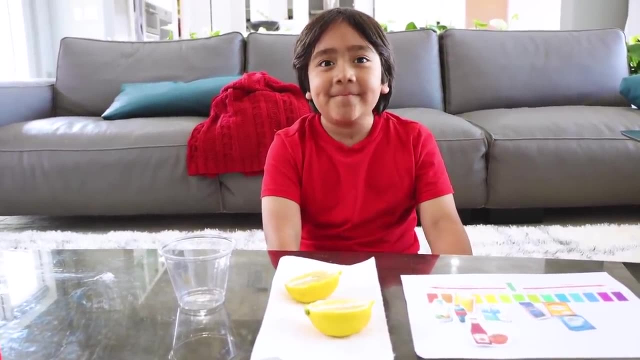 basic or is it a strong basic? It's a weak basic? Yeah, And there you go. Next I'm testing out lemon. Do you know lemon is really sour, Mm-hmm. So do you think lemon is acidic or basic? Probably. 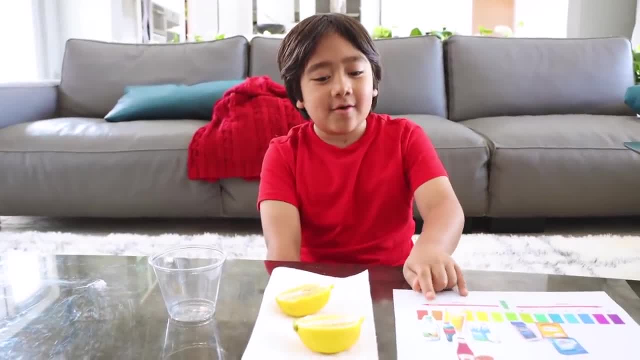 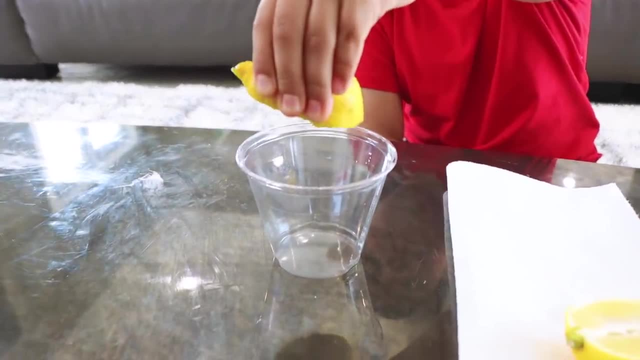 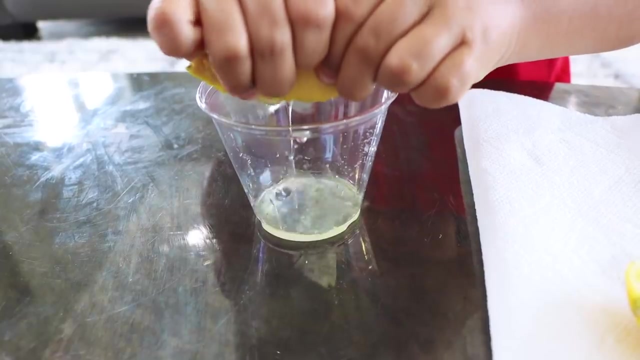 acidic, Really. Okay, It's probably gonna be a three, two or a one. Is that strong? Yeah, Okay, let's test it out. Okay, That one has two hands. Now let's put it inside. It's probably acidic. 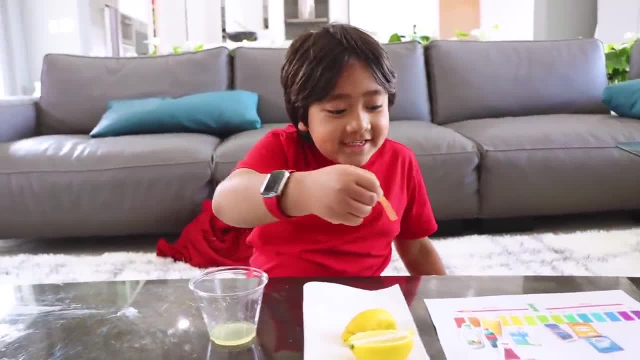 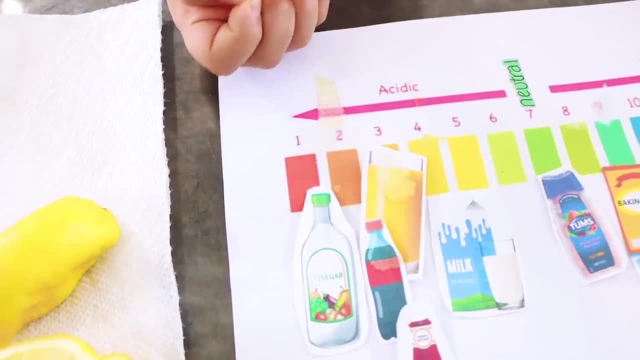 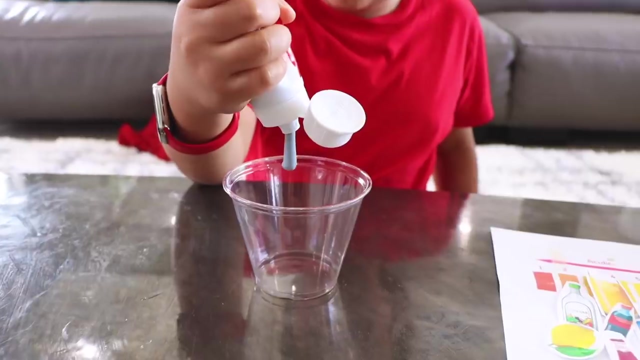 It's number two. It's that acidic, Whoa. Oh yeah, you're right, Ryan, So it's pretty strong. huh Yeah, We can get it right after the vinegar. Now the last thing we're gonna try is some toothpaste. 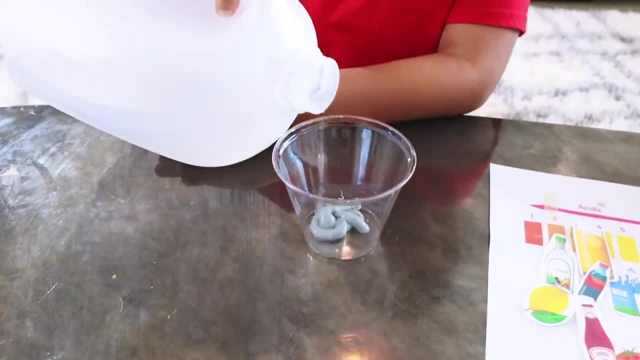 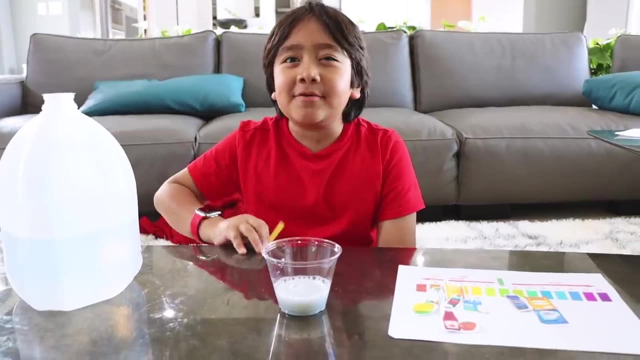 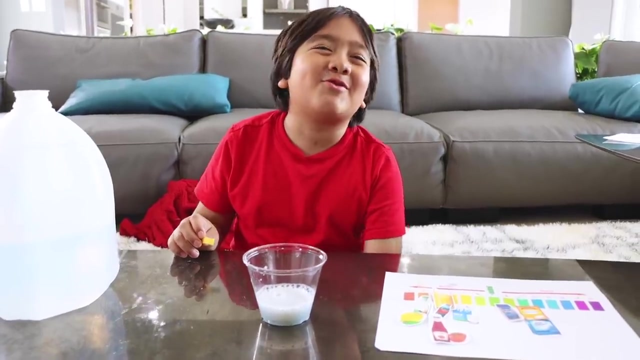 I'm pretty sure we need to put water. That's enough. Agitate, Agitate, Agitate. It's probably done Time to use the universal indicator. Wait, What do you think? it is Probably neutral. Neutral, I mean no, not neutral. 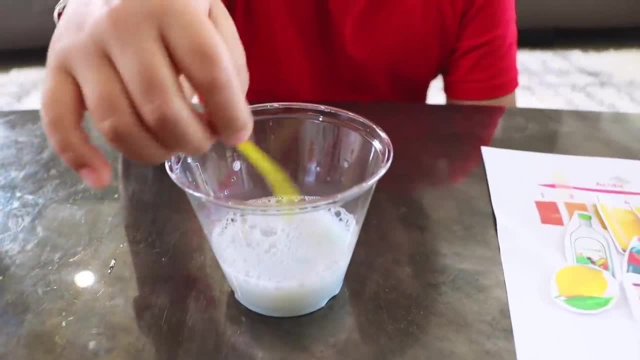 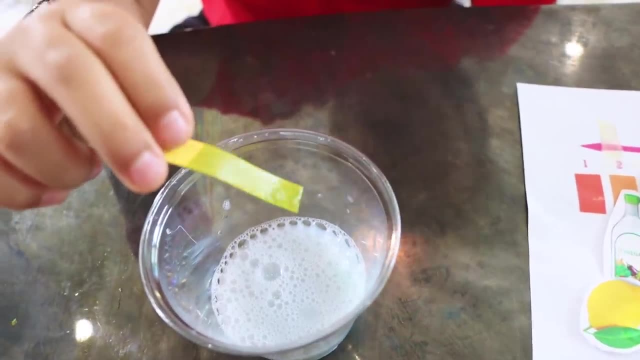 I meant a basic. A basic, I'm gonna say it. What do you guys think? Okay, you gotta wait for it to dry. Wait, I think it's already green. It's getting green, but it's still wet. so we'll wait for it to dry a little bit, But yeah, 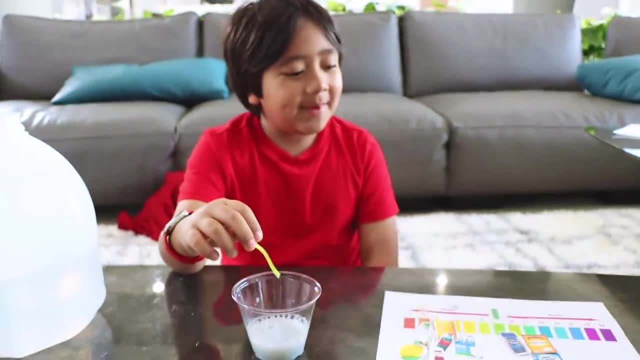 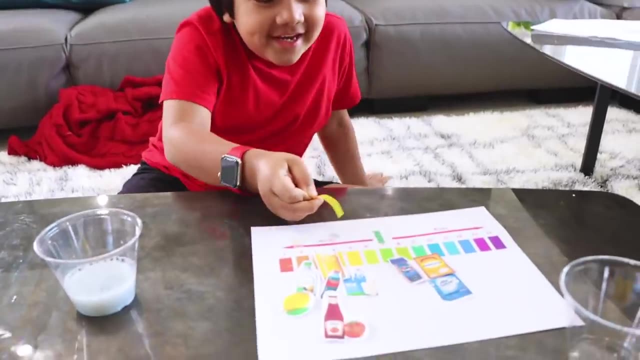 it's already turning green, So it's either a neutral or a basic Seven or eight. Let's wait a little bit longer, Let's see what it is. I think it's an eight. An eight, Yeah. So what does that mean? 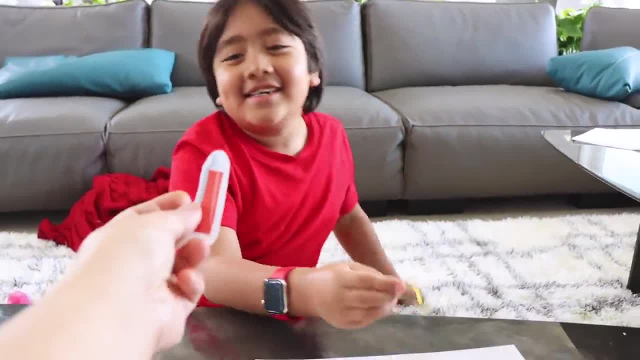 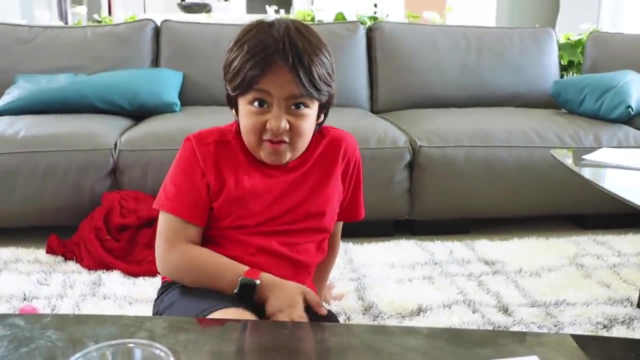 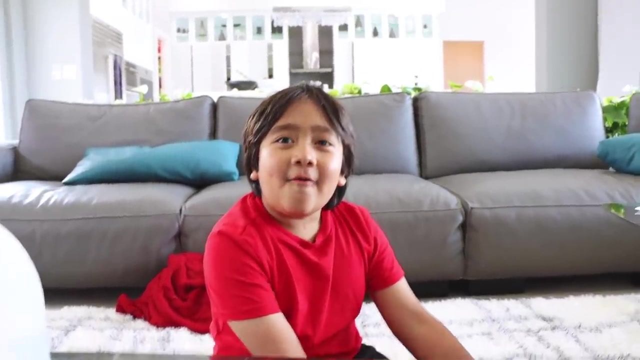 That means it's a basic Basic. Here you go, Here's your lube of toothpaste Basic. A lot of things that you drink and eat are acidic. Since a lot of the things that you eat and drink are acidic, how do you get rid of it Like what's the best? 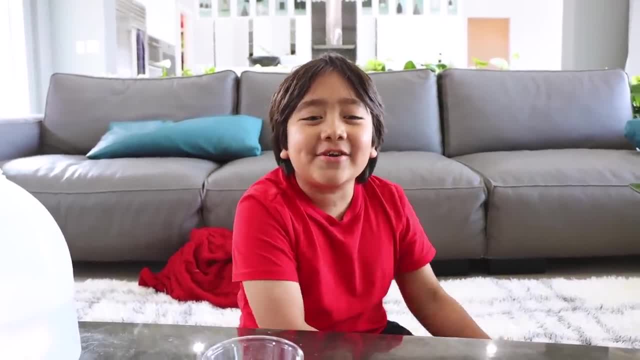 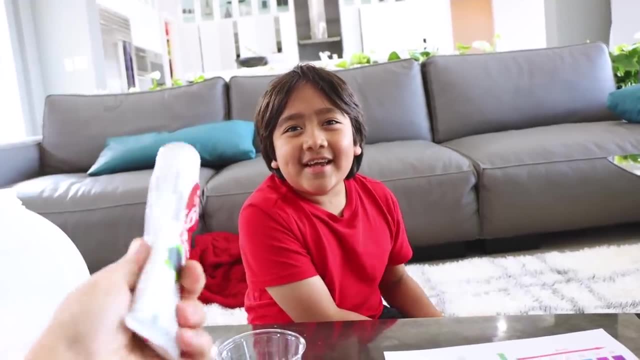 way you think. You eat and drink and put on your teeth. basic things, Basic right. So that's why you have to use toothpaste, and toothpastes are basic to get rid of the acid. We'll be in the video. 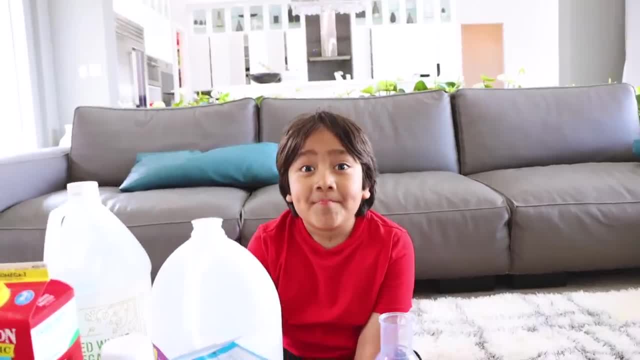 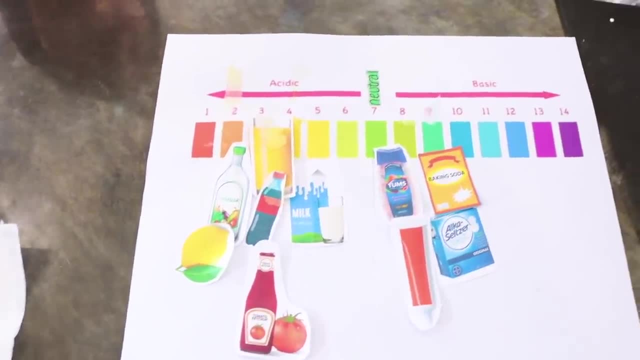 I want to ask you, Ryan, do you know how we always do the baking soda and science experiment video? Yeah, According to the chart, which one is an acid and which one is the base. So the baking soda is the basic Uh-huh And the vinegar. 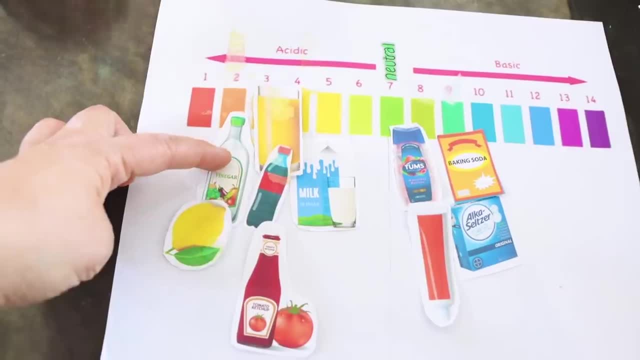 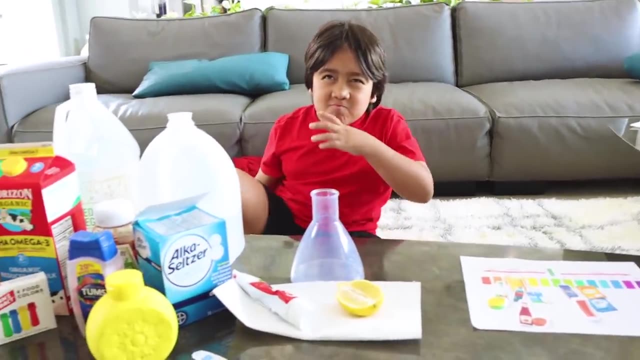 is the super duper acidic Good. So it's kind of the same as the lemon. So do you think that if we replace the vinegar with lemon juice, will it still work? Hmm, Probably Okay, let's find out. Instead of vinegar, we will use lemon juice. 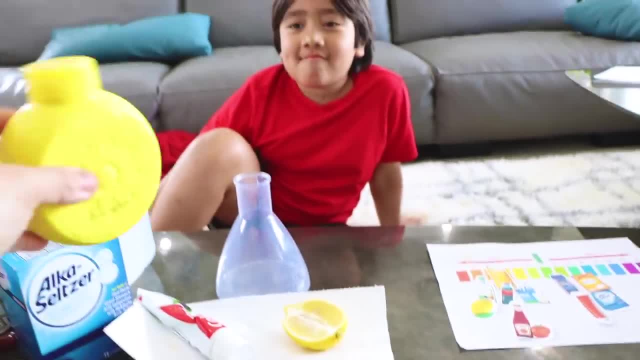 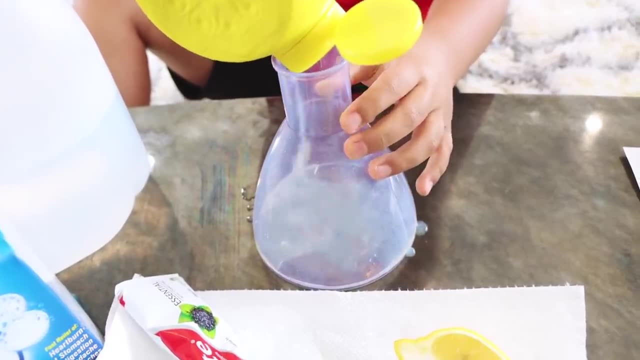 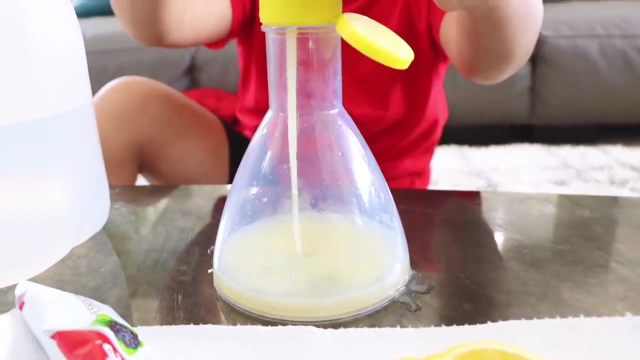 because it will take too long for us to squeeze, and we're going to use the one that they already squeezed for us: Lemon juice, Lemon, Oh, oh, Let's put it like that. Yeah, good idea, Is that enough? 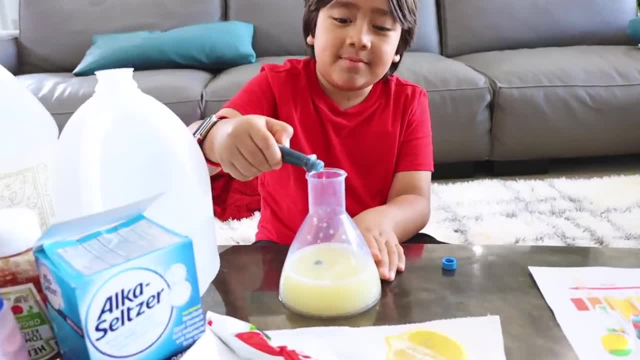 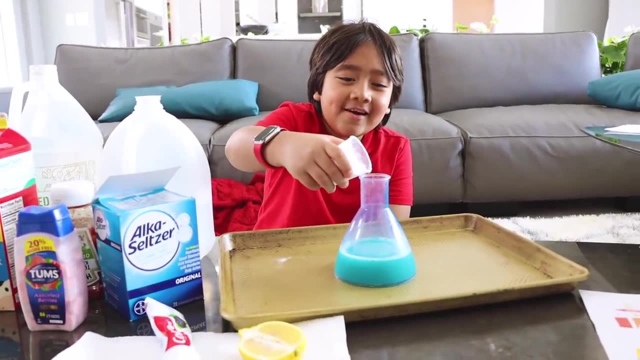 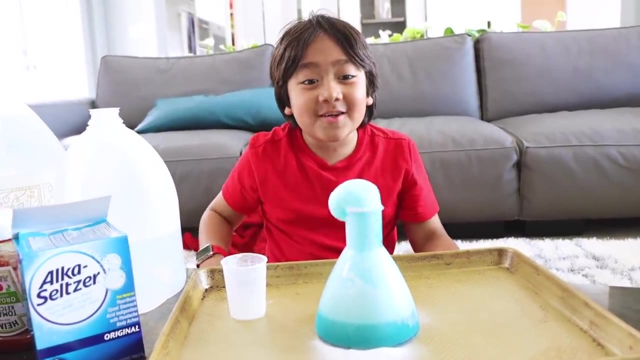 A little bit more Good, Put some glue in. I'll mix that Perfect. Okay, guys, here's the baking soda. Okay, is it going to work? Maybe It works. It's just a little bit less than the vinegar. 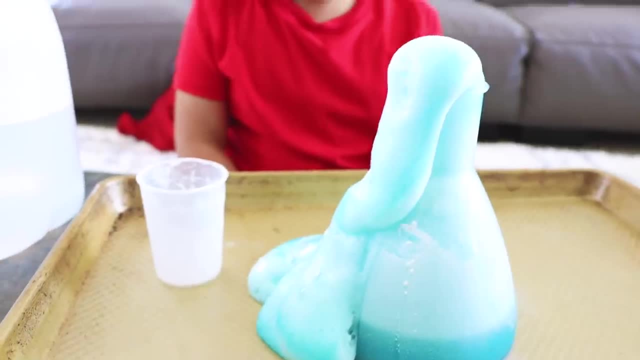 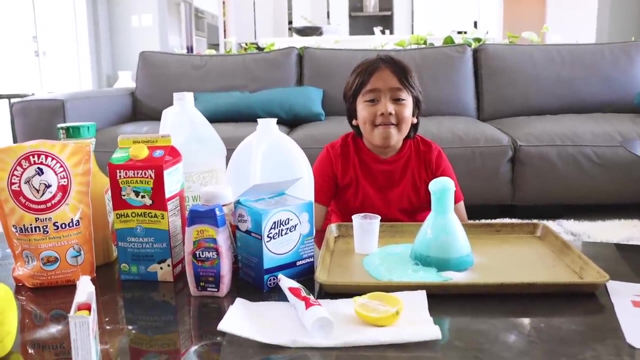 but it works. Yeah, Oh, wow, look at it coming out. That's cool, Yeah, So you guys should also go out and try your own experiment. There's so many other items that you guys could test. Yeah, That we didn't test like a soap. 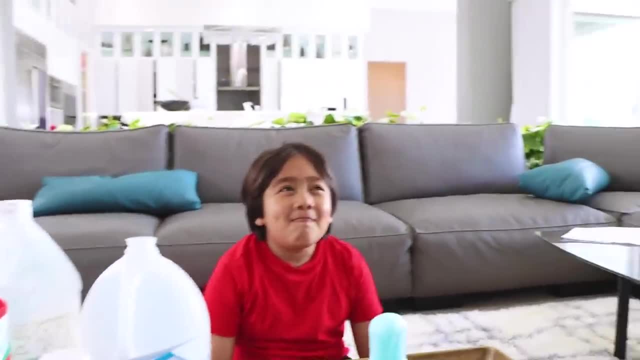 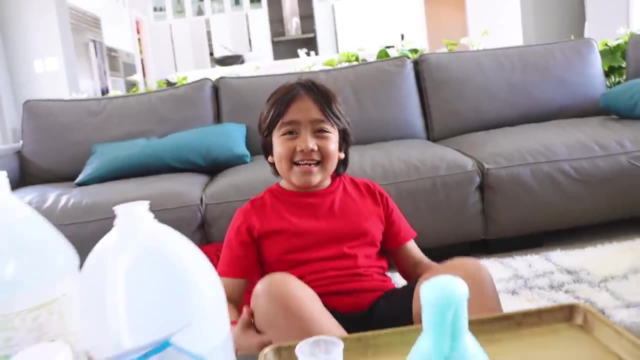 or honey. What else can you think of? Or mayo, Or mustard, Or ocean water, Ocean salt water? Good idea, Yeah, if you guys test it, let us know. Hey guys, today we're going to blow out balloons. 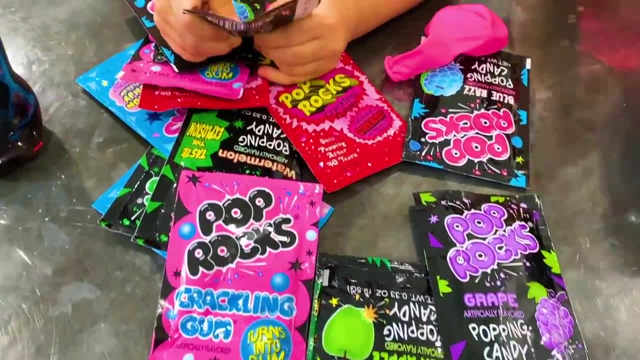 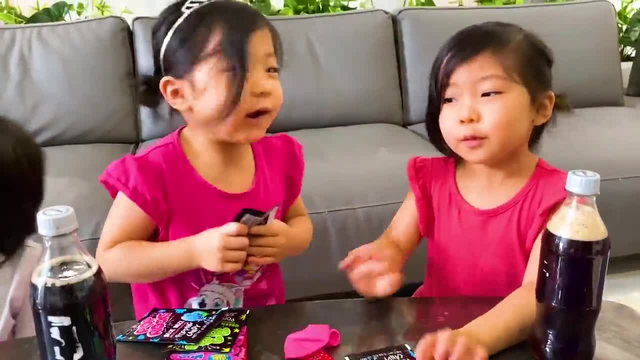 rock candy and Coke. So we got a whole bunch of rock candy here. Have you guys ever tried rock candy before? No, Yeah, You have. Yeah. How about you guys? No, we didn't get it. You want to try it? Yeah. 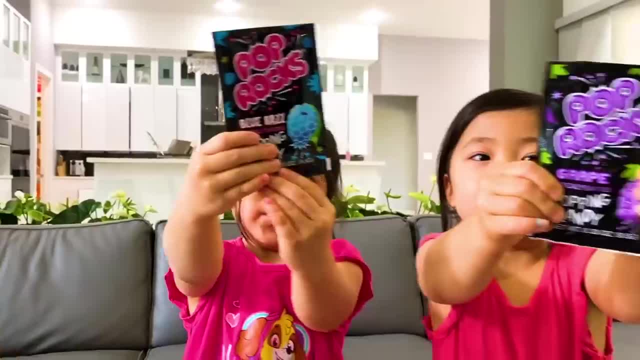 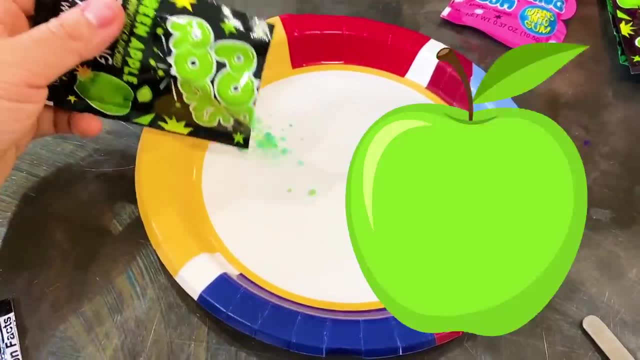 Okay. so which flavor do you want to try? I want this one, Okay. so Emma wants to try blue, Kate wants to try grape And Ryan Green apple. Green apple, okay, Okay, some green apple there, Some grape. 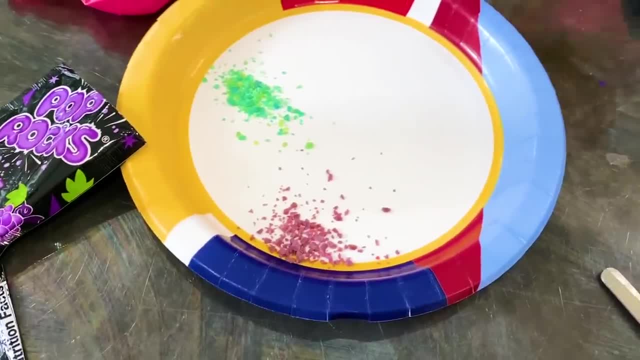 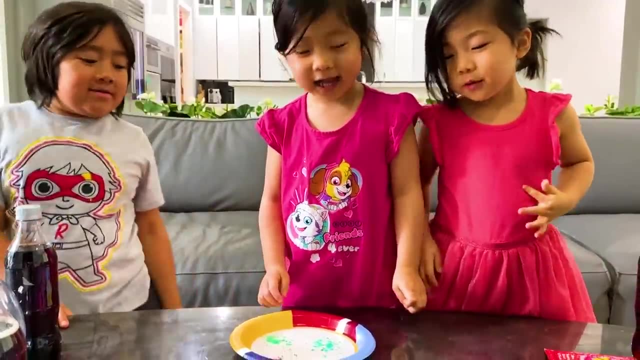 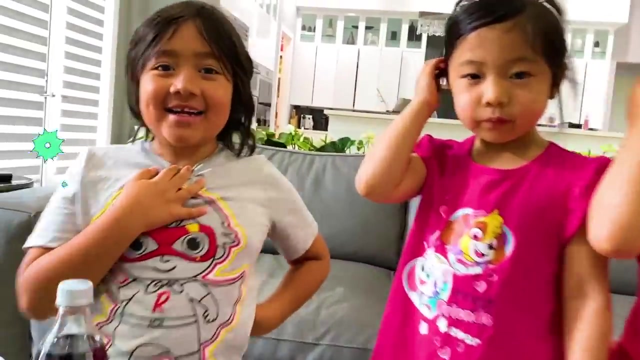 Grape Grape And some blueberry Blue. Can I try, Ryan? Yeah, you guys can try it And you don't have to chew. You just put it in your tongue and it's supposed to pop. Tell me if you feel the pop, Do you? 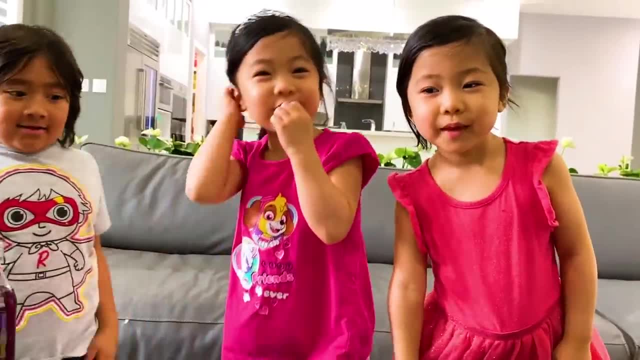 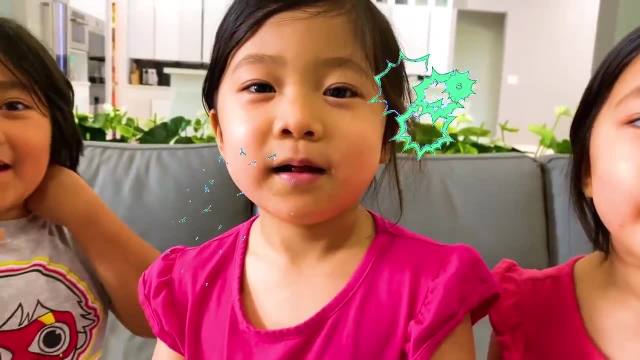 I feel it. I hear it too. Do you feel the pop? Yeah, just put it in your tongue and just keep it there And close it, Close your mouth. Whenever I eat it- and I do this- I hear a lot of pop, I know. 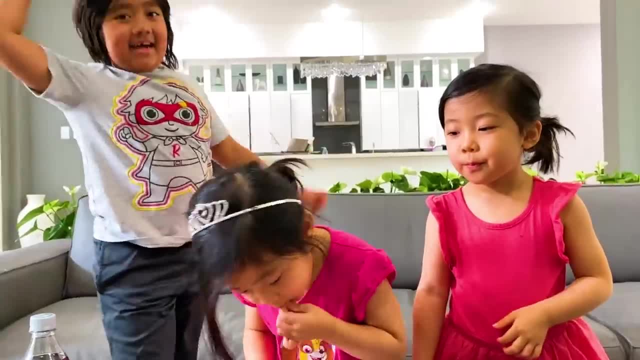 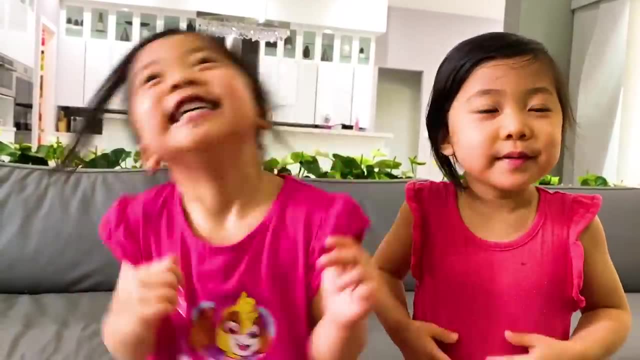 Well, what do you guys think? Do you guys like it? Don't like it. Weird, You like it. How about you guys? I don't feel the pop. You don't feel the pop. What about you, Emma? You probably ate it, Yes, Okay. 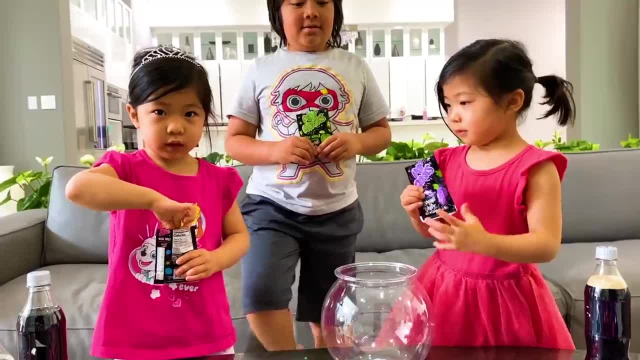 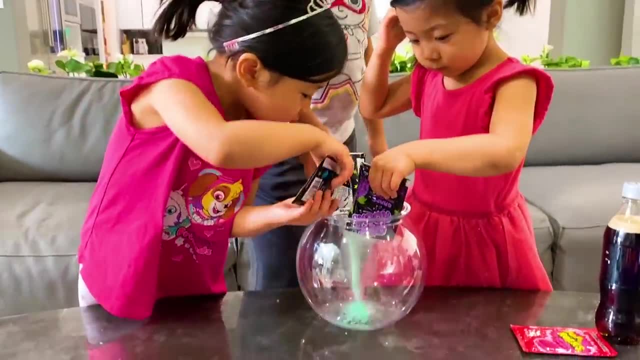 Blow up some balloons, Yeah, Okay, actually, before we try to pop a balloon, we're going to see what it looks like with the Coke. Okay, so everybody pour in their rock candy. Whoa, All of them, Yeah, all of them. 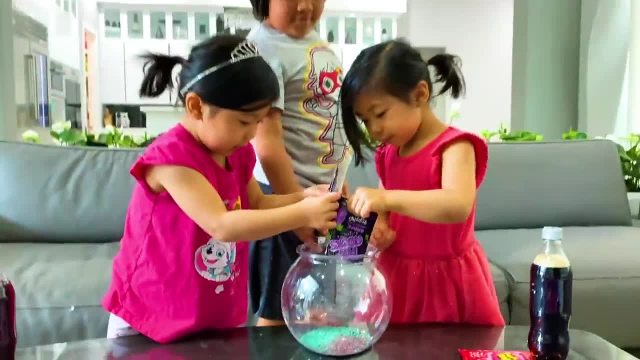 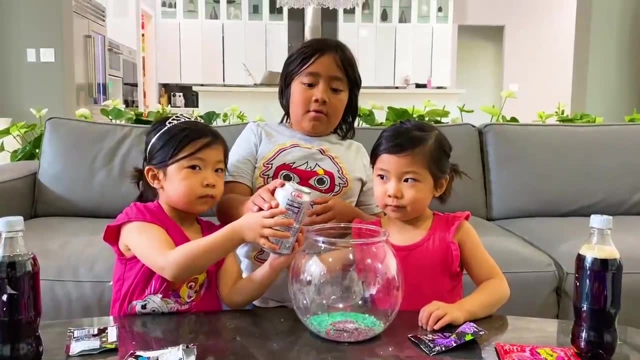 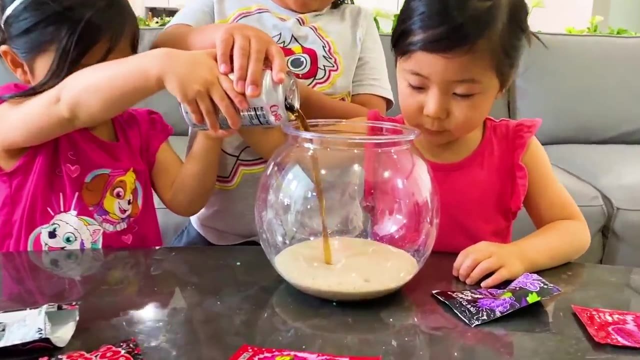 All of them. There you go. There's a lot of green, I know, Emma, Yeah, Okay, so now we're going to try the Diet Coke in there and see what it looks like. Whoa, Wow, that's a lot. 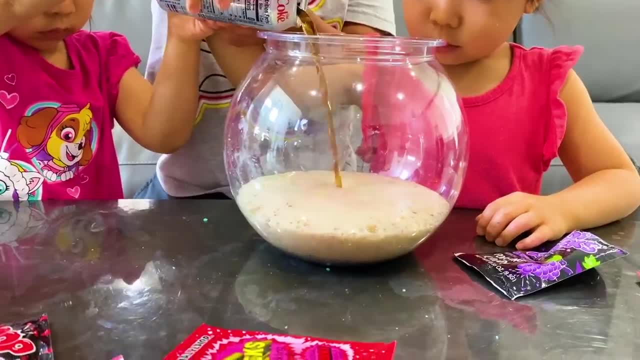 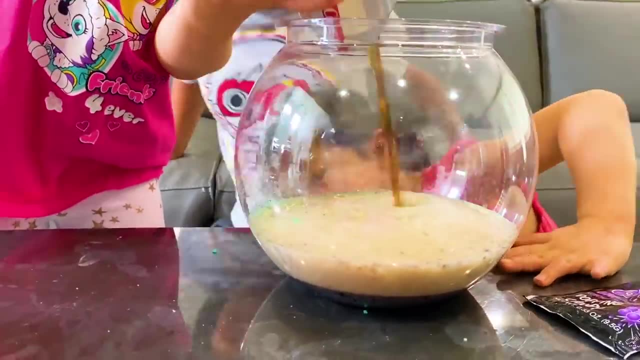 But we want to eat it. I know we have a lot more Whoa. Okay, I don't know if we need that much. Okay, Wait, there's like, it's like kind of changing different colors the Diet Coke. 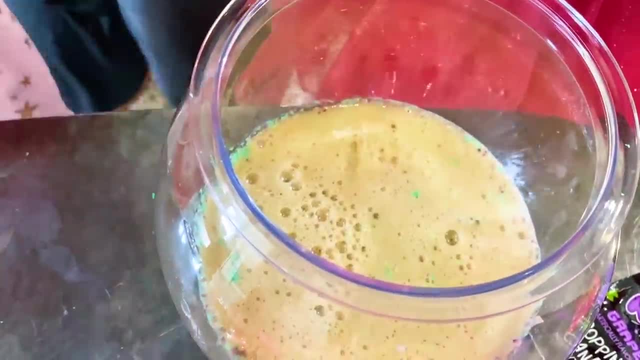 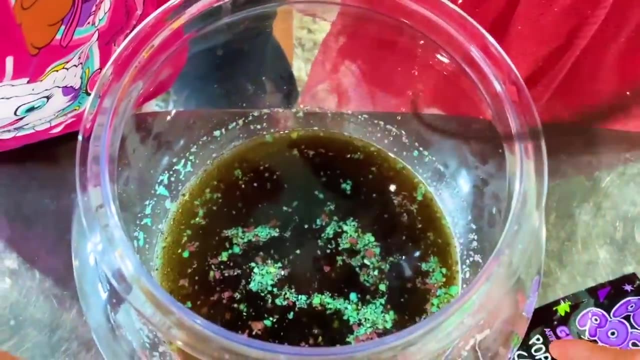 Do you see the pop in there? That's too much Diet Coke. Yeah, maybe we're adding too much, you guys? Do you guys hear the popping sound? Yeah, Whoa, it's popping. I want to put up more. 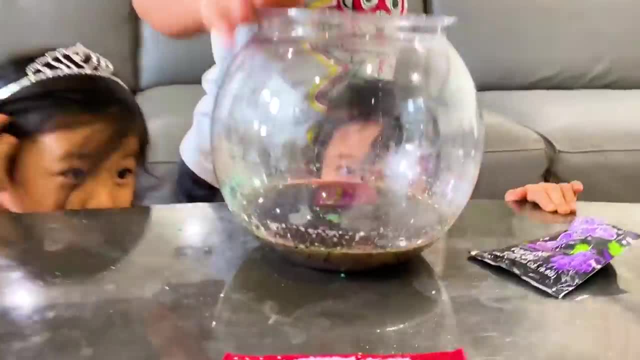 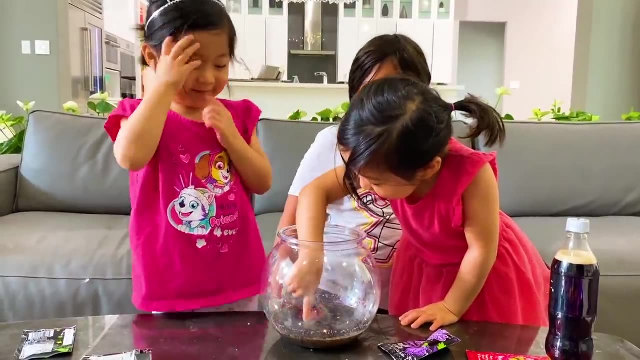 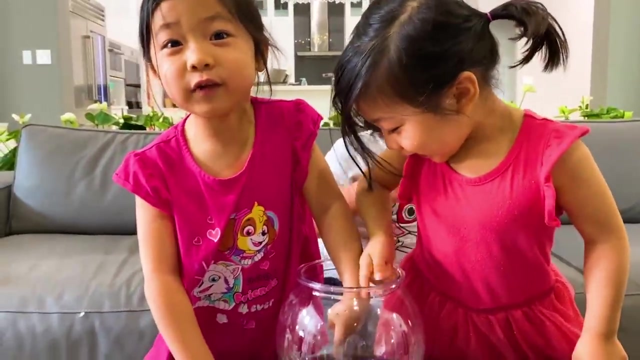 Do you see the popping? Thank you, Mommy. How does it taste? How does it taste? It tastes good, Does it? Yeah, Okay, just one little taste Thumbs up. It kind of tastes like 1% of the taste of Sour Patch. 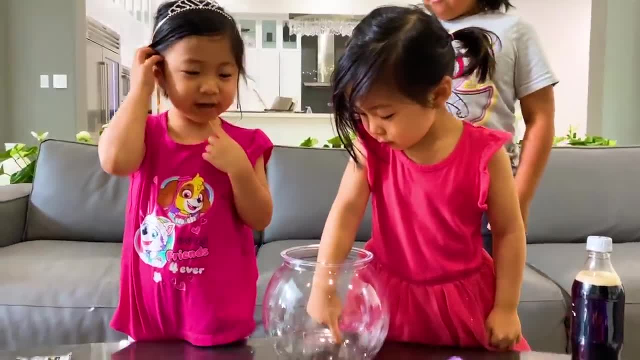 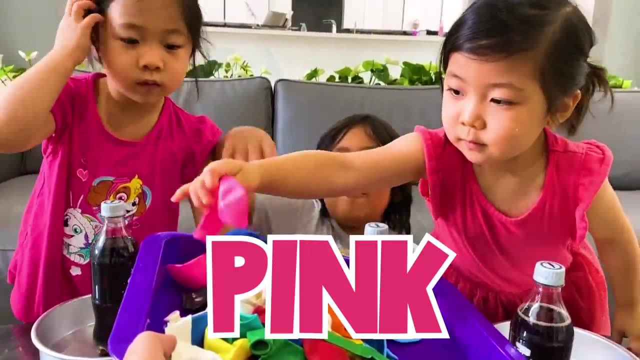 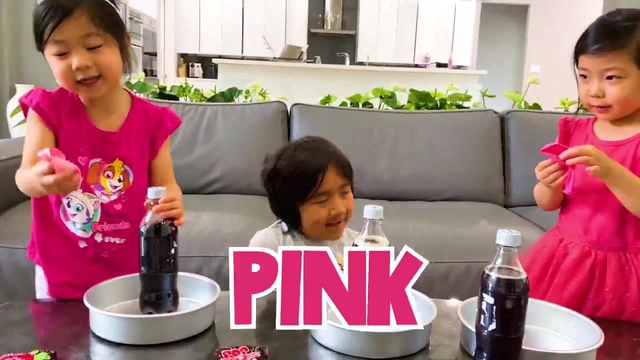 Really, Yeah, Sour, Interesting, Okay. so now we're really going to do this experiment. Okay, first you're going to pick your balloons. Pink, blue, pink, Okay, change your mind. Pink, okay, I like this pink. 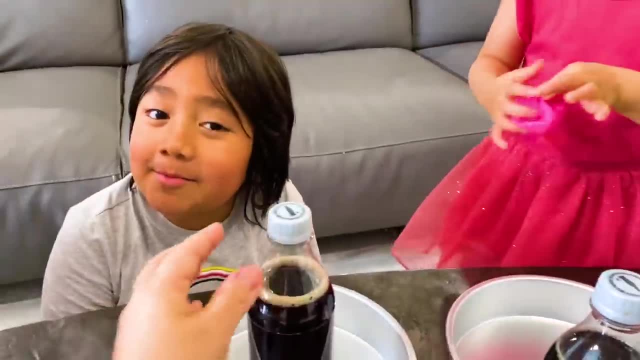 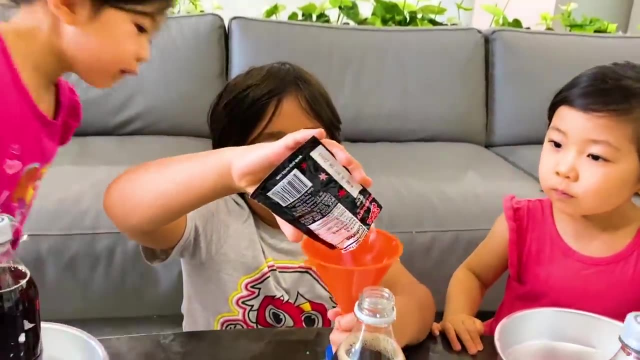 Okay, I like this pink. Should we put the rock candy in the balloon? Yeah, so first, that's right. Good job, Ryan. yeah, Alright, we have a funnel to the balloon. Now. Ryan's going to put the rock candy inside, like that. 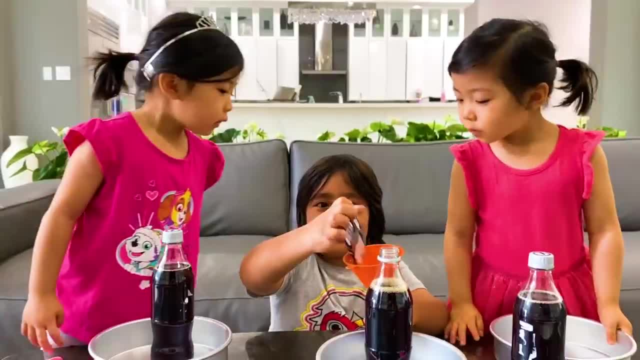 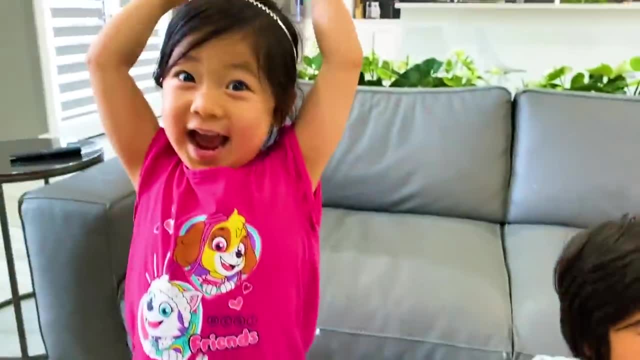 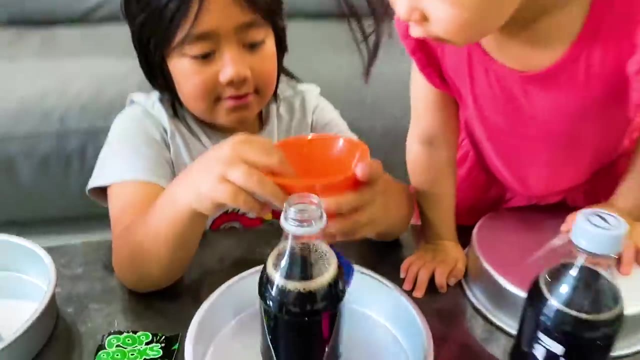 Okay, we're going to use both because we are courageous. Yeah, Go big, or go home, right. Yeah, Go big, Go bigger. Oh it's a lot. Yeah, Shake it, Shake, shake, shake. Okay, Ryan, here's for the hard part. 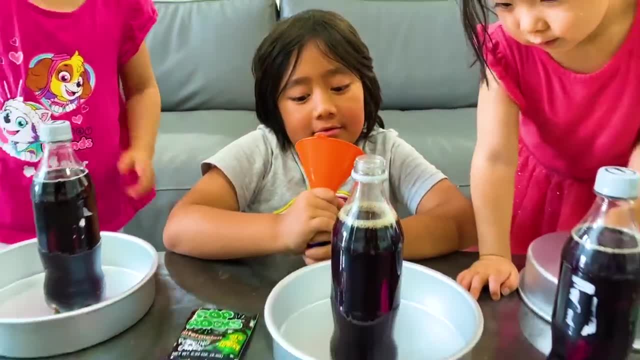 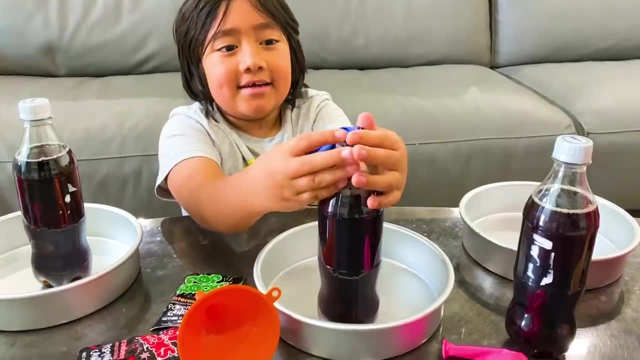 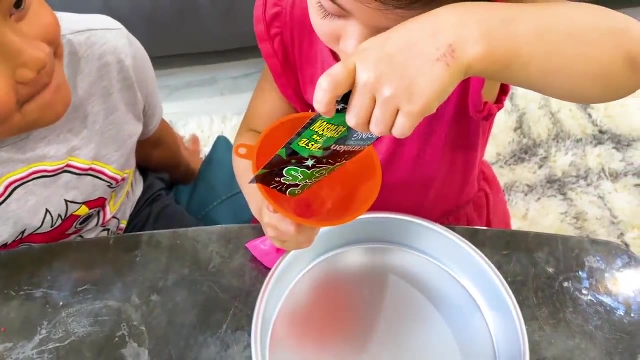 Can you put your balloon over this without it going in? Yeah, Maybe You got it. You got it, Got it. Alright, Kate's turn. Good job, Kate. There you go The whole thing My turn. Yes, Emma, your turn. 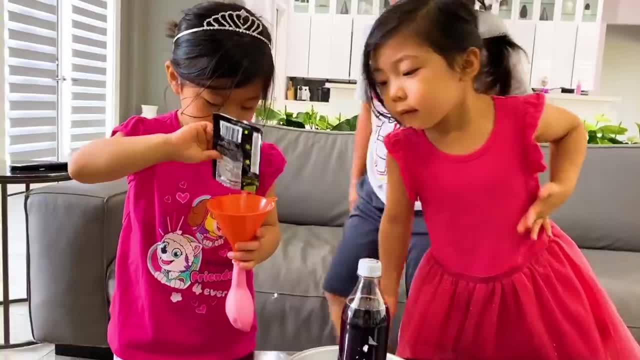 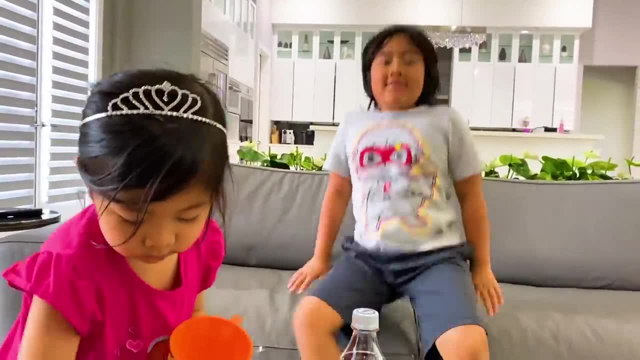 Yes, your turn, Emma. Okay, now Emma's turn, of course, But this part needs two. Yep, we're going to try two. Probably works with one, but maybe we can get a bigger balloon, right? Yeah, Now we're going to put it down. 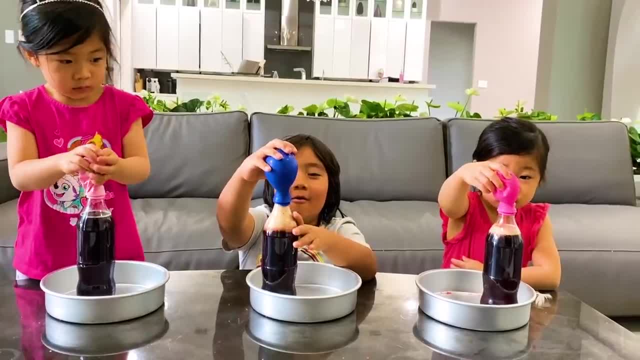 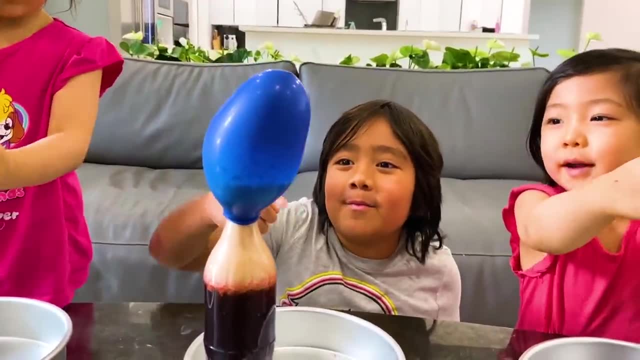 Three, two, one go One. Whoa, whoa. The balloon is getting bigger. It's so big and I still see a lot of it. Mine's bigger, Mine's more bigger. Yeah, Mine is more bigger. Yours have a weird shape. 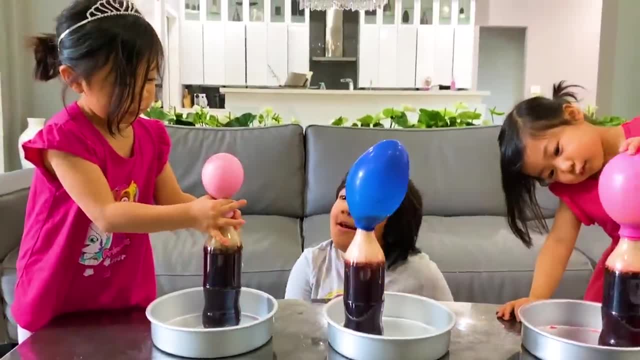 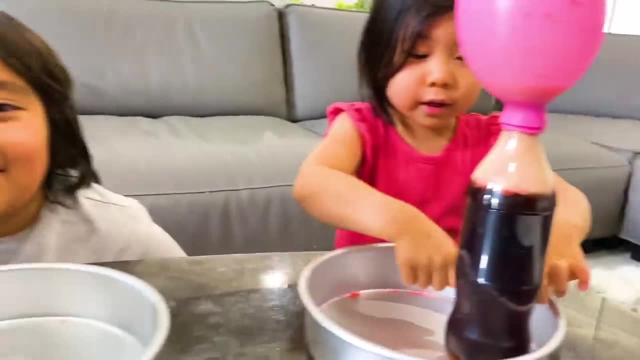 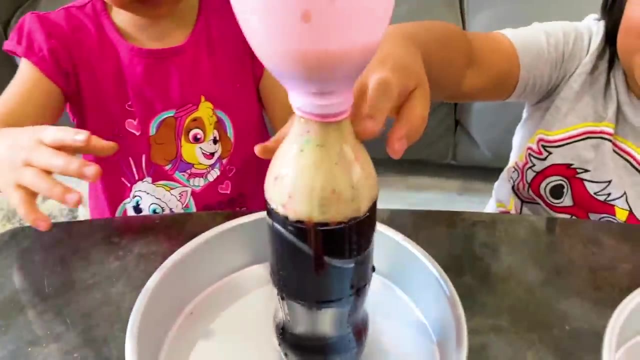 Ryan, Emma, yours is working. now. It's going down here. Oh no, it's going down here And these are going down here. Yeah, Wow, Oh, Emma, it's spilling, Oh, it's spilling. That's why we have a trick. 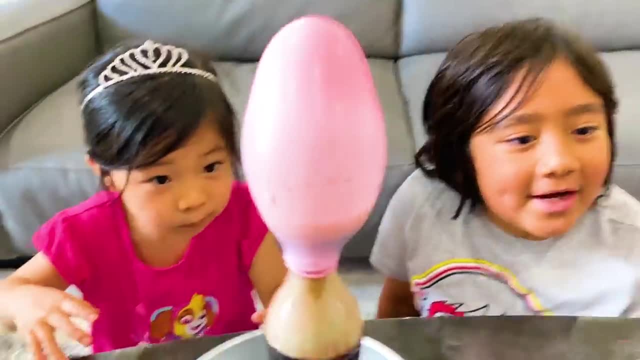 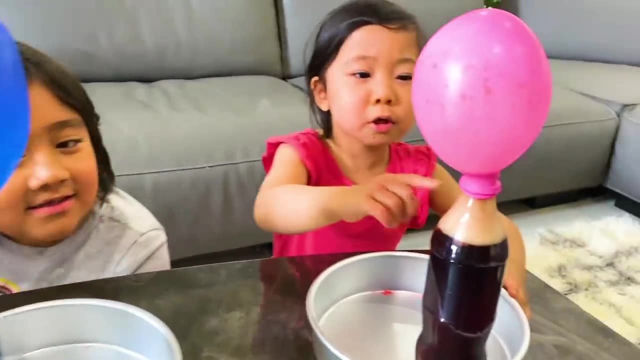 It's spilling a little bit, but it's okay. That's why we have a tray, you guys. I want to taste it. Okay, I want to taste it. I want to taste something else? Okay, when we're done, we can open it and you can taste it. 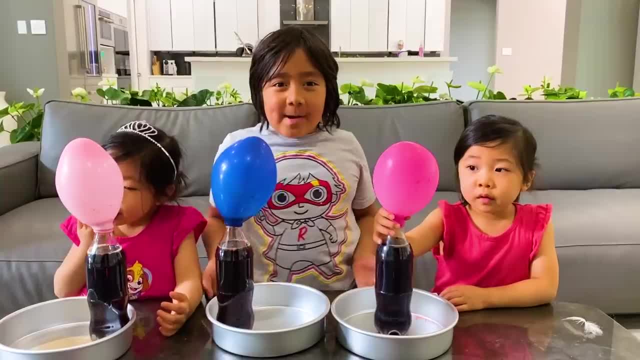 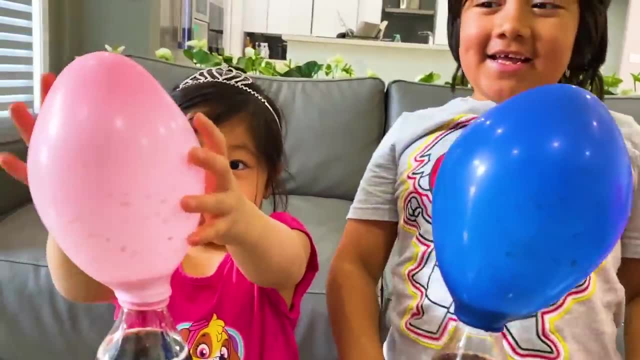 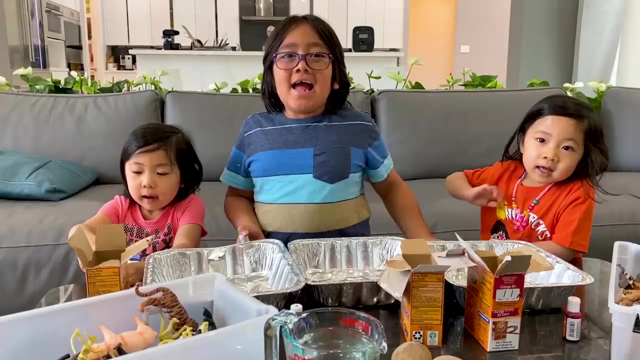 Okay, guys, Thank you for watching our video. Remember: always: stay happy and rise up. Bye, Rise up like a balloon. Yeah, Okay, Okay, High five, High five. Today we're doing a science experiment where we hide surprise toys. 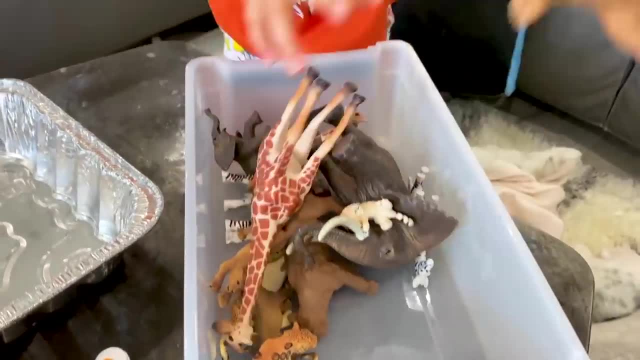 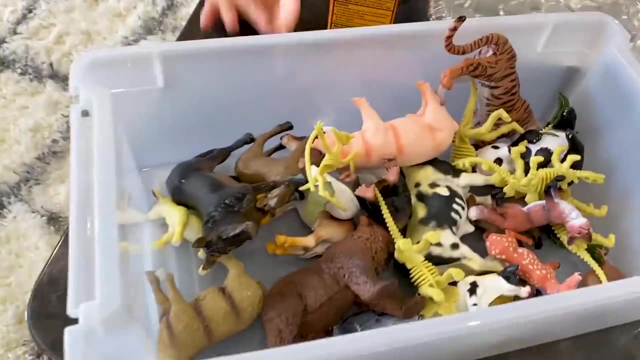 I want to go mom in the bath. Yeah, so we have all these leftover toys here. Scary, Scary Where we're going. Yeah, so we have all these surprise toys here We're going to hide First. we're going to put in baking soda. 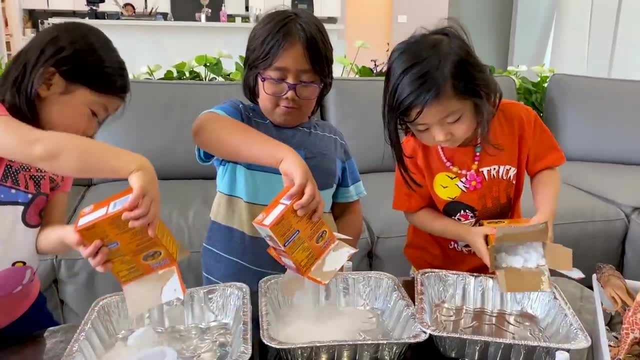 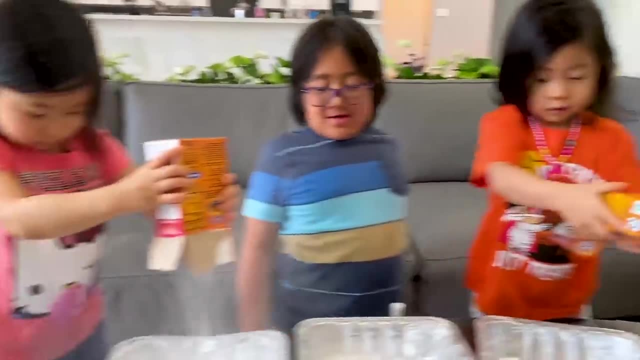 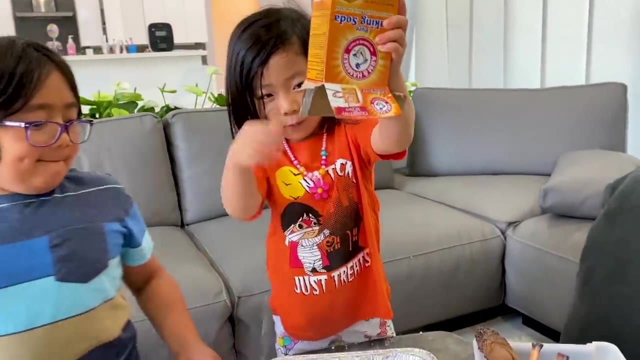 All of them, All of them, The whole thing, The whole thing. yeah, Wow, Do you have a lot? Yes, Emma, Wow, Does it look like we'll be cosplaying? Yeah, It looks like snow. Looks like snow. 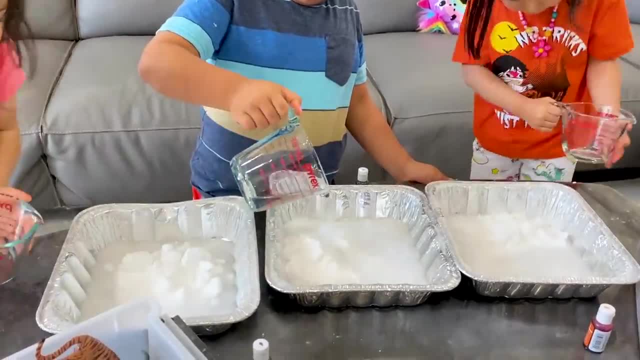 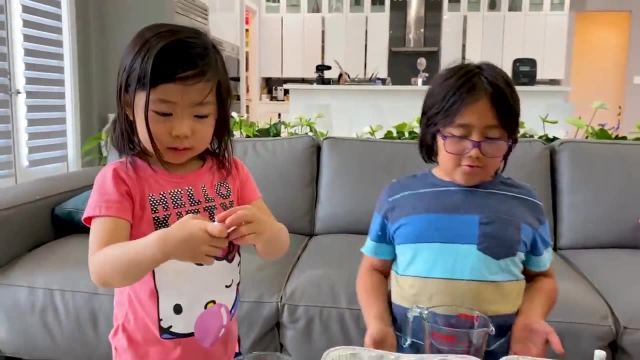 Next, let's add in water. All of it, All of it. yeah, Wow, Add the color. Yeah, that's right. Okay, so now we're going to add color. But don't forget, this is a science experiment. 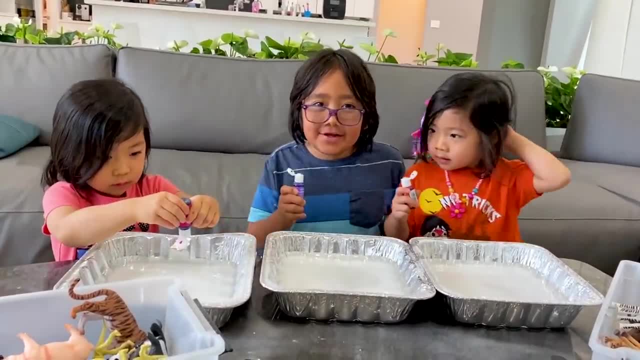 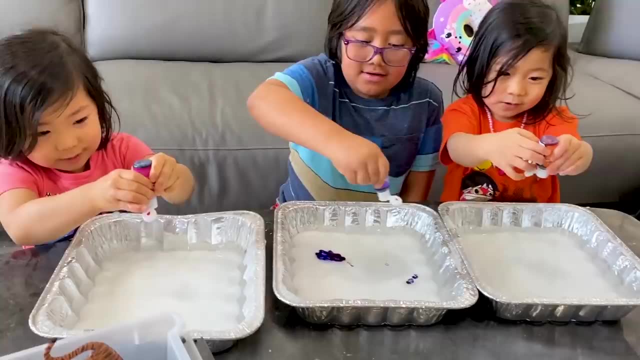 You guys cannot eat it right? Next, add food coloring, And I'm going to use purple, I'm going to use pink, I'm going to use pink Like a pig. I add one drop. Next up, let's add the paint. 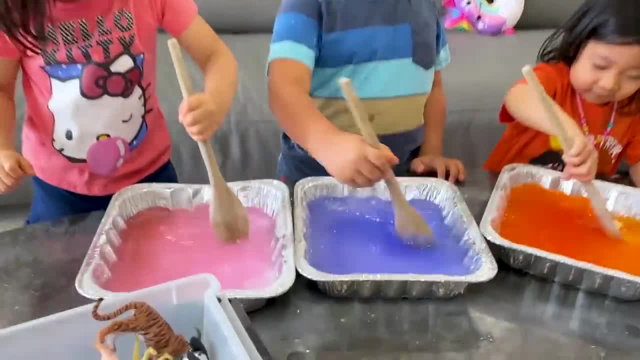 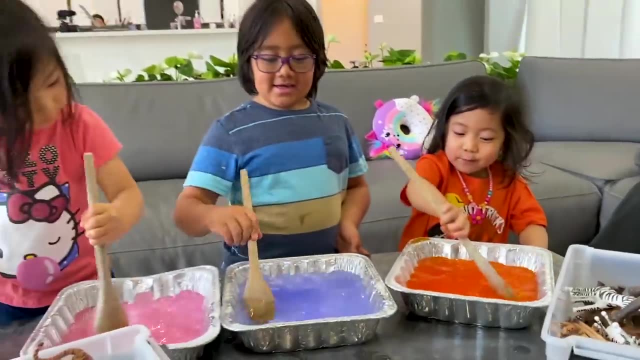 Add the paint. Mine looks like a piggy. That looks good. Mine looks bubbly like a piggy. Mine looks purpley. Mine looks bubbly. Mine looks purplier. Mine looks bubbly, bubbly, bubbly. 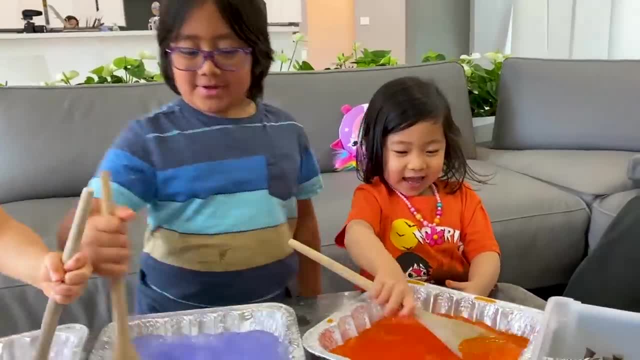 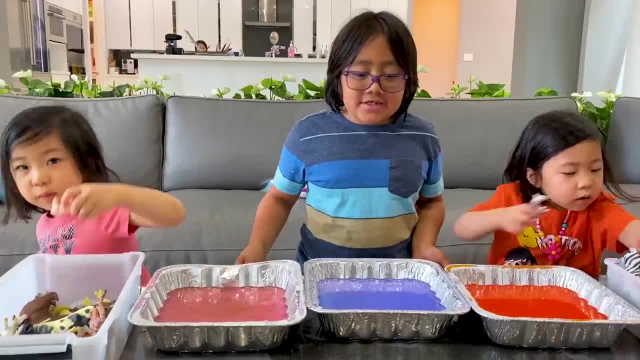 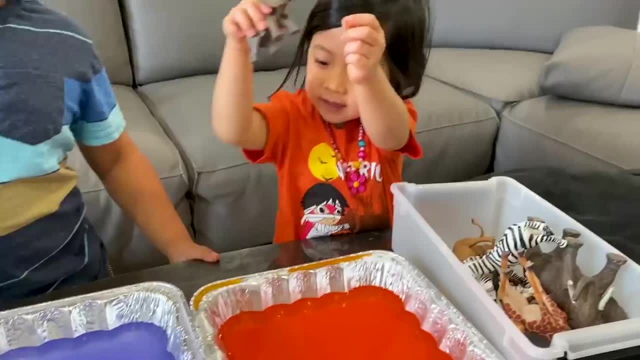 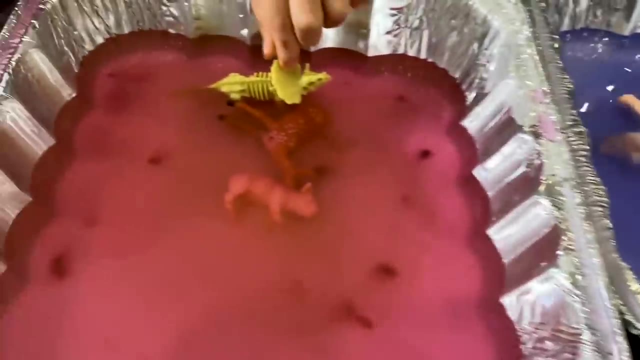 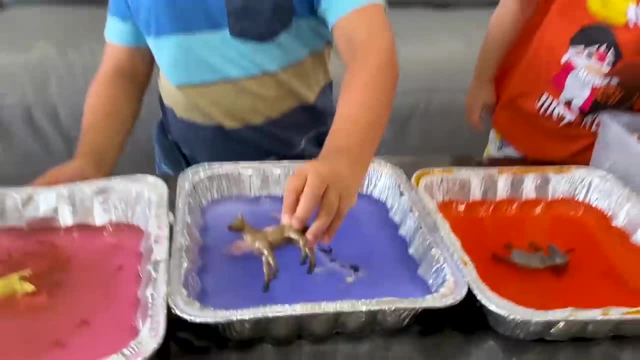 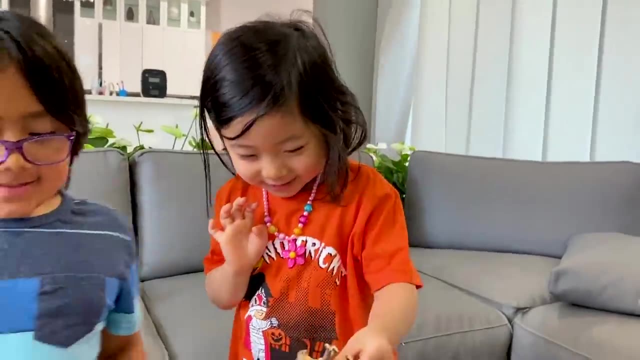 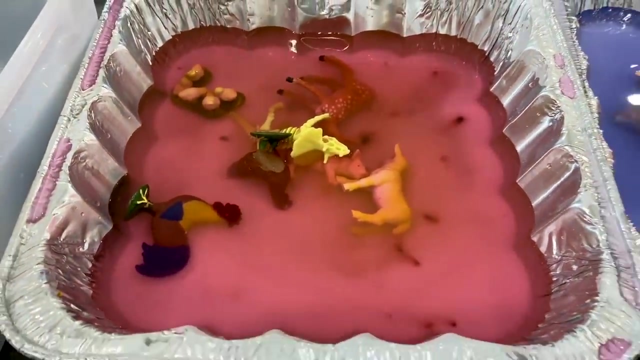 You can put it Triceratops, I'm putting in a horse, Or Okay, so just add in a couple. Wow, what about this one? Sure, Okayع, Whoa chicken, Whoa chicken. 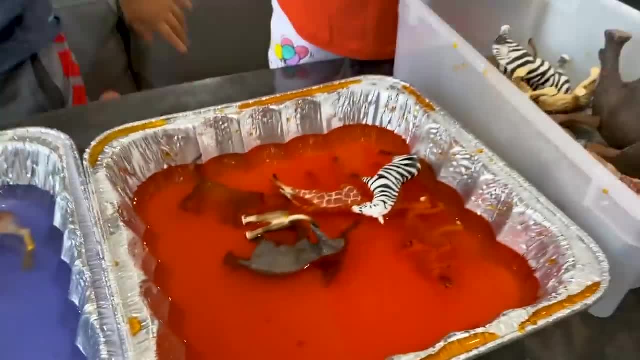 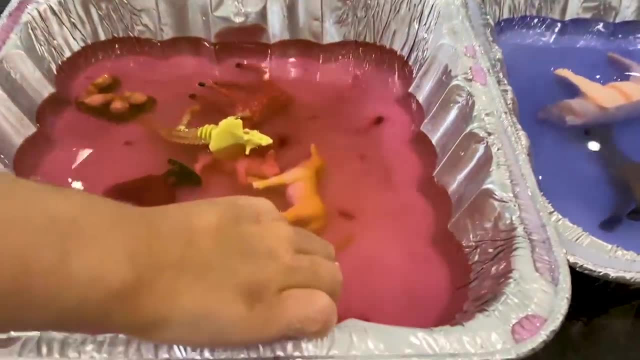 Are you guys done? Yeah, I'll just put one more. Okay, Emma, Just one more. Okay. Mommy's a bear, Mr Outer Bear. Oh, another dinosaur, Mommy, Mommy, Now let's put it in the freezer. 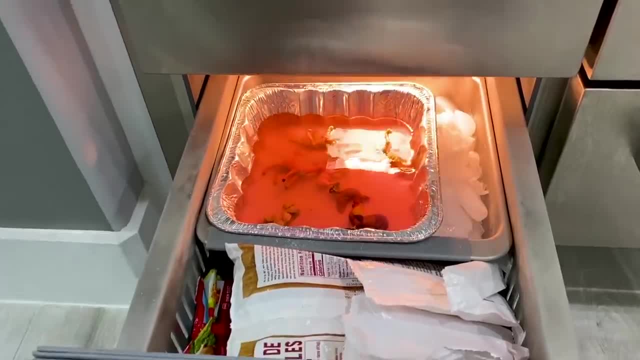 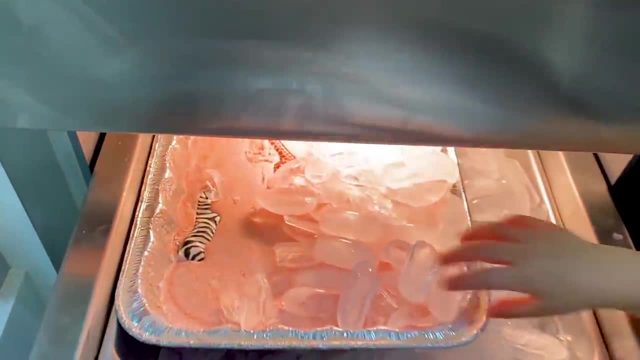 All right. so Mommy's going to do that Freezer time. Okay, we're going to freeze it. All right, I think it's ready. I'm going to see. Whoa, Wow, it looks cute. Oh, this one has ice on it. 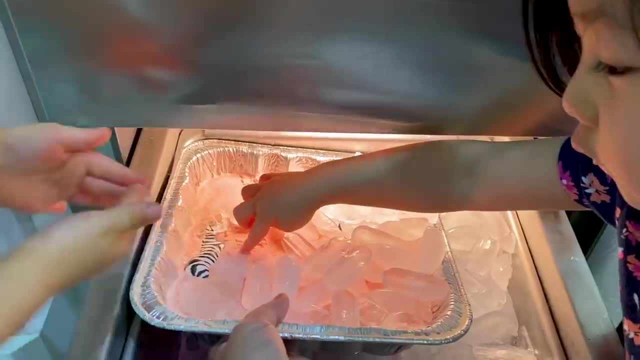 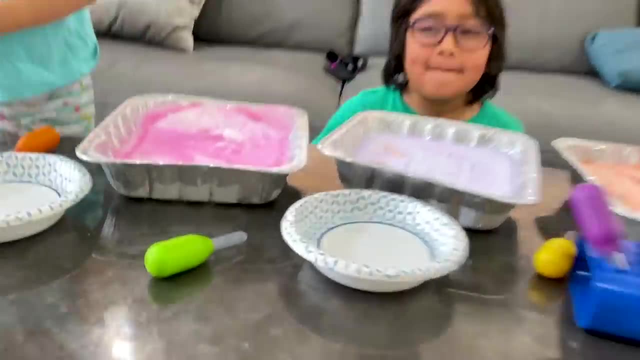 because I accidentally put it in the ice tray. Is it cake or hope, Ryan? I don't remember. All right, let's take it out, guys. Okay, guys, All right. so now that we got it out of the freezer, 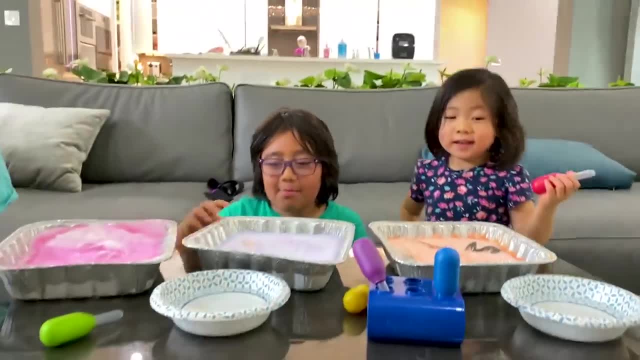 that's what it looks like. Some of them have ice in it, but it's okay. Oh, Ryan, did Ryan put high with his hand there? So now these are vinegar. So what you're going to do is you're going to put vinegar. 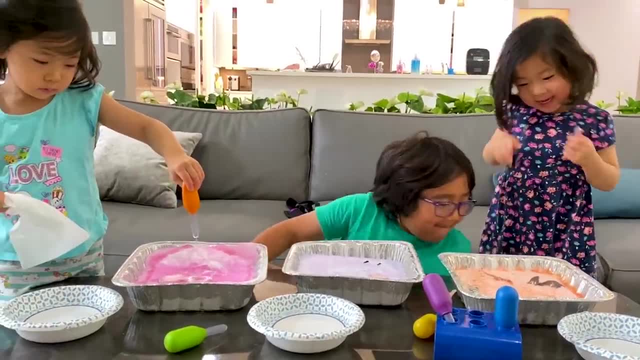 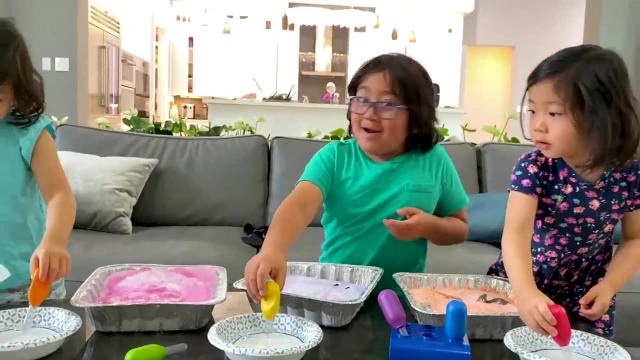 into your baking soda. I made ice, Oh, so what we're trying to do is rescue the animals that we put in there. Rescue the animals. Yes, that's the goal: Rescue the animals. So why do we put the animals there? 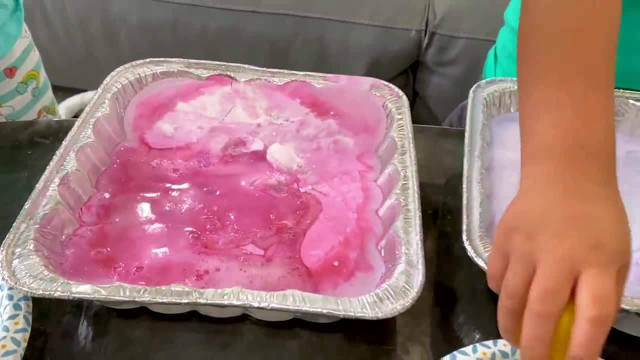 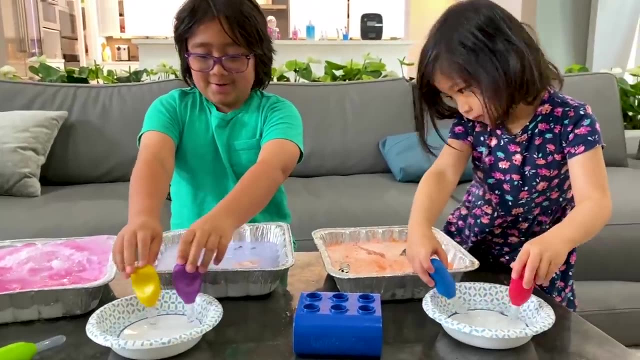 They're having a fun bath. I'm trying to get this one animal. What was that? Did y'all see it? I don't know what it is. It looks like a pig or something. Now it's Kevin. Oh, I didn't even bump into that. 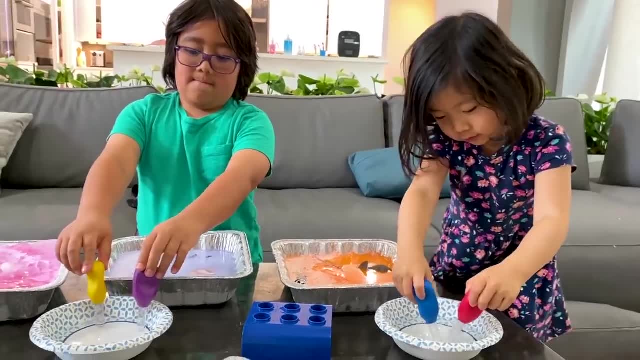 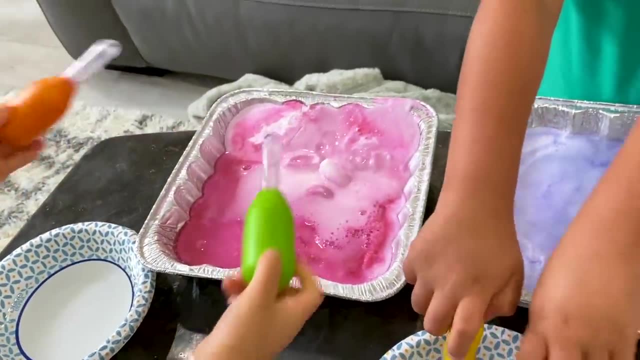 That was a lie. I had enough of that. I had enough, I know. Good job, Kay. We're going to save the animals. Yeah, save the animals. And why are they having a bath? They're having a bath, yeah. 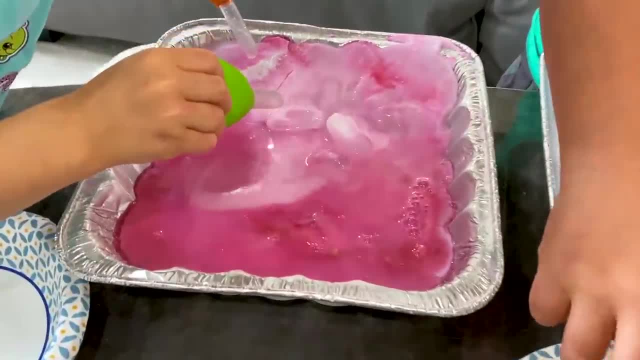 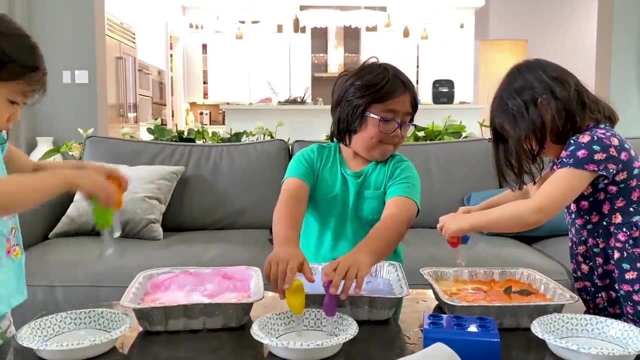 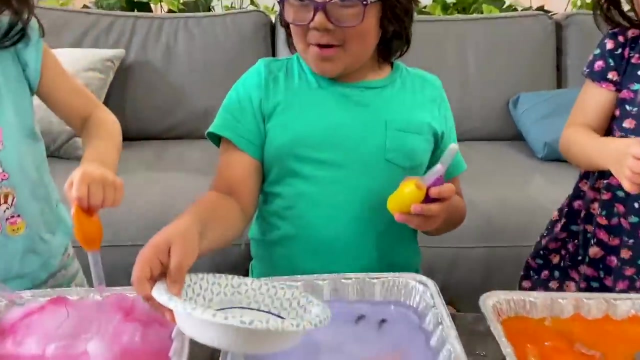 Why, Whoa, What. Everybody helping each other. How nice Looks good, Emma. Yeah, I'm going to put the whole thing in because it's not going that fast. Me too. Whoa, You want to do that too? 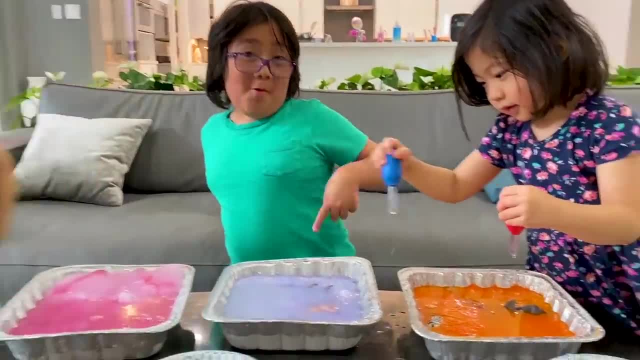 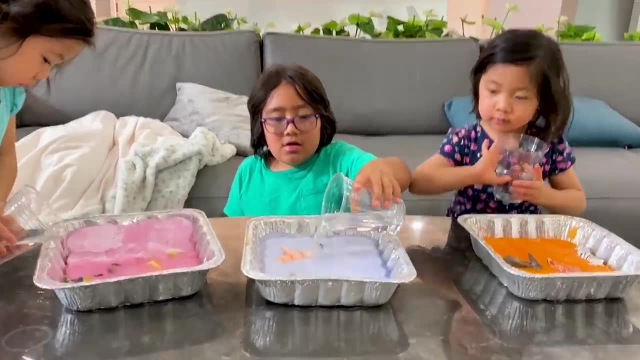 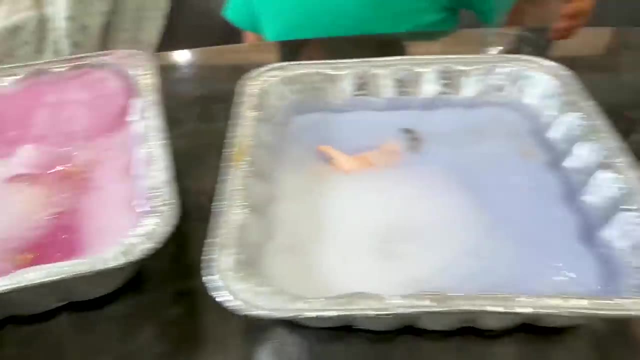 Not yet. Okay, We need way more. Yeah, Emma, All right, so now I'm just going to give them a cup of vinegar. Whoa, look at the bubbles. Look at the bubbles. Yeah, It's bubbling. 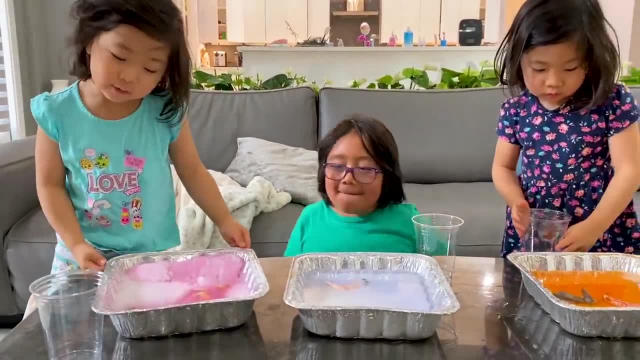 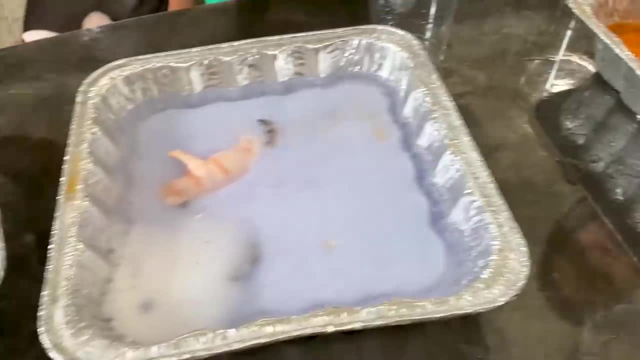 Yeah, Can we save the animals. Yeah, Can we save the animals? I don't want that animal. Oh, Oh, Almost, Can you take it out? Let's see if Emma can take it out. Almost, I cannot. Ryan. 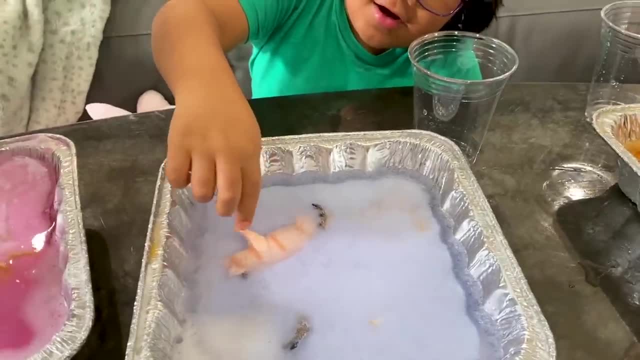 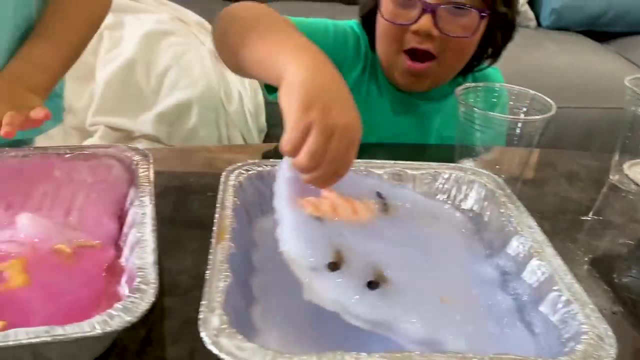 Not yet. Whoa, So close. Oh, look The animal's on the other side. Okay, guys, We are so close. We're going to try one more. We're going to try one more, One more, One more. 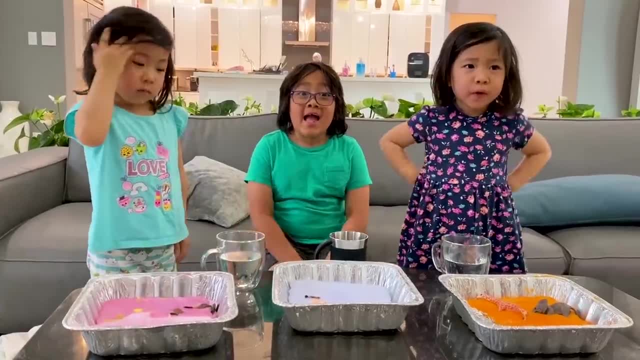 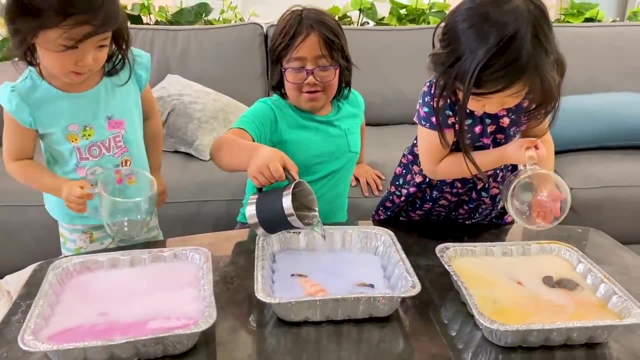 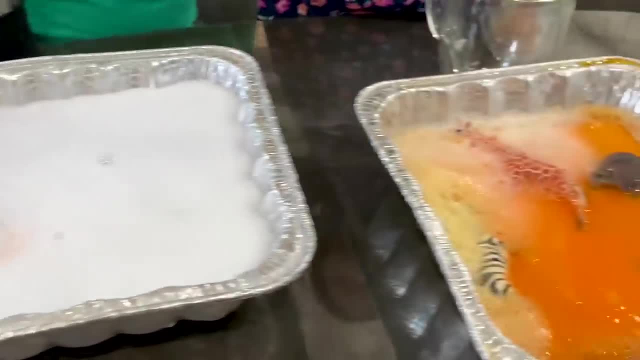 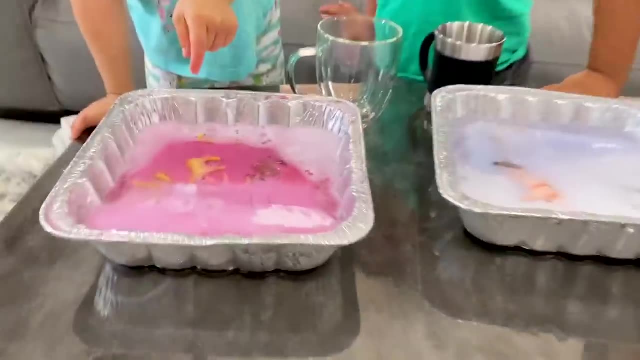 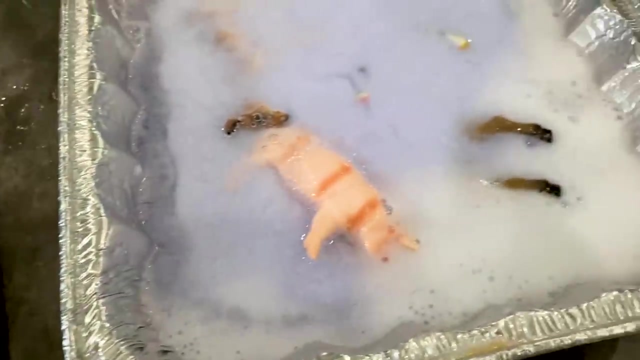 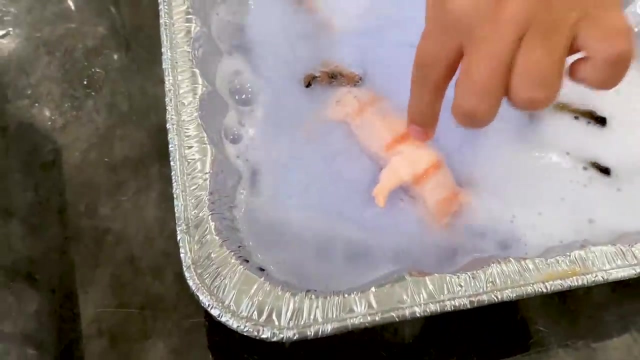 This is a fun video because the kids can help each other figure out how to rescue the animals. Mommy, It's almost getting out. Yeah, almost So close. You can see. You can see the animals here. I'm going to get mine down. 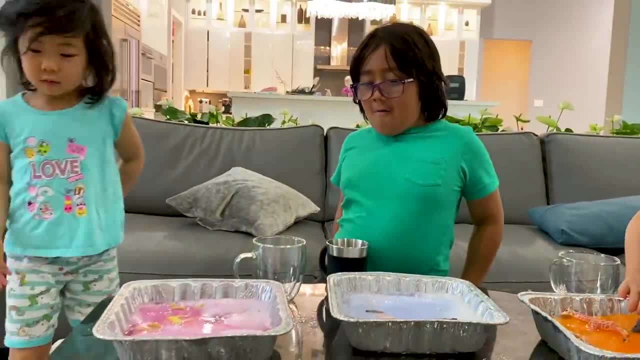 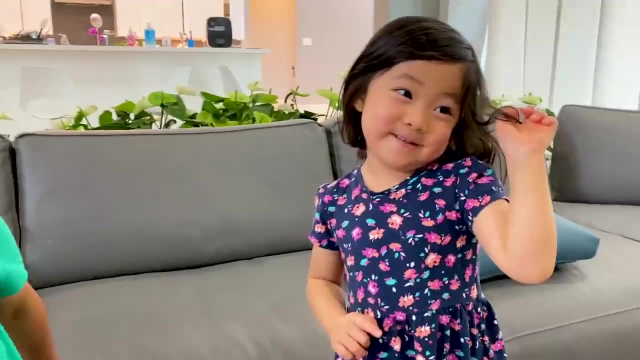 I know That's the point. We've got to figure out how can we rescue the animals. How about we do a hammer Hammer? Good idea, All right, Not strong hammers for us? Yeah, not strong. Yeah, Good idea, Ryan. 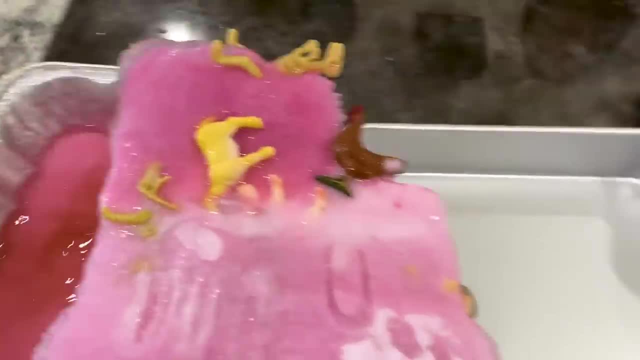 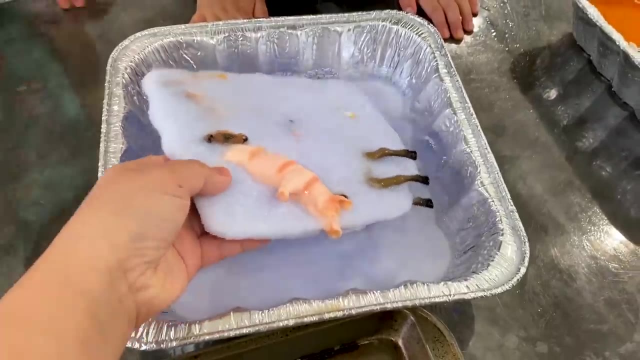 First, Mommy's going to help put it into a tray so you guys can break it up. Look, We got one. Yay, Good job. Okay, this is Ryan. I'm going to get out for him, And it's almost done. 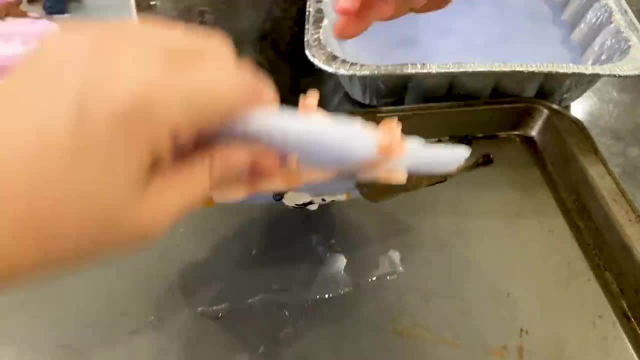 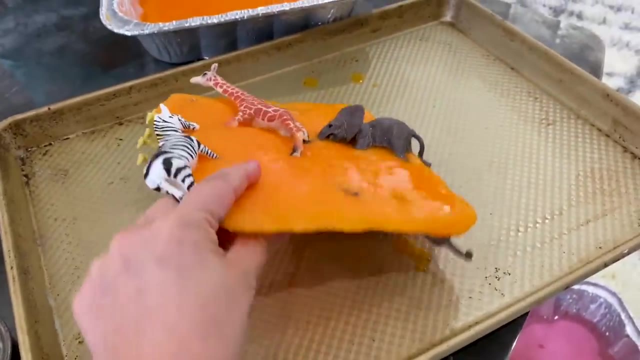 Look, Look at the back side. You guys can see what animals he picked out, And this is Emma. Really really close Her front and back side here. She also picked a dinosaur. We actually don't have a hammer, so I'm giving him a spoon. 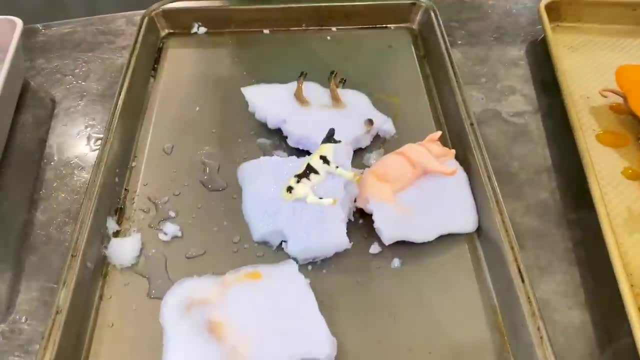 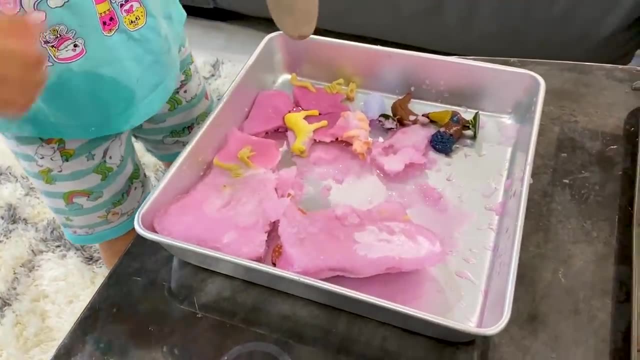 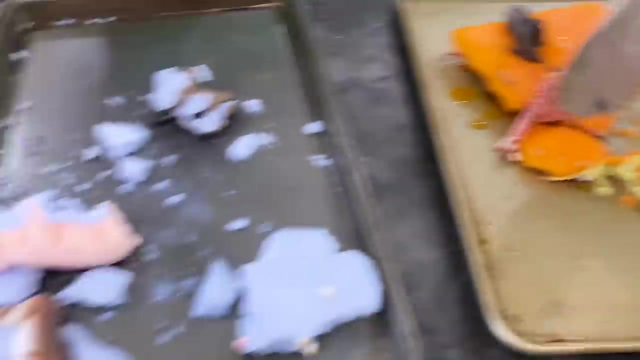 Well, Ryan, good job. Whoa, Whoa. okay, This is a very messy experiment. I think I got this: Wow, you rescued a zebra. I'm going to rescue the pig. Is this really rescuing? What about you, Kay? 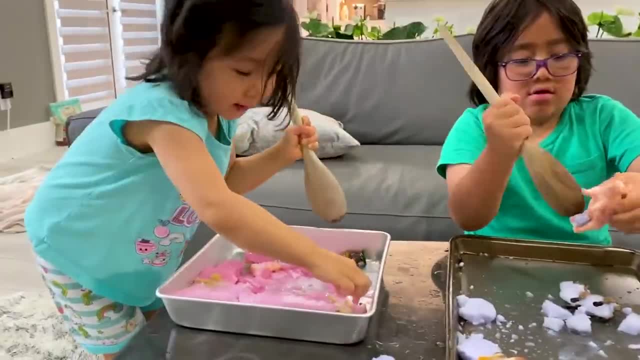 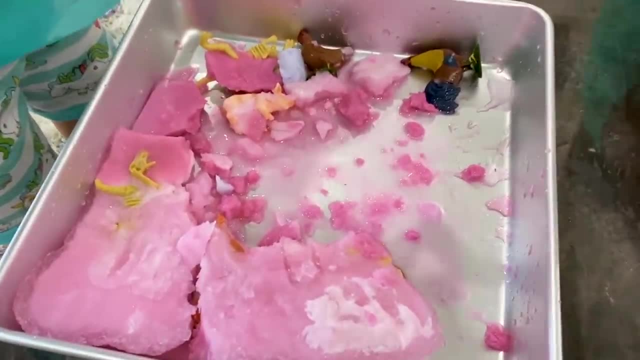 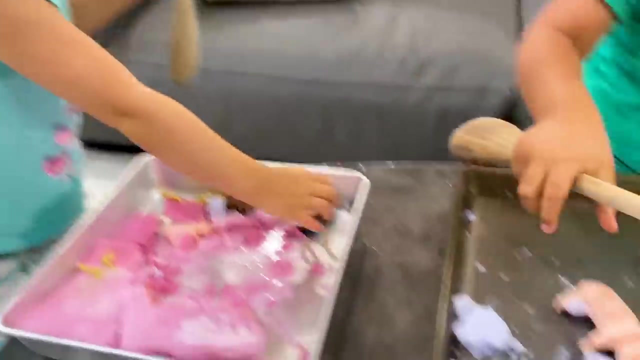 I rescued a dinosaur, You did. Did you rescue anybody Me? Wow, almost done. Whoa, baby giraffe. Good job, Mommy. look, Look, I got the pig. You did. Ryan, Nice, No, this has a little girl. 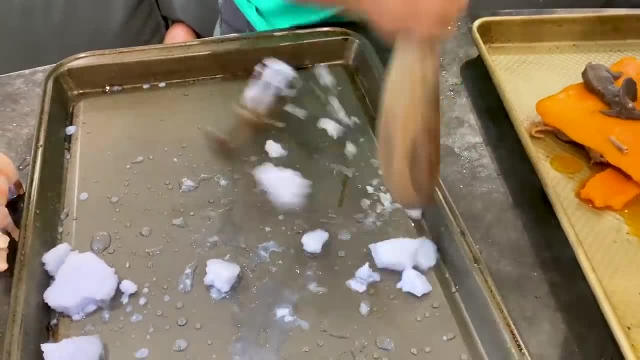 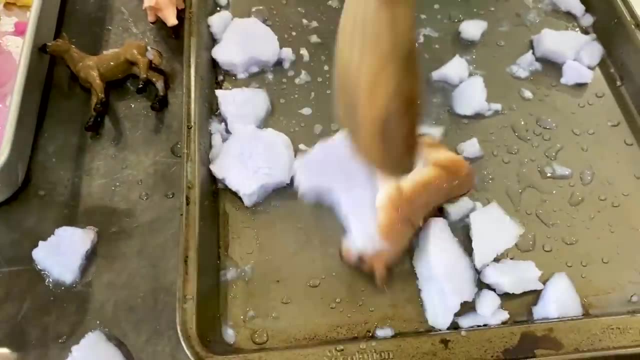 Just one more, That's okay. The horse, I got the baby tiger, I got the horse. Nice, Oh, one more. What is that? Is that a donkey? I forgot, That's a hyena, A hyena. 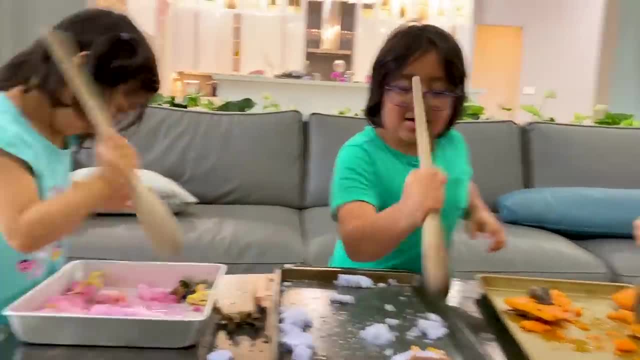 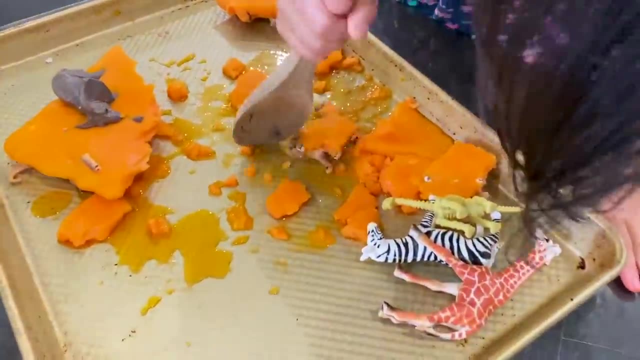 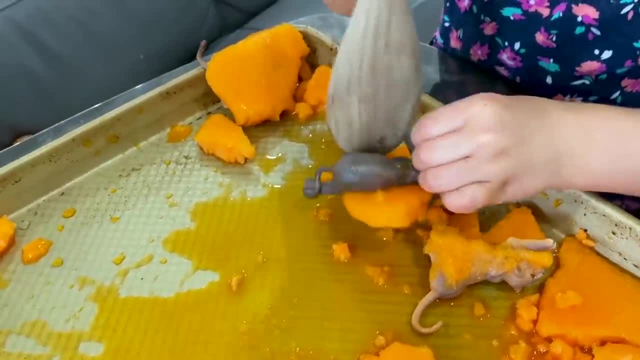 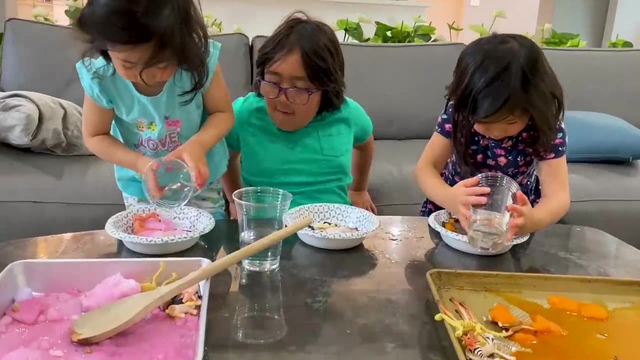 It is. it is a giant. Huh, What is that Elephant? It was the mommy elephant for the baby. Whoa, almost done, Okay, So we just have it. You just have a few more animals here to rescue. 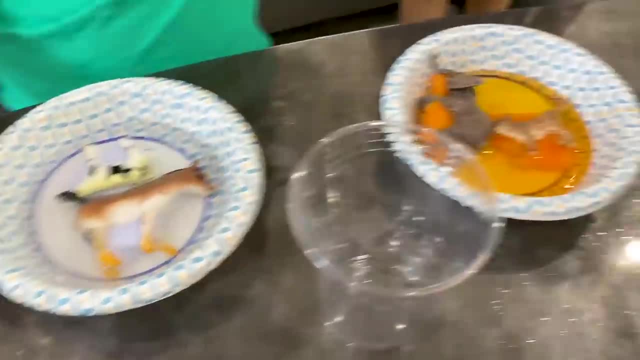 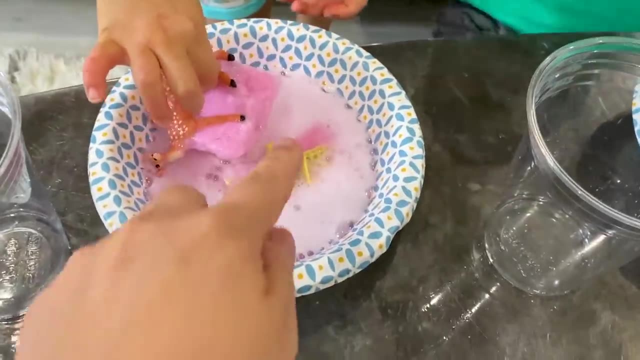 Uh-hm, Okay, Yeah, Probably get that big pig. Yeah, They rescued pretty much all the animals already, except for these. Yeah, Oh, look It's going. You see the bubbles? Yeah, I can see, Look, it's moving. 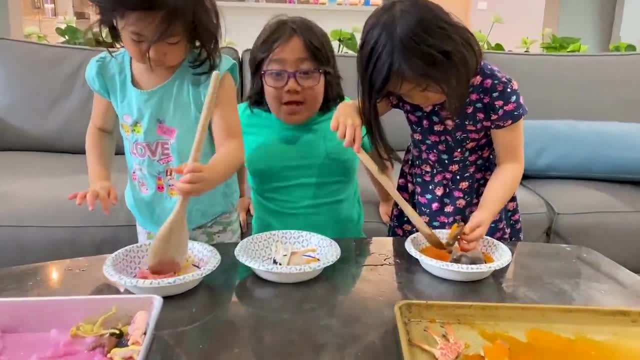 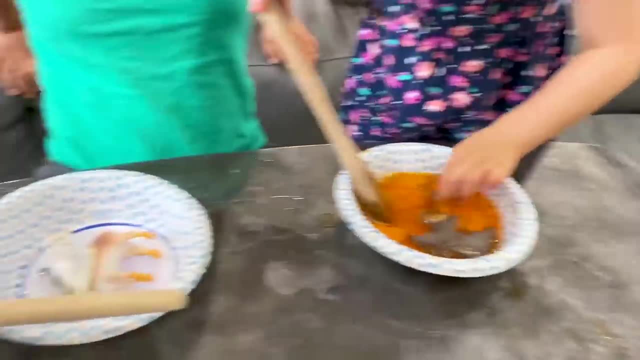 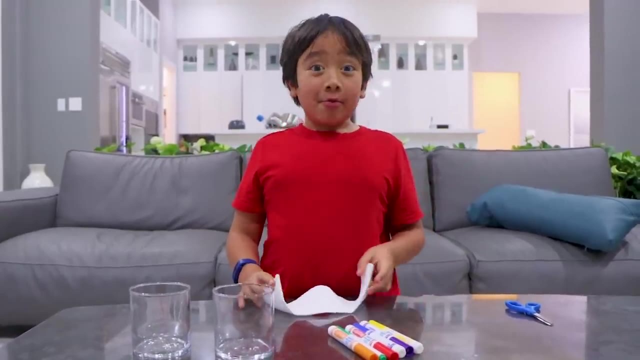 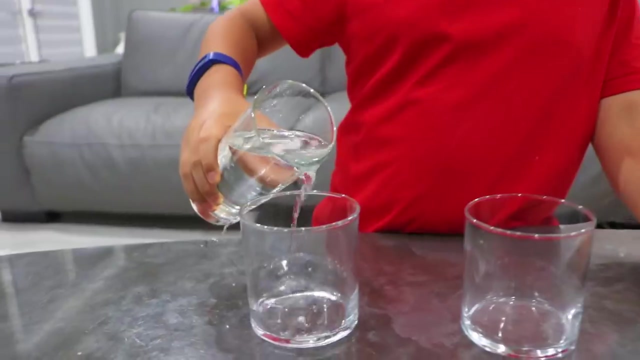 Okay, Look, we rescued all the rest of the animals. Look, it's out. So Emma's almost done with hers. Yeah, good job, Looks like soup. No, Guys, today we're going to grow our own rainbow. All you need is a paper towel, scissors, markers and cups with water. 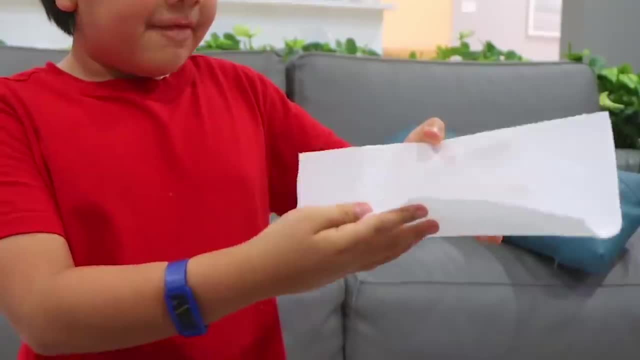 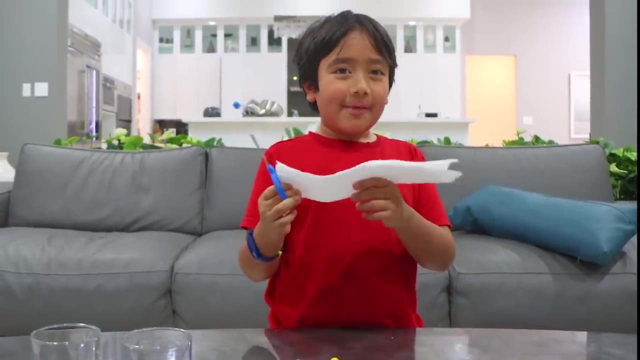 First, using your paper towel, you're going to fold it in half, and then we're going to cut a one-fourth. Don't forget to ask a grown-up for help, and I have Mommy here. Hi, Hi, Thanks. 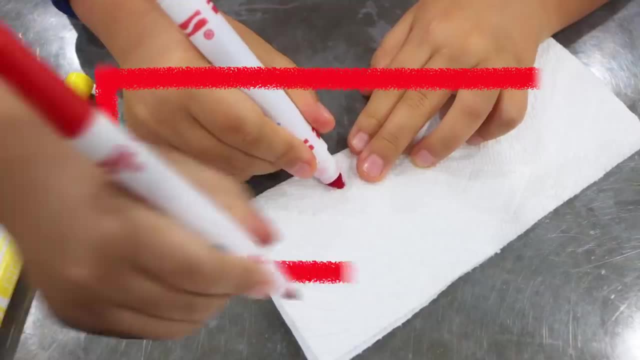 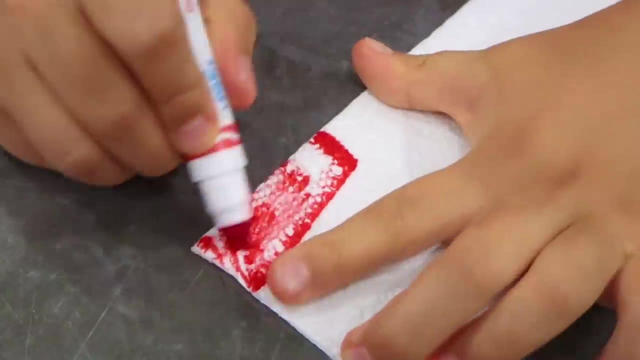 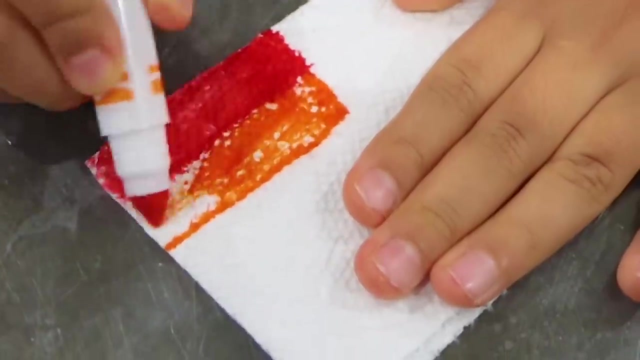 So first, with any marker you want, make a rectangle like this: Now let's color it in. The next color in the rainbow is orange. Put it like this: Now let's fill it in. Next is yellow. Okay, let's fill this in. 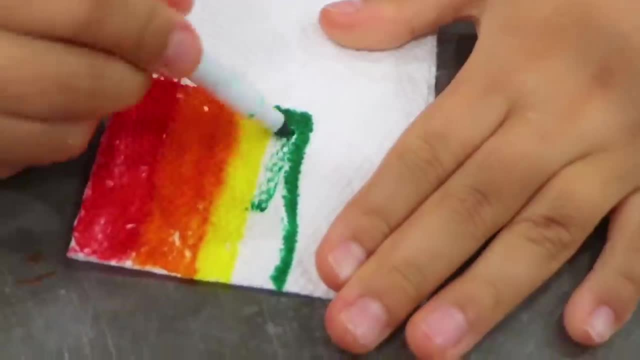 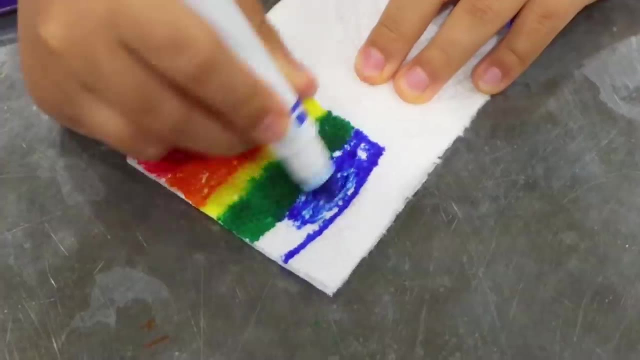 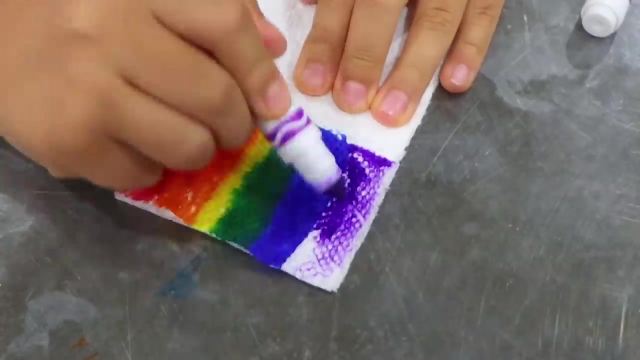 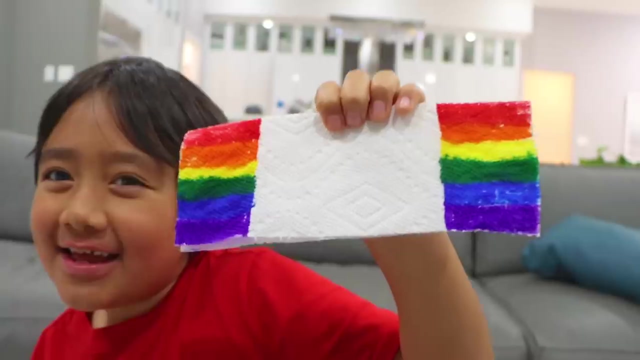 Next is green. Fill it in Green. Next up is blue. We're going to finish it off with my favorite color, purple. Now do the same thing to the other side, like this, See, Like. so Next, fill up your two thingies of water. 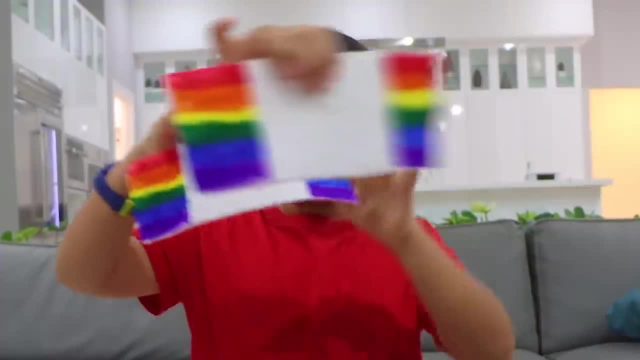 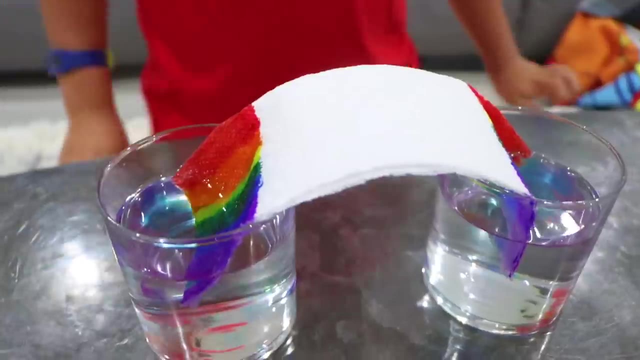 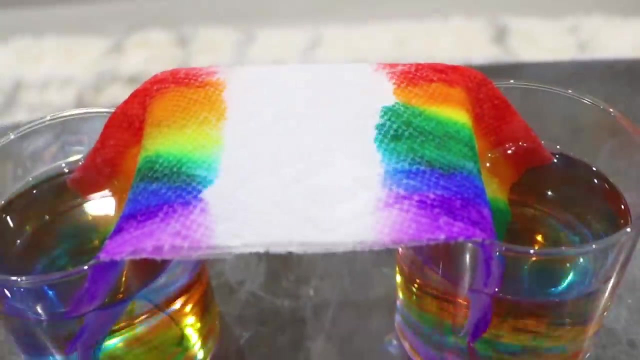 And the second one. Now take your rainbow paper that you drew and put half of both of the sides in the water. Now we wait. Watch the rainbow form. Look, it's already forming a little bit. Whoa, guys, did you see? 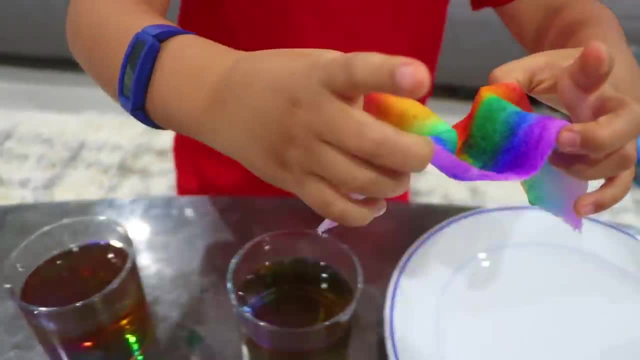 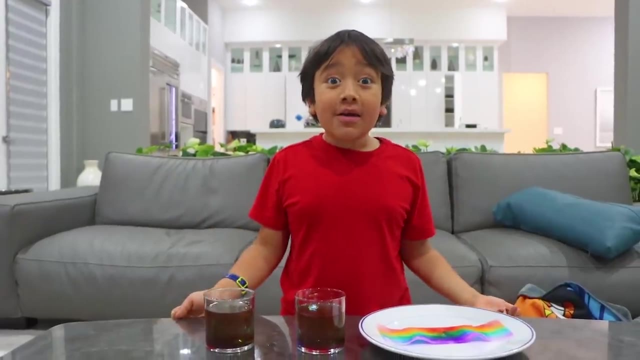 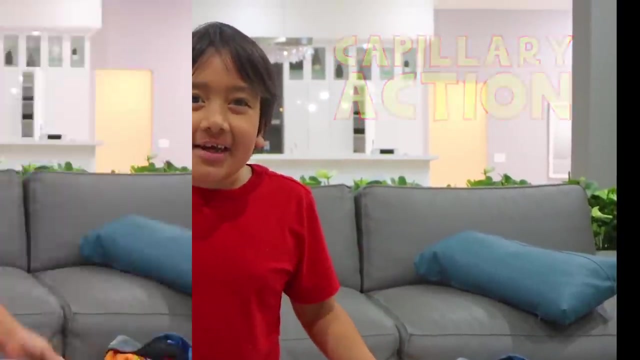 We made our own rainbow. Whoa, Let's put it right here. This is so cool. Did you see the marker die? move up the paper towel and touch each other, Because that's called capillary action. Did you know regular plants also use capillary action? 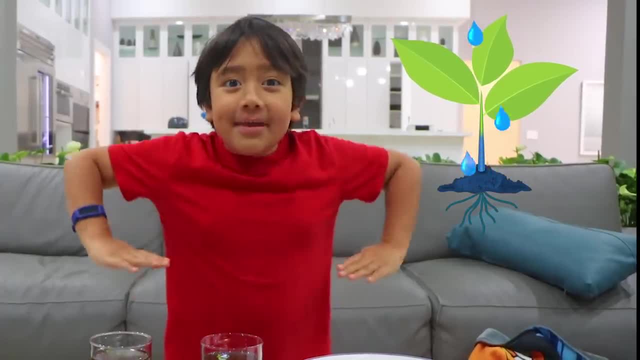 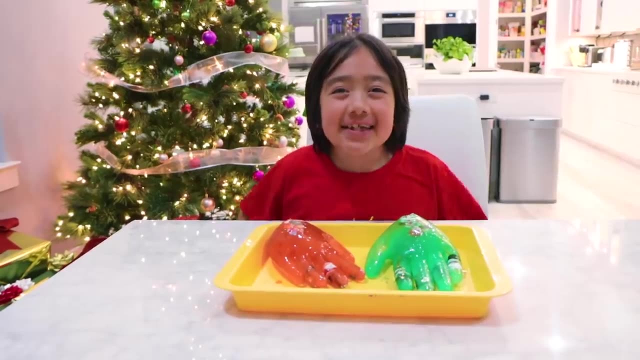 Because they bring the water from the roots and make it go all to the other parts of the plant. I hope you guys had fun making our own rainbow together. Hey guys, the holidays are coming up And you know what would be perfect. 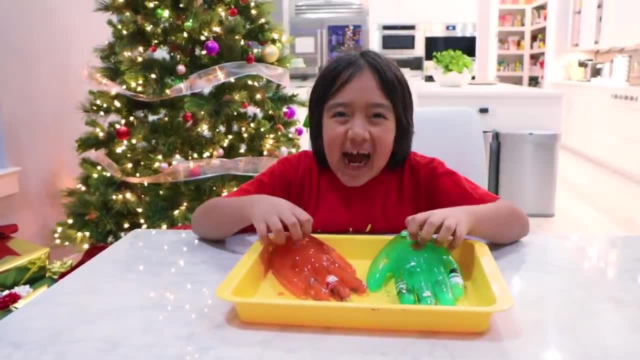 A science experiment with holiday ice hands. They're made out of ice and my job is to rescue them. Santa Claus is right here, But first here's how to make it yourself. Take it away, Mommy. Roll the clip. 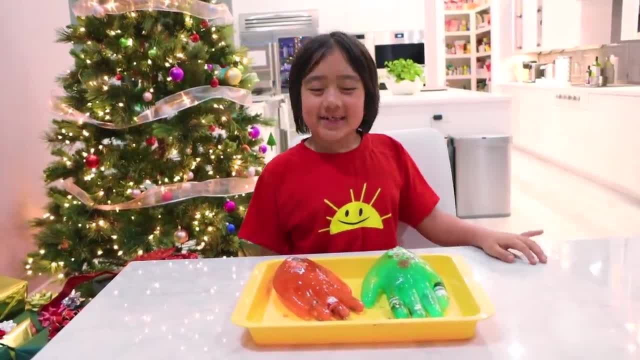 The first thing to do is gather all of your favorite holiday things. I also have some confetti and some sea quince, And you can add in some fun glitter. Next, grab a paper towel, And then you're done. And then you're done. 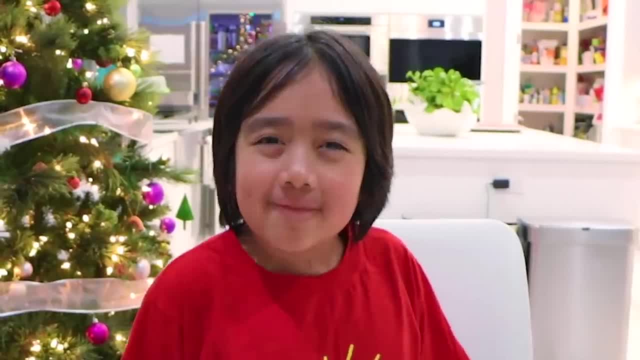 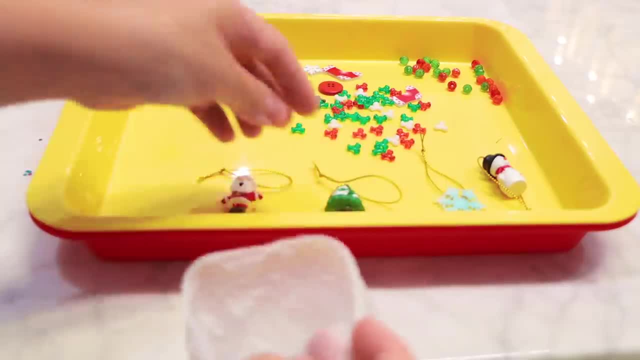 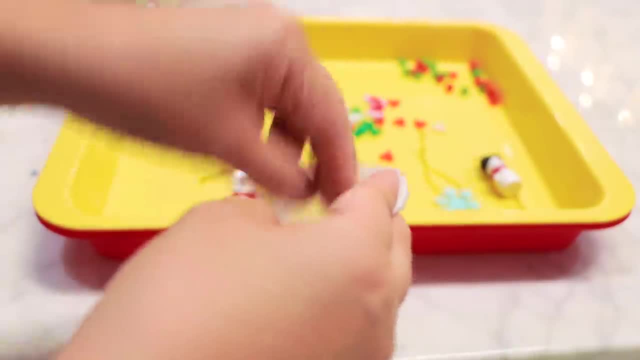 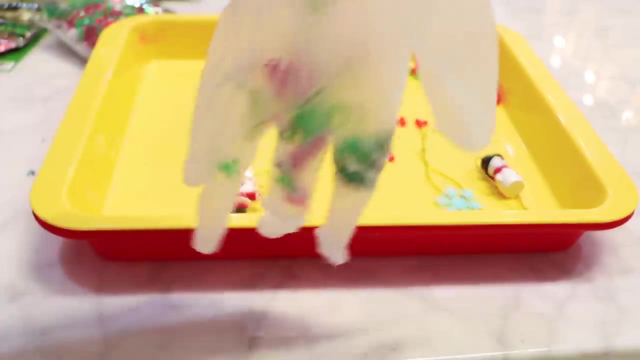 Here I'm going to put in a Christmas tree, some other fun things, A stocking, a little cute reindeer and some fun Christmas patterns. Just put it all in here, Little glitter. Then add in a few drops of food coloring. 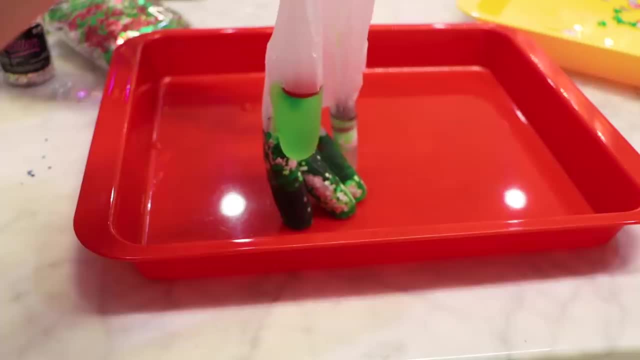 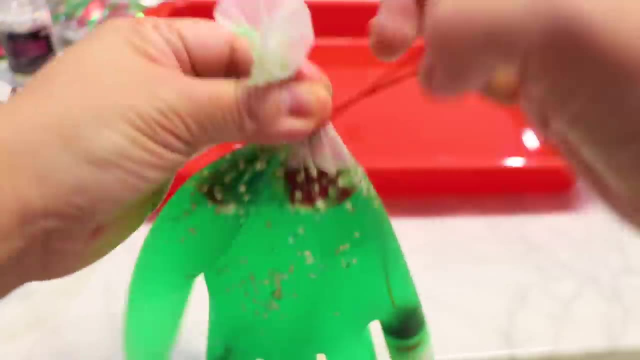 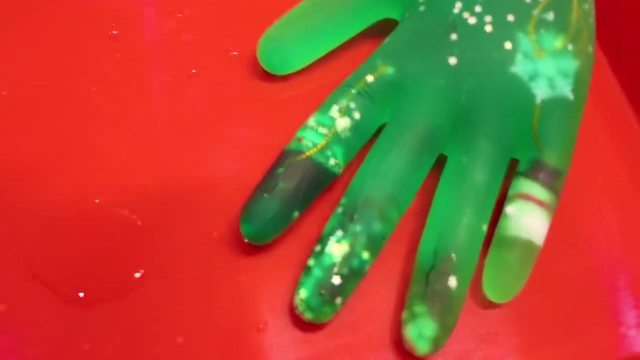 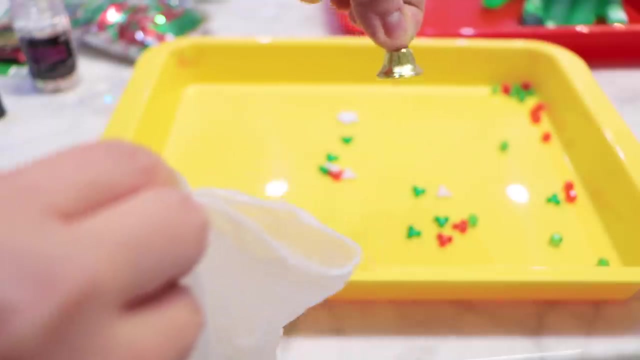 I'm going to use green. Drop it in there, Then fill the glove up with some water. Okay, fill it with water three-fourth way, and once you're done, tie it with a rubber band. and here's my first hand for a second glove. cute little bill into the club, some fun. 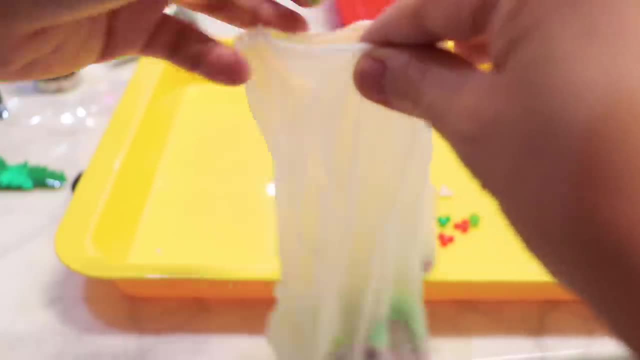 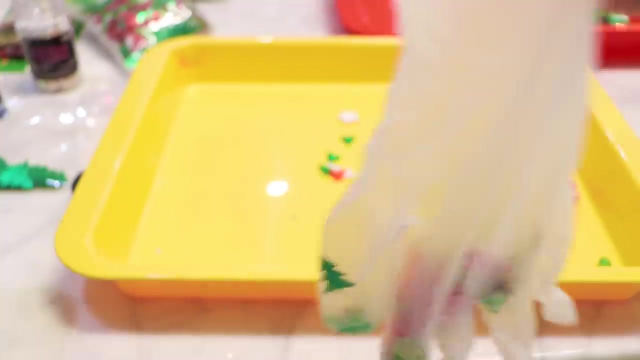 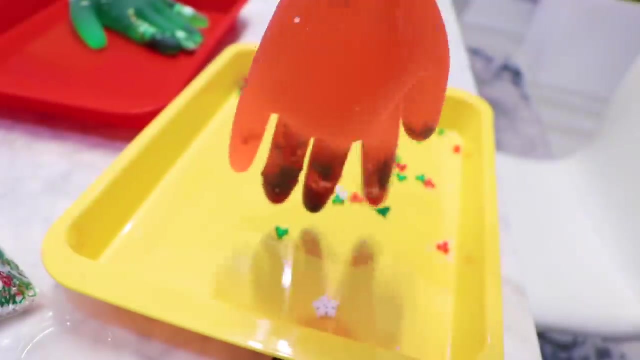 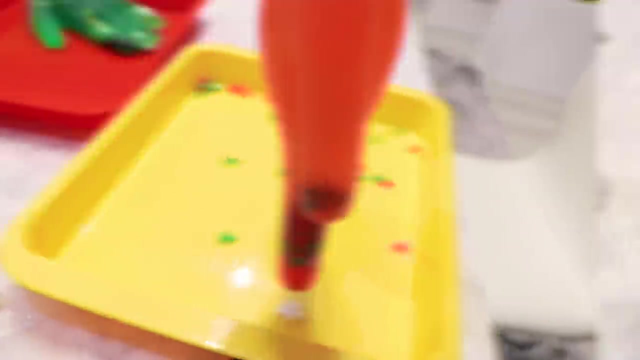 Christmas trees, some Christmas words. that's a fun glitter. who doesn't like glitter? and if you drop a red food coloring, then add water. once you're three-fourth done, tie it with a rubber band. okay, there's my red one. look, I see Santa Claus. you guys see it once you're done. 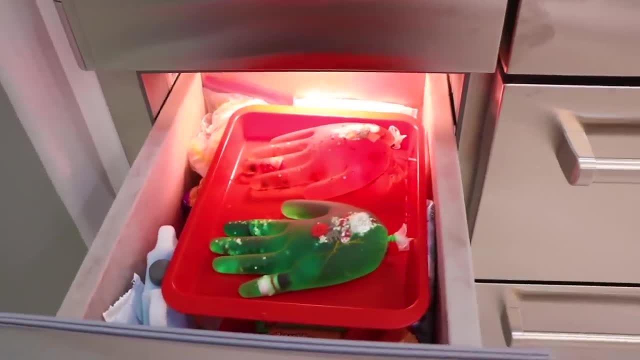 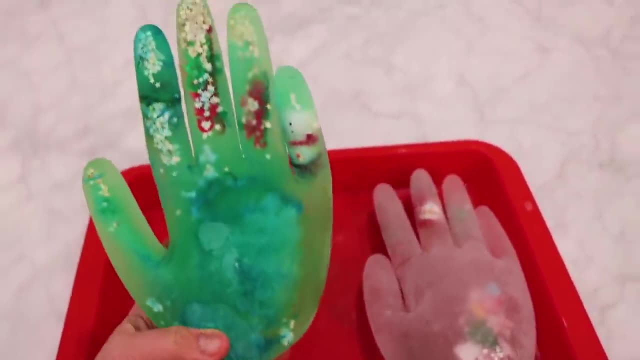 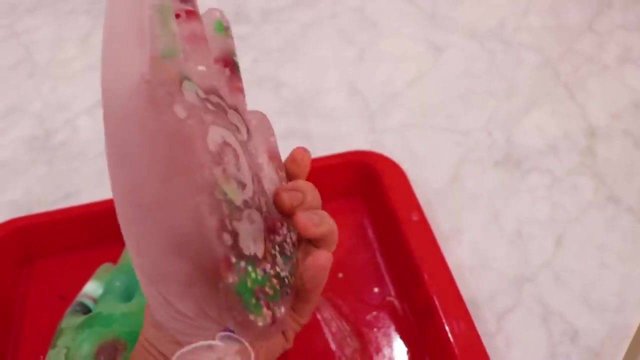 just put it in the freezer. there it is, I put in the freezer. I'm gonna keep it overnight. once it comes out here, it's all frozen. you guys see it. it's all frozen. you guys see it. it's all frozen. you guys see it. it's rock-solid hard. the red didn't stay very Well. I should add more red food coloring, but it. 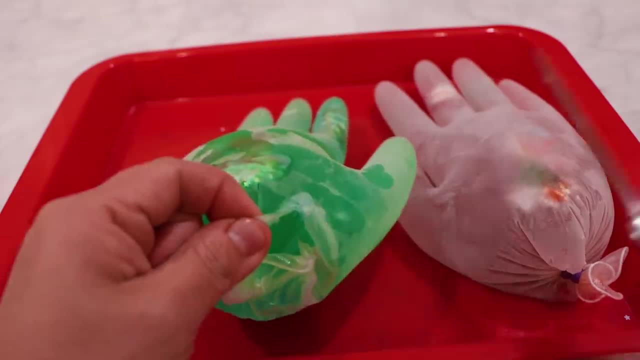 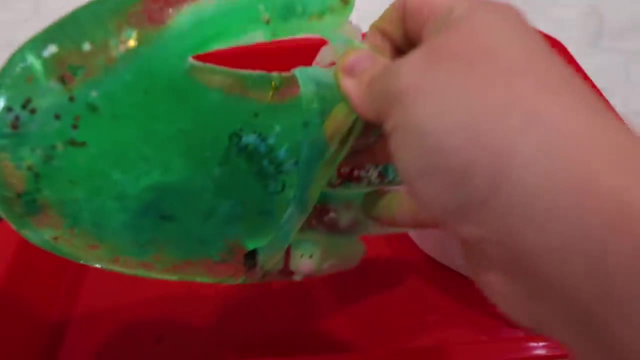 comes out pretty good. you guys seen in Santa right there. next, open up the rubber bands and then cut and joue very carefully at the fingers and thumb. once you're done, you'll be proud of your Santa and thumb once you're. Hey everyone, it's É Phil And will be using the new Santa Clausạo recipe. I had a lovely Christmas present for you today. remember to buy the gift right today at home, and if you do get your eSports version from the description, you will get the Fan agrade guarding your Santa Claus gift at an affordable price. I know that in the end of the day, Santa Claus will be doing all of these Christmas웁. Mantist responded to your questions in the comments, So feel free to send your little people. take your best wishes for this Christmas gift today. and how wonderful, Santa Claus, It was fun to be singing and other friends here. later I'm coming back to youVER ick. 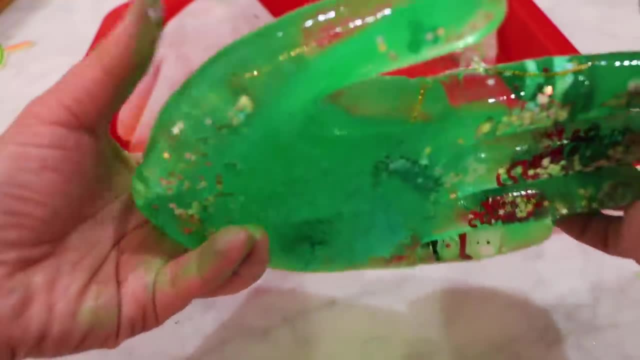 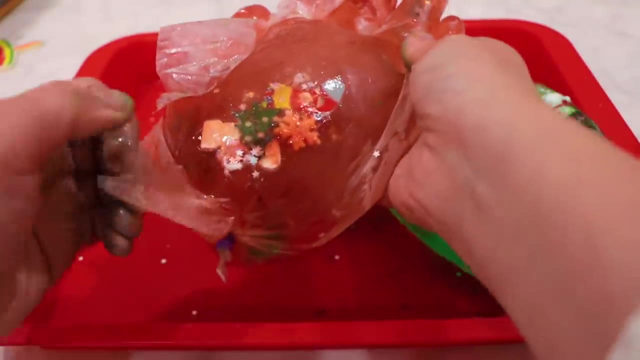 Once you're done, you'll have something like this: Isn't that cool? Look, be a snowman. Okay, here's the other one. Just pew and cut away. Look, there's Santa. Okay, and it looks like this: 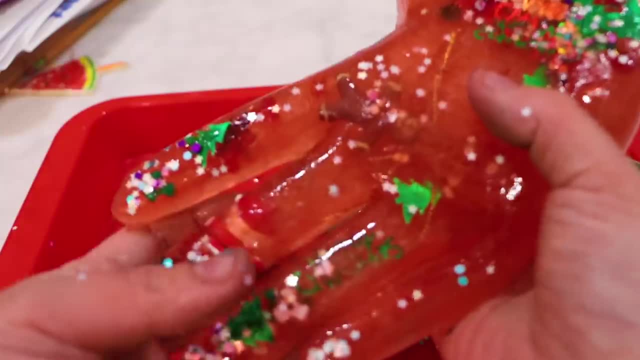 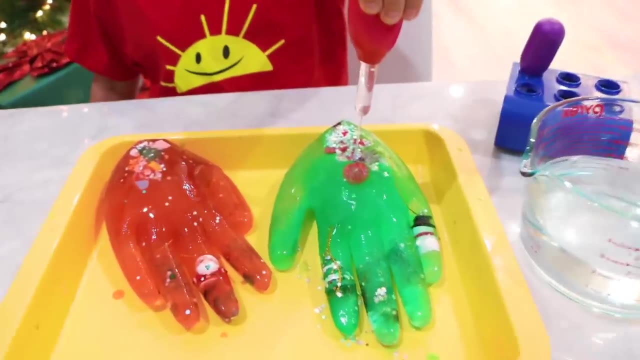 But guys, look, I broke off the thumb. Oh no, So okay, it's still fun. Look, there's Santa. Okay, let's get started. I'm going to try to melt it with some warm water, Mmm. 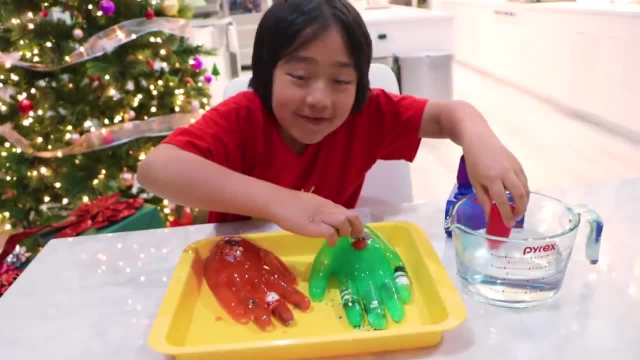 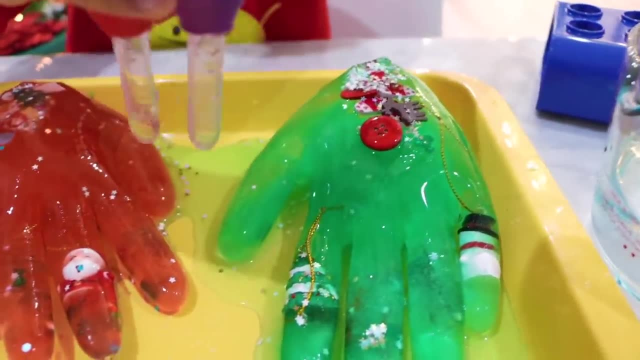 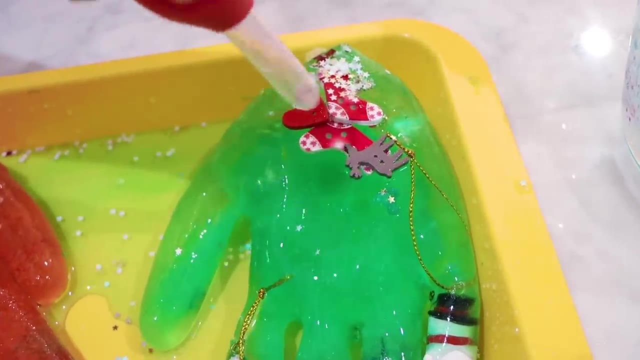 It's working a little bit. Wait, wait, I can feel the objects. It's working. Okay, Did I get the button out? I got the button out. There you go, And there, I think this time I'll be able to free something. 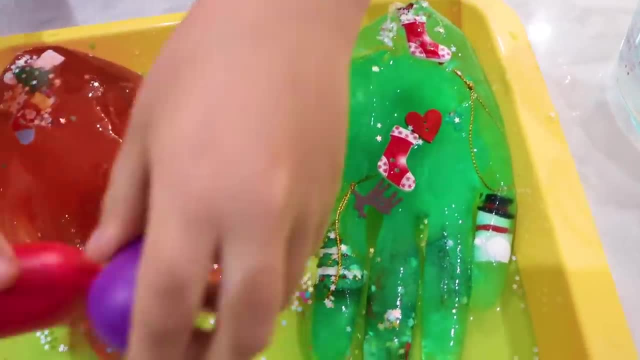 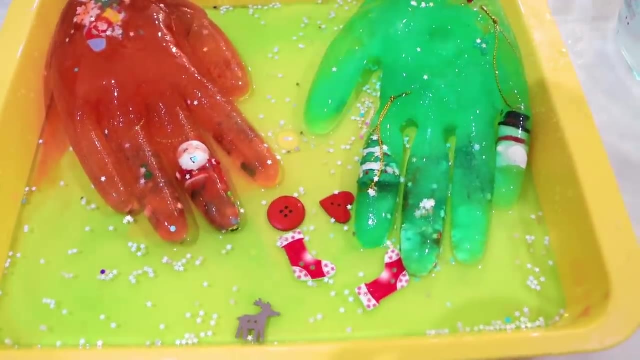 Oh wait, I freed socks And a heart, Heart, Heart And socks And a deer. Oh, and another sock. Don't worry, snowman, I'm coming for you. I think I have to put all the water in one spot. 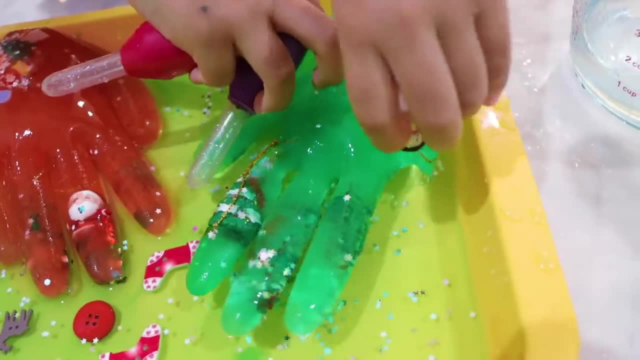 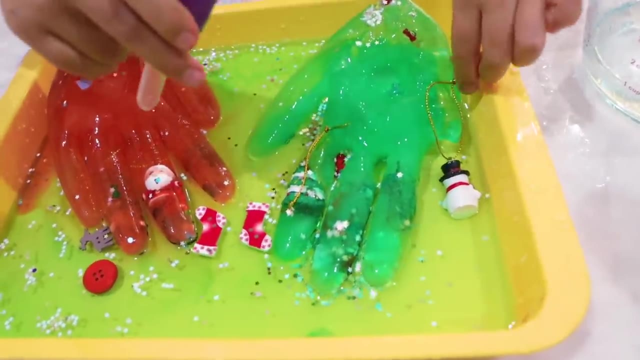 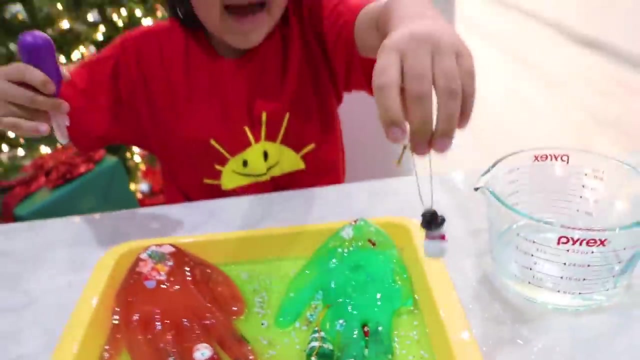 I think the snowman's out. Oh oh, no, there's a chain. I've got to get the chain out. Oh oh, oh, yeah, I think I got him out. Oh, oh, oh, Ah, got him out. 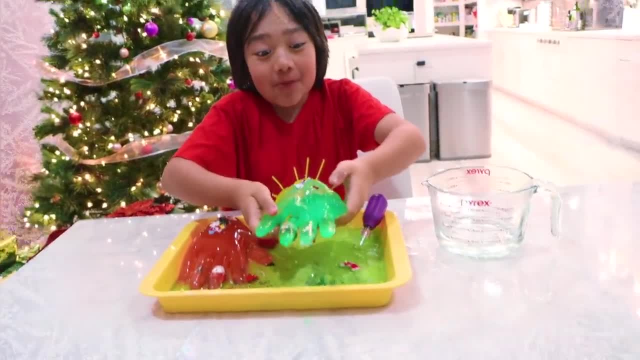 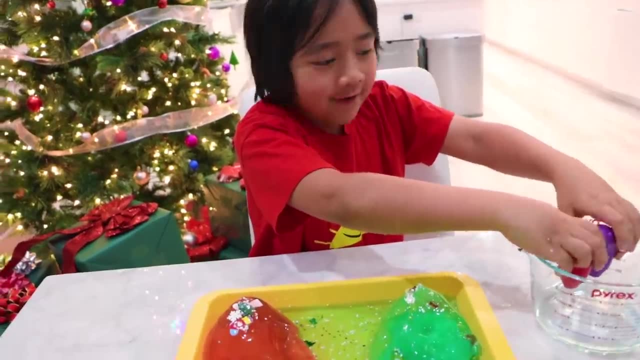 Yes, Okay, guys, I'm going to try to pick it up. Oh, it's super cold and it's missing a pinky. Ah, this one's also missing a thumb. Okay, Santa, I'm going to try to rescue you now. 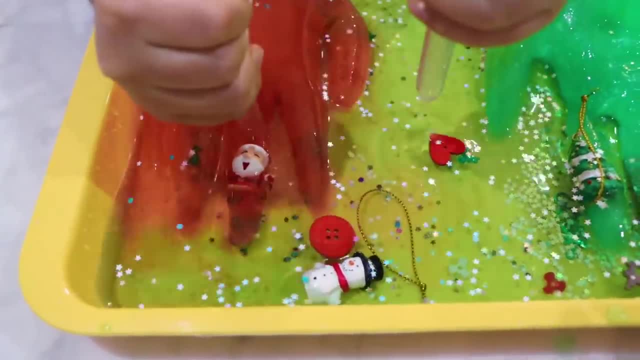 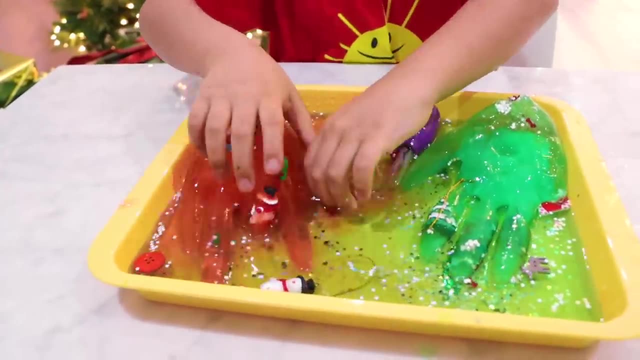 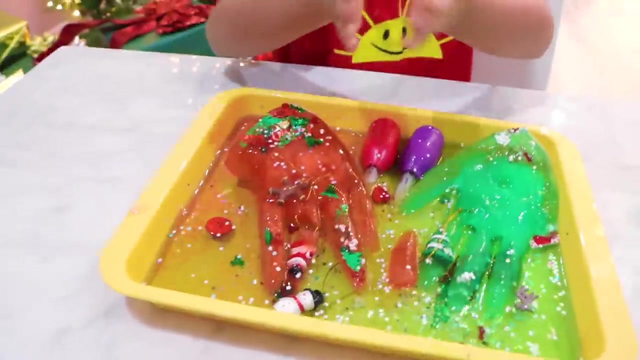 If I put all of the force right here. Oh, there's another golden chain. No, Where does the golden chain lead to, Guys, the chain is super long. It's all the way up to here. What do I do now? 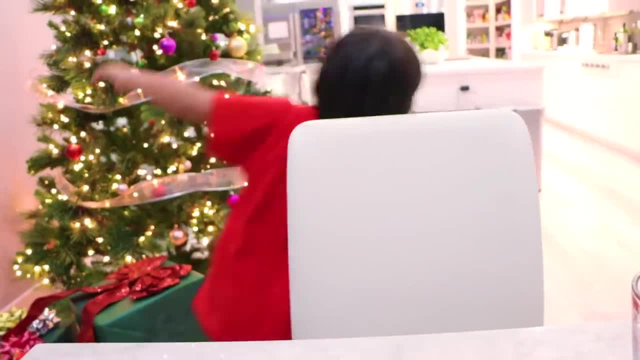 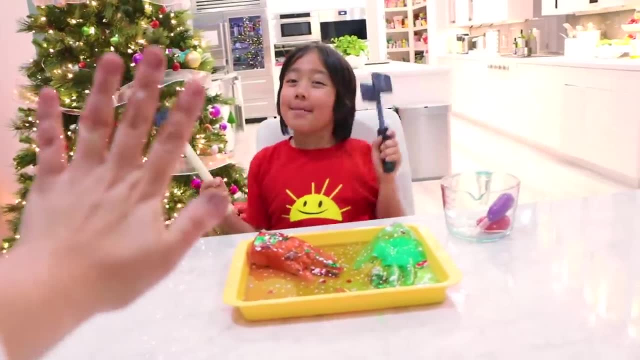 I have an idea. I'm going to go get a mallet, guys. Okay, guys, I got two of them, But remember to ask your parents for permission, because my mom said: yes, Right, Mommy, That's right. Okay, let's try this one first. 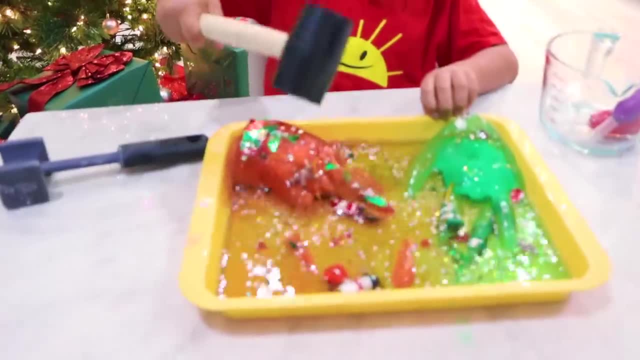 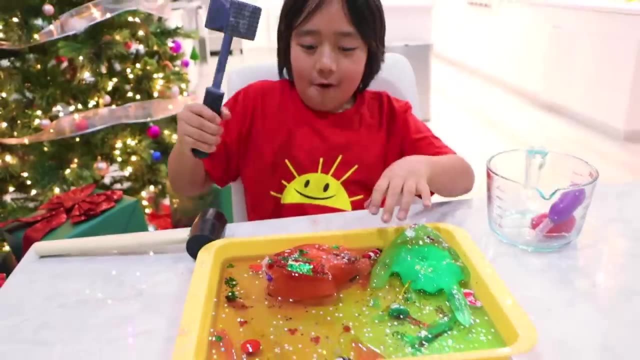 I think that one will be stronger. Whoa, it's working. it's working. Wait, Santa's out a little bit. Okay, maybe I should use this one now. Whoa, splash of a lot of water. What's breaking the ice? 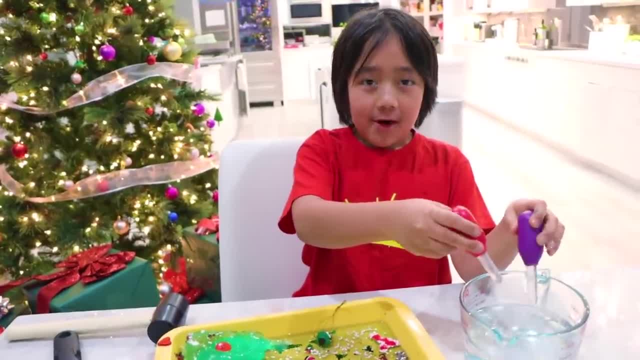 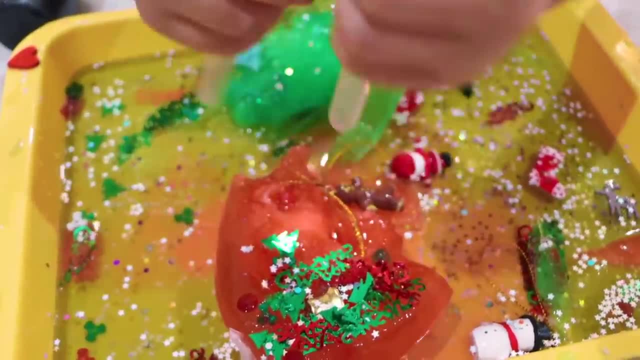 The ice is shattering. Okay, guys, I'm going to put some more warm water, And this time it's even hotter. Whee, I got the chain out, Chain out. I didn't get Santa. I got Santa, Wait, and I got the gingerbread man. 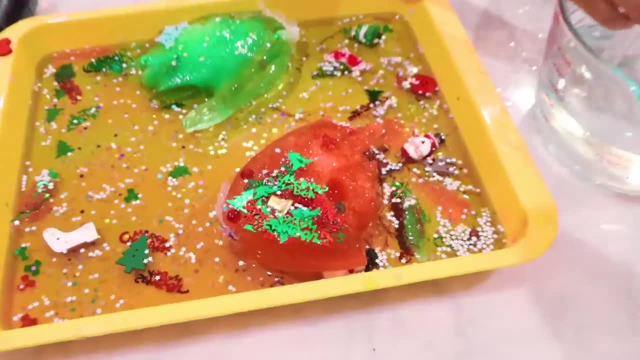 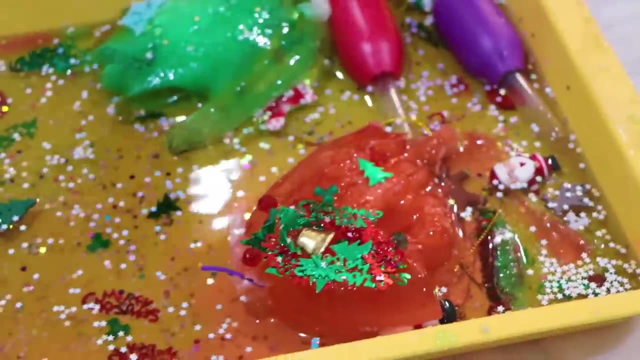 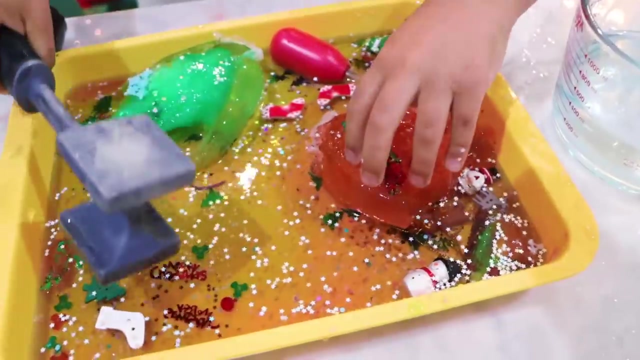 Whee, Yes, and the gingerbread man. Guys, one more the bell. Okay, Come on, you can get it. This time I'm going to use the hammer again. Wait, did I get it out? Wait, I got other stuff out. 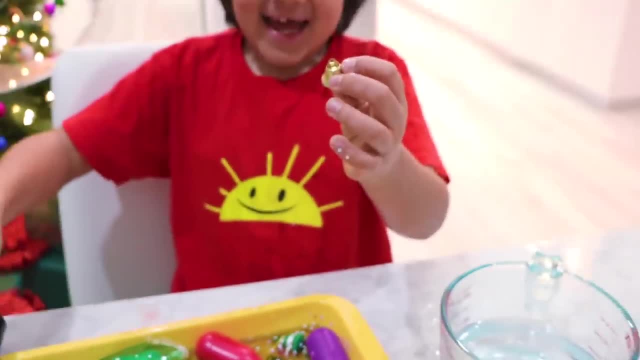 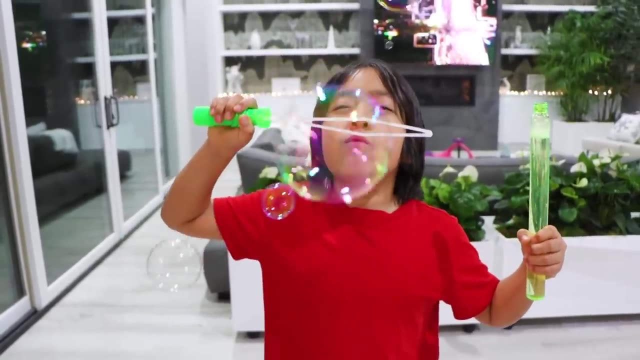 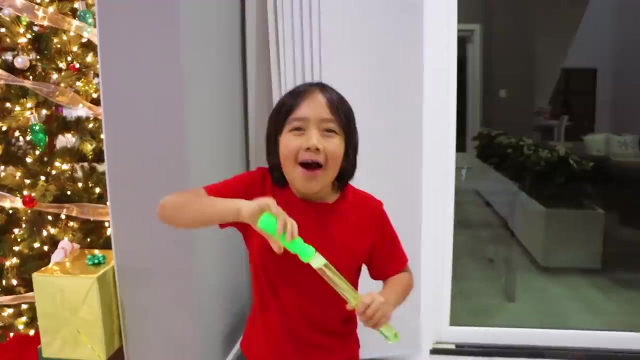 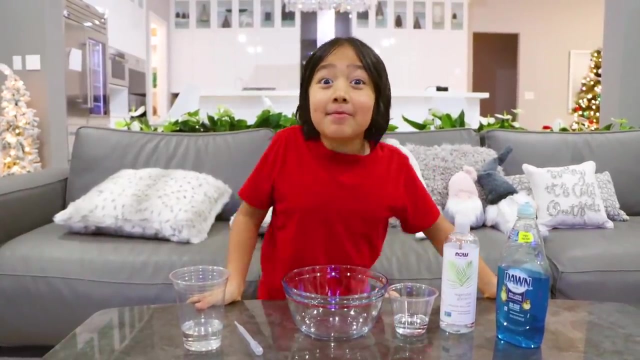 Wait, I got the bell. I got the bell out. Yeah, Guys, are you tired of bubbles that always pop? Aww, Today I have a solution for you: Non-pop, Popping bubbles. Let's go. Hey guys, today we're going to make bubbles that don't pop. 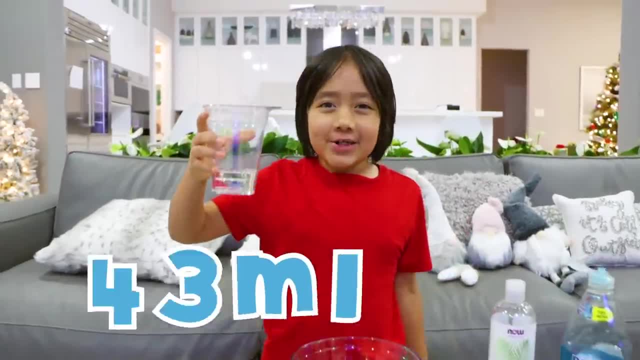 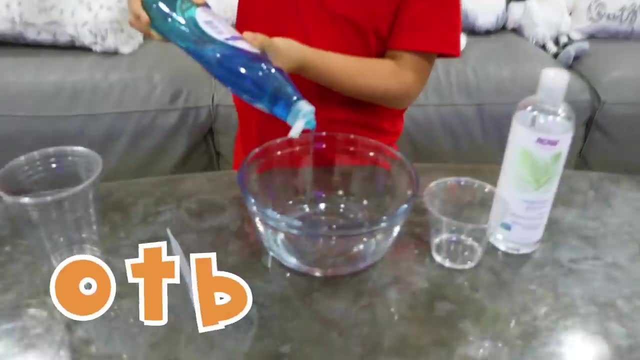 But always ask a parent for help. So first you need 100 milliliters of water and then 50 milliliters of glycerin and a squirt or one tablespoon of Dawn's soap. Next let's agitate, or another word for mix. 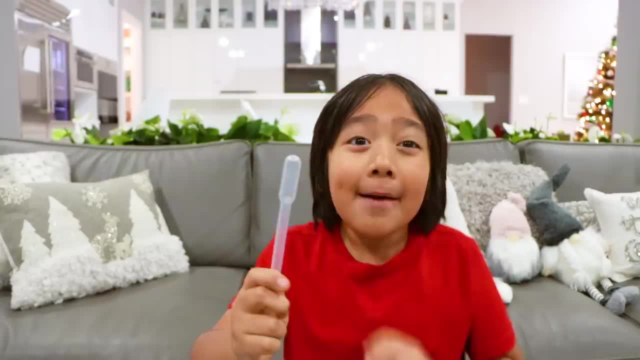 Next, get a pipette and cut it right here. I'm going to ask my daddy to help me. Hey, Ryan, All right, so we're going to cut right here. All right, I'm going to cut this for Ryan. 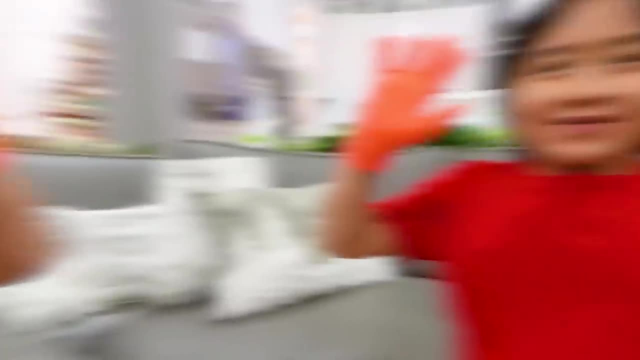 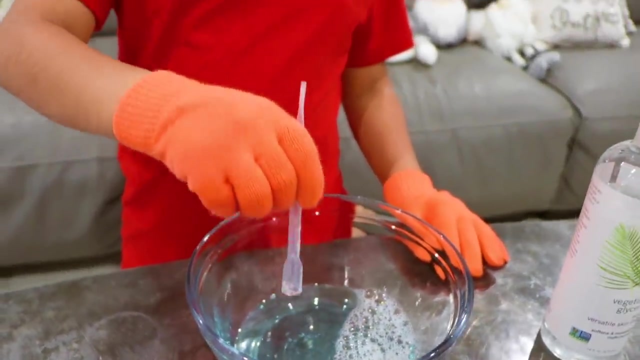 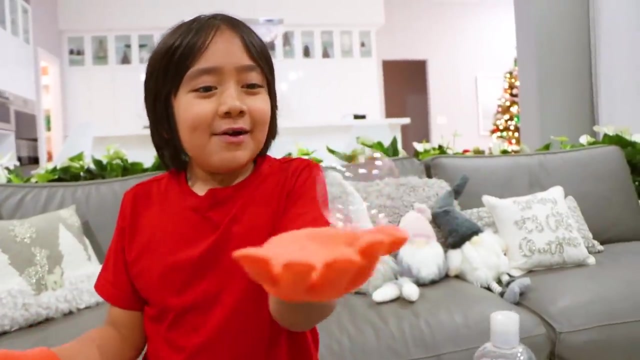 Boom, Is this what you wanted? Yeah, Next you need some woolen gloves, and then you take the pipette, dip it in the water and glycerin, and then there you go, Whoa, Whoa, Whoa. 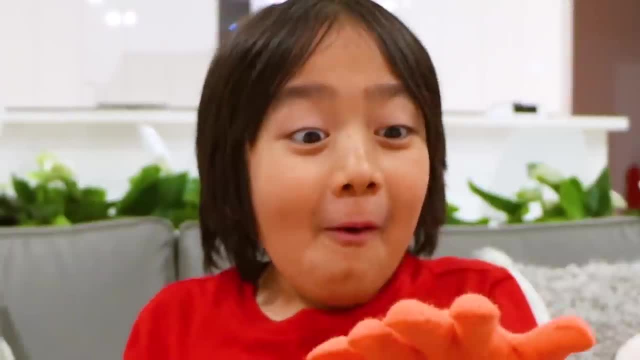 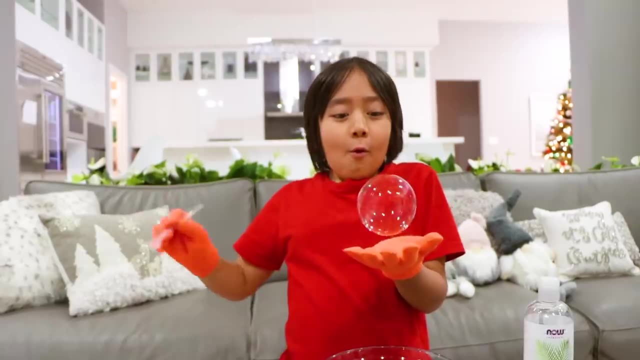 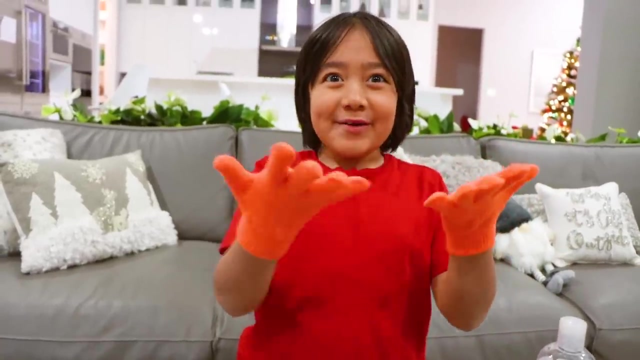 Whoa, Whoa, Whoa, Whoa. Let's try that again. OK guys, we're going to see till it pops. It already popped. Now me and Daddy are going to throw the bubbles to each other until it pops. 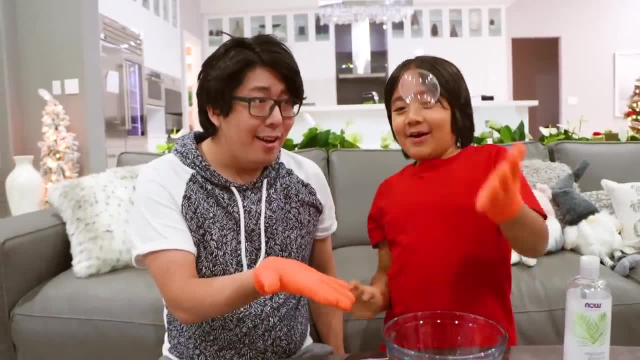 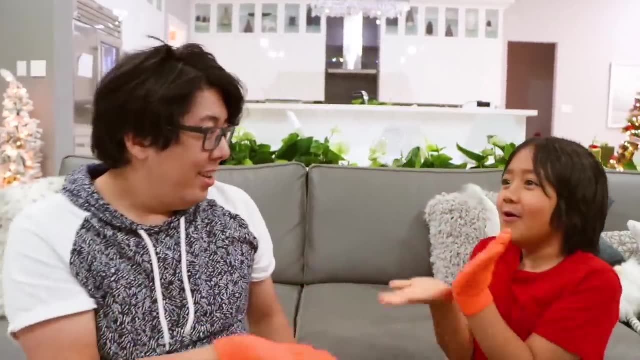 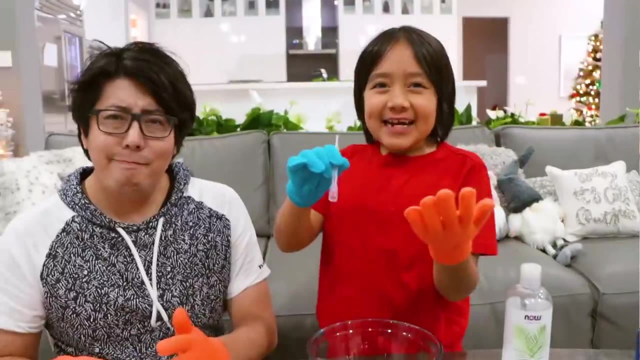 Whoa Whoa, It's not popping, Whoa Whoa, it's bouncing. Yeah, Whoa Whoa. oh, oh, my real. yeah, make sure you use your glove. okay, guys, now I'm gonna make a bunch of bubbles and I'm gonna see how much me and Daddy can hold. break the. 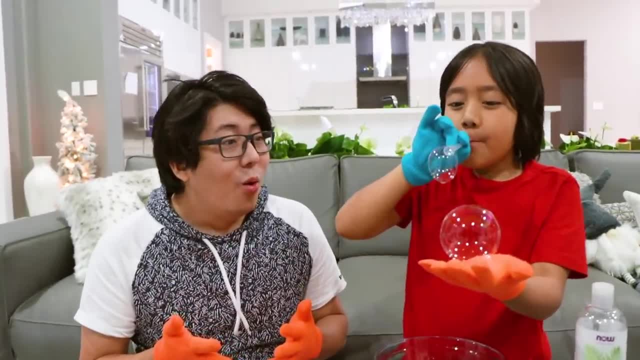 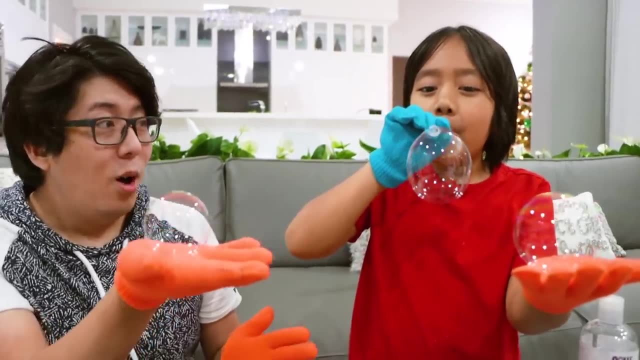 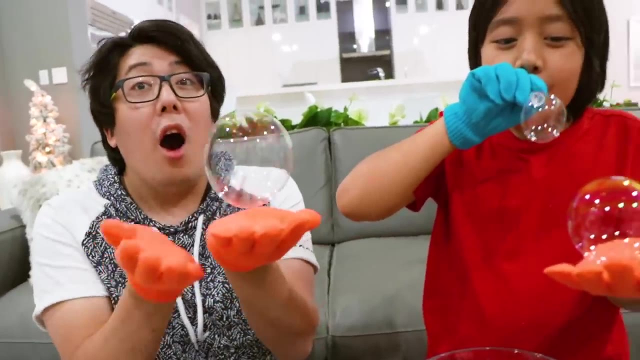 world record. Whoa, oh, whoa, whoa, whoa, come here. whoa, Ryan, that's huge. oh, it bounced on your tummy. can I put it together? oh, oh, did you guys see? it became one wait, so can. 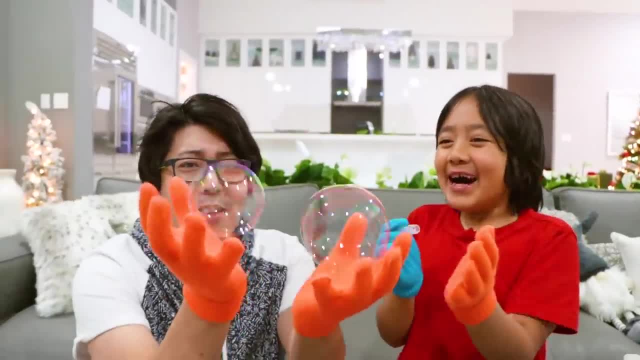 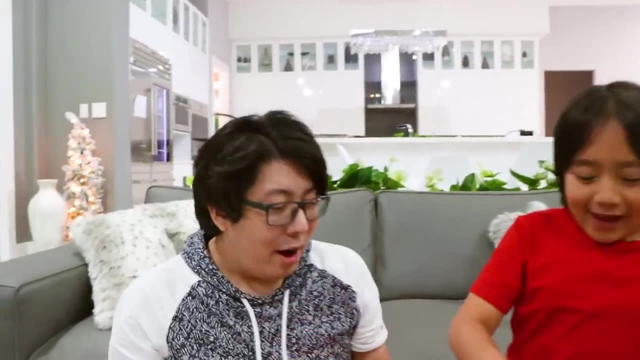 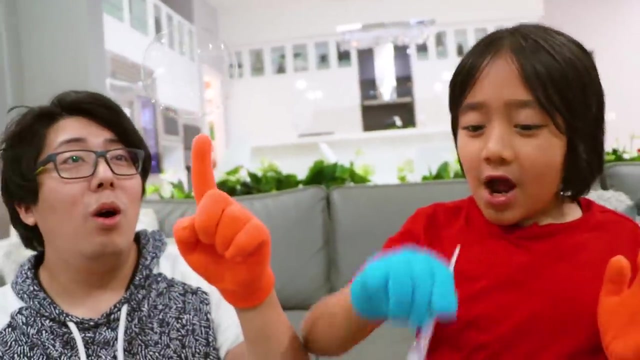 we combine ours. yeah, oh, never mind. oh, it popped. oh, you can just bounce it with your. oh, never mind. oh well, I made a giant. one. nice, here you go. oh, whoa, whoa. 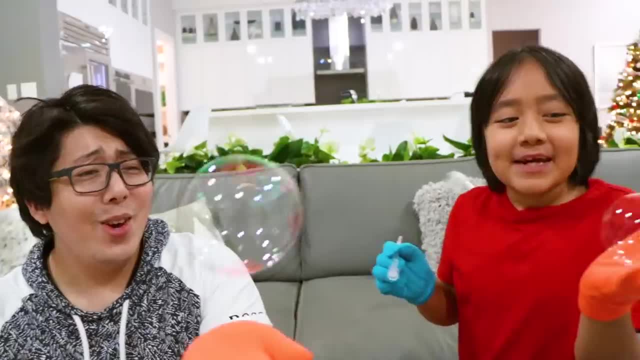 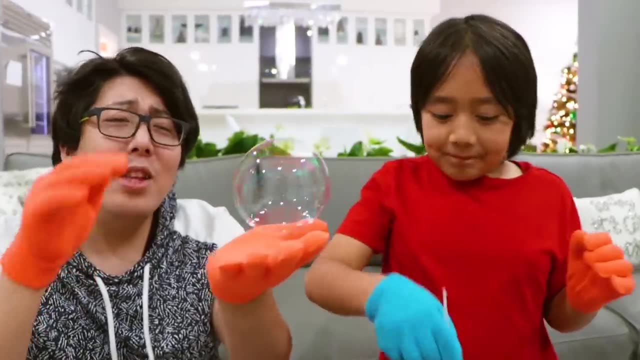 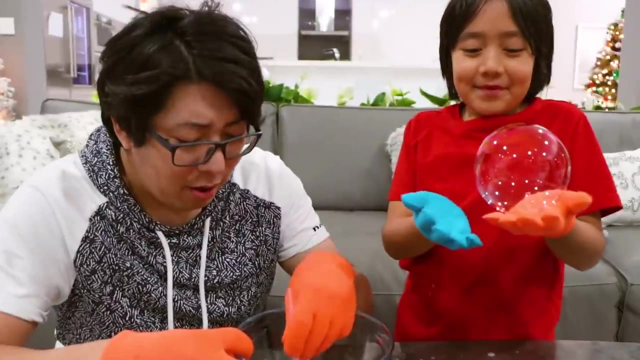 whoa, whoa, whoa. can I throw mine at yours? yeah, let yours pop. it's like a pet, you know, can I pet it? oh, no, it's gone. oh, all right, my turn. 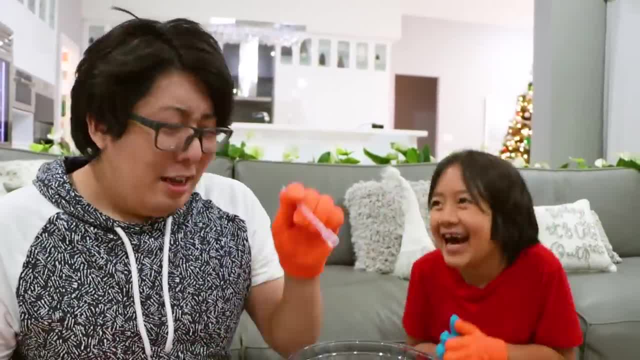 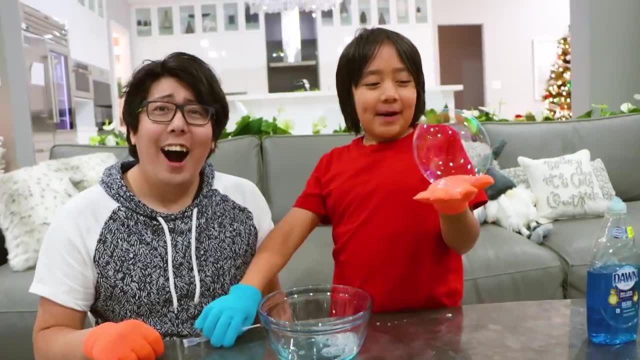 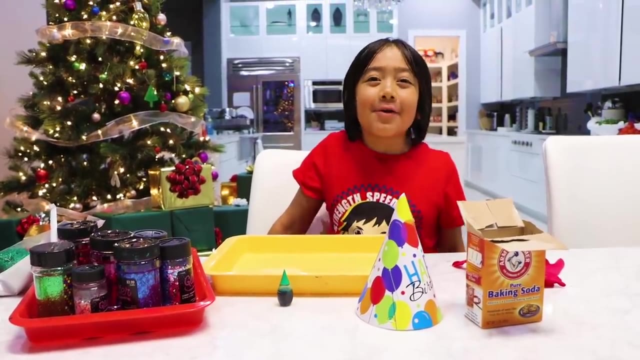 oh, oh, I can't break those records, okay, guys. so that's how you make a not-popping bubble. thank you for watching. let's do a fun holiday science experiment. we're gonna make a baking soda Christmas tree, obviously first. 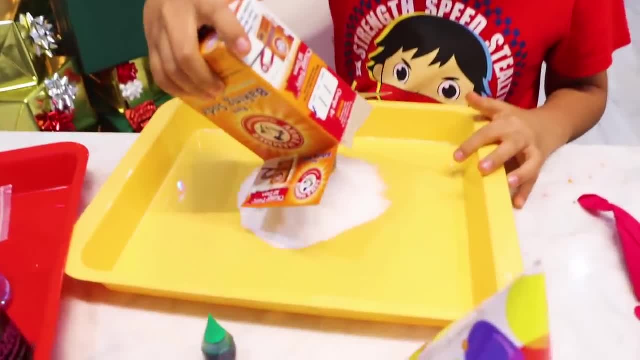 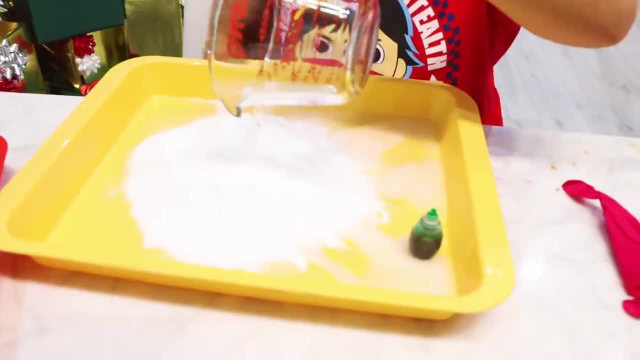 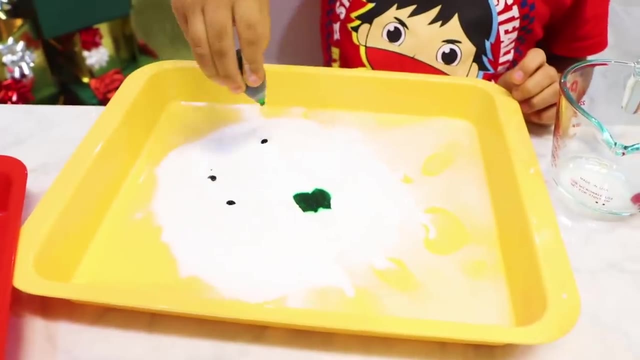 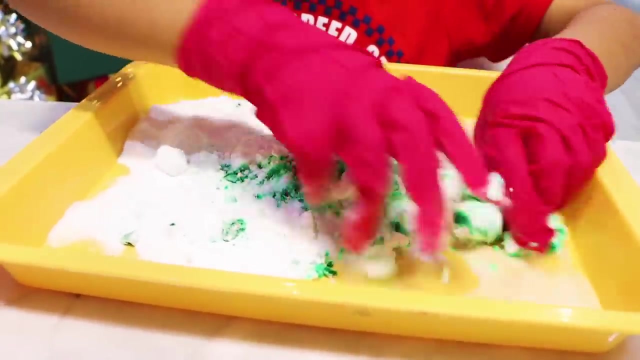 you need baking soda- all of it over here, okay, so next, use one-fourth cup of water and you can use any color you want, but for a Christmas tree I'm gonna use green. next let's mix it together, but I'm gonna use gloves because I don't want to get dirty. 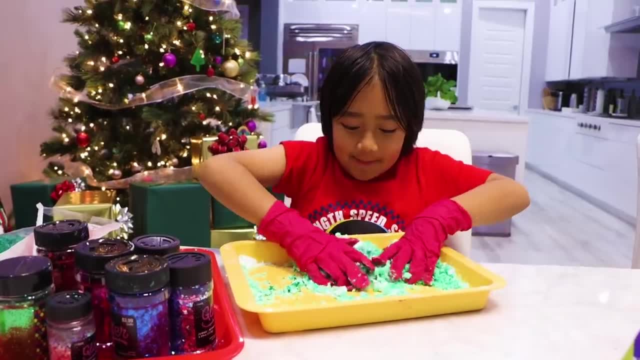 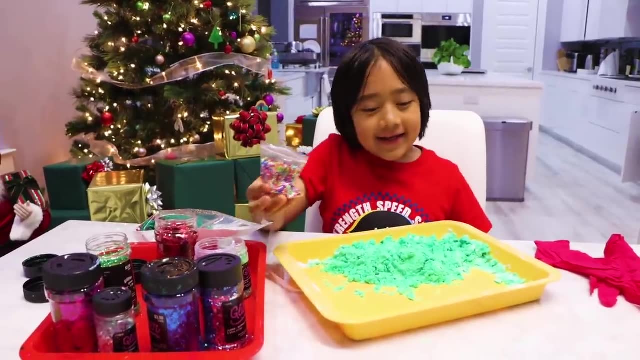 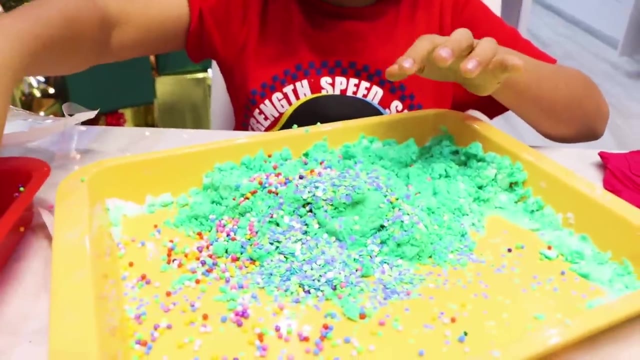 mix it with the water too. mix, mix, mix. I'm mixing them all together. look guys, everything's almost green. next, add in some glitter or anything you like. that's a lot. okay, then I'm gonna add some of this. oh, that's a lot. 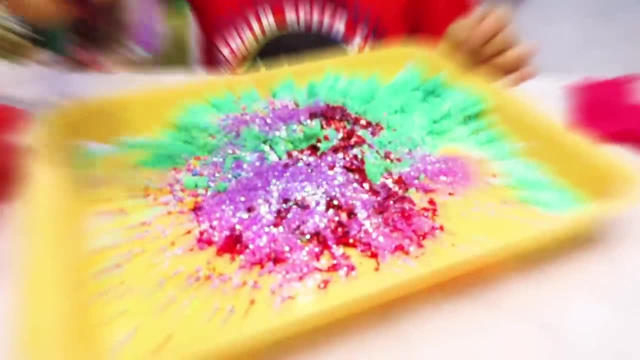 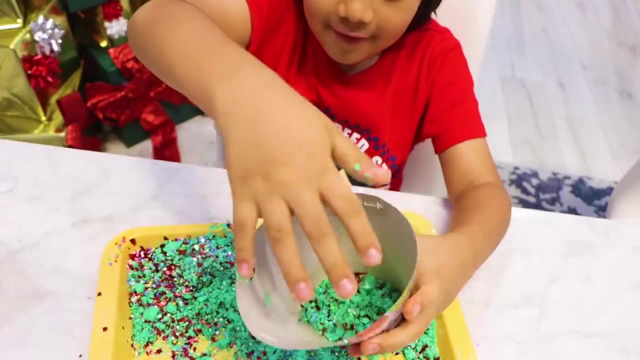 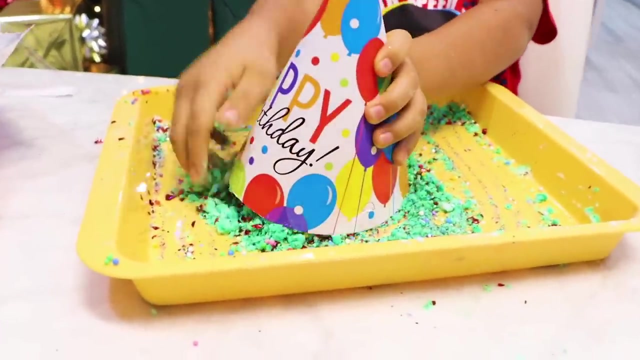 whoa next. mix it again. I have so many. find yourself a party hat or anything that is shaped like a cone and put the baking soda inside. flip it over. make sure your hand is over like this. whoa put it in the refrigerator. sorry guys, I'm at freezer. put it overnight. 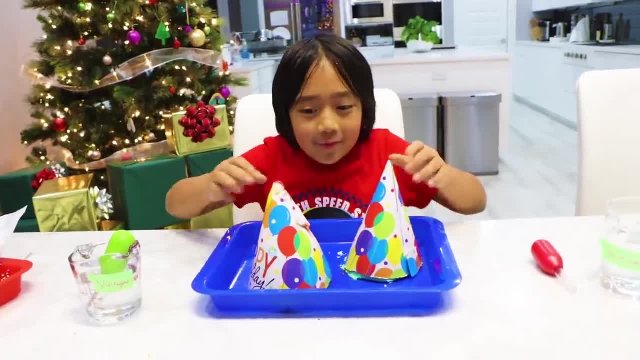 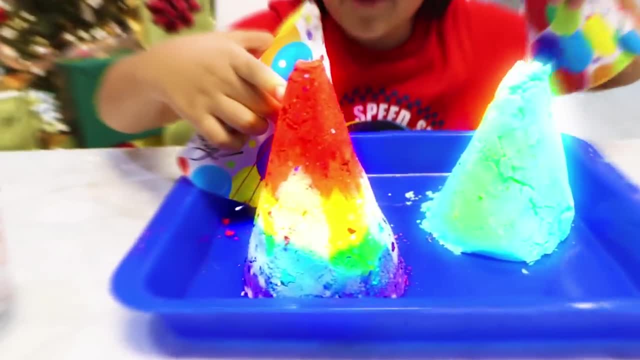 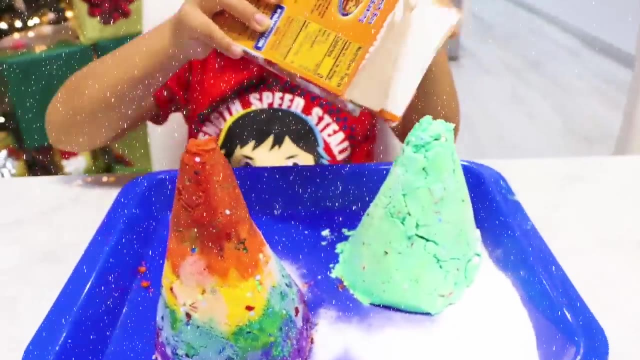 it's a few hours. so my mom actually pre-made these for me and she said: there's a surprise inside. there's a green one and a rainbow one. I'm gonna make it look like snow, so I'm gonna put baking soda all around here, here, here, baking soda everywhere. 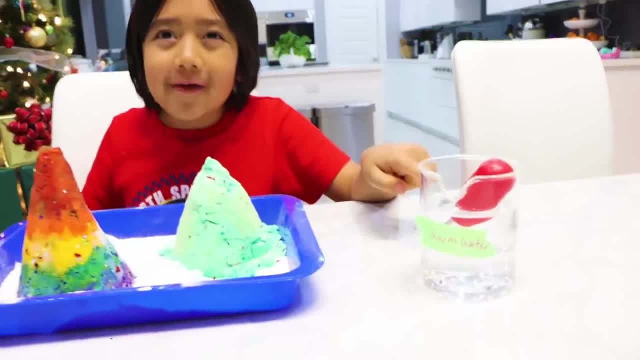 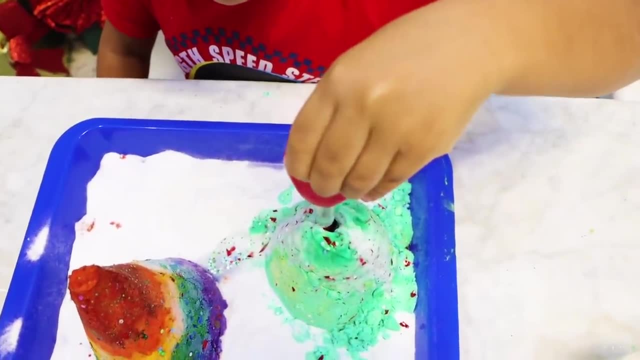 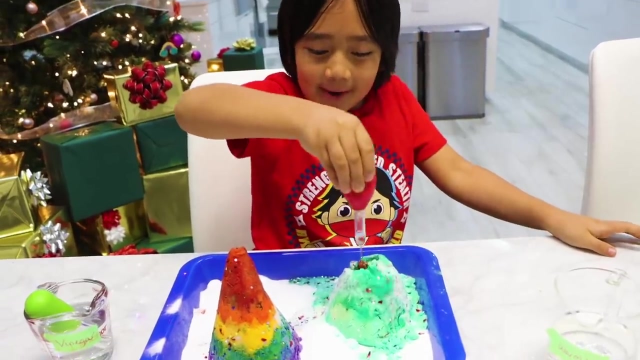 I have warm water and vinegar. we're gonna see which one reacts better. okay, first I'm gonna try the warm water. wait, I see something, it's a gingerbread man. I think I'll get him out this time. yay, I got gingerbread man. 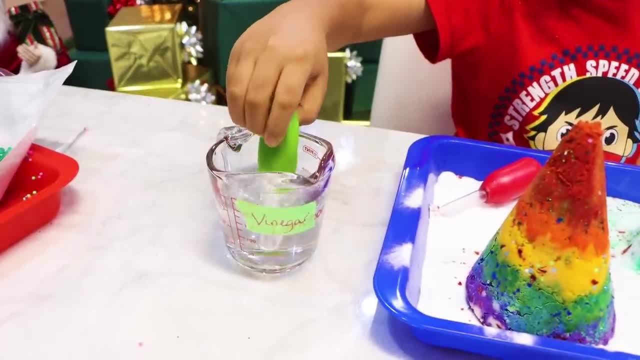 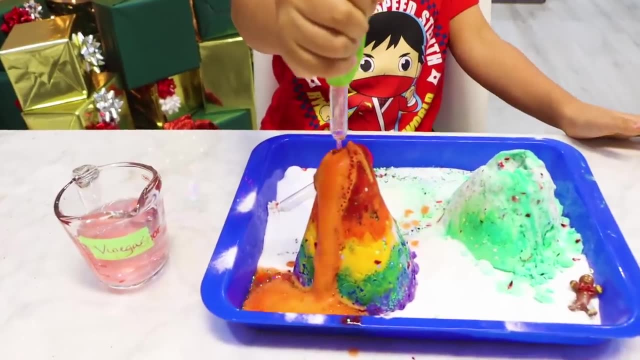 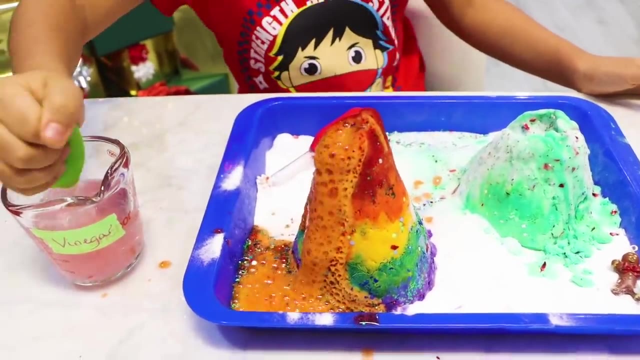 now I'm gonna test out the vinegar. okay, three, two, one, whoa. oh yeah, since this is baking soda, we're using vinegar. it's gonna make a reaction. I think this one's way stronger. okay, guys, I'm gonna pour the whole thing now. 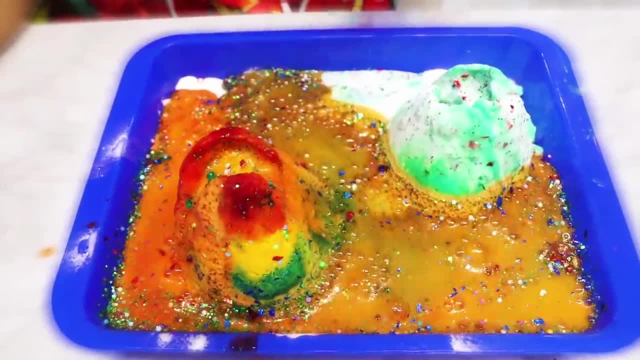 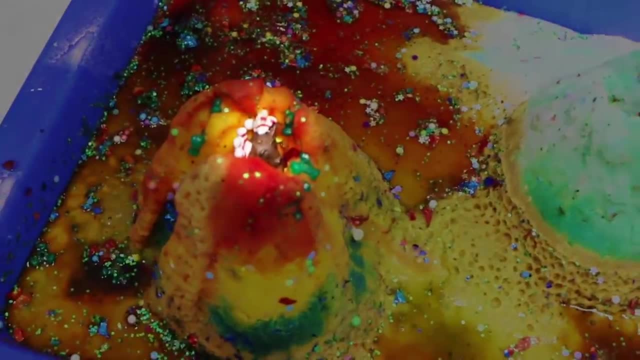 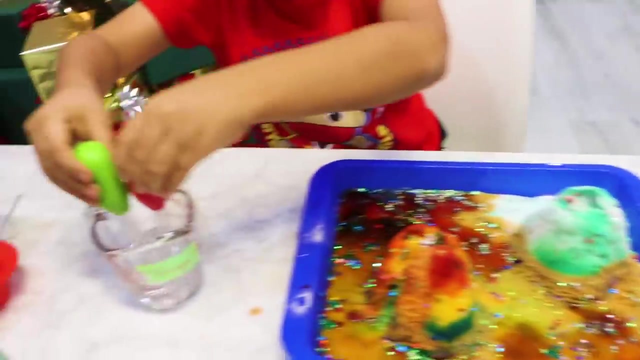 whoa, oh, it's touching the other one. whoa, wait, I see something. it's a reindeer. guys don't worry, reindeer, I'm coming for you. double vinegar: hot water into the vinegar. 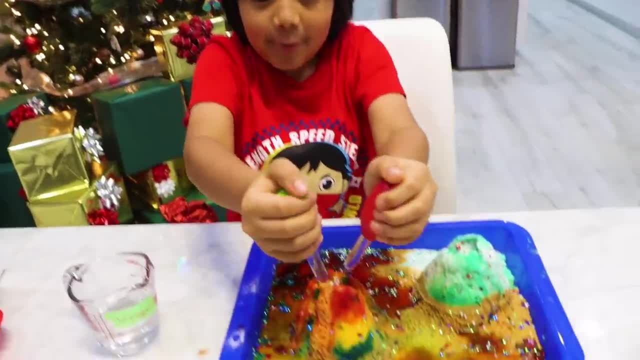 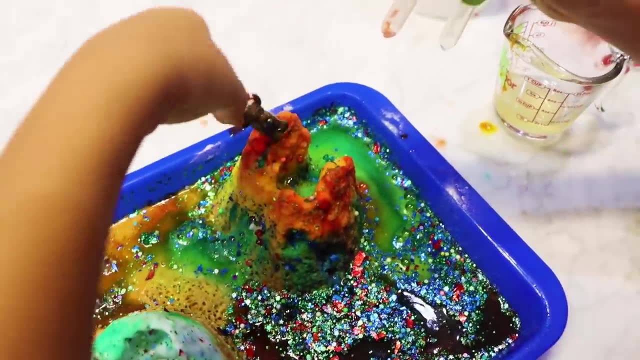 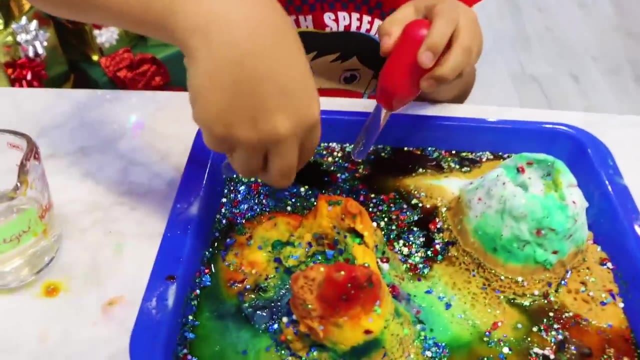 then it's gonna be hot vinegar. then boom extra strong. whoa, oh, I got him out. yay, my mom says there's actually two more surprises, let's find them. and I just took out a big part, so I think I'm gonna do that with this part too. 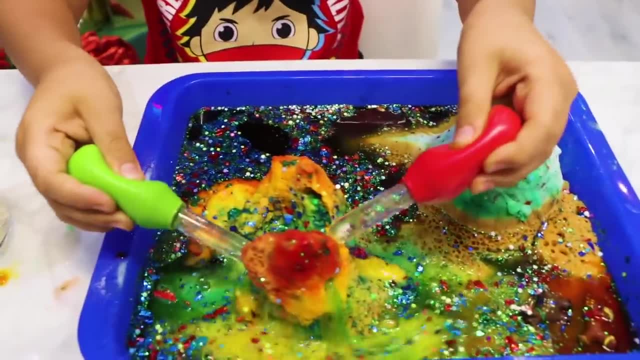 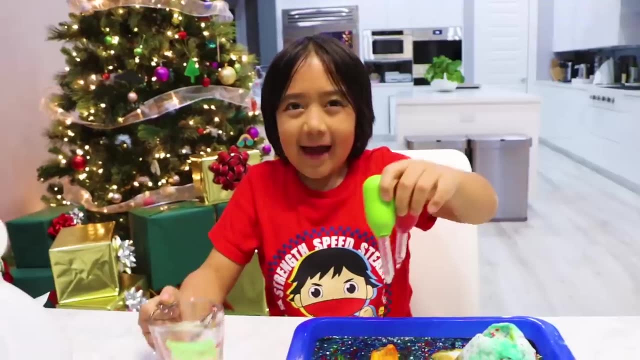 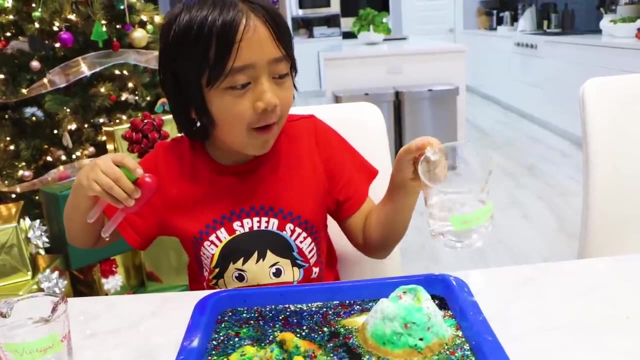 okay, oh, what's there? one more, one more, boom, yeah, I'm gonna dump the whole thing. whee, now I'm gonna pour all of the warm water. whee, whoa, that's super strong. 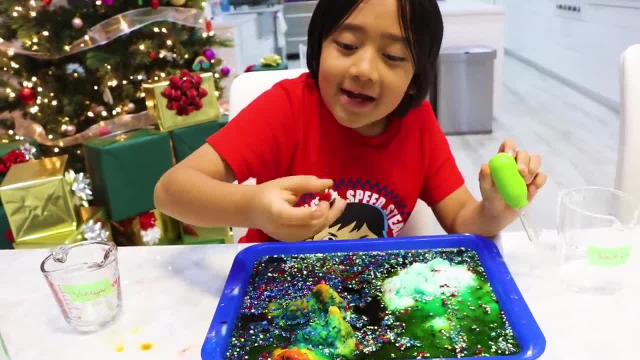 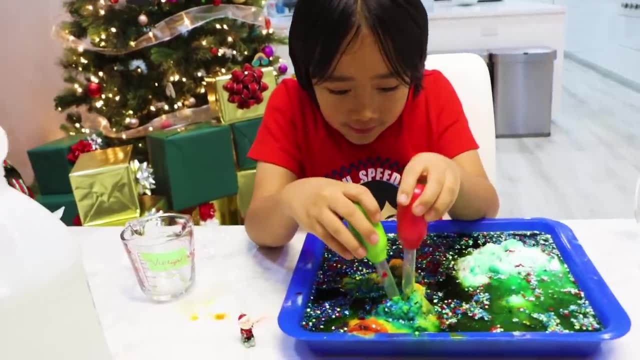 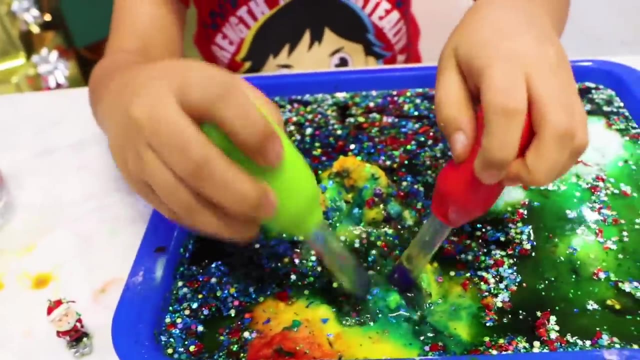 I see something. it's Santa. yay, we saved Santa. okay, guys, there should be one more here. wait, I see something I'm gonna save you. oh, there's something here. no, oh wait, where'd it go? 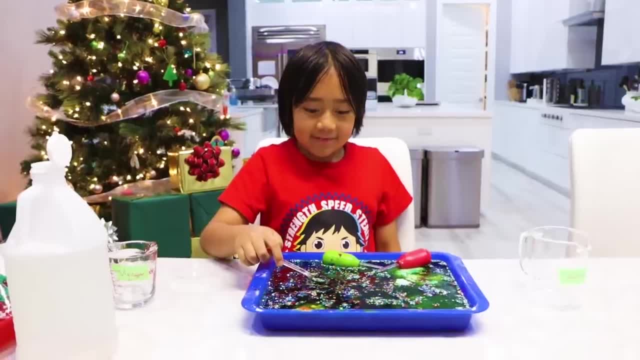 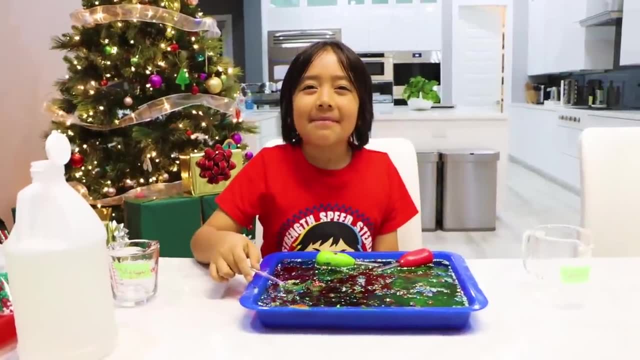 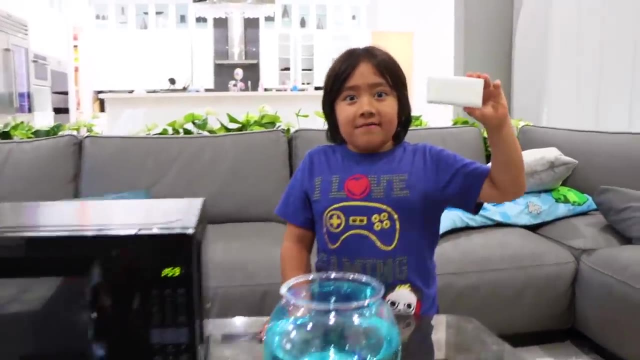 no, no guys, I'm using a spoon. oh, I found something: it's a mitten. I hope you enjoyed my baking soda. Christmas tree science experiment. hi guys, today I'm going to microwave a bar of ivory soap and see what happens. 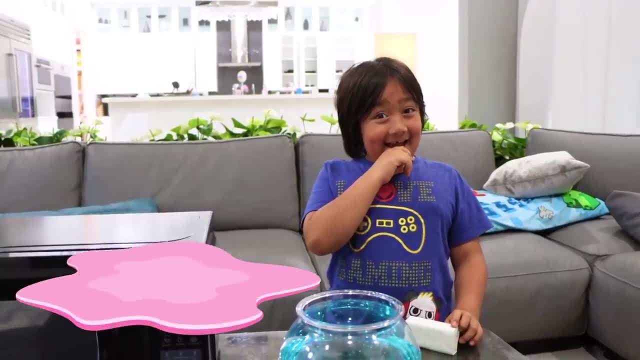 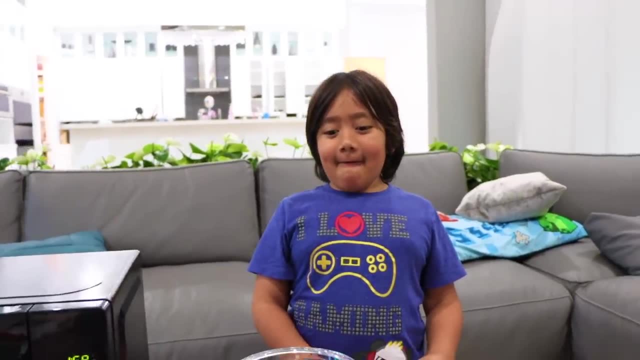 what do you think will happen, Ryan? do you think it's gonna melt? do you think it's gonna become bigger or smaller? disappear, what do you think? disappear, disappear, disappear. I guess we'll find out. so what I want you to do first is: I have water here and I want you to put the ivory soap into water. 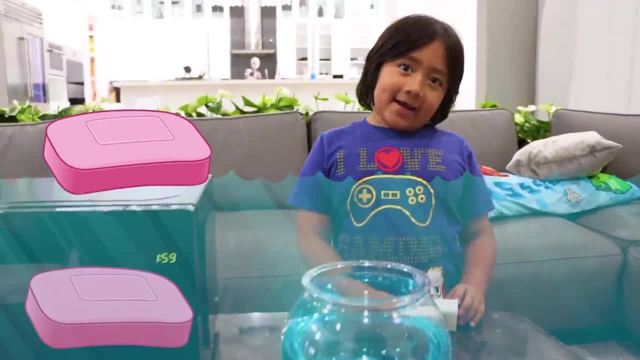 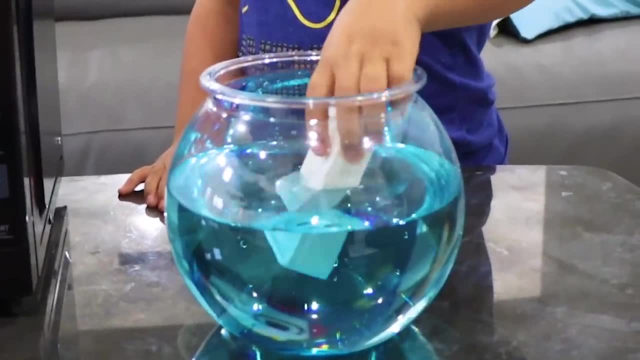 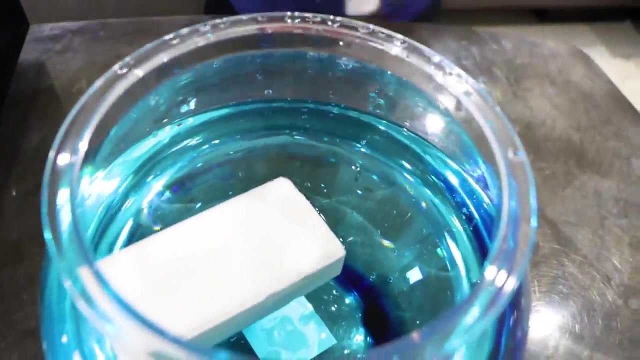 and first we're gonna see if it's gonna sink or float, okay. Okay, Do you think it's gonna sink or float? Maybe float? Okay, let's try it. It's floating. Yes, there it is. it actually floats in water. we don't have other bars of soap, but if you have a different brand, you can see if it also sinks or floats. 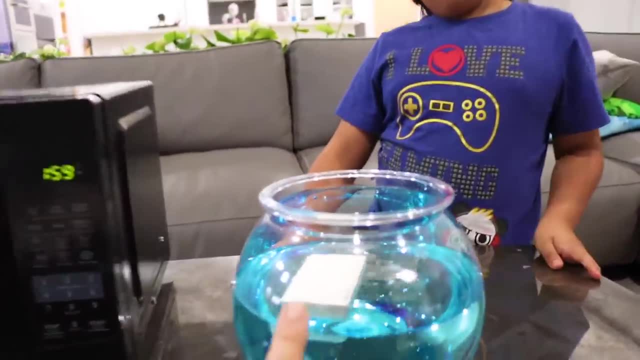 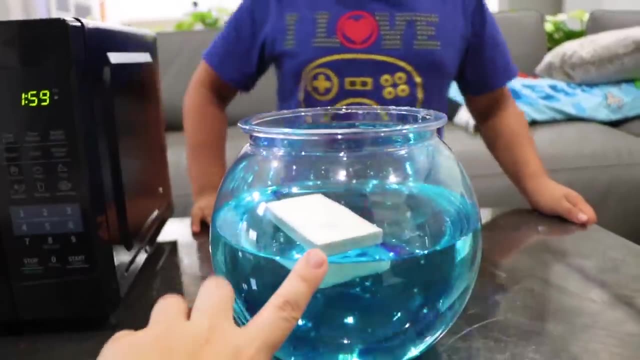 these are ivory brands, so what does it mean when it floats on water More dense or less dense than water? Less dense? Good job. The bar of ivory soap floated because it's less dense than water, probably because there's lots of air holes inside. okay. 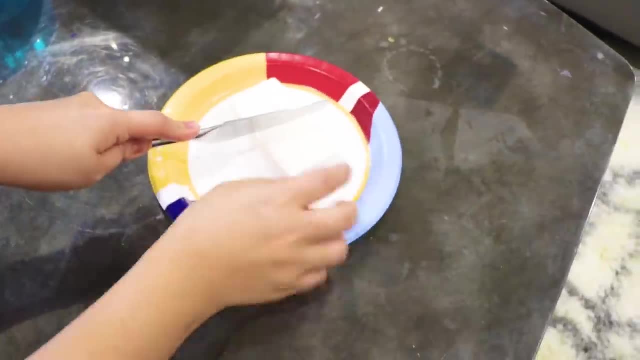 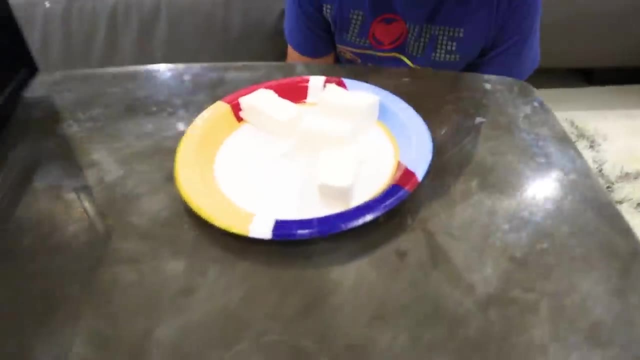 Yes, So we're actually gonna cut it open and see: okay, I'm gonna cut the bar of soap in half. okay, Alright, so I cut it more. if you examine it very closely, it has like little holes of. 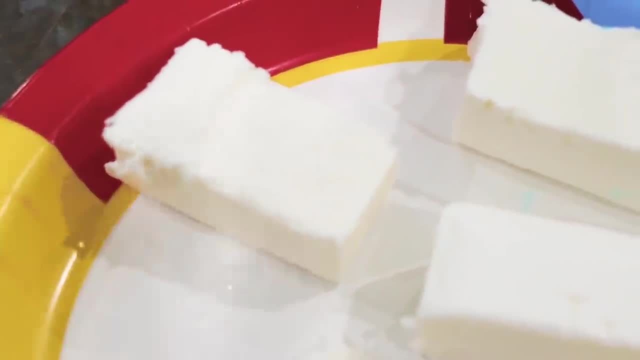 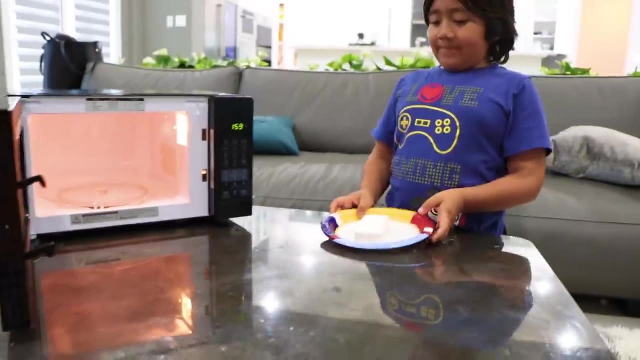 uh, emptiness. I guess it's where all the air is. Are you ready to microwave it? Yeah, Alright, we got our new ivory bar of soap here, put it in the microwave, closing it. Start. Here we go, alright. 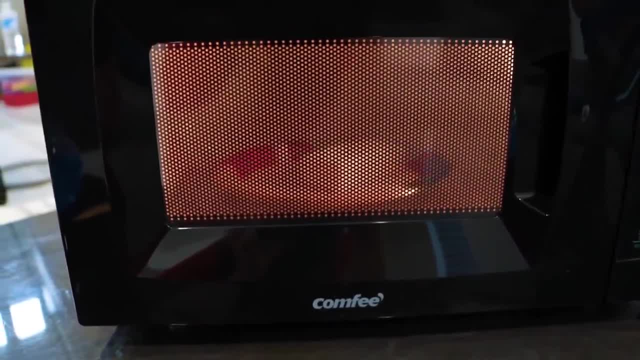 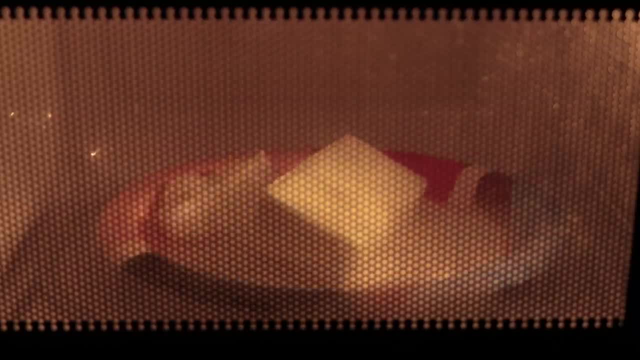 We're keeping our eyes on the bar of soap. make sure you use a microwavable, safe plate. Okay, let's see There's like stuff coming out of it. It's hard to see because of: Do you see like the stuff? 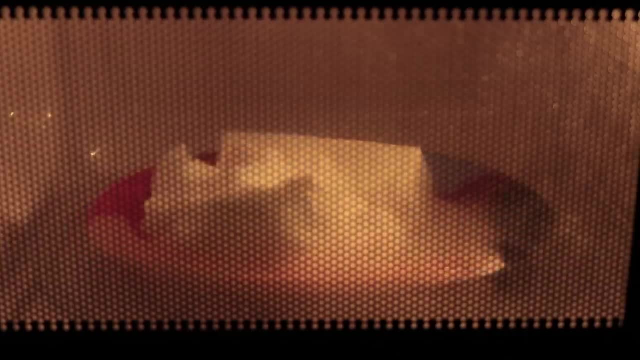 Oh, I do see. you guys see Whoa. keep your eyes on it, Look, guys, It's a little bit hard to see, but look, it's expanding. Yeah, it's expanding by a lot, Whoa. 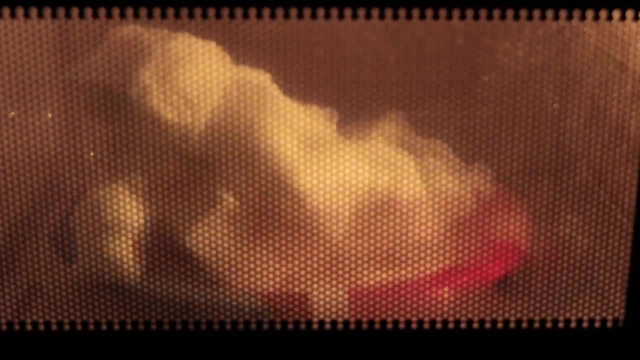 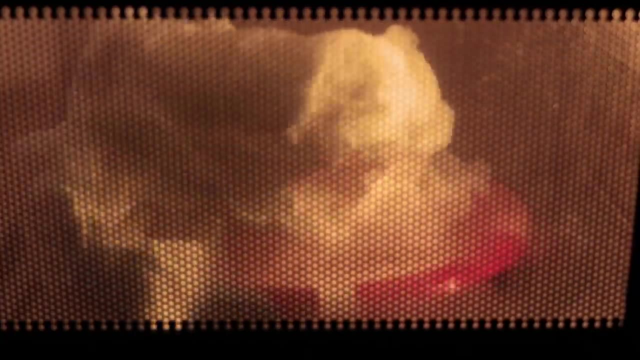 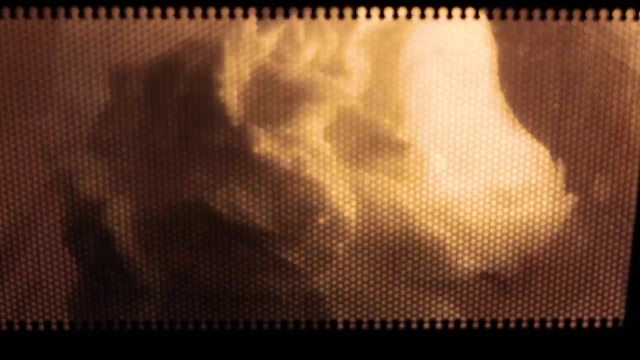 I think it's melting the soap or something. Whoa guys, look That's big. Should we stop it? It's gonna go all over the microwave. Whoa guys, look at this. Whoa, whoa, it's like it's the whole microwave. 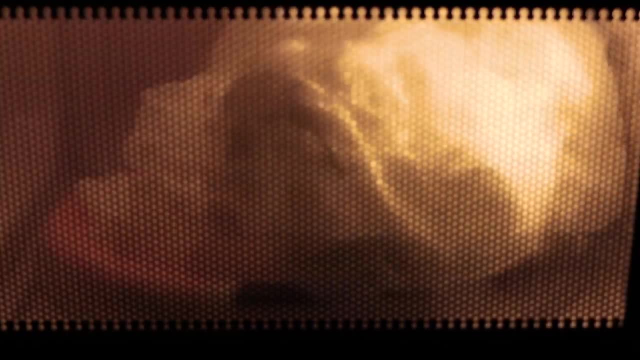 It's melting, Oh it's melting. Oh, what's happening? Oh, it's melting, Oh it's melting. Wow, look at that, Oh it's melting. Hey sweetheart, look, you're melting it again. 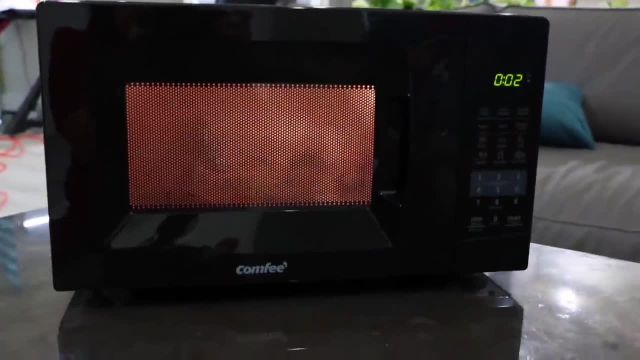 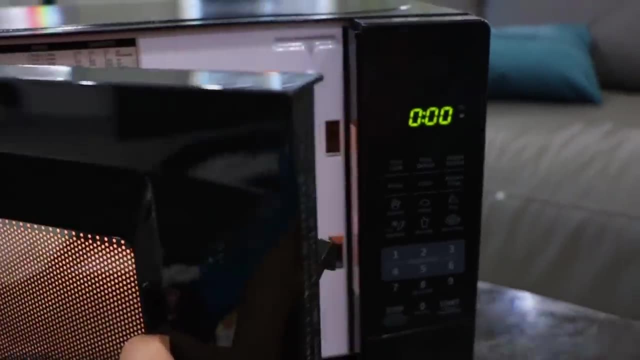 It's melting. Oh, what's happening? Oh, it's melting. Do you smell anything? A little bit It smells like soap. Yeah, Whoa, it looks fluffy like marshmallows. Okay, done, Okay, Okay. only adults do this, because it might be hot. 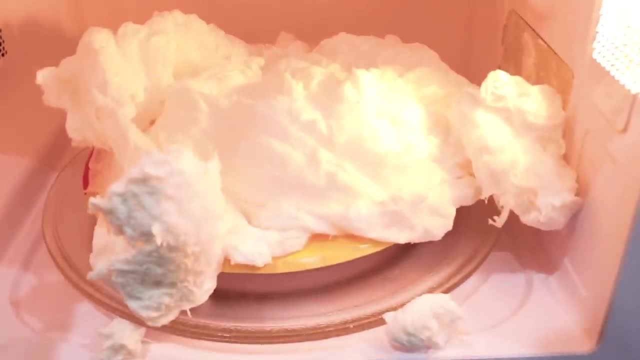 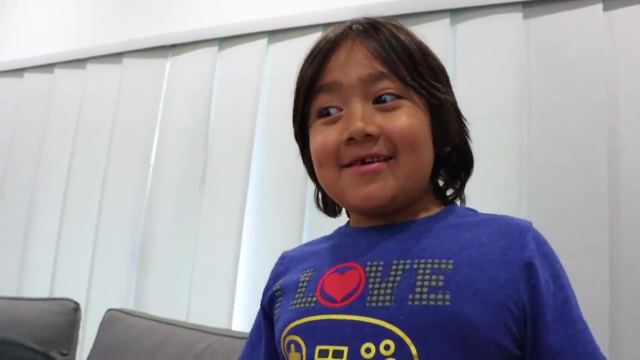 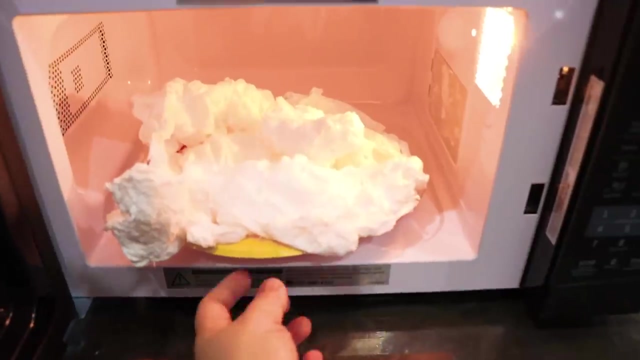 Oh, Whoa, Whoa, Did you expect that? No, So what happened? It got melted. and then it got, It's all melted, All melted, Ha-ha-ha. then it got bigger. it expanded, yeah, yeah, look, super expanded. look at that. okay, only don't touch. 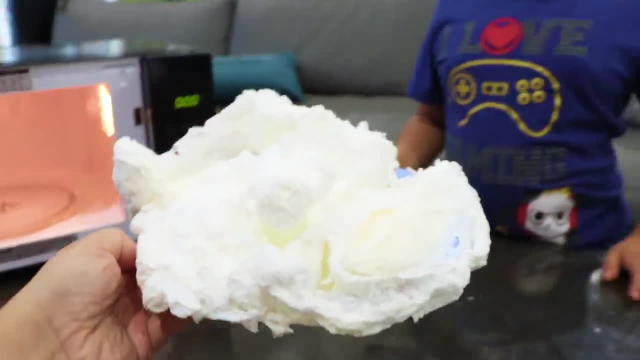 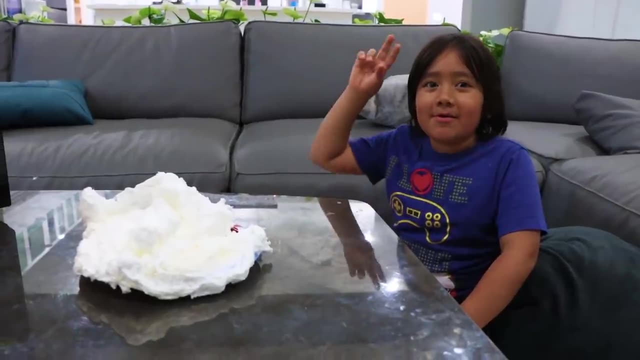 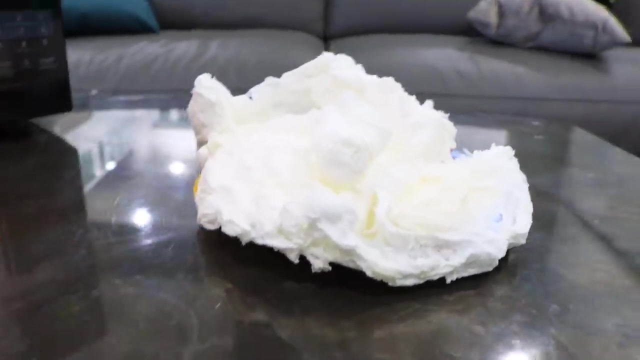 this. it might be hot. whoa, don't touch it yet. okay, it might be hot. okay, we're gonna wait for a little bit. but just looking at it, what does it look like? toilet paper that's you like, uh, scramble it a lot, got it. it looks like toilet paper to ryan a lot kind of looks like whipped cream. yeah, let's see. 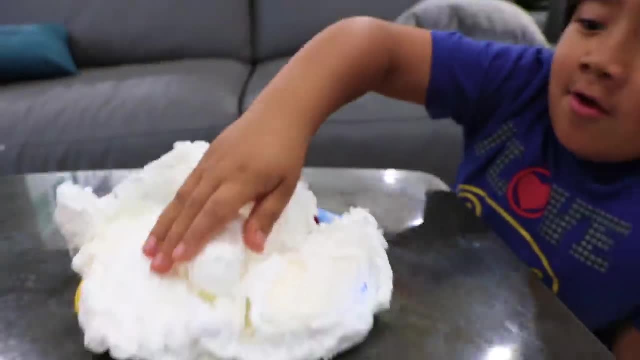 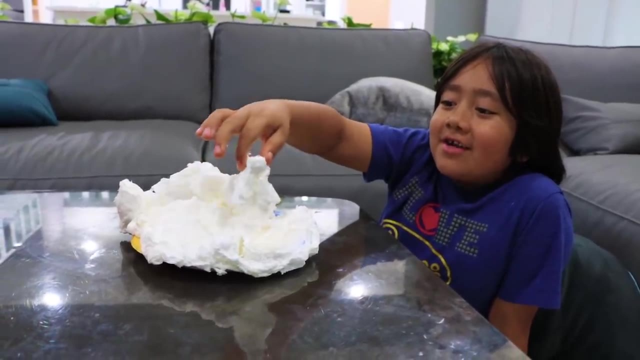 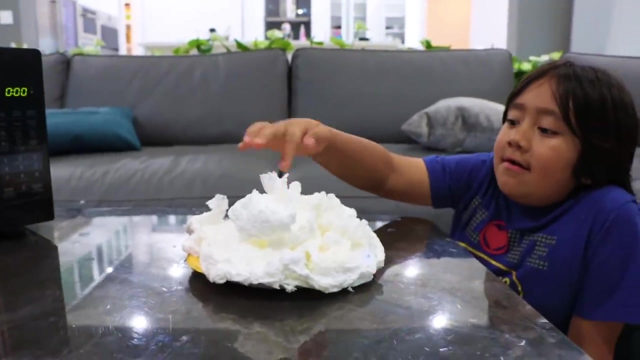 okay, so safe to touch. now, ryan, touch it and see what it. what does it look like? maybe, uh, like cotton candy really? yeah, wow, it's a little bit more rough. yeah, so this one actually only works with ivory soap. but wait, i don't understand how does it work? so why did the ivory soap expand to the microwave when it was made? there are air that is trapped inside the mixture and because of the air that's why it floats in water. so when you put the soap in the microwave, the air and the water molecules that was in the soap starts. 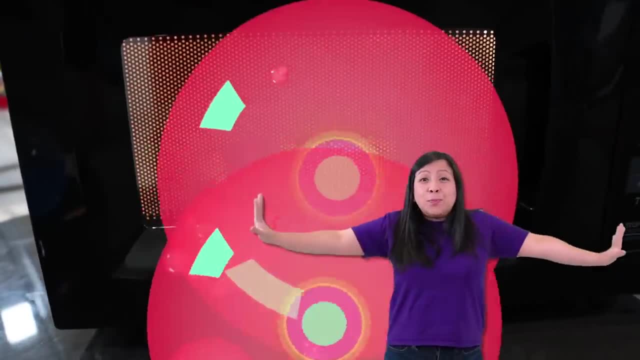 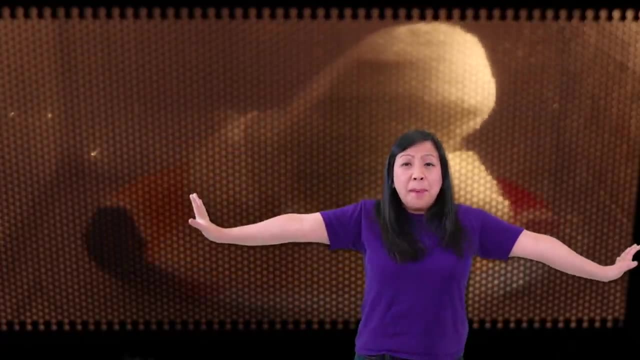 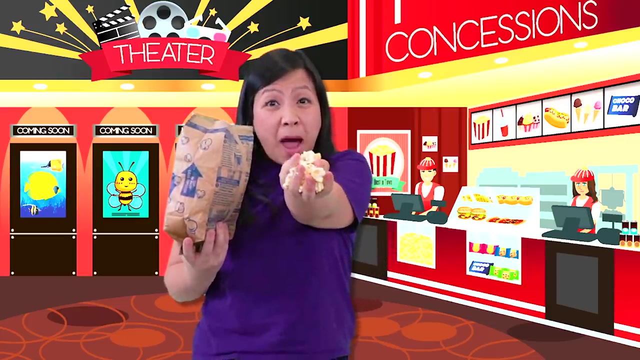 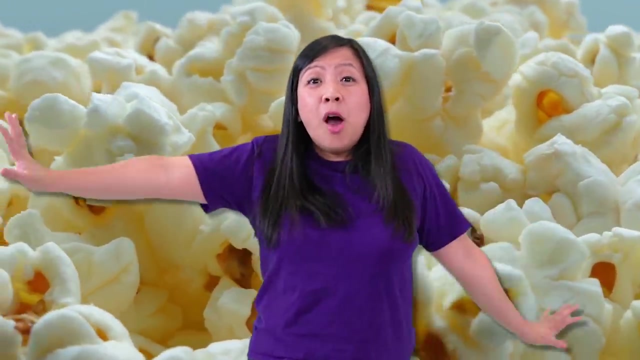 to heat up, vibrate and expand and spread farther apart. they push us against the rest of the soap mall. it kills expanding the bar into a fluffy cloud blob. do you guys like popcorn? it works the same way. water inside the kernel expands and pushes on the walls. as it's being heated inside the microwave, the water will turn into steam. 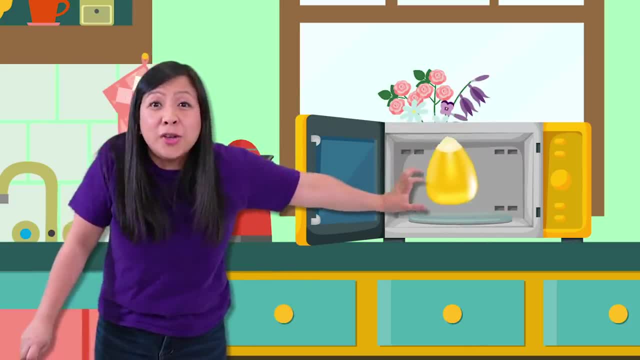 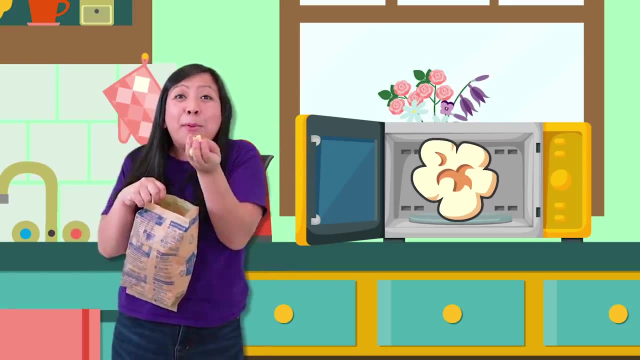 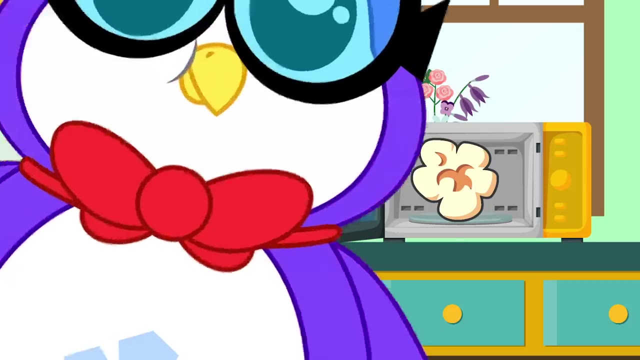 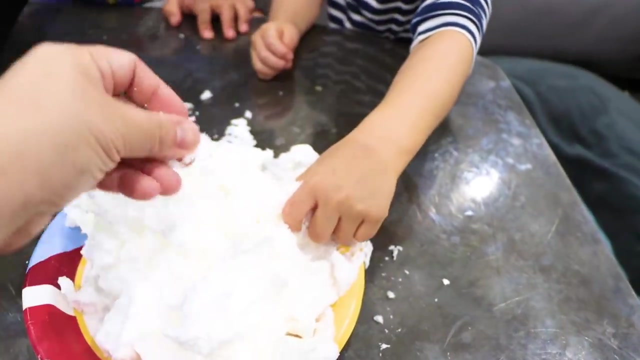 and expand and pushes along the wall of the kernel until, pop, the kernel explode and we have a yummy piece of popcorn. that was so cool. let's get back to ryan. now emma wants to touch it. yeah, so, emma, this is soap. apparently it's like coming apart. oh, i microwave it well, because i wanted to show ryan. 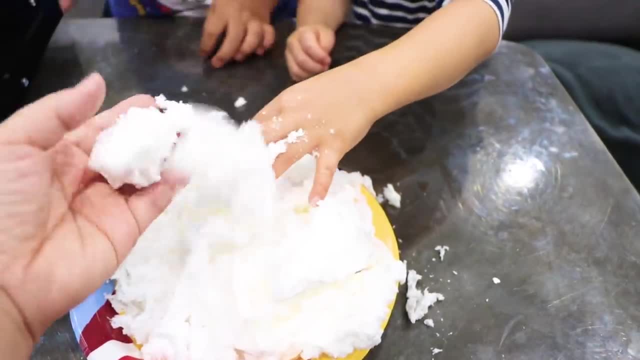 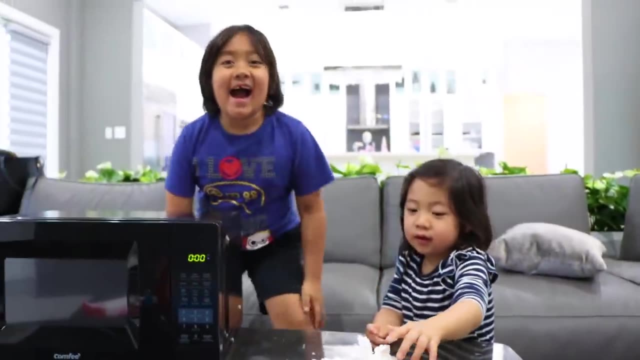 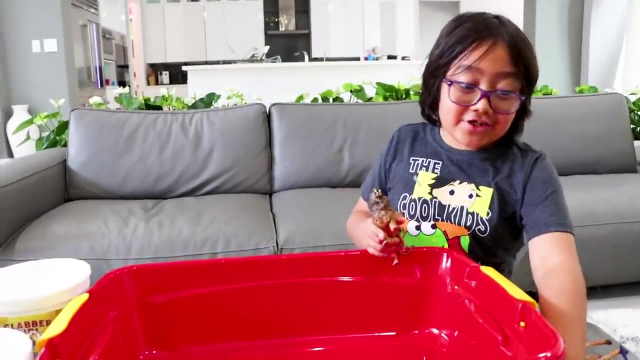 how soap expands when you microwave it. look see, but it's all mushy. yeah, but it's okay, it's just soap. we can go wash your hands, okay, isn't it cool? i'm going to go wash my hands, okay, isn't it cool? yeah, hi guys, today i'm doing the dinosaurs dig kit, but with animals and also one dinosaur and 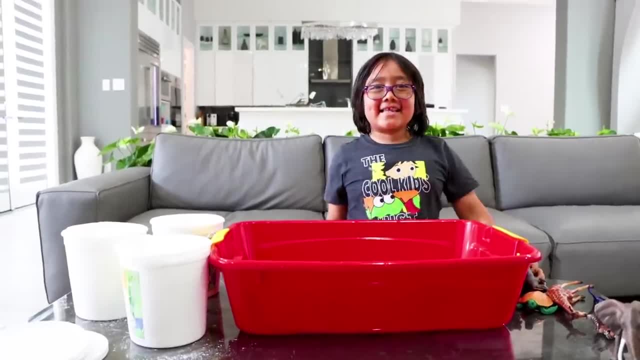 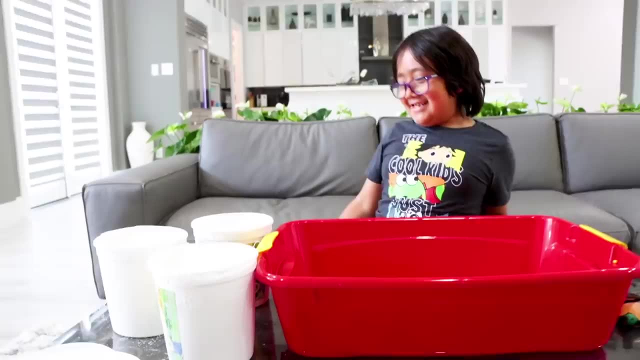 animals more so. this is a do-it-yourself at home science experiment, so all you need to do is add cornstarch. that's a lot. that is a lot of cornstarch. we're making a giant dig site, ryan, using all of it. yeah, let's try it okay. 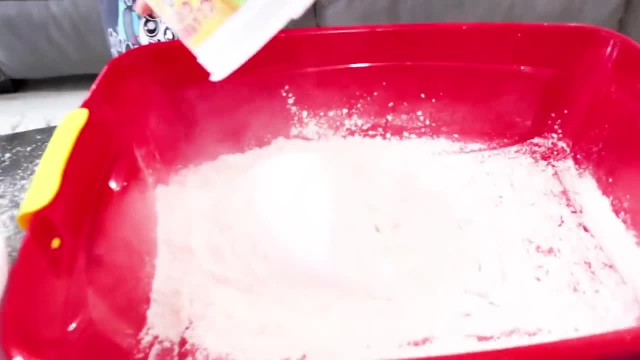 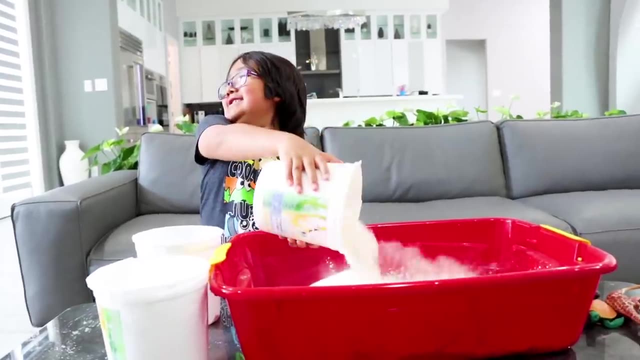 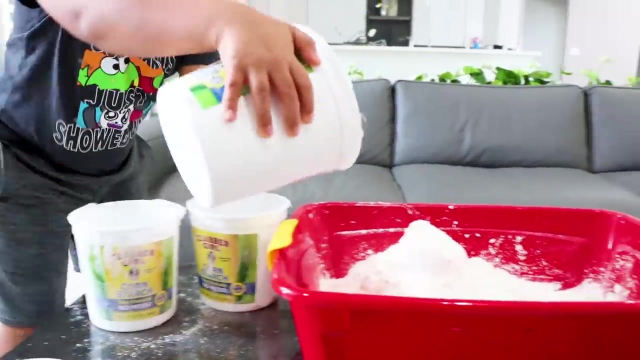 okay, get ready this video. it's gonna be messy, you guys, so please do it with an adult or do it outside. except, it's super hot outside right now, so that's why we're doing it inside- already very messy. one more: i know better outside, but outside right now is like whoa, it's like 90 degrees. so we 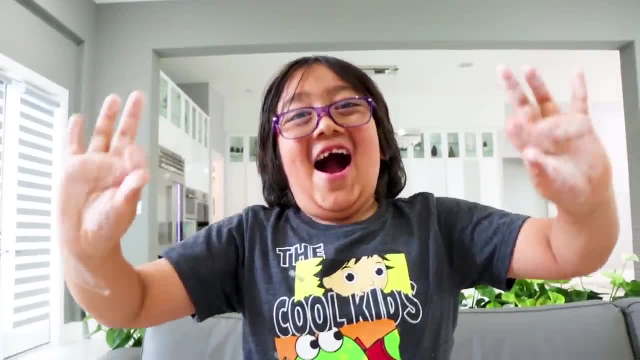 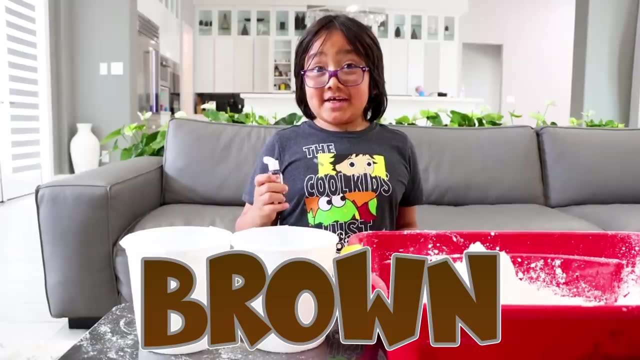 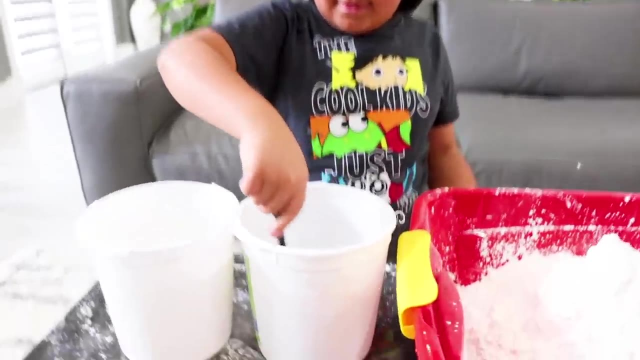 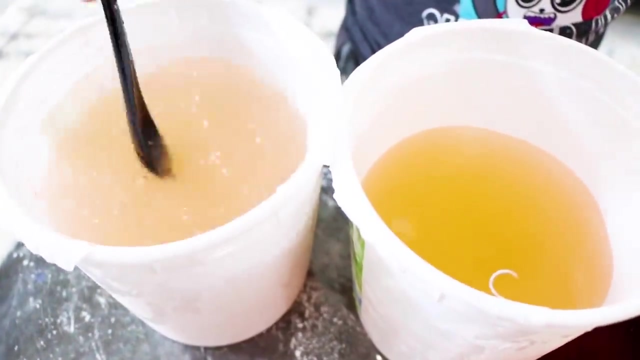 are risking it indoors. oh, poor animals already covered in corn starch. so i'm gonna make my water ground like sand. uh, eat, eat. now i'm gonna mix it already. perfect, there we go. oh, this one's better. okay, now we're gonna have to add the water into our 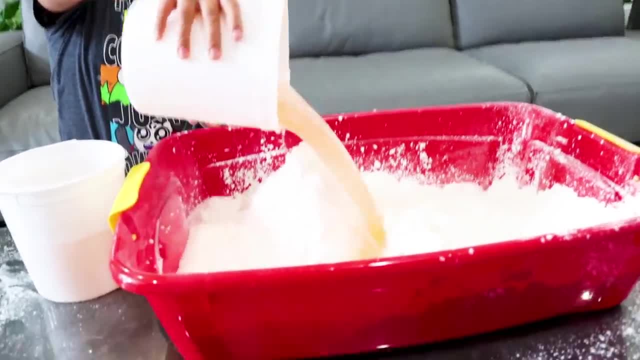 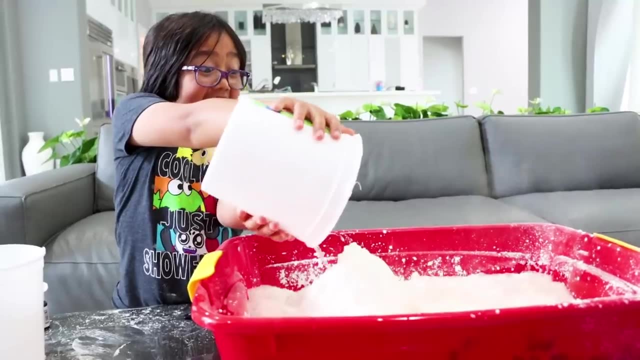 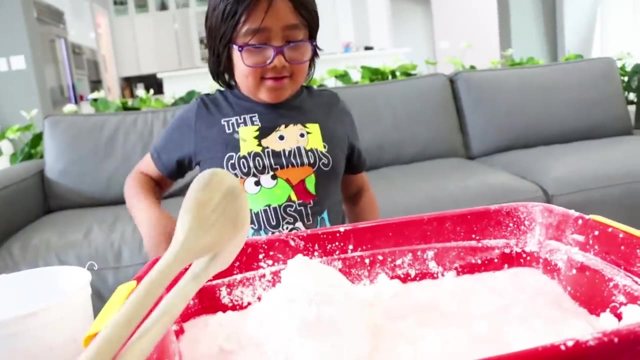 giant cornstarch. oh, that's a lot of water. we're actually making black. have you guys ever had black before? oh, we're making oobleck. yeah, this is like black. do you remember? oobleck is a substance, that it's a fluid where it could be a solid or a liquid, depending. 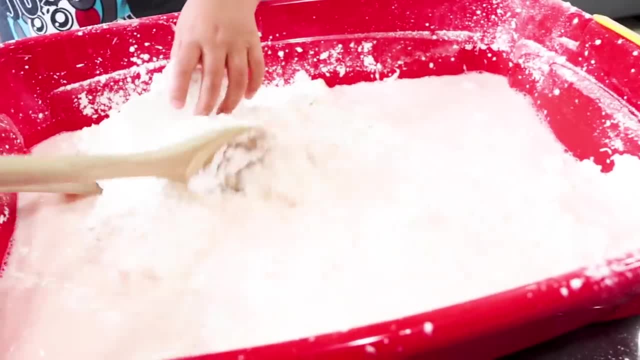 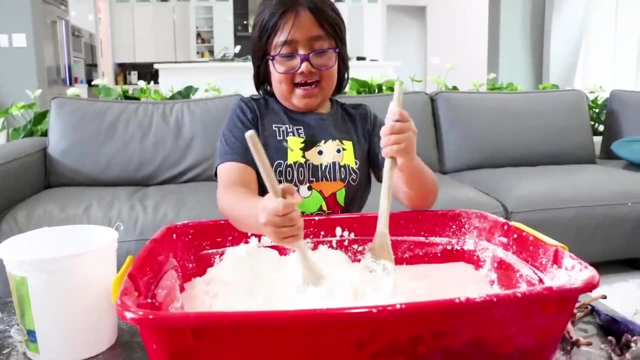 yeah, it's both all right, depending how much pressure or force you add. but next all we're going to do is just add: agitate, agitate, agitate. it's very hard, it's very sticky. huh, yeah, it feels. it feels like quicksand, or what does it feel like? 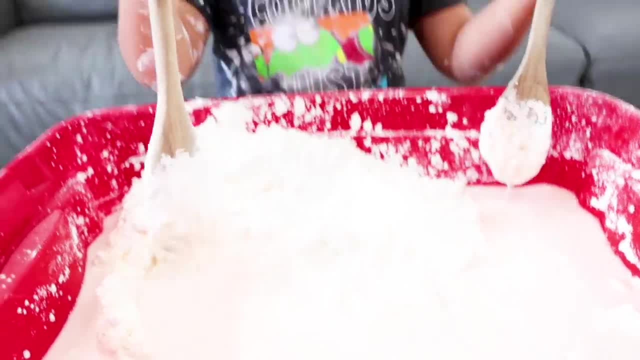 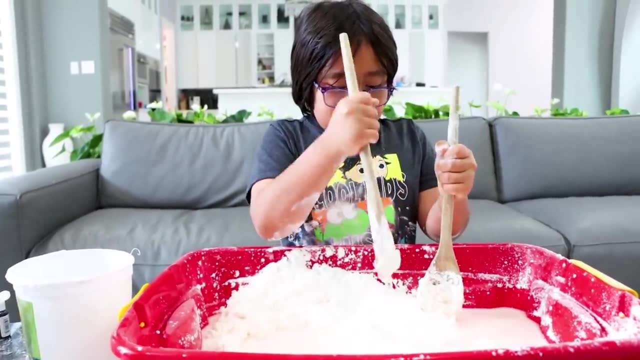 maybe, yeah, like quicksand, wait, it's already oobleck. yeah, you feel it. it's like down here already. all right, guys, we're gonna keep mixing it and then we'll show you guys when it's ready. okay guys, we got our oobleck. look, it's a liquid. 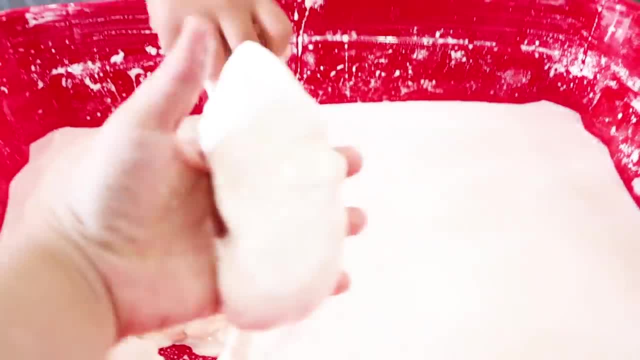 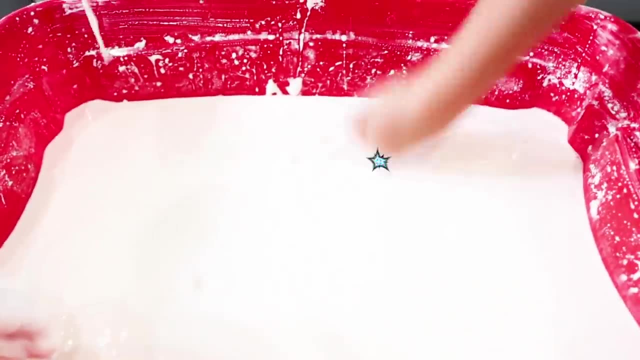 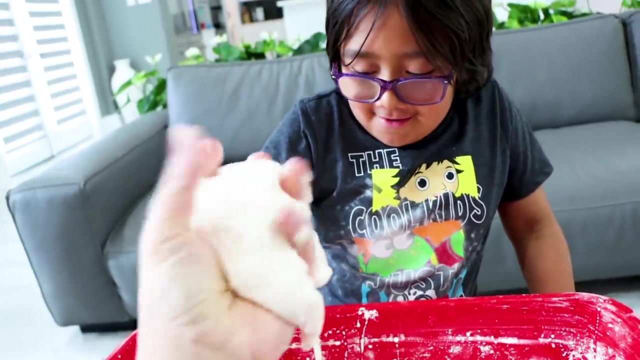 are you guys tasting a little bit hard? but you guys can see, when you pick it up it runs, yeah, but if you punch it it's a solid whoa. you pick up a whole bunch. maybe just squeeze it like this. it's hard like a rock, see, super hard, but if you let it go it just drips like a liquid. 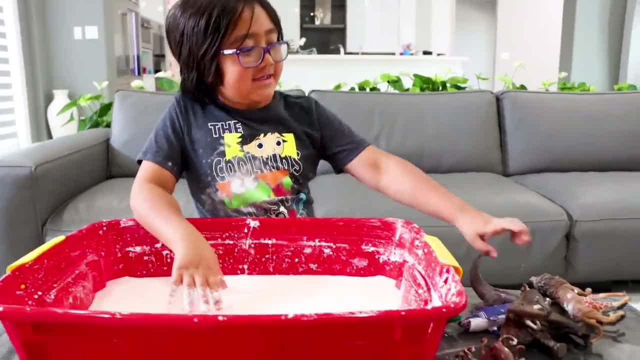 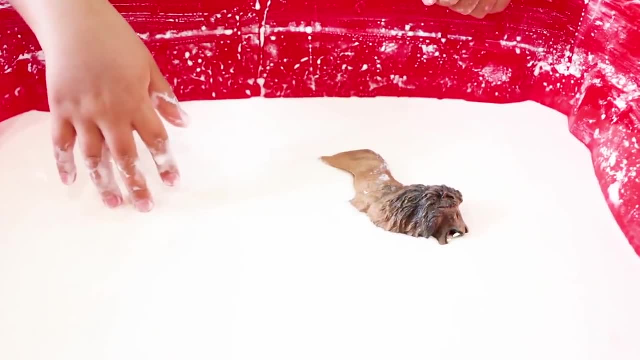 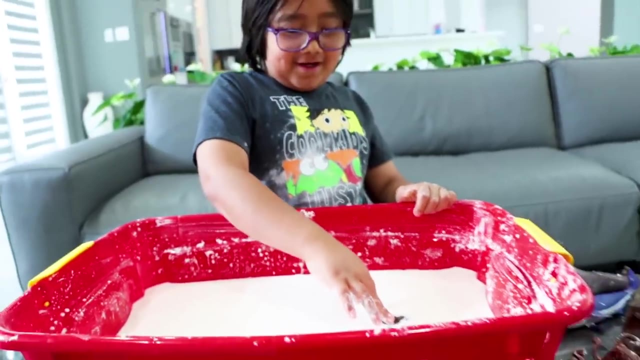 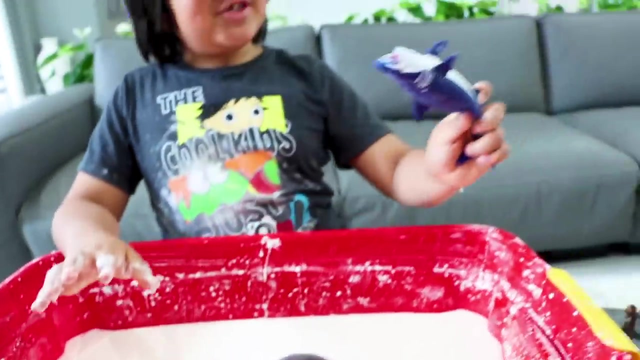 isn't it cool time to bury the toys? goodbye, mr lion. it just sinks like quicksand. we're gonna go down, bye-bye, see you soon, yeah, if we see you soon. bye-bye mr dinosaur, bye-bye shark. he's going down into the water. 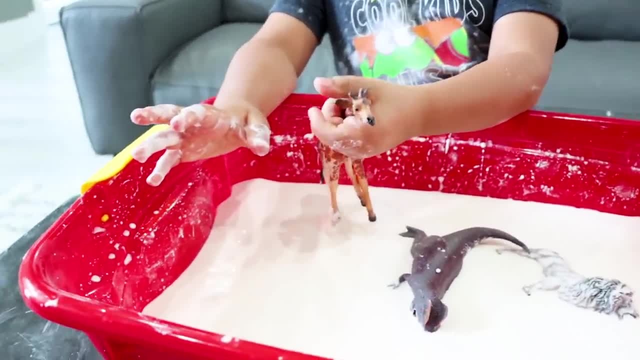 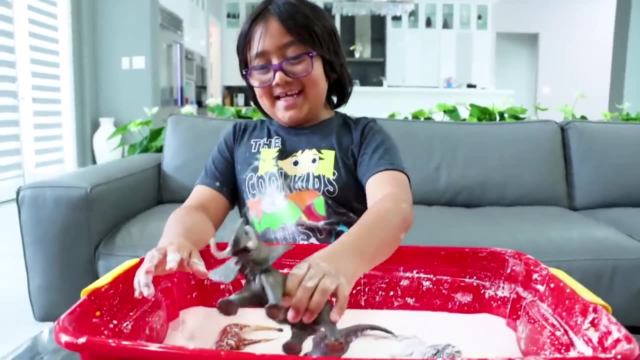 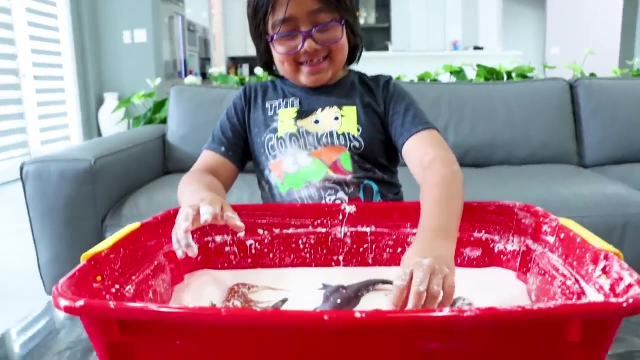 bye-bye mr giraffe. wait, how is this one gonna like go all the way in, like this, i guess? so we should have picked smaller toys. these toys are too big. goodbye mr elephant, goodbye mr octopus, or business, i don't really know. yeah, it could be a girl, could be a boy. 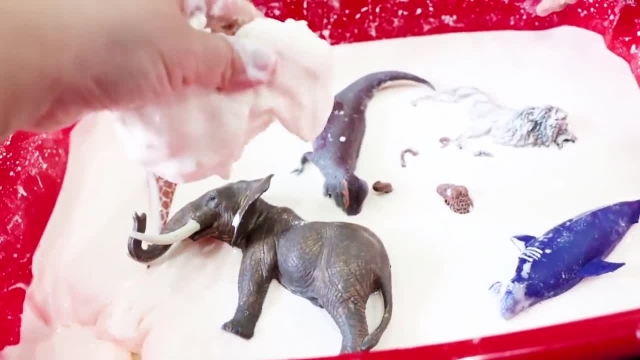 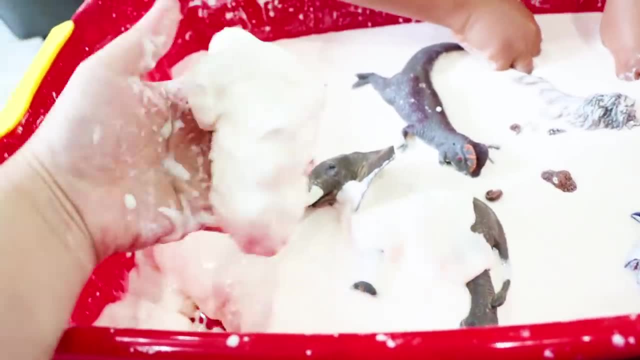 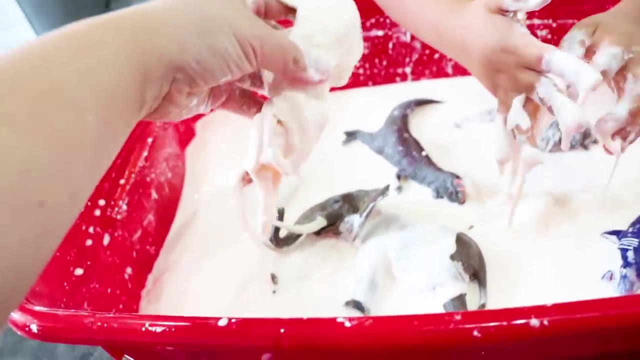 we don't want to assume we're gonna try to bury them the best we could- probably not going to work, but it's fun. it's hard to pick up. huh, wayyyyyybleeeb picking up things with force. Yeah, that's right. 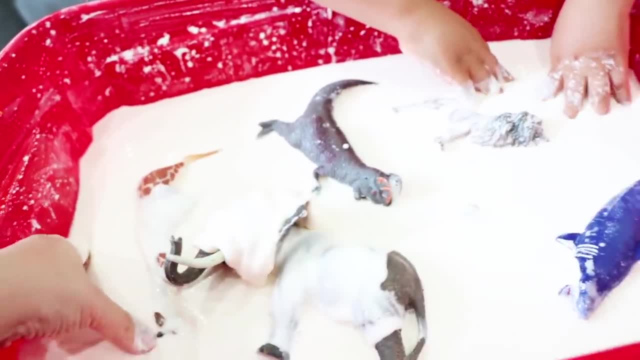 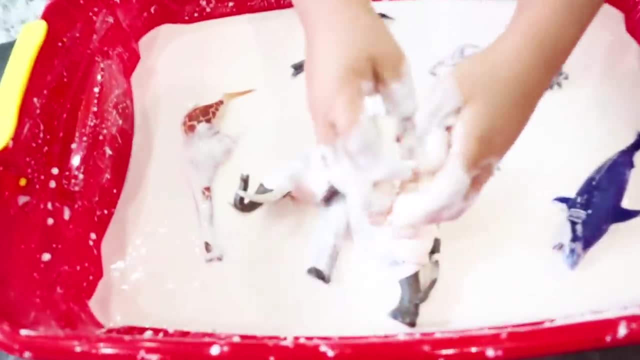 But you're not supposed to use force. Yes, if you use force it becomes a solid, But it's like hard to pick it up, because when you pick it up you have to use force. You're right? Yeah, Elephant. 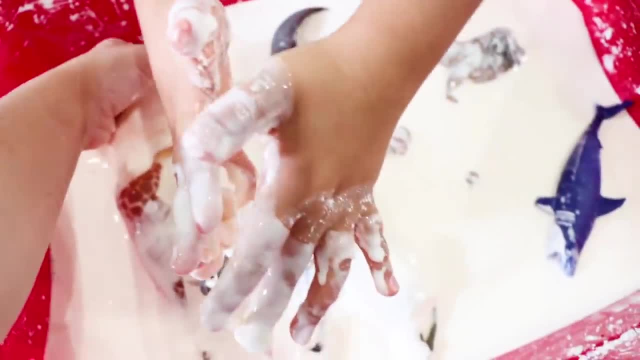 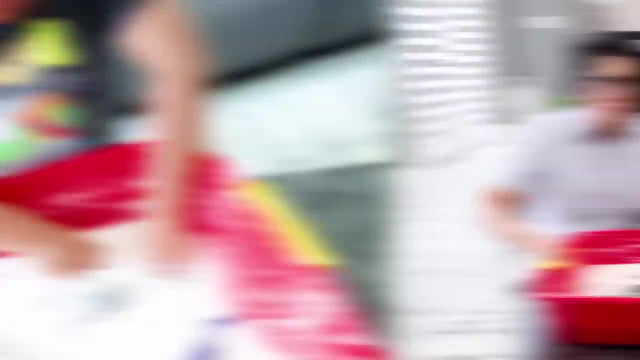 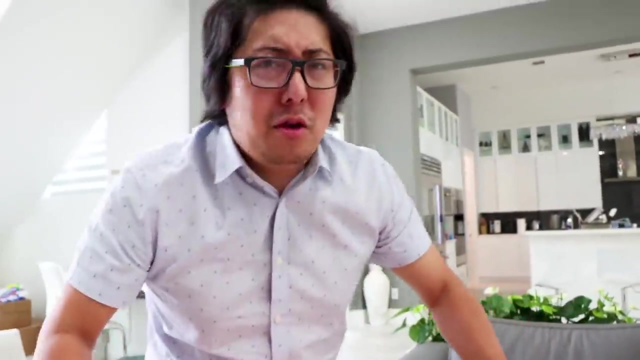 Yay, almost done. Almost got the elephant. Yeah, How are we gonna rescue the animals? That's for you to find out. Okay, now my daddy's gonna bring it outside. I don't know, it looks heavy. Yeah, there's so many animals in here, it's heavy. 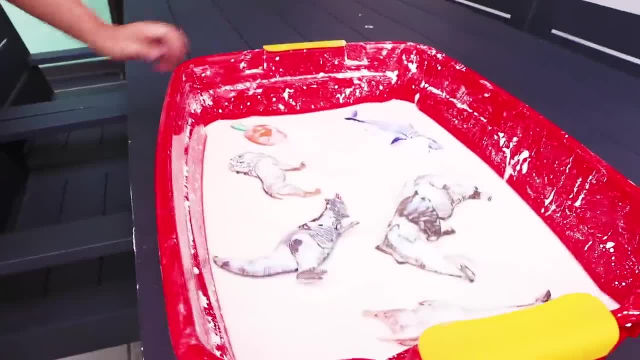 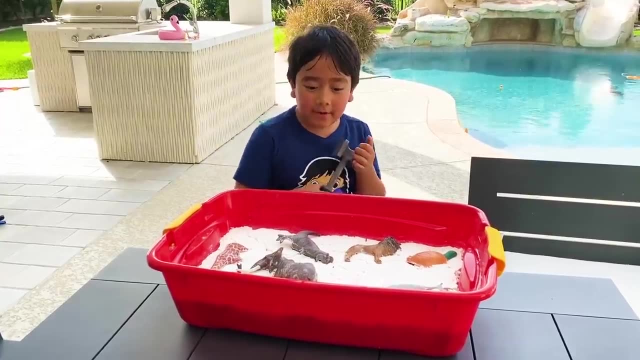 Woo hoo, Okay, guys, we are gonna wait for it to dry, probably in one or two days. See you soon, Okay, guys. so it's been about a month and look at all these animals. it looks so hard. Yeah, you ready to see if you can break them free. 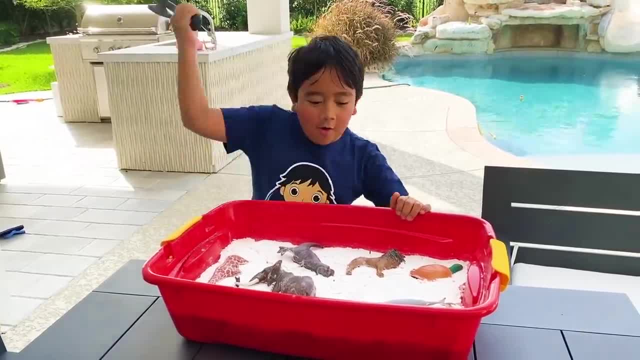 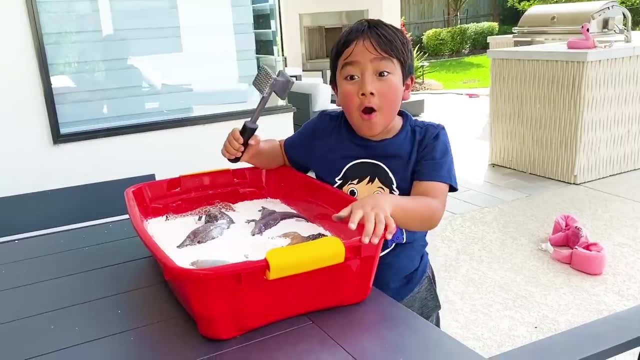 Yeah, Good luck. Okay, three, two, one whoa whoa Did it work. Yeah, But wait, what did we forget? Oh lashes, yeah, That's right, Very important for your eyes. good, 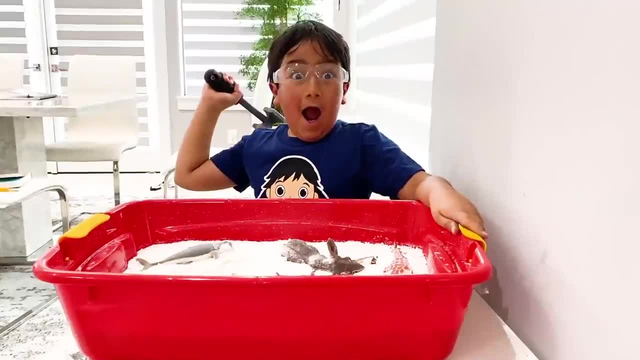 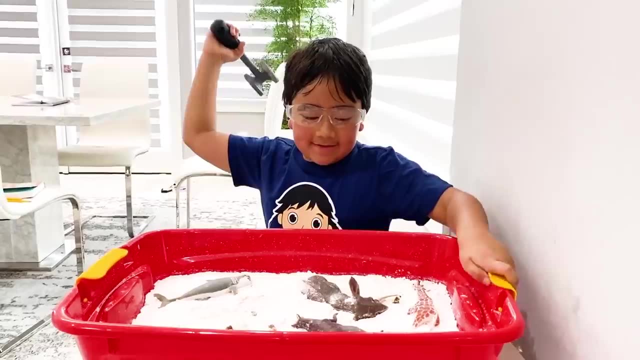 And you know it's kind of hot outside, so we're gonna take it inside, okay. Okay, guys, we're back inside You, ready to get started. Yeah, Yep, and only do this with an adult supervision. Three, two, one. 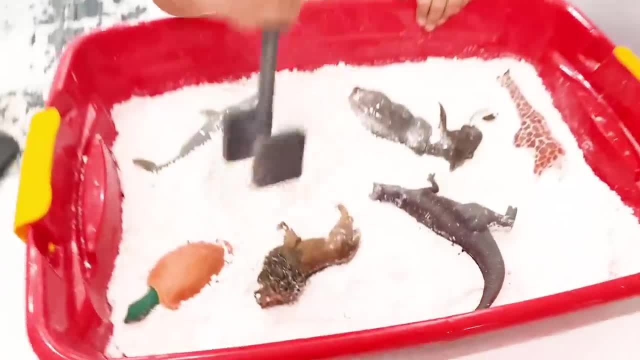 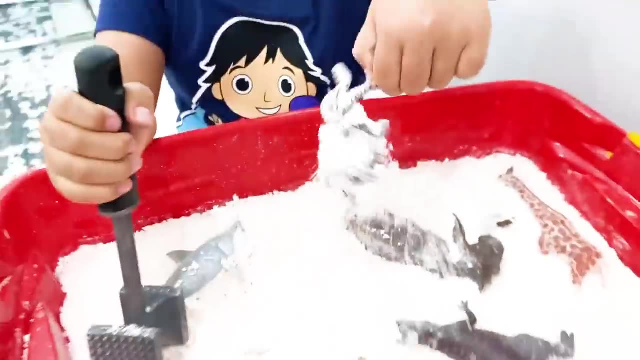 Oh, look, there's somebody tail right there, you see. Oh yeah, Dig site. Yeah, Look a turtle. Oh, it looks like a turtle. What is that? Ooh, Do you remember that animal? What is it? 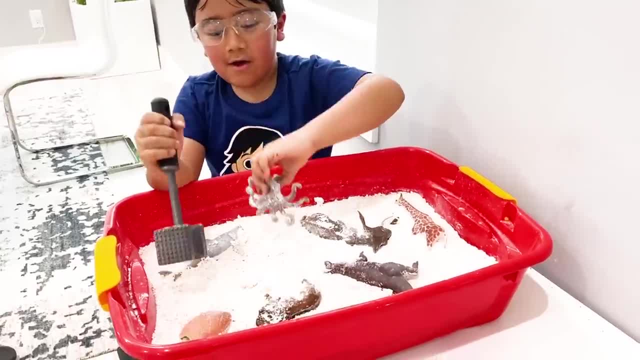 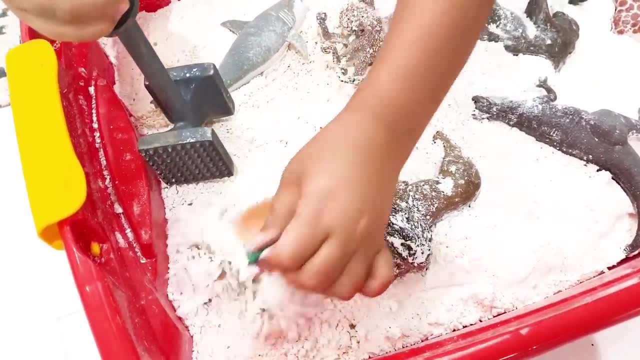 I don't get it. Octopus, Hi octopus. Oh turtle, you wanna get out turtle? I can already pull it out. Woohoo, nice Turtle. Okay, and then we have a few more left. Yay, elephant. 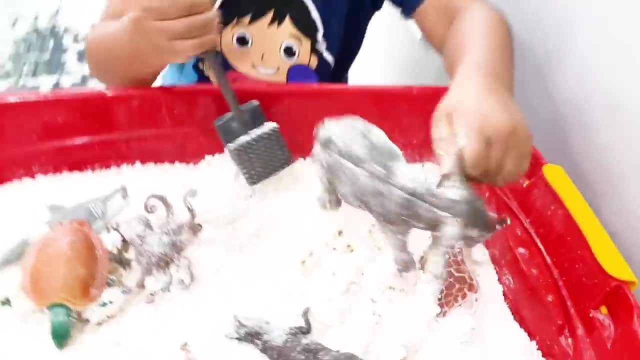 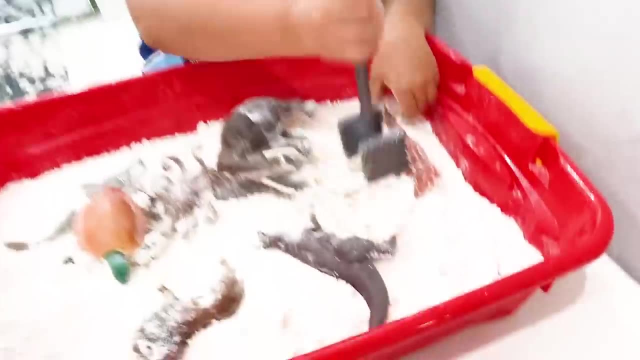 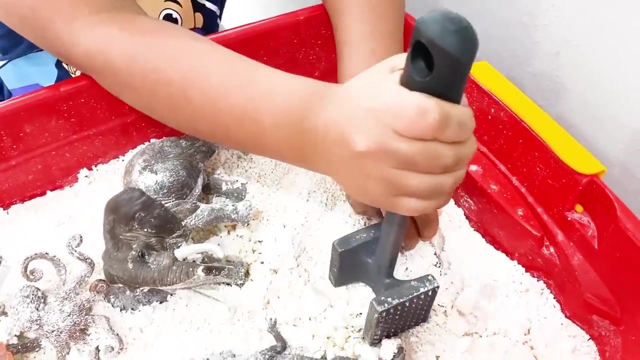 Whoa nice. Oh, look at this. Look at this. Thank you, Ryan. What about me, Mr Giraffe? I'm stuck. Can you help me out? I got the giraffe out, Yay Ooh. 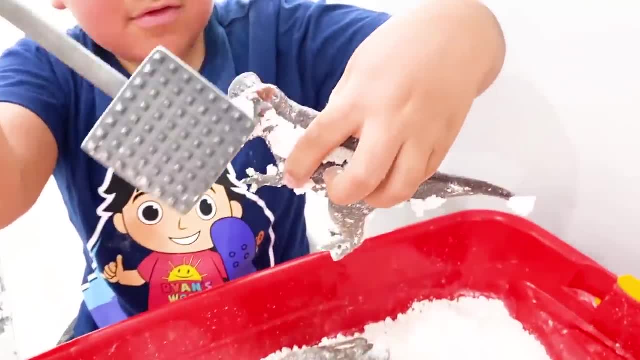 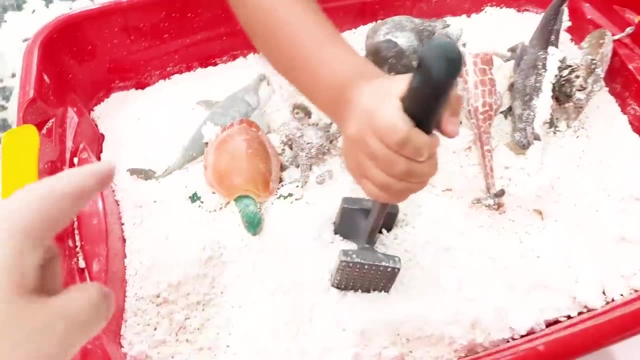 Who is that Dinosaur? Hi, Mr Dinosaur. Okay, I think we have one left. Ryan, Mr King of the Jungle. Yeah, I think we missed Mr Sharky here. Oh yeah, Help me, Ryan. 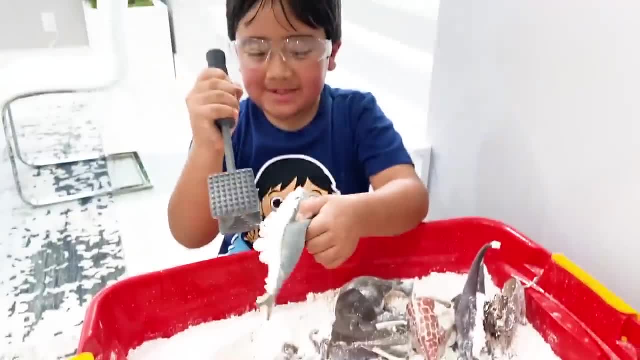 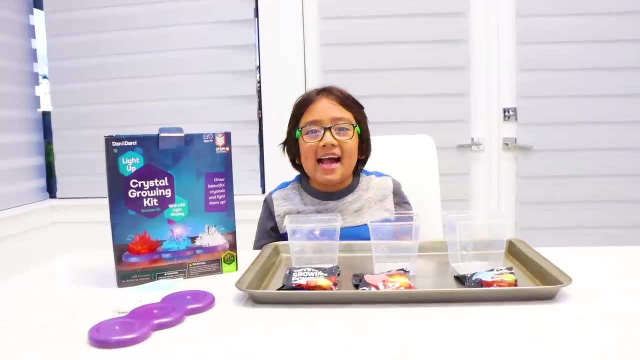 Save me, Save me. There's so much on Mr Sharky, I know, Yay, I saved everybody. Yay, Hi guys, Today I bought a crystal growing kit and we're going to grow crystals. Yay. 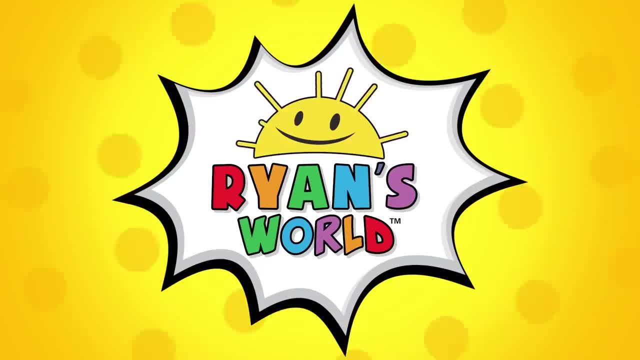 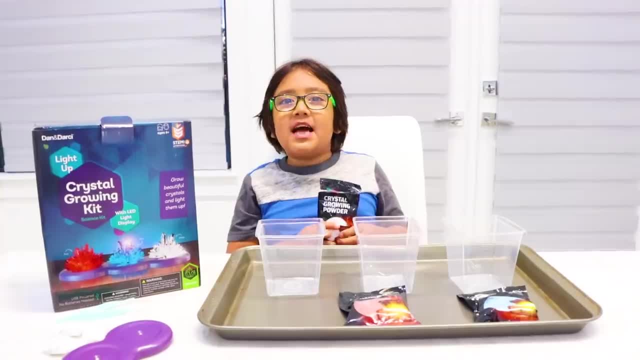 Welcome to Ryan's World. Did you know the most common crystals are salt and sugar. First up, the crystal powder. First we're going to do white, Next is red, Last is blue. Next up: you have to ask a parent for help. 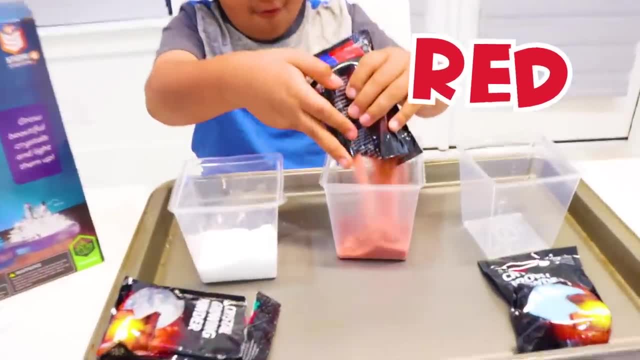 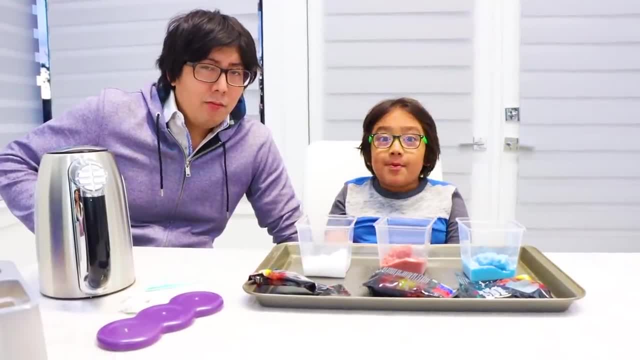 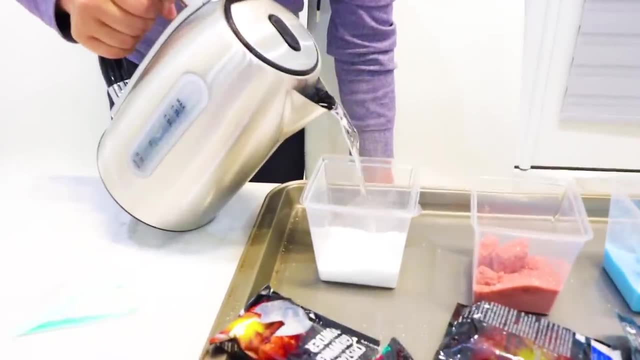 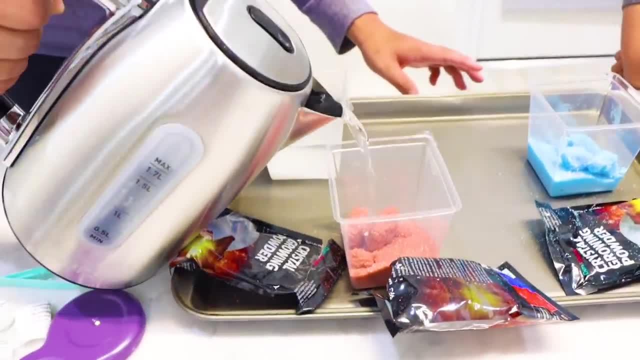 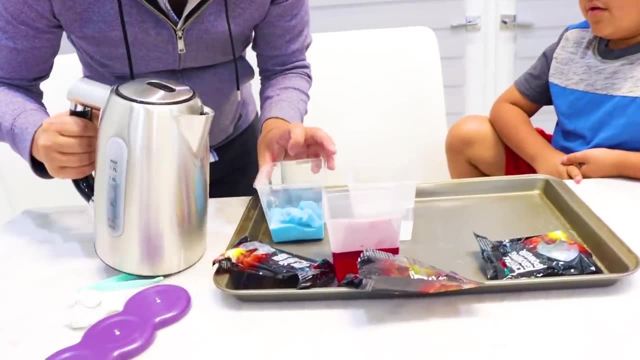 It's hot, It's hot, It's hot. You see the steam coming out. Whoa, I love the color. Look at it. Last one, Make sure you don't touch it. Thank you, Daddy, You're welcome. 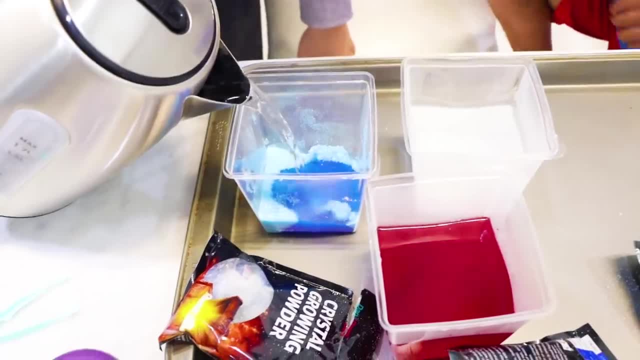 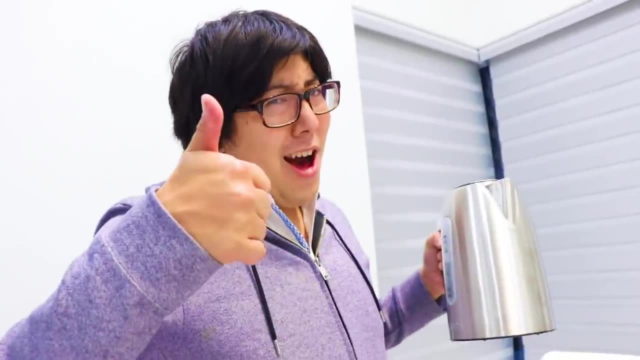 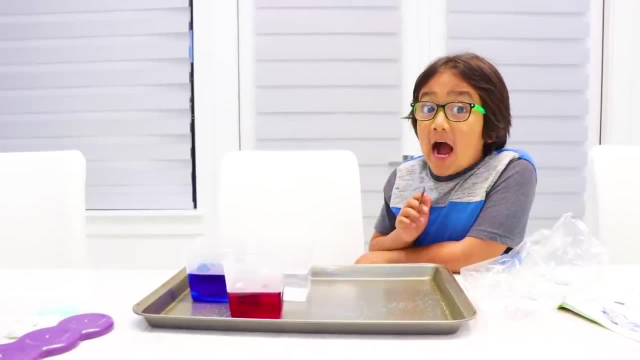 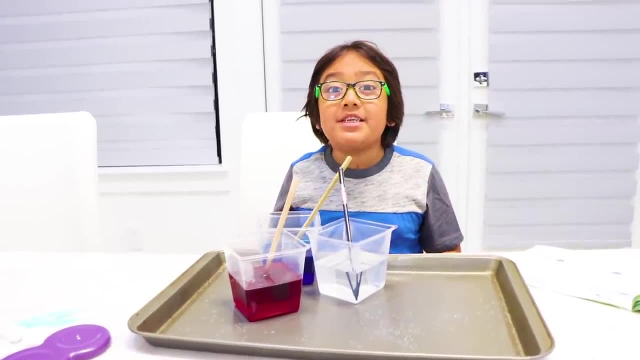 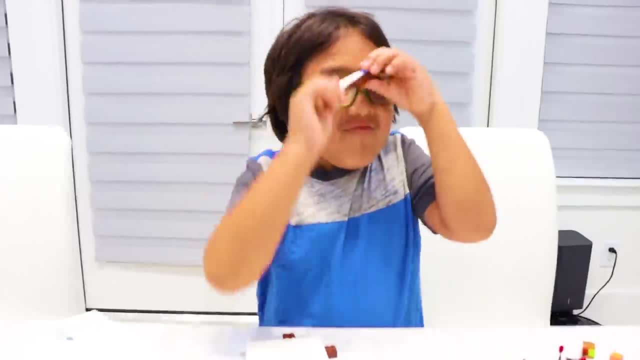 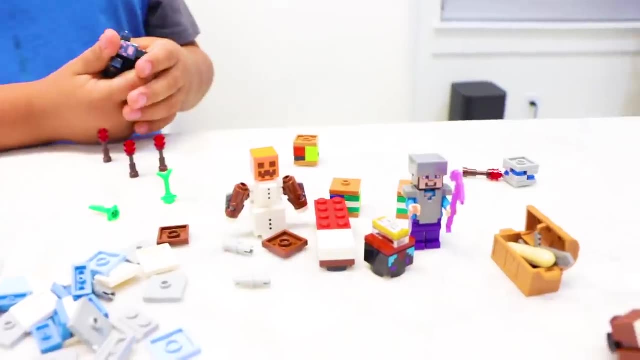 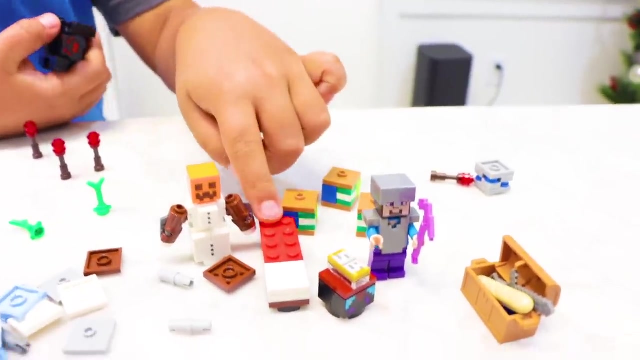 Now we gotta wait 10 minutes and I'm going to play with LEGOs. If you guys are curious, I'm building Minecraft. These are all the things I made so far. This is a snow golem, and these are bookshelves, and this is a bed and this is an enchanting 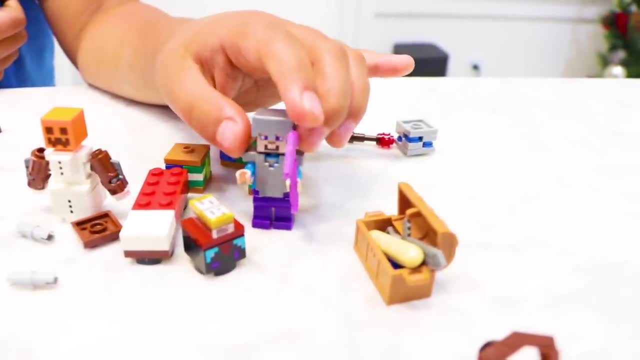 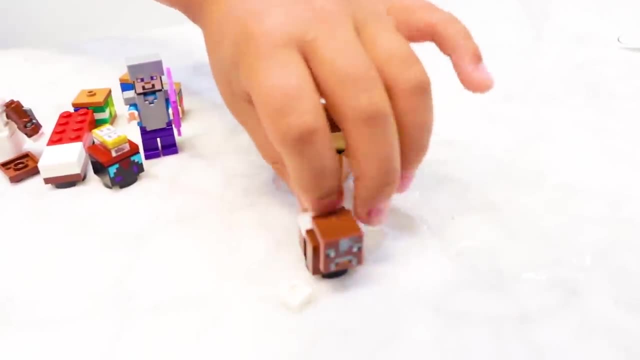 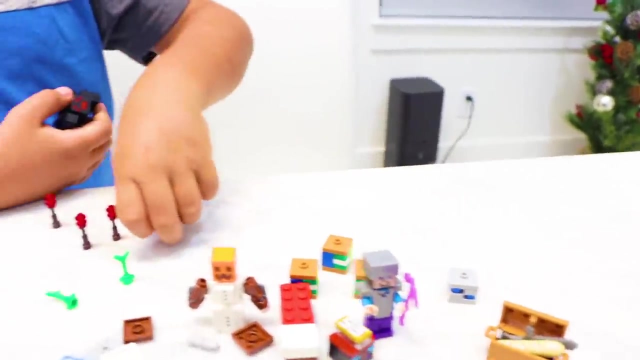 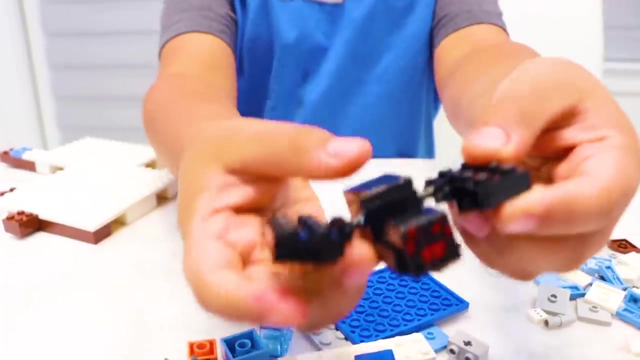 table. This is Steve with a racehorse obsidian pickaxe and this is a hidden treasure chest, and this is a cow and this is probably an anvil. I don't really know what that is. And these four things are torches, and I don't know what these are. And here's my favorite: spider Waddup. 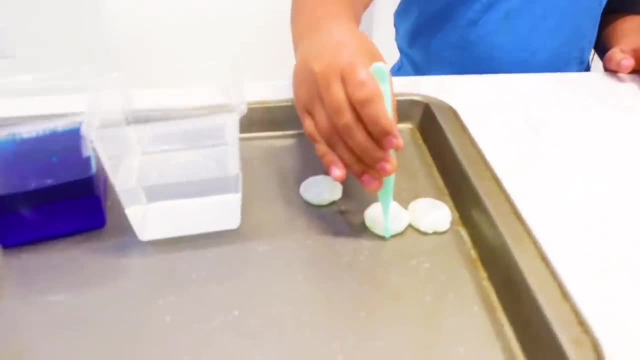 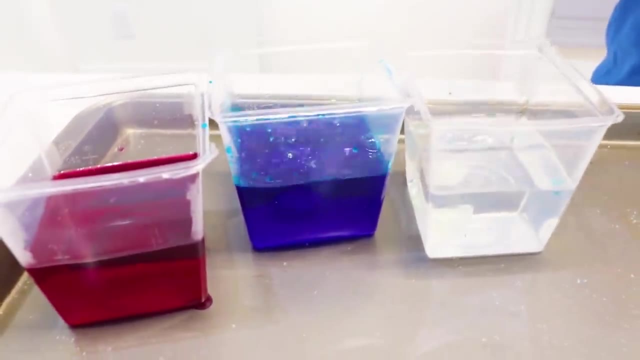 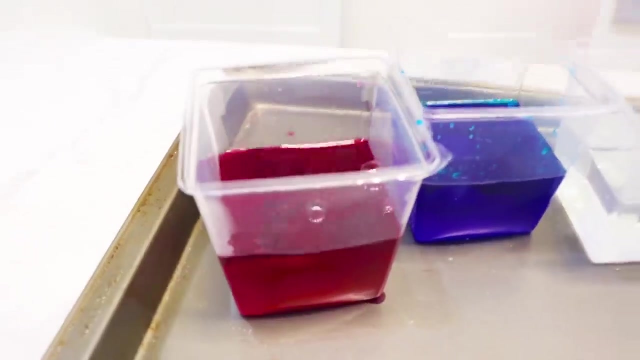 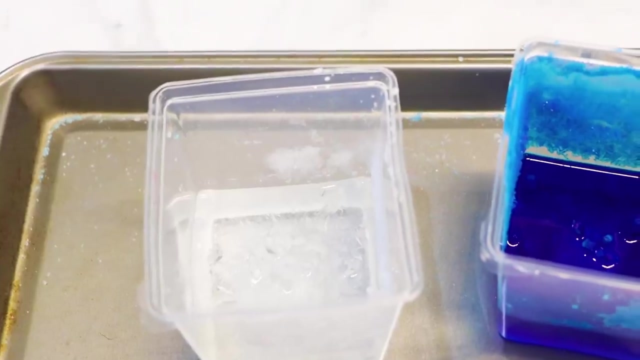 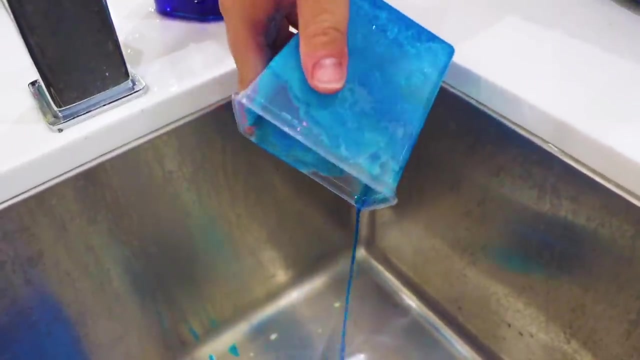 Now we gotta put in the crystal starters. Now we just have to wait and see our crystal grow. Guys, it's been a whole week And look what happened. you can see the crystals inside. Let's pour out the white crystal. Now let's pour out the blue crystal. 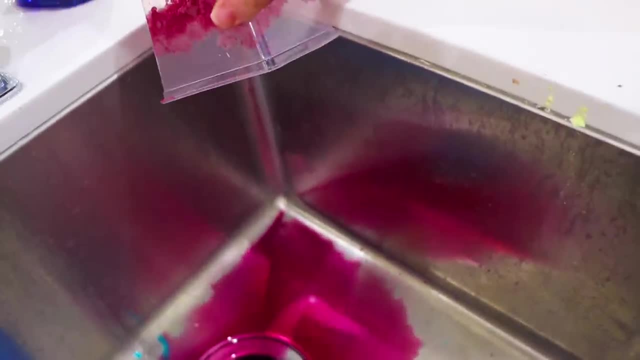 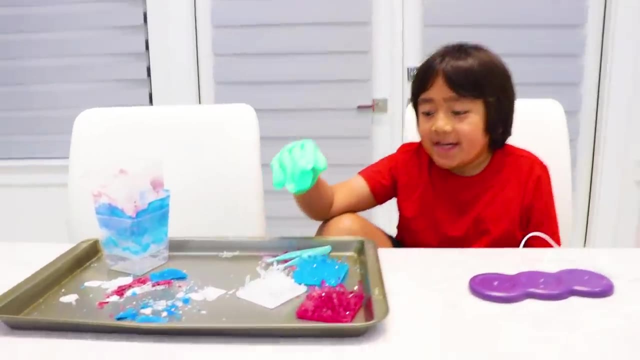 Now let's pour out the red crystal. Whoa, the water looks so cool. Wow, it looks so cool, But now I need to wait eight hours for it to dry. I took out the crystals. Here's what it looks like. 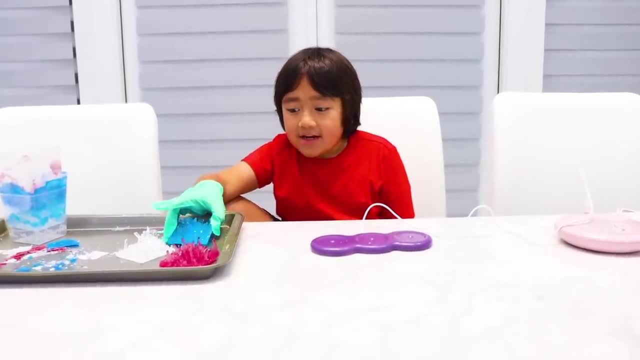 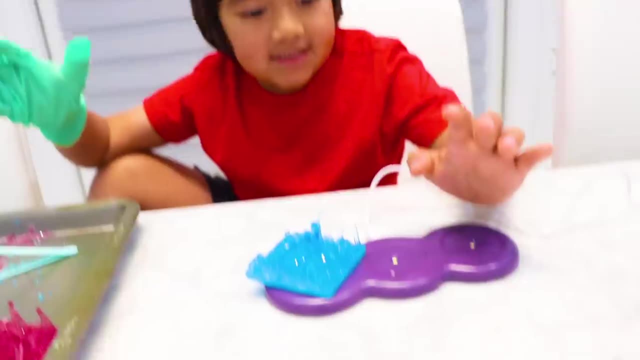 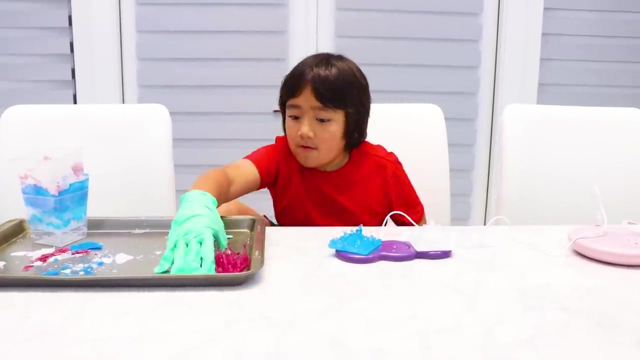 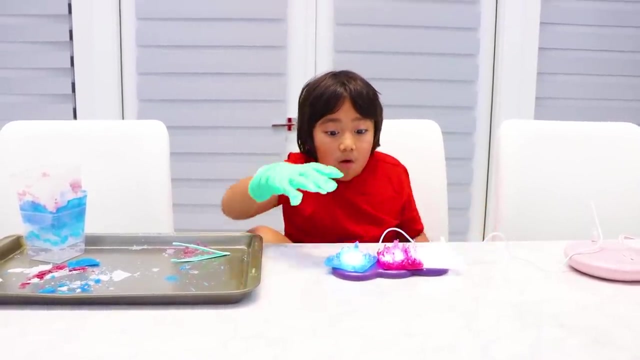 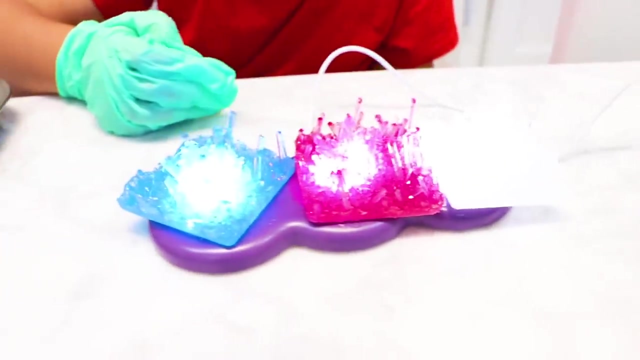 It comes with a display case And I can put these crystals on the light So you can turn them on like this. Oh, that looks so cool. Good job. It took us about one week to make the crystals. Hi guys. 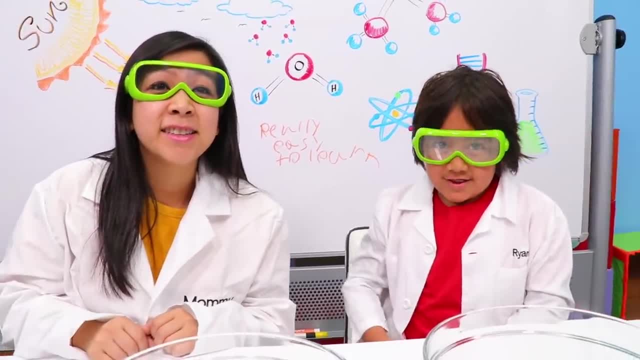 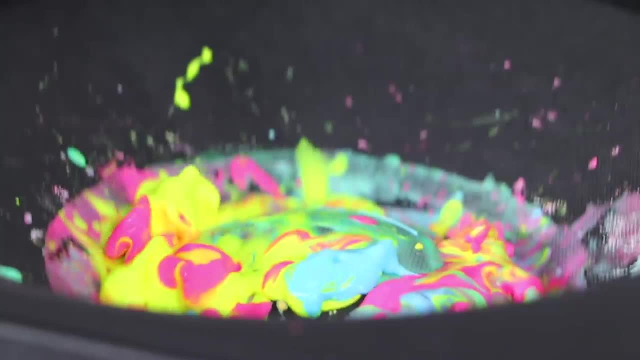 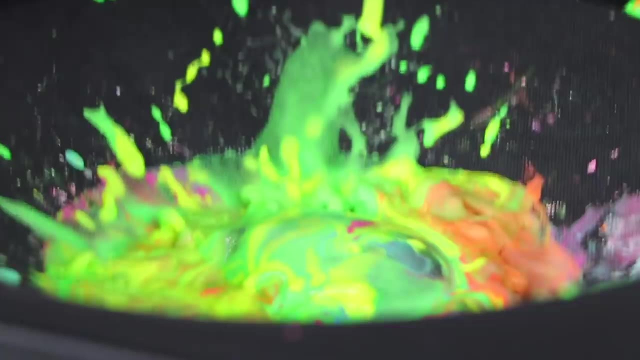 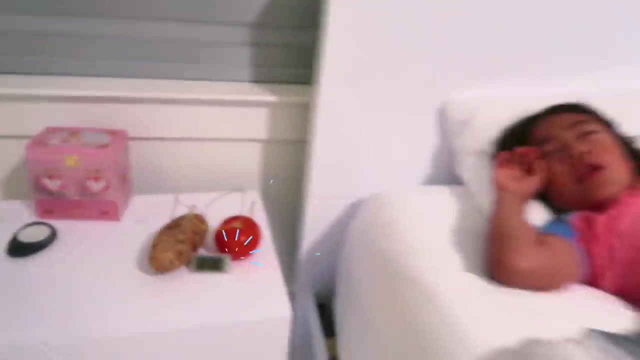 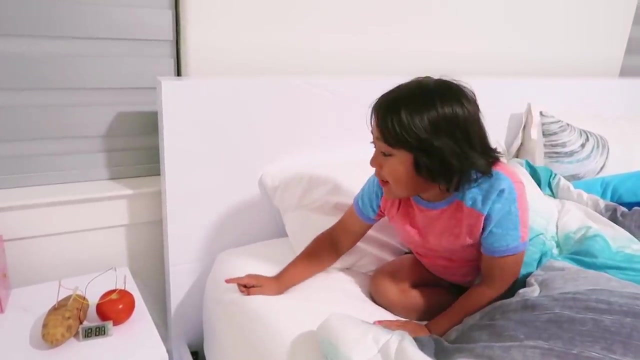 Today, we're going to make oobleck And once we're done, we're going to make it vibrate like this: Oh, hi guys, This is my fruit and vegetable alarm clock. It helps me wake up, And I'm going to show you how to make one on your own. 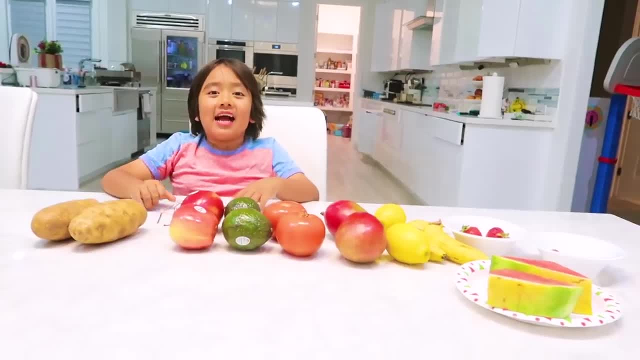 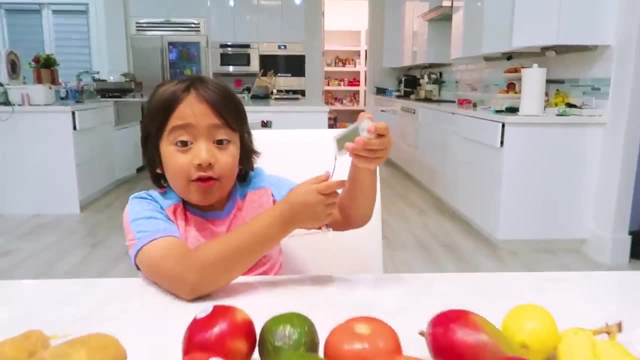 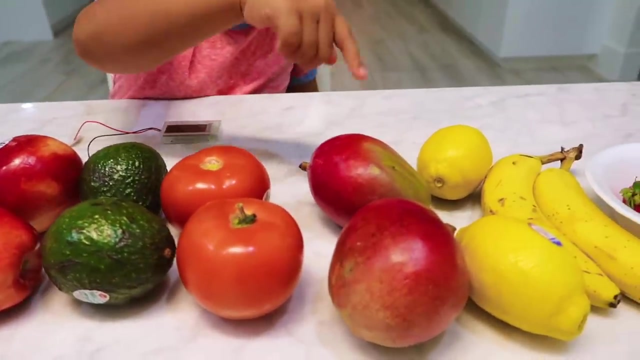 Let me show you how to make your own alarm clock. Let's go, Hi guys. So today we're going to be using 10 different vegetables or fruits And we're going to see if they can power this alarm clock. So we have potatoes, apples, avocados, tomatoes, mangoes, lemons, bananas. 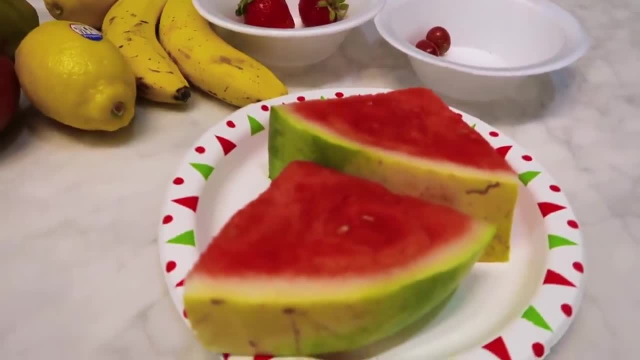 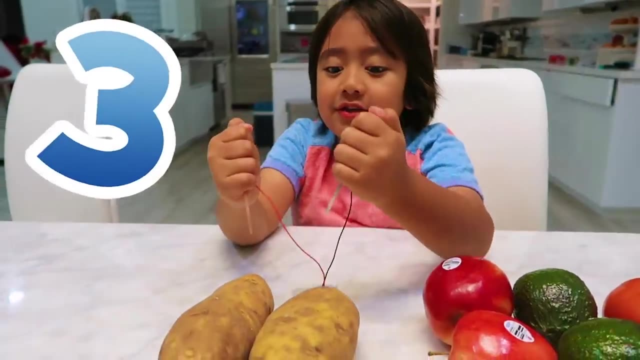 strawberries, grapes and watermelons. First we're going to try the classic potato. It was made for potatoes, so I think it's going to work. Three, two, one. So if you notice here, look at the alarm clock. 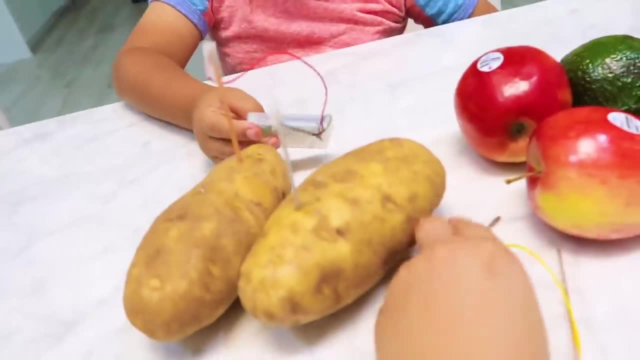 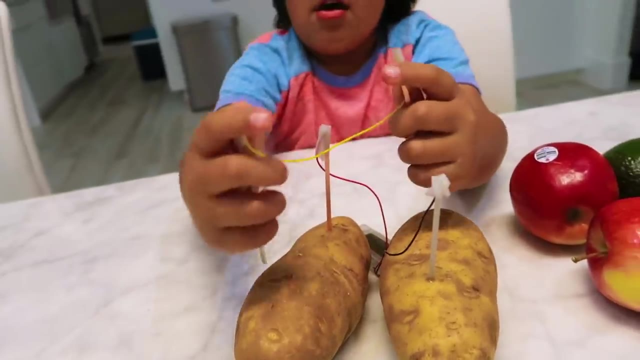 Is it working yet? Not yet. We got this kit online, So it comes with a magnesium wire and a copper wire. You have to connect this to it. This Uh-huh Hi, Yeah, And here, All right, You tell me. 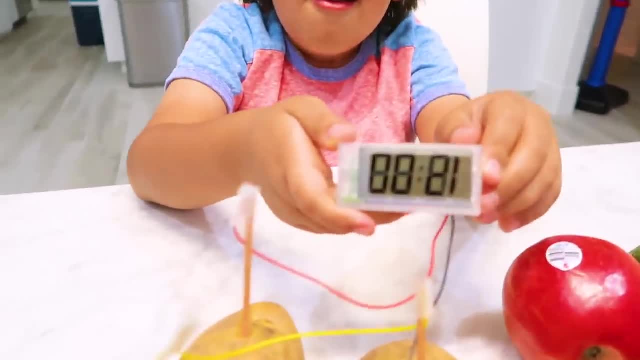 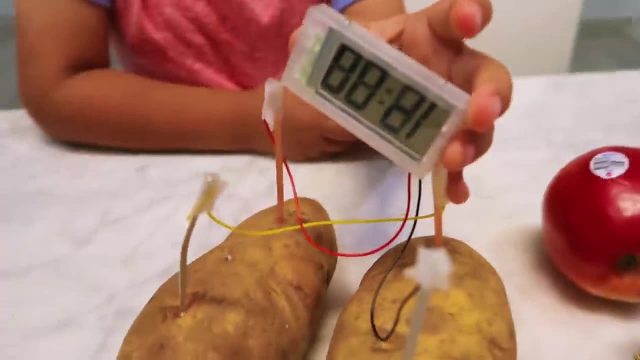 Is the alarm clock working? Look it's working. Yeah, it turns on. It's got enough energy? Yeah, so we have to manually set it. But you know, there it is A potato works. I'm going to use a potato. 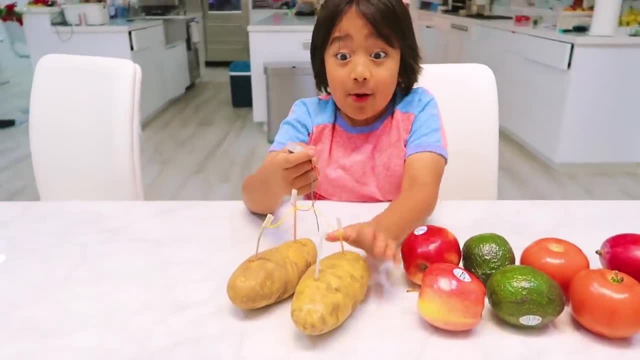 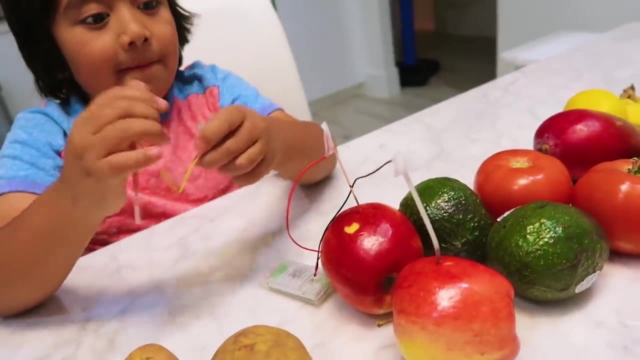 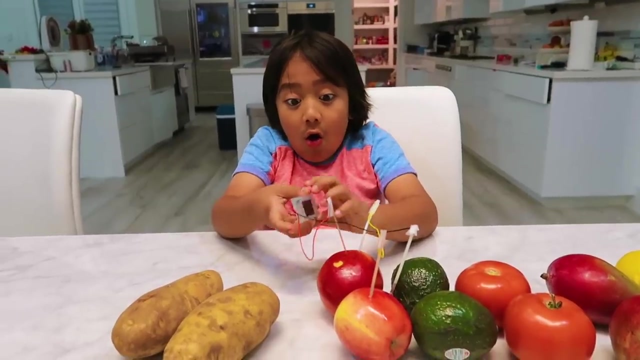 For my alarm clock tonight. Okay, now let's try the next one. Next, I'm going to test out the apple And do the opposite on the other one. Yes, like up here. There you go, Moment of truth. Does it work? 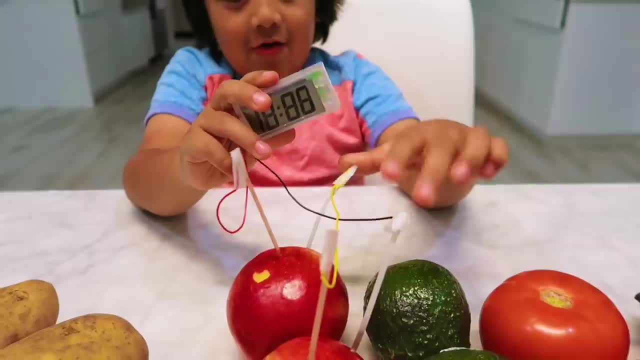 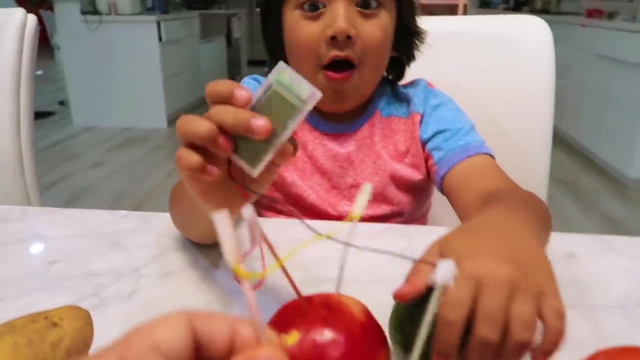 It works. Yay, So an apple can also power it on. You know, it's true, because look what happened when I take out one. Okay, if I take out one, it stopped working, But if I plug it back in, Whoa. 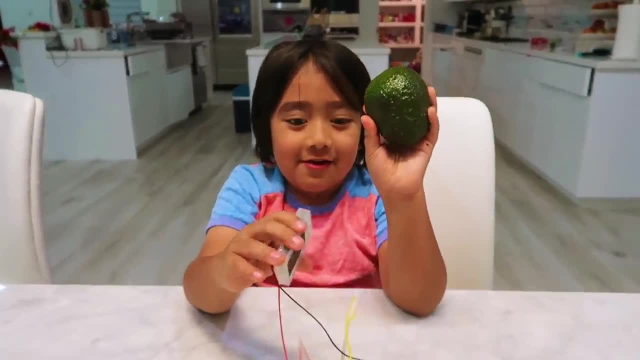 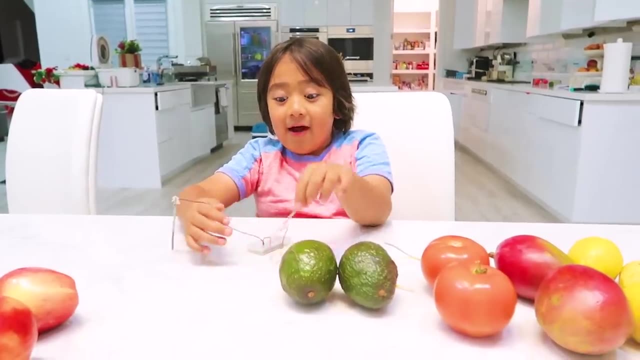 It works. I'm really interested for this one, The avocado. Yeah, Guys, let us know if you think avocado can power on the alarm clock. Now we're going to try the avocado. What? Oh, I think it's going to work. 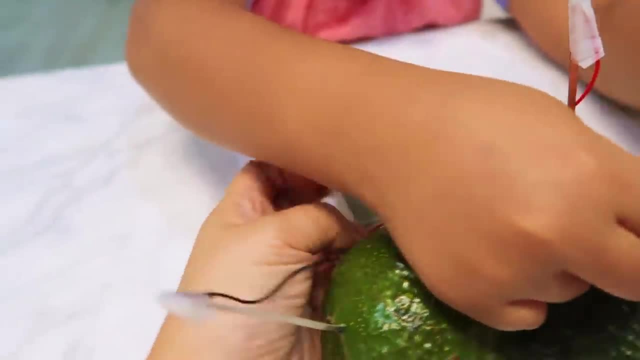 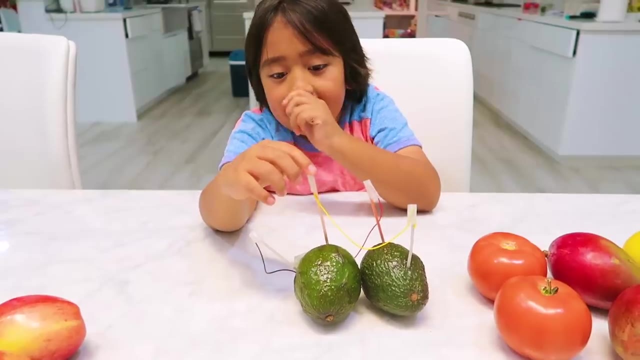 You think so. Yeah, You guys notice right now nothing's on right, So it doesn't work right now. So Ryan's going to put it in. Can you use an avocado alarm clock tonight? Wait, isn't that so? 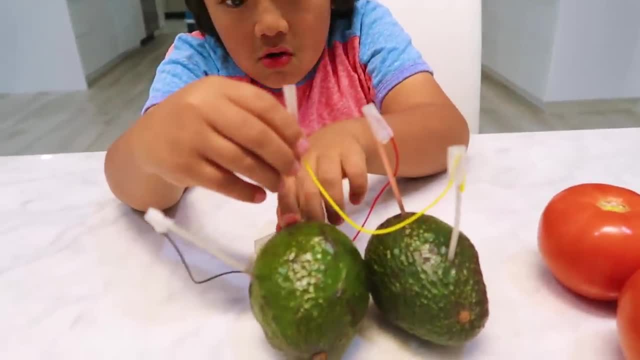 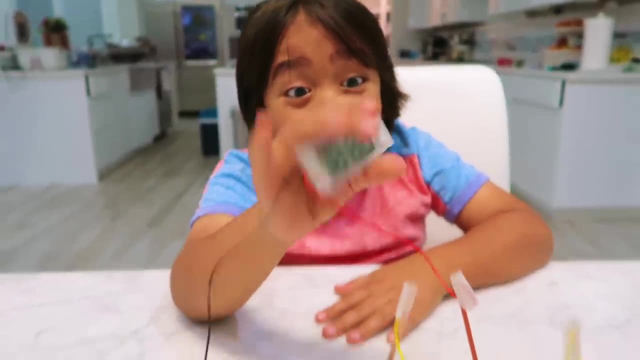 I know What You're supposed to put this. No, that's right. Yeah, it's supposed to be opposite. Uh-huh, You need that to complete a circuit. Does it work? Avocado work, Whoa. Now the most interesting one is one. 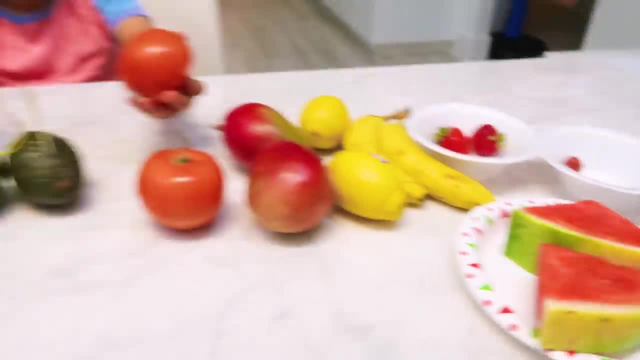 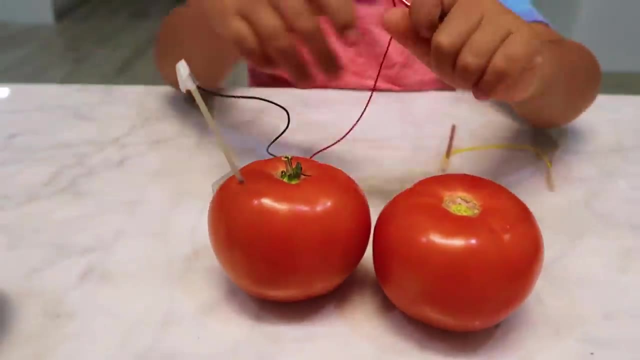 That's true, That one we're not sure. I want tomato. Wait, no, I think tomato will work. Tomato will work. Okay, let's see. Now we're going to try tomatoes. They're really messy. Don't poke it too hard. 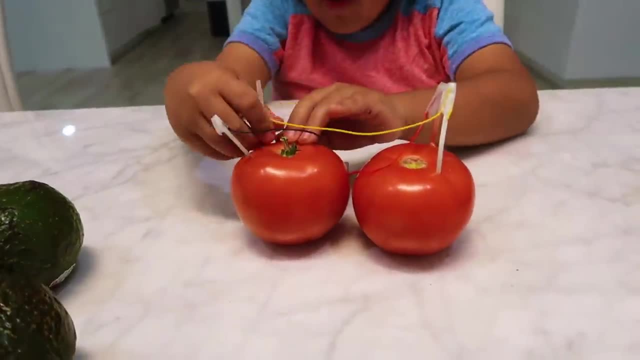 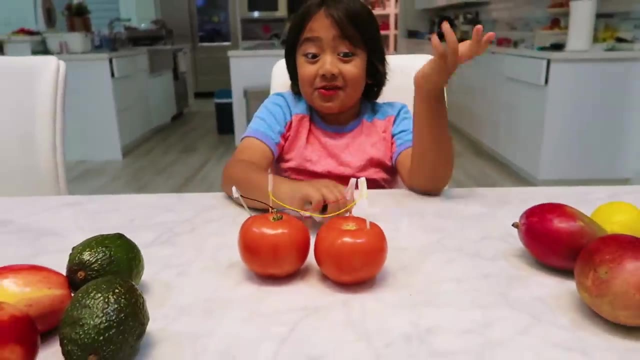 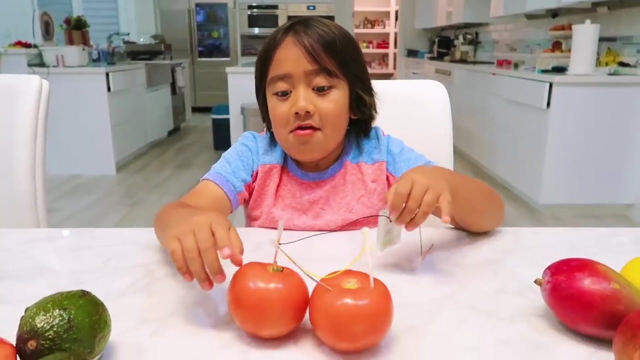 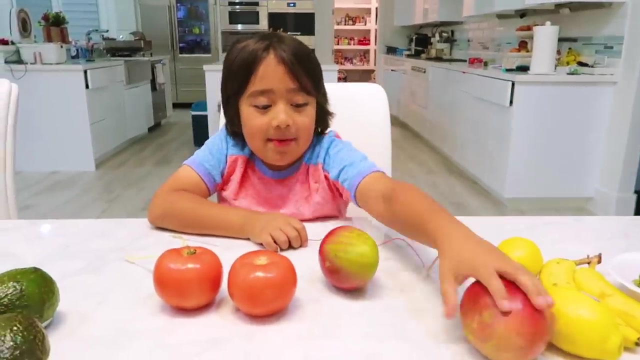 And like this: Does it work? It works, It does work. Wow, Maybe we do need just fruits and vegetables Power alarm clocks. You think fruits and vegetables can power on your iPad? That's a fun experiment to do later. Okay, now let's try mango. 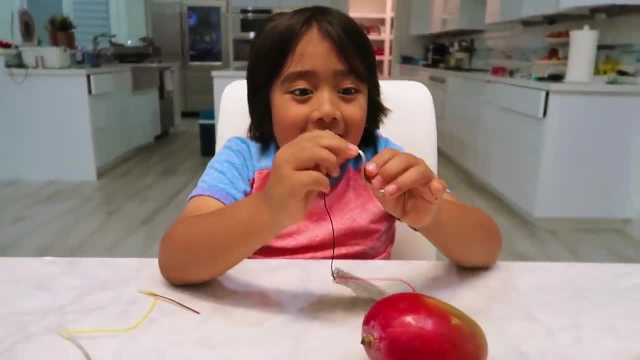 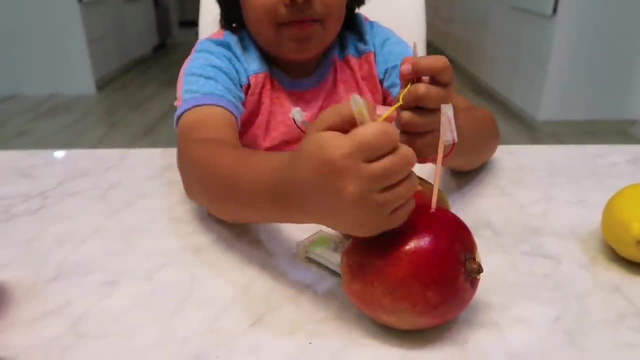 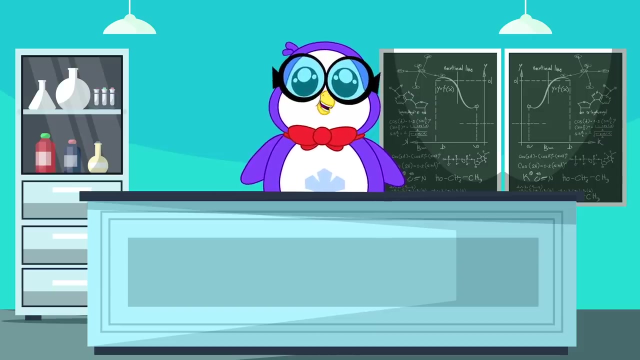 It's bending the wire Here And then one, So you need the other part to make like a circle. You have to complete the circuit. That's why you need it. Actually, the potato clock works by converting chemical energy into electrical energy. 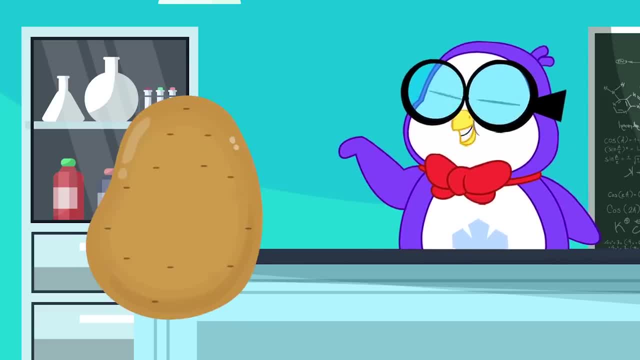 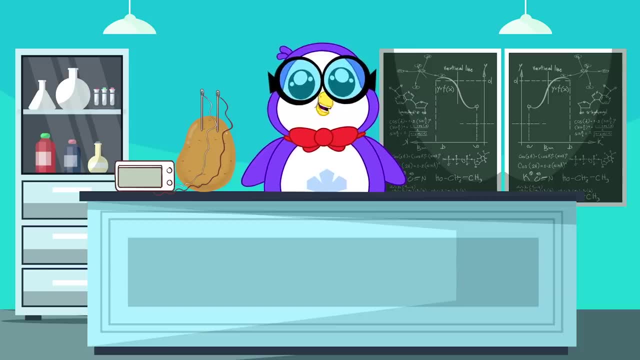 Did you know that the energy doesn't actually come from the potato, But rather the energy comes from the metal dissolving inside the potato? The energy made from the reaction moves to the copper strip, down the wire and into the clock, making the clock turn on. 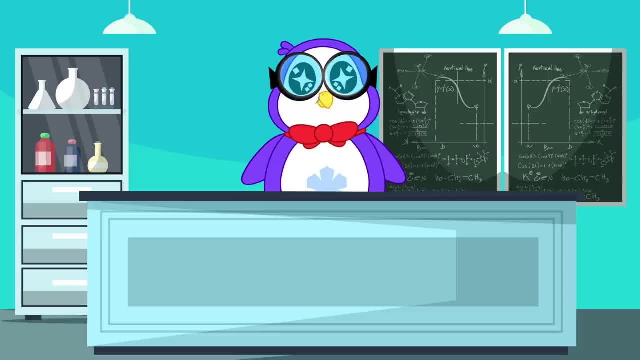 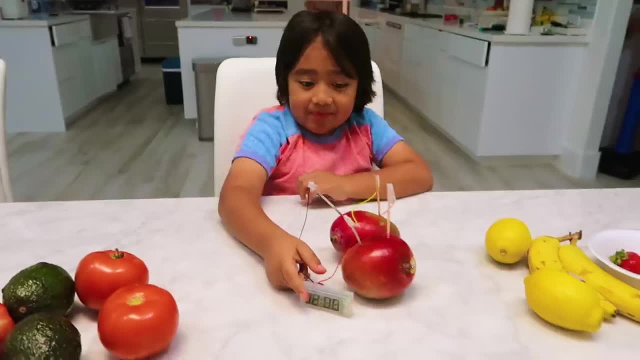 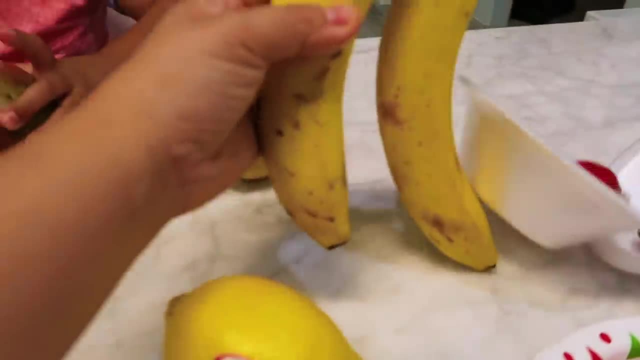 That's spectacular. There you go, Yeah, Wow, everything worked so far. Look, Yeah, Which one do you want to try next? I want to try the banana. The banana. Wow, that's interesting, I think it'll work. 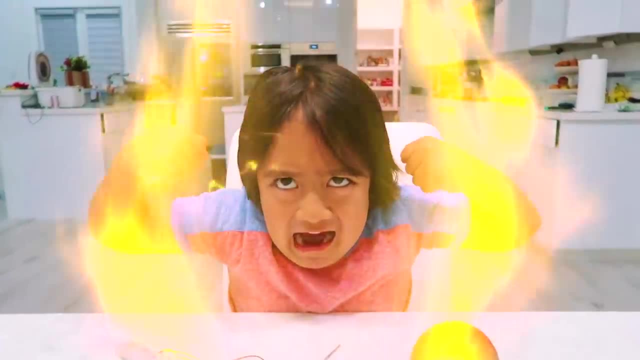 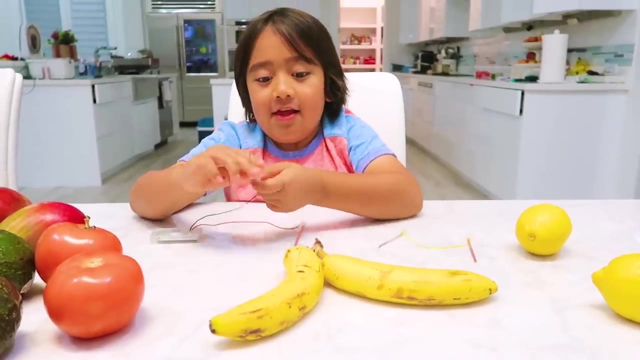 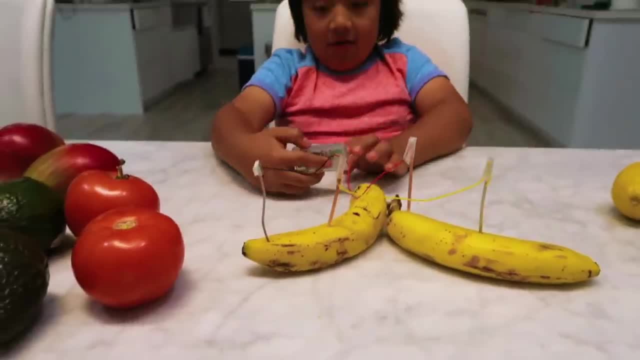 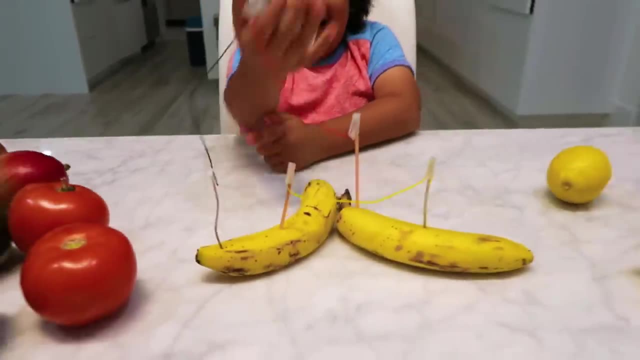 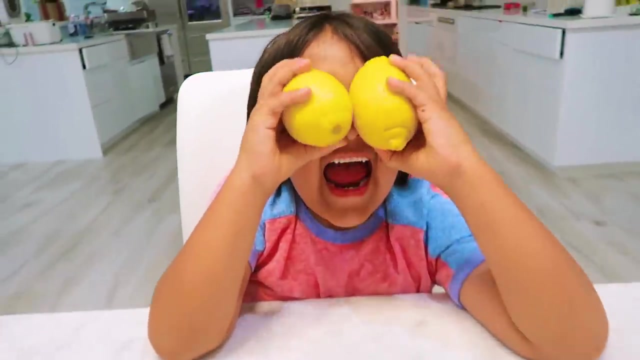 Well, I'll put it here. Yeah, Put it anywhere you like, Well, Enjoying a different time, but yeah, Oh, it does work. Yay, You have a banana clock. Now let's try. What do you think, Ryan? 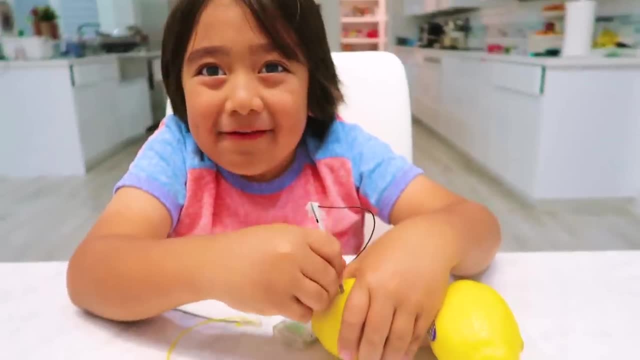 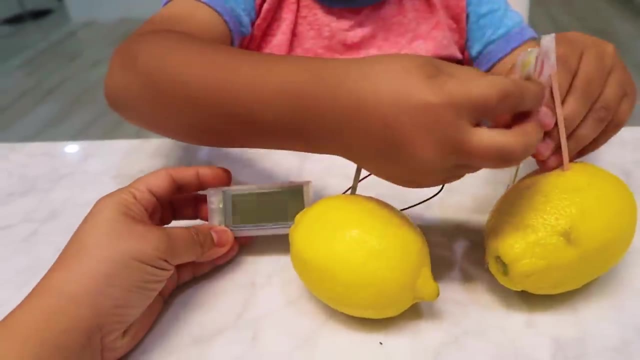 The lemon's going to work? Yeah, I think so. Oh, yeah, it's going to work. It's hard to poke in. Jamie has a smell. See, right now it is not on you guys. Three, two, one. 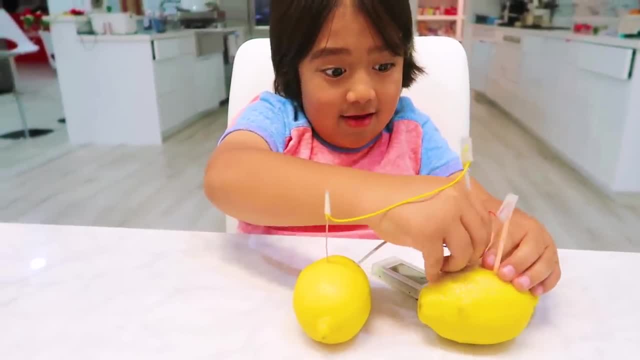 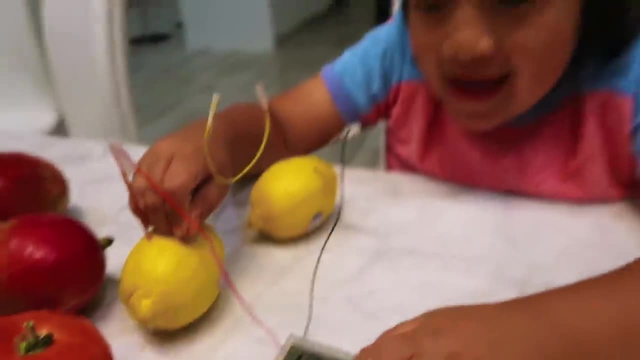 What do you think it's going to do? work or not? Definitely work. I don't even have to poke it in. What That's crazy. So I guess you don't really need a lot of power. So so far, everything works so far. 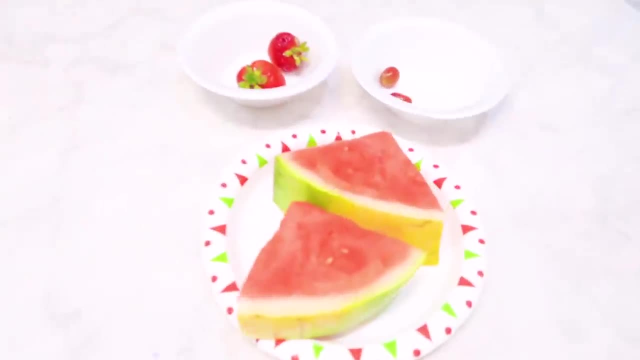 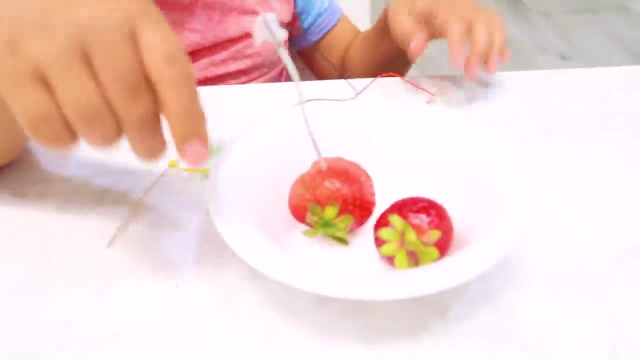 Oh, Which one do you want to try next? These three I'm very interested in. Yeah, I'm going to try this one, The strawberry Strawberry. You barely have to poke this in. to poke it in, I'm going to see if we can do the same thing we did with the lemon. 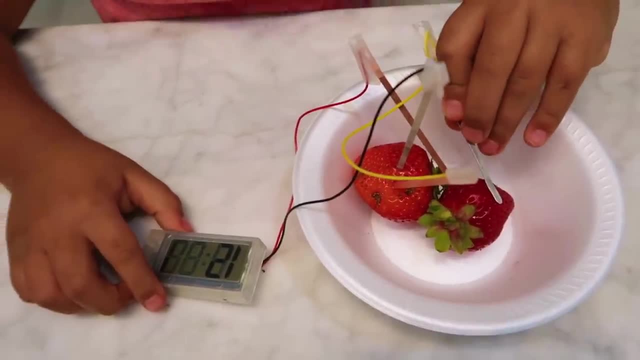 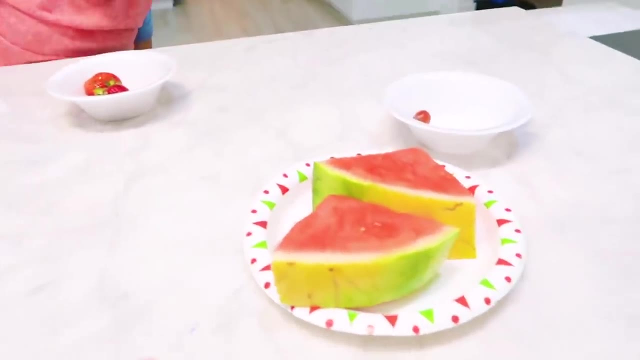 Oh, good idea. Look, Look at it. Wow, very cool. Which one do you want to do on here, grapes or watermelon? Watermelon, Okay, because grapes it's so small I know, Is it going to work. 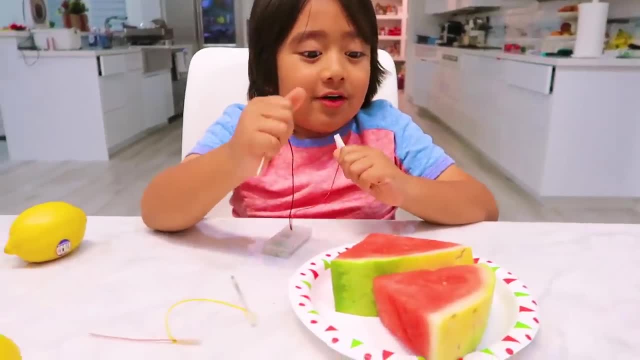 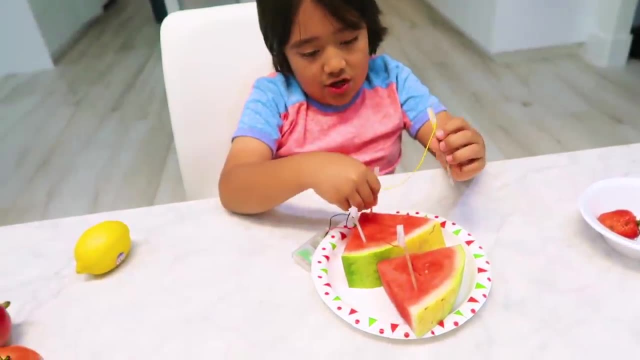 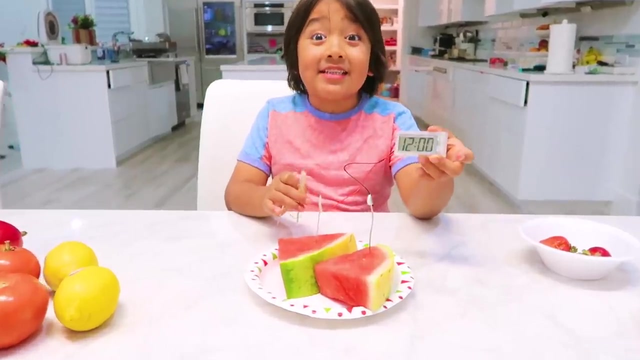 Because it's so tiny. Do you think watermelon's going to work? Let's see, Okay, Oh, it's so easy to poke in. Is it working? What Guys? I didn't even need to complete the circuit, It just powers off with two. 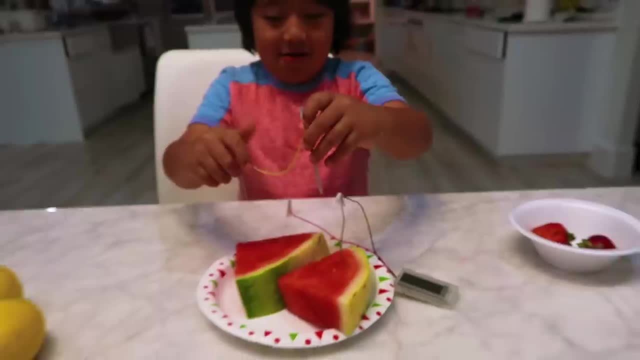 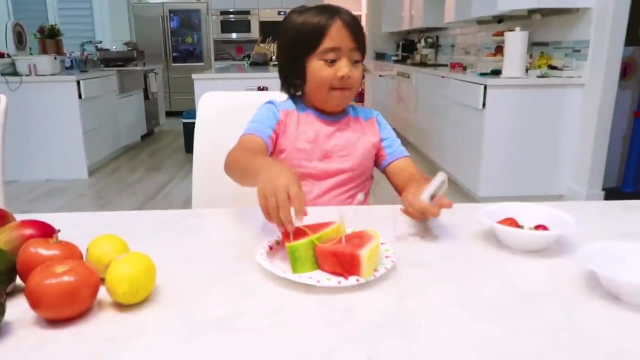 Wow, I didn't know watermelon's so powerful. Well look, But this makes it a lot more powerful, So it does work. Yay, Let's try the last one, The last one In the most. Wait, how is this going to work? 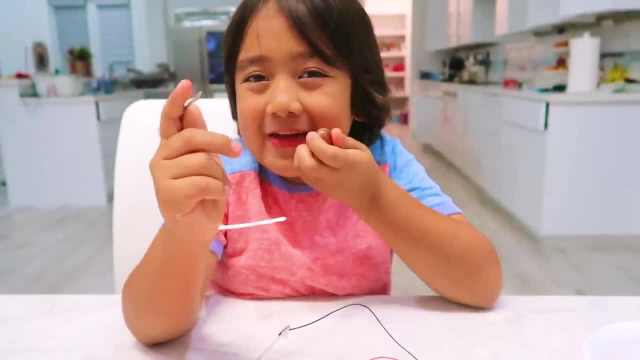 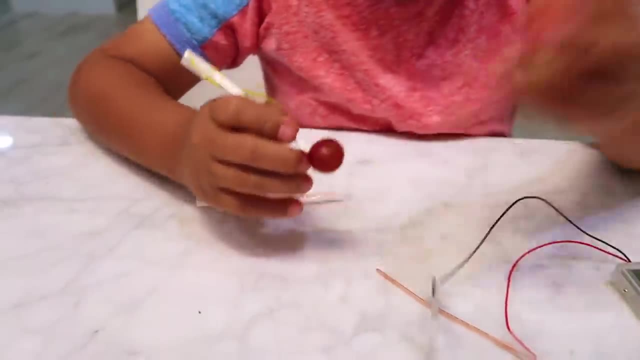 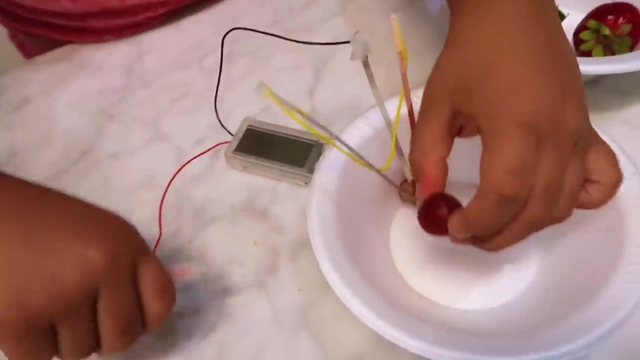 I don't know. It's so small. How are we going to make it opposite and positive? You have to stick them very gently, Can you do it? Yeah, I did one, Now I do the other one. Okay, so far it's not working. 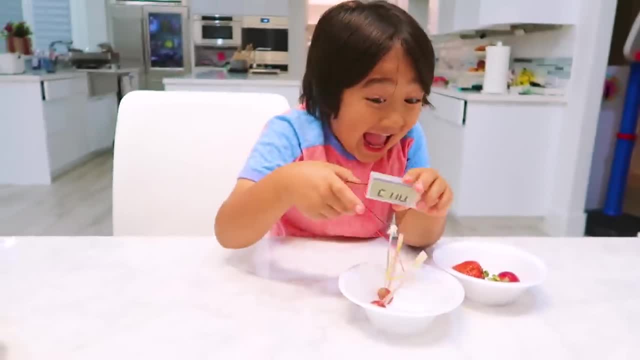 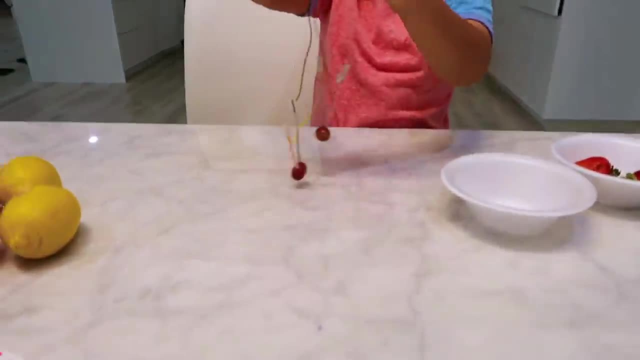 Let's see What It worked. It worked. Grapes can power on a clock. Look at that, you guys. Just two grapes, That's it. that's all we need. Don't need a whole potato, you just need two grapes. 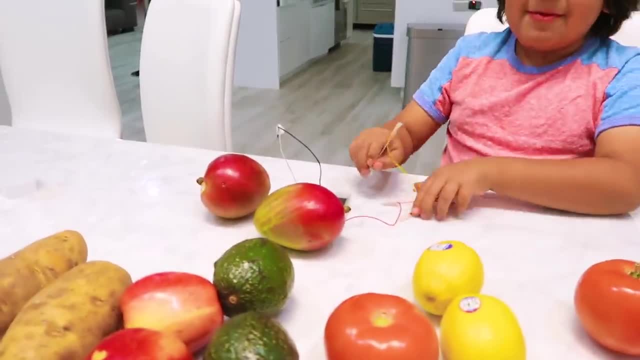 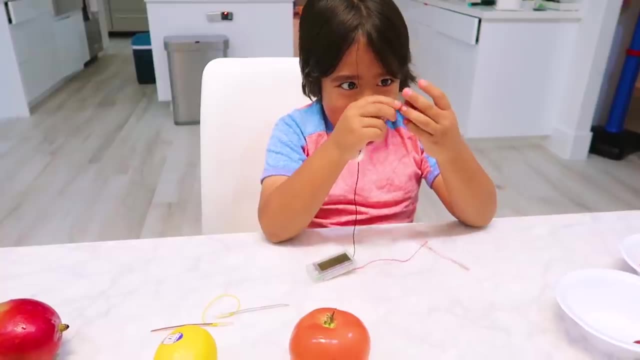 Well, what if you just try one of them? Yeah, With all of them, It's working. Yeah, all you need is one fruit, One grape. it is, It does work. look, It just worked too. We don't even need to complete the circuit. 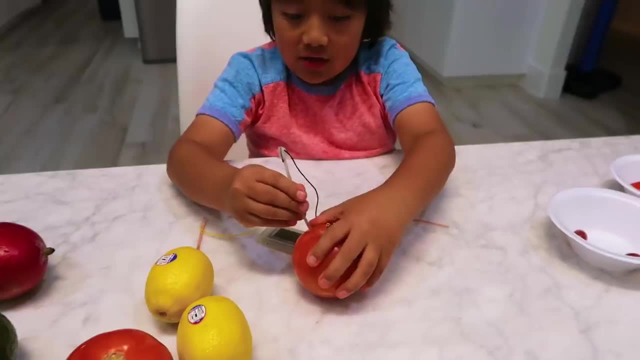 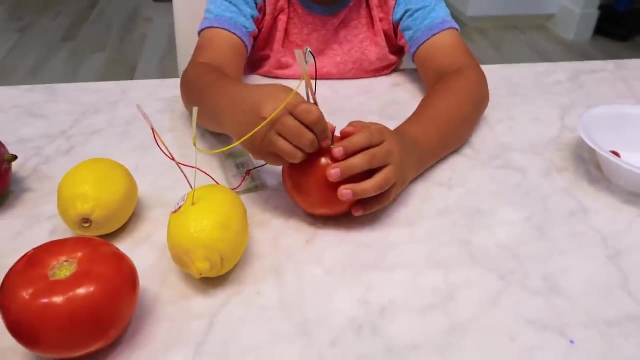 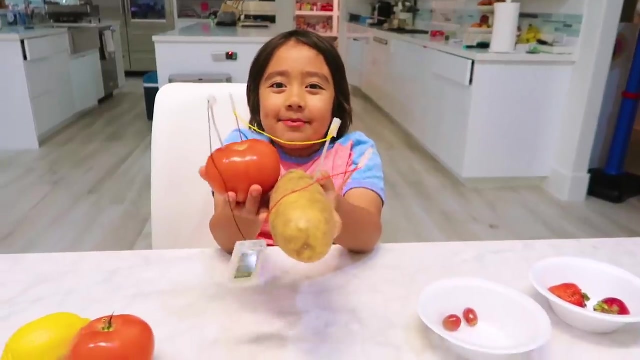 It's so powerful, It's the most powerful. Yeah, I think all you need is one, Ryan Like this. So Ryan's trying out different ones. So one tomato and one lemon, It works, Woohoo. Okay, guys, I'm going to take my alarm clock to bed. 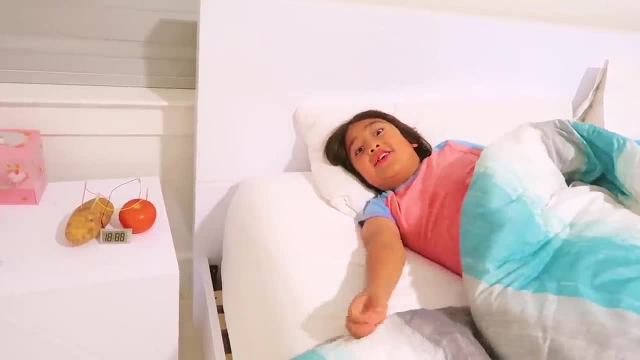 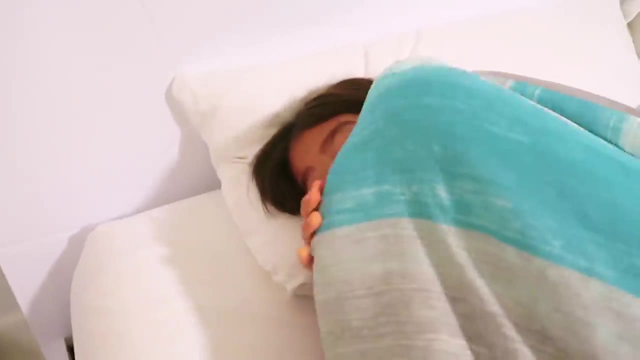 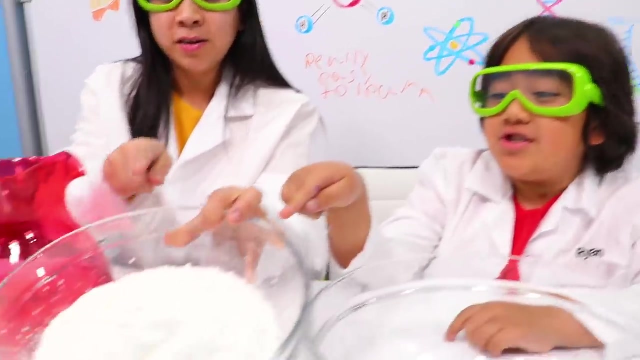 Let's go. Bye, guys. I'm going to go to bed now, And that's how you make a fruit and vegetable alarm clock Bye. All you need is cornstarch and water Aqua. Okay, so you're going to need two full cups of cornstarch. 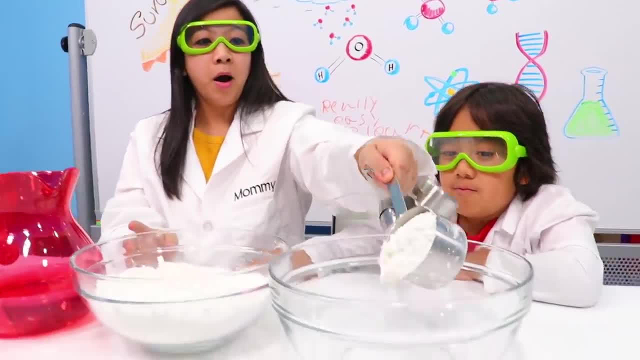 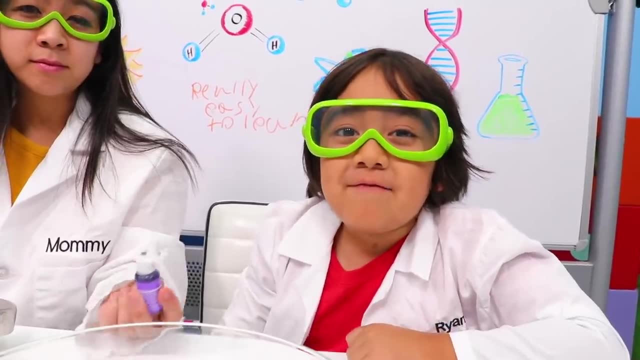 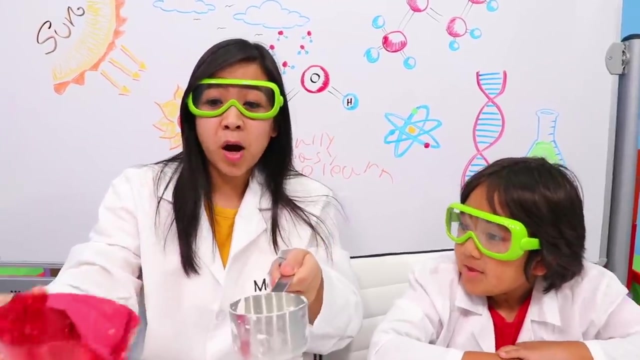 One, One, One, Two. Now my mom's going to put in food coloring for me. This is optional. you can put any color you like. Ryan likes purple And one cup of water. Don't forget: always ask a grownup for help. 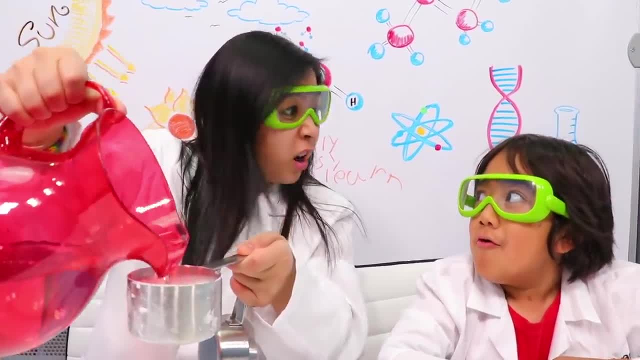 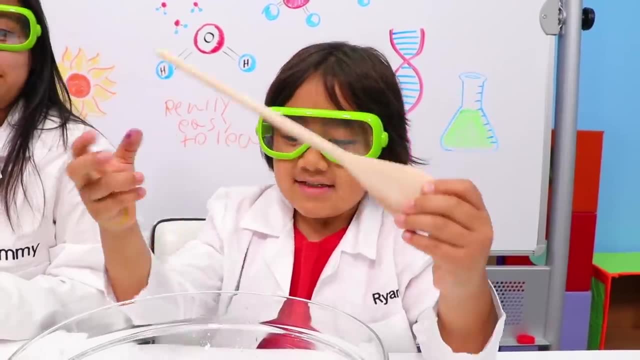 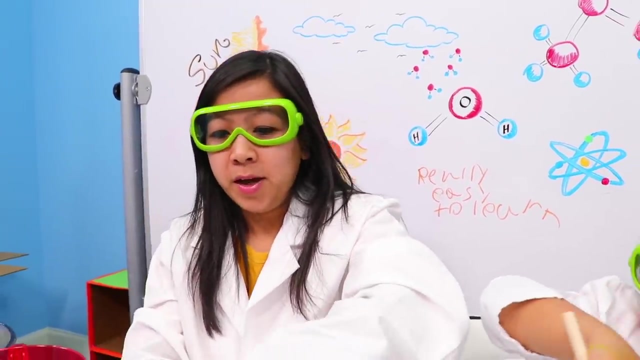 And never eat your science experiment correct. Yeah, Here we go. Time to mix. Okay, so while Ryan's mixing, I'm going to actually make my own so I can pick different colors. Again, two cups of cornstarch. 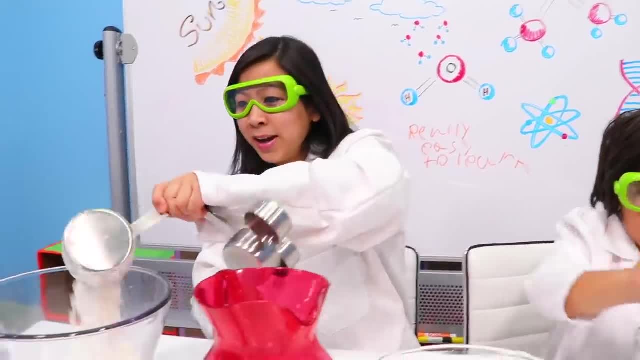 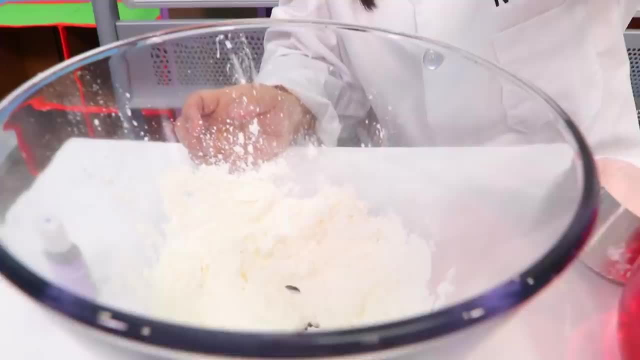 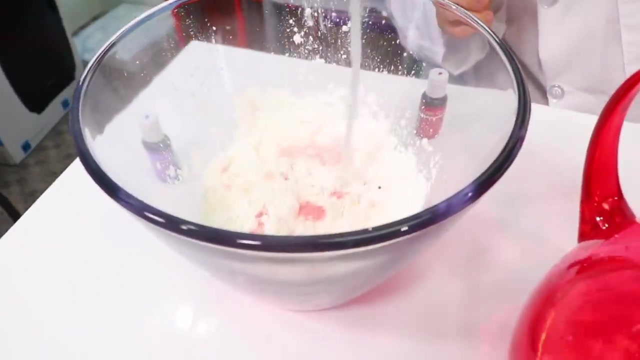 One, Two, One, Two. I'm going to pick red Red Wee- Okay, and one cup of water Wee- Oh. look, it's looking red already Time to mix. We're having an agitating mixing party. 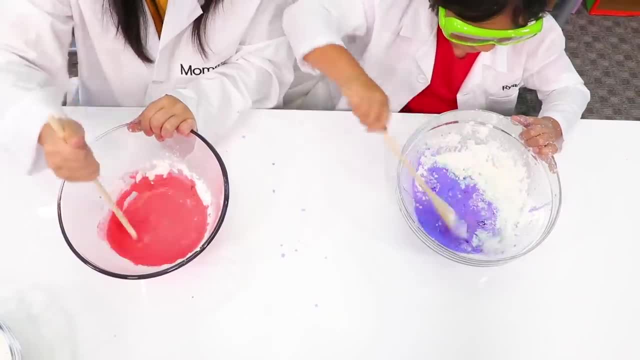 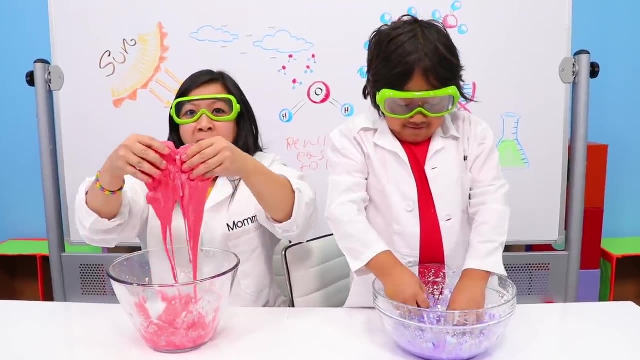 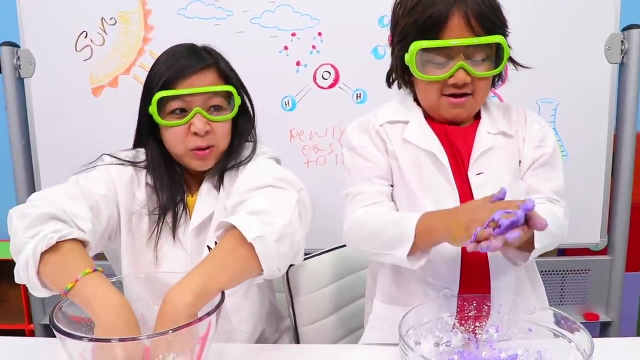 Mommy, it's already kind of working. Oh nice, yeah, Wow, Okay, it's done. Whoa, Whoa. Look at this, It's like slime. Yeah, It's so liquidy. I'm going to make a ball. 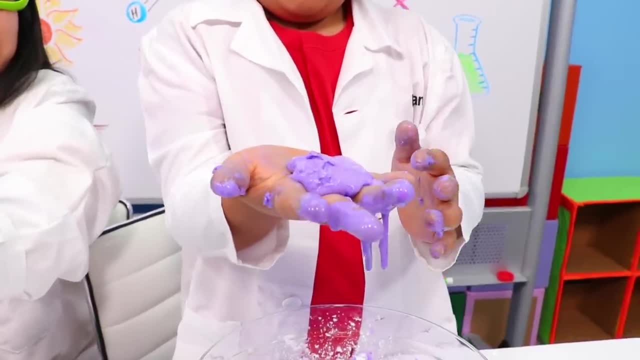 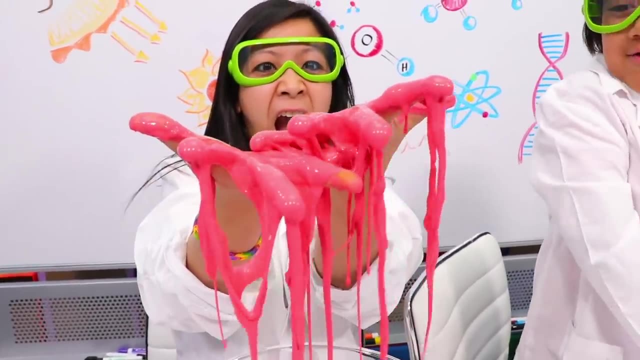 Now I have a ball. Oh, it's melting ball. Whoa, Whoa. Look how it's melting through my fingers. Yeah, it's so cool. How much can you pick up? Ryan, I can pick up a lot. 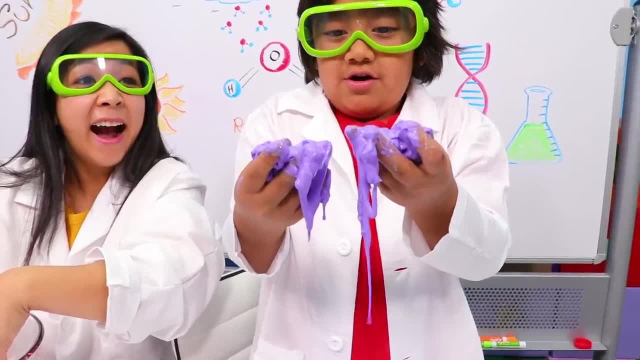 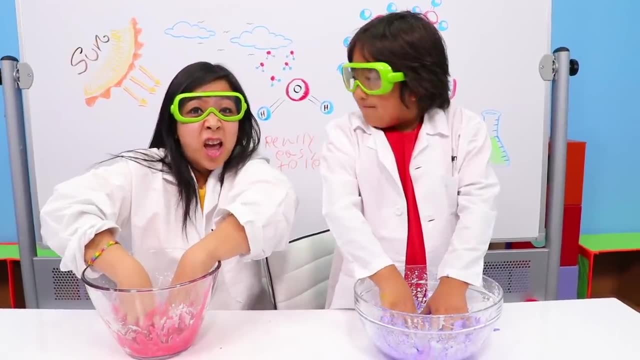 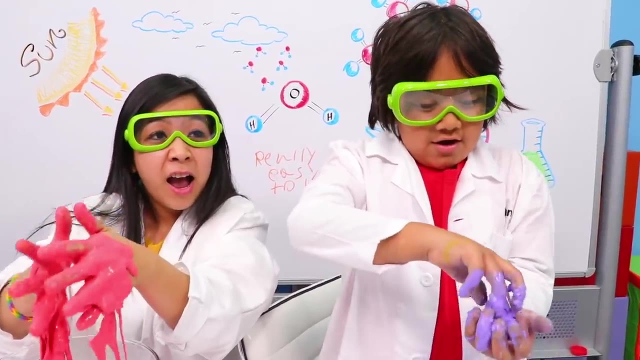 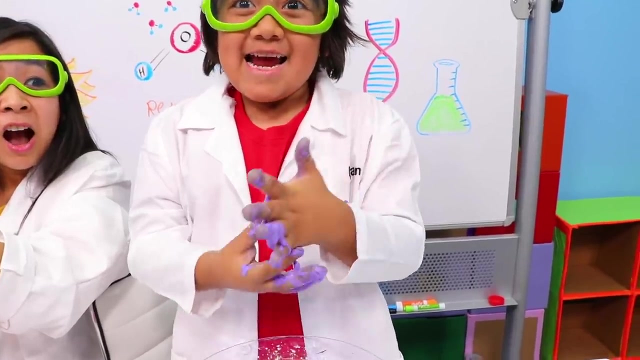 Whoa, Whoa, Whoa. that's so cool, Cool. Hey Ryan, do you know if oobleck like this is a solid or liquid? I think it's a solid And it's a liquid. It's called non-Newtonian fluid. 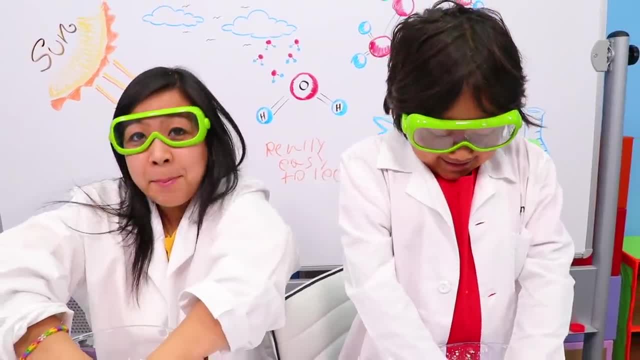 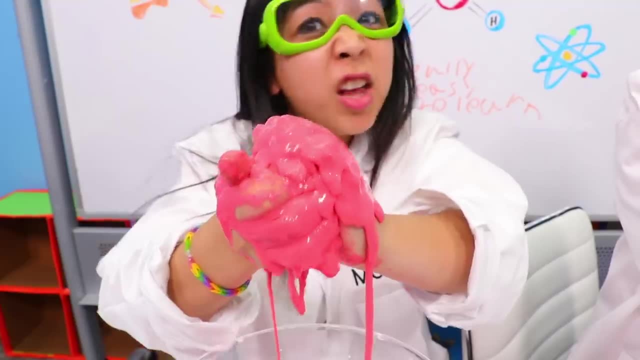 Oh, so Ryan already knows. So what happens is when you pick it up, it flows down like a liquid, right. If you squeeze it really hard, it feels like a solid. Yeah, I'm trying to pick it up like really weak. 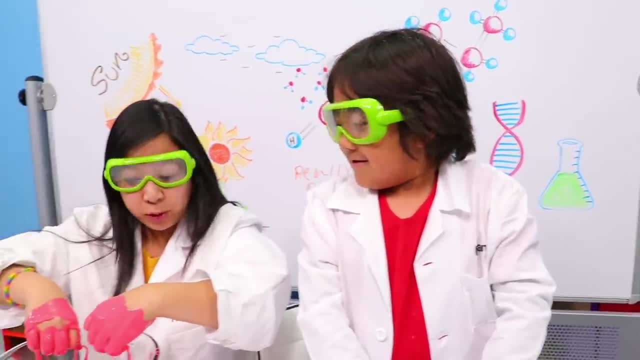 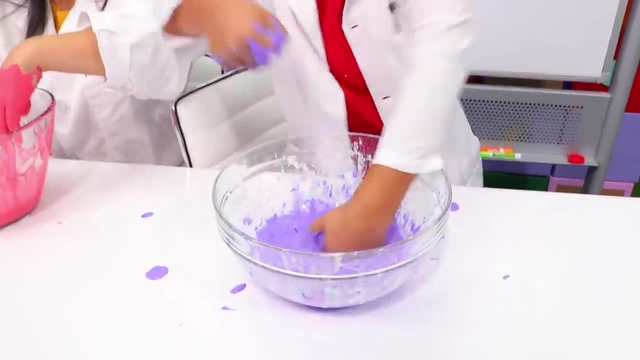 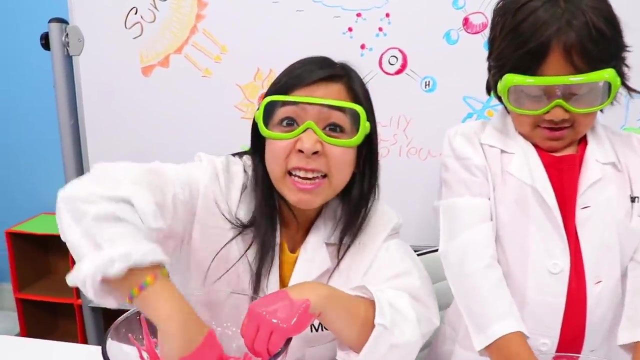 and using barely any energy, and it's really easy. Why don't you try to punch at it? and what does it feel like when you punch at it? Boxing gloves? It's really hard to punch. It is because it's a solid Yeah. 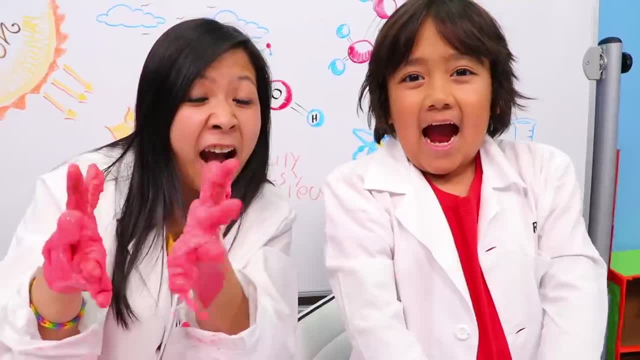 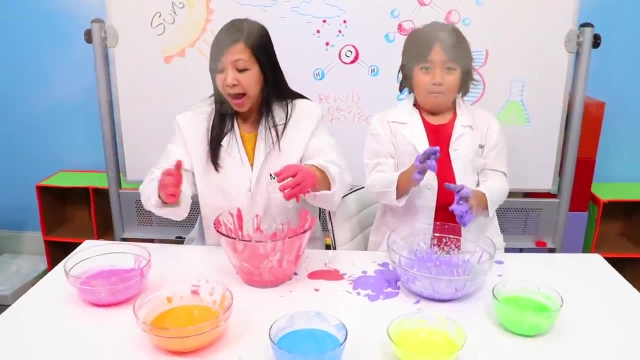 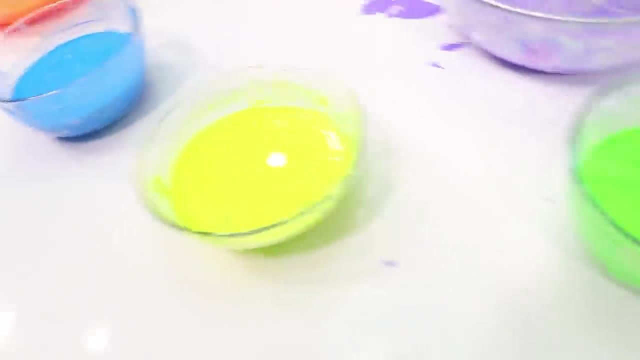 Okay, Ryan, are you ready to make other colors? Yeah, One, two, three snap. So there it is. We made all different color oobleck. So we got pink, we got orange, we got blue, we got yellow. 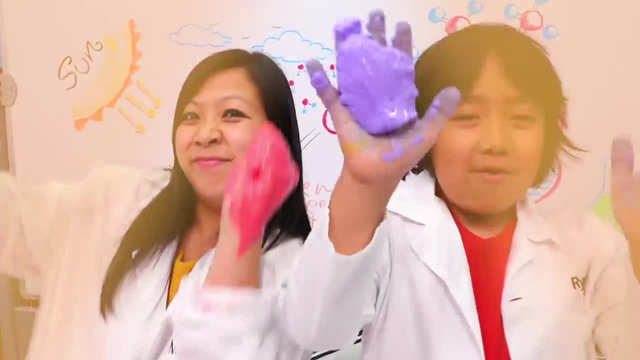 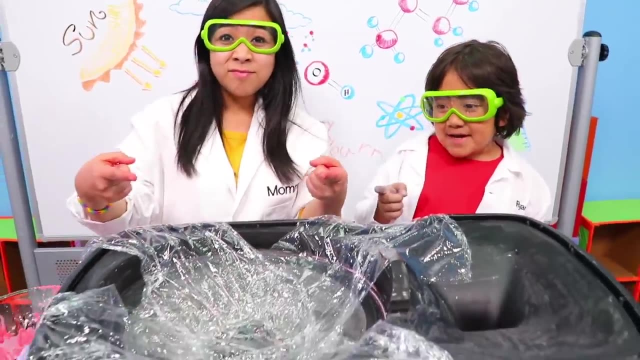 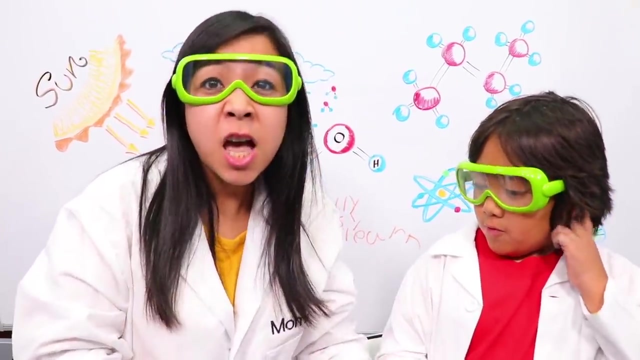 and green. Now let's make a vibration party. Okay, guys, we got a giant speaker, Yeah, so we're gonna need something with a lot of bass so we can see the oobleck vibrate. Now, before we begin. 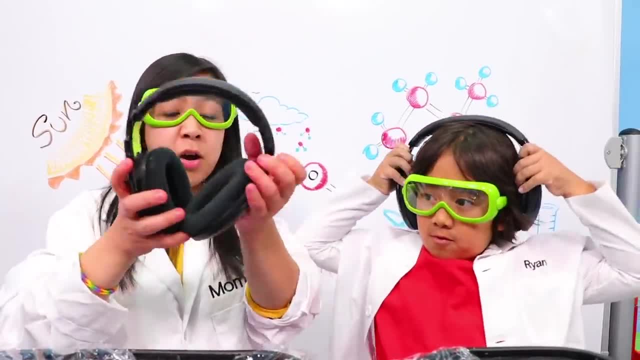 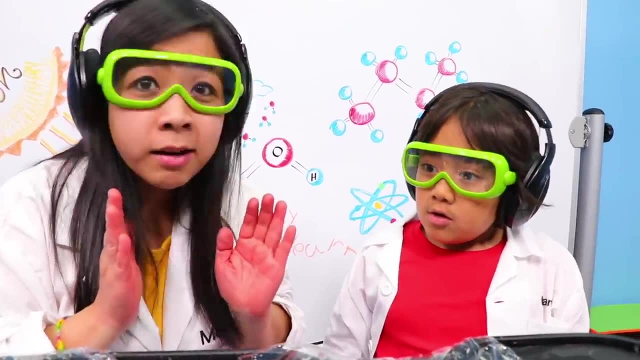 the music's gonna be very, very loud. So there we go, Get noise cancellation headphones. Okay, Ryan, do you even hear me? Ryan, Oh, he doesn't even hear me. Okay, guys, let's get the oobleck. 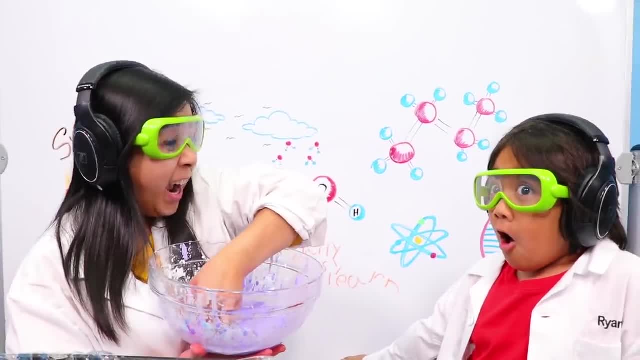 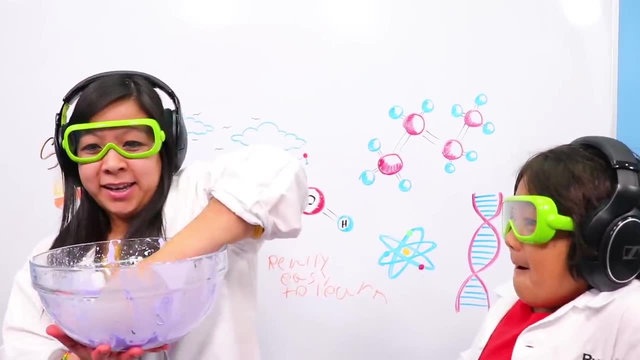 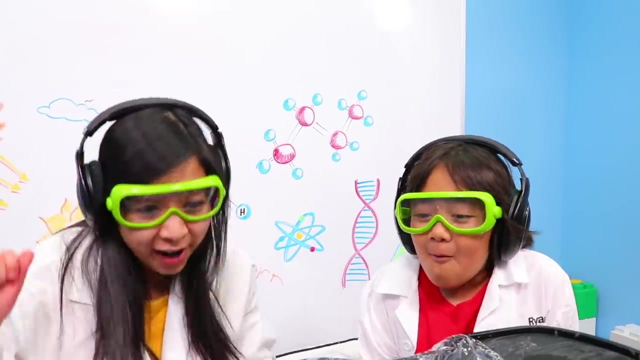 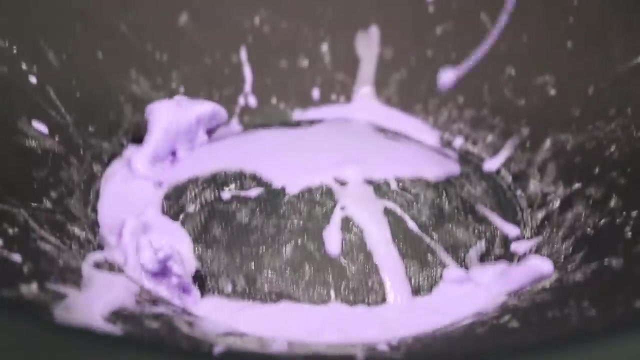 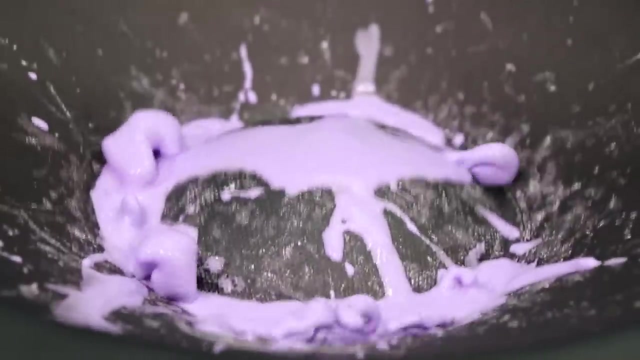 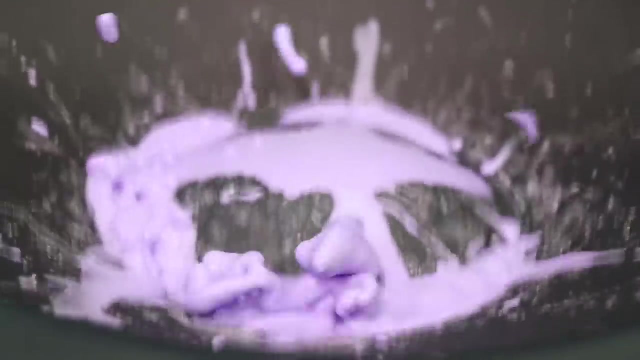 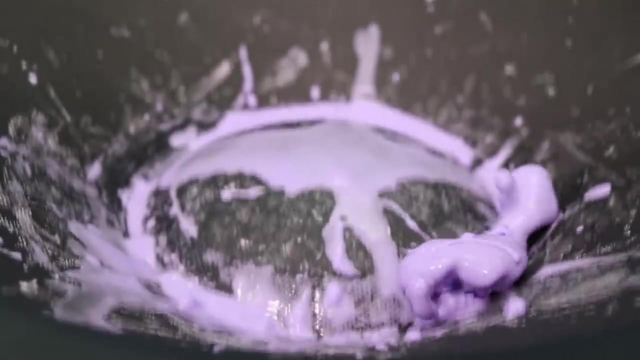 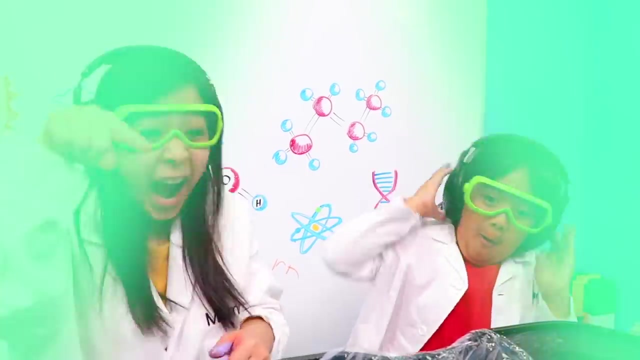 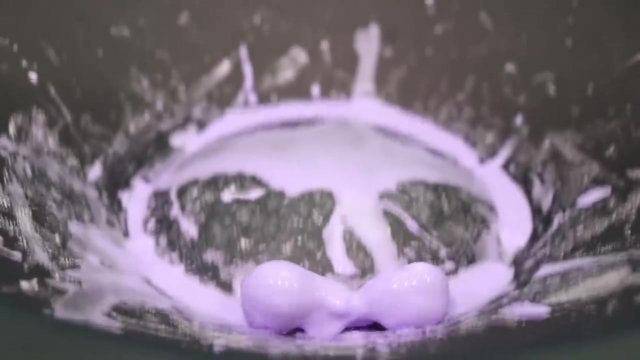 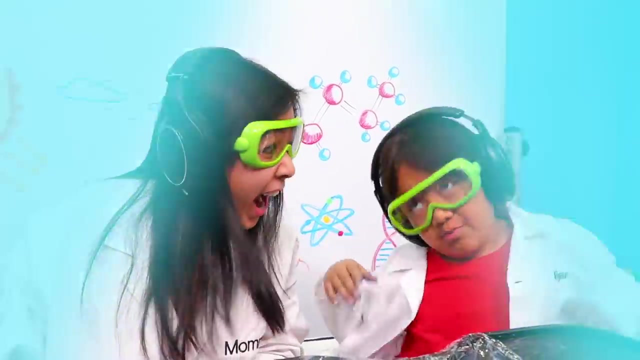 and let the dance party start. Are you ready? He's ready. Okay, here we go. I'm pouring it in. I'm so excited. Okay, Whoa, Whoa, Whoa. It's like this. All right, music stop. 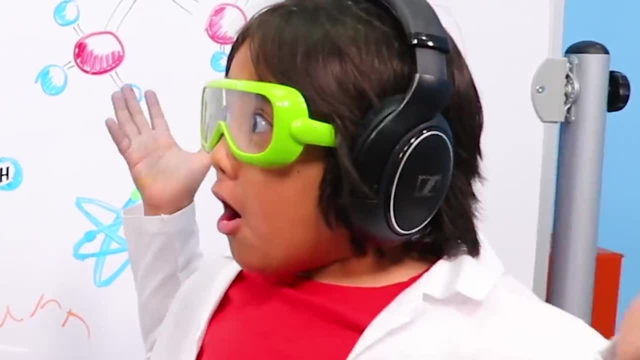 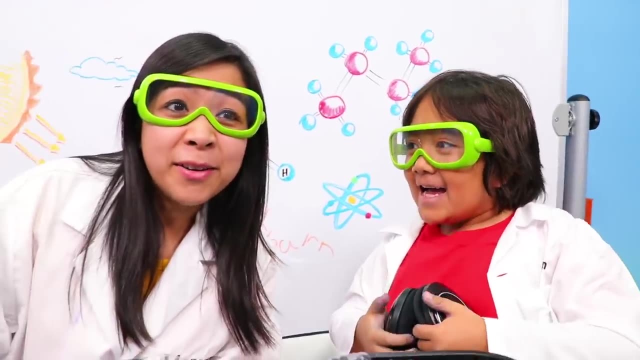 Okay, that was like so cool, Ryan, you can take off your headphone now. Take off your headphones There. do you hear me now? Yeah, Okay, guys, that was like the most amazing thing. We're gonna clean up and we're gonna test out. 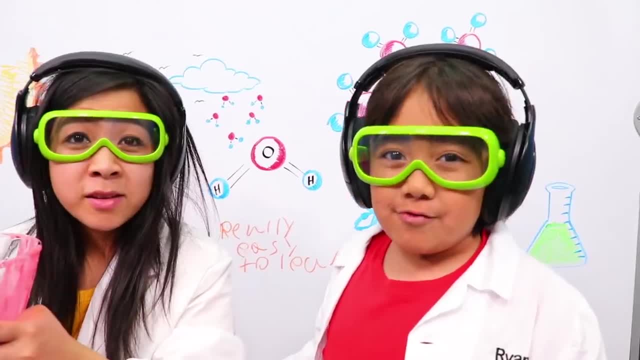 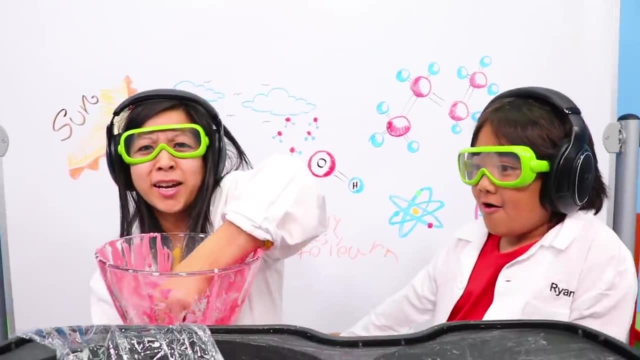 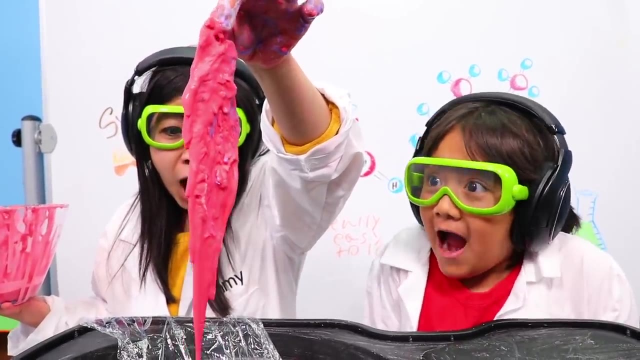 mine. okay, Now we're gonna try out the red. oobleck. What, What Red. Okay, all right, guys, let's get the party started again. Here we go. Whoa, Wow, Whoa, Look at that.